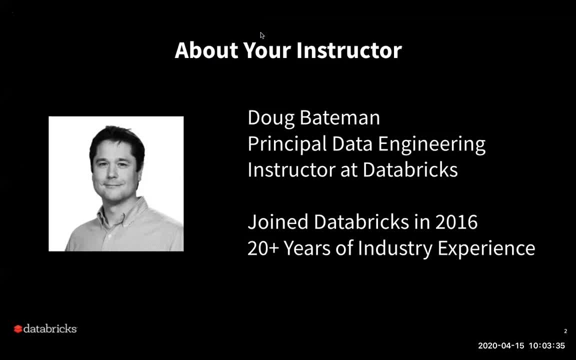 four years ago and in Databricks time that is an eternity. Back then we were roughly 50 people and now we are significantly larger than that in the several thousand. We are growing very, very quickly and really taking the internet by storm. With that said, I have roughly 20 plus years. 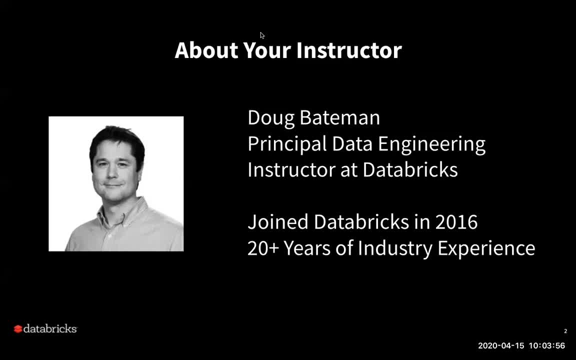 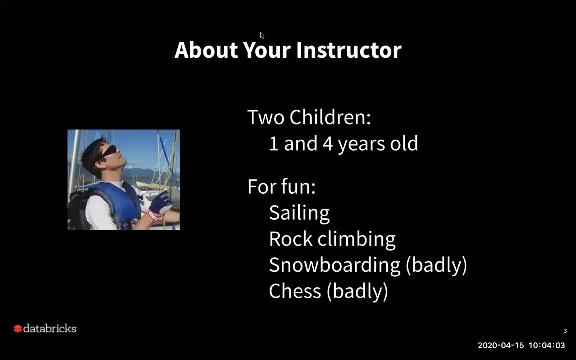 experience architecting and delivering large systems, as well as training and consulting, and I always like to introduce myself as a human being as well. So I have two children, one and four. they're downstairs playing. hopefully we won't hear them, and if they come they'll say: hi. 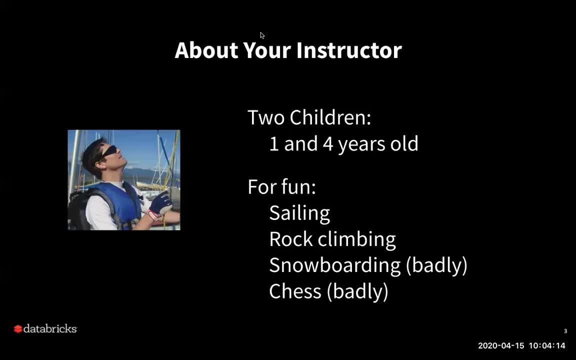 with the working from home And for fun. I enjoy sailing and rock climbing and occasionally we get out to Tahoe to go snowboarding. although I won't claim to be a terribly amazing snowboarder, I do enjoy it, And in my spare time I enjoy playing chess. I'm actually a volunteer administrator at the internet chess club. 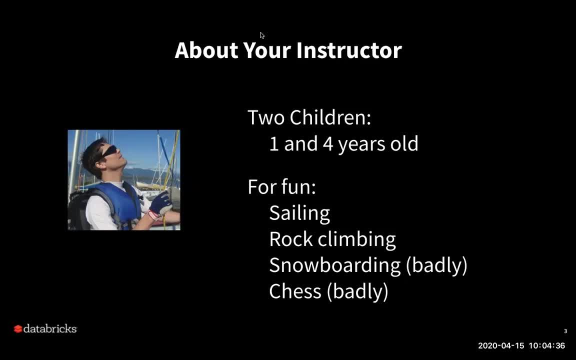 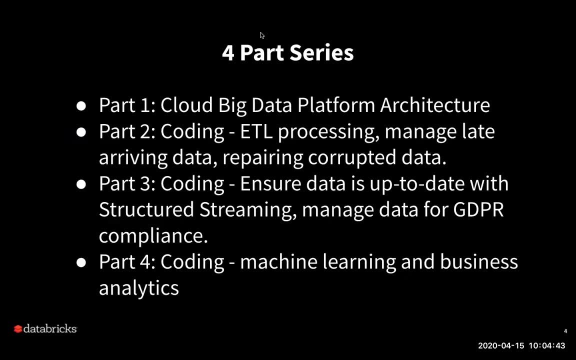 but I certainly wouldn't claim to be terribly good at chess, but it's still a fun hobby of mine. So that just introduces me as a person as well as an instructor here at Databricks, and what I'd like to do is I'd like to introduce myself as a human being and I'd like to introduce. 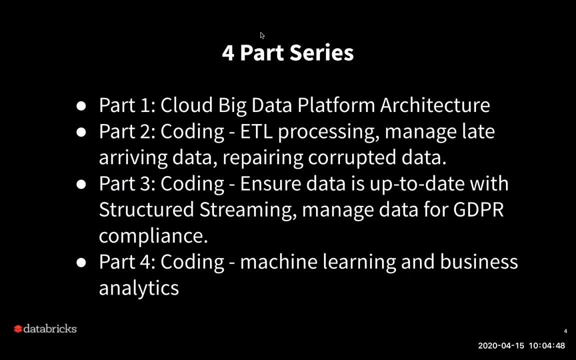 myself as a human being as well as an instructor here at Databricks. so the first thing now is to introduce these series. this is part two of our four-part series on how to build a cloud data platform. Yesterday, for part one, we talked about the architecture. Really, what does a cloud data platform look like? what are all the tools involved? what does the processing pipeline look like? 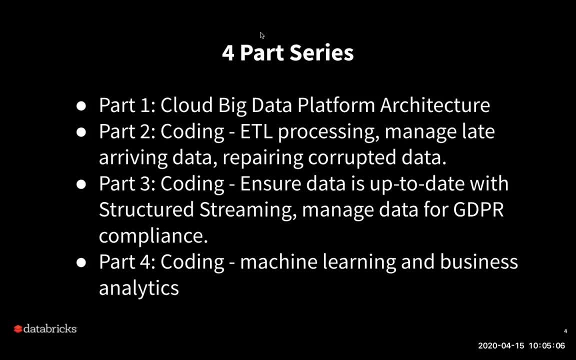 and we set up the big picture so that today we can dive in at a coding level and actually start constructing such a pipeline. And the construction of our pipeline will take up parts two and three of the course of the conversation, and I just want to let you know that it is now the end of the five minutes and we have another one on the next few minutes. 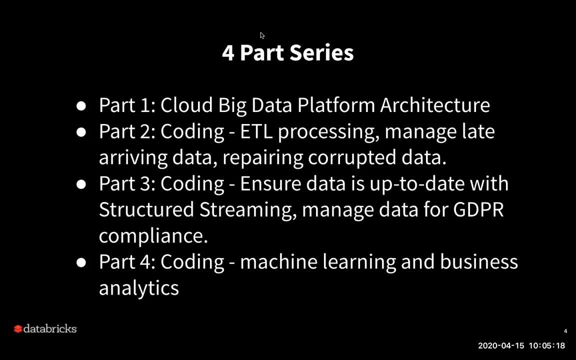 of this series. So we're going to get as far as we can today and then we'll continue with it in part three. So today we're really targeting doing ETL processing and loading the data into our pipeline. So we'll read some JSON files. we'll upload them to Databricks. read some JSON files. 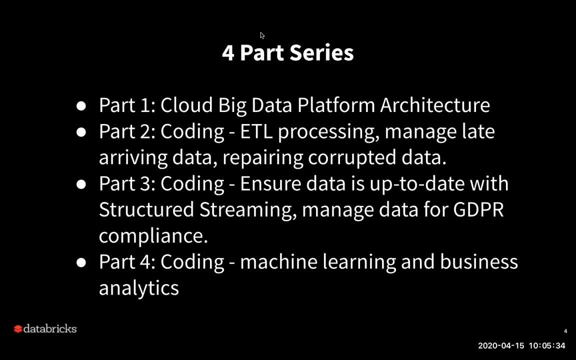 write them out first as parquet, and then we'll actually convert our parquet files into delta tables instead for higher performance. And then we'll start dealing with other challenges that come with ETL, For example, dealing with late arriving data or repairing corrupted data, which 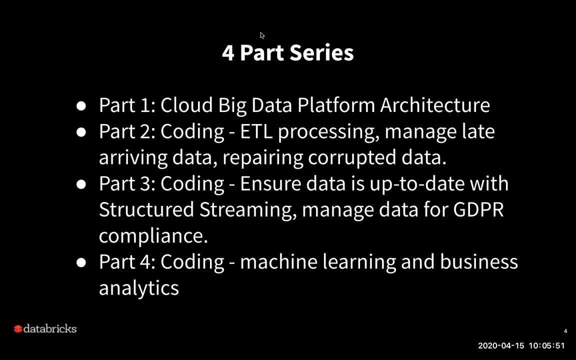 are standard challenges that people deal with when they're building their data warehouse and doing ETL. And then part three. we'll continue with that and we'll introduce the structured streaming component, And structured streaming is incredibly powerful because it allows us to work on deltas. 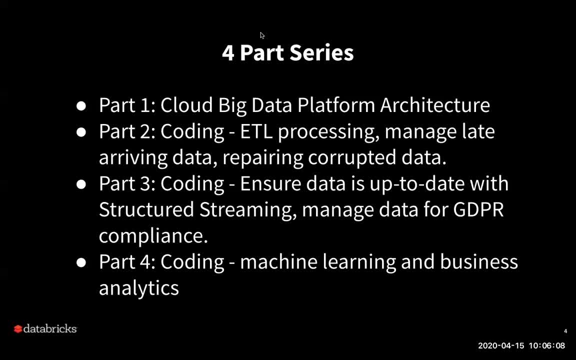 what's changed in each table. So rather than having to read the entire table, I can say read what's changed since last year- Last time I ran this job and process that- And so we treat this as a constantly changing streaming source, reading each table and writing to the next table downstream. 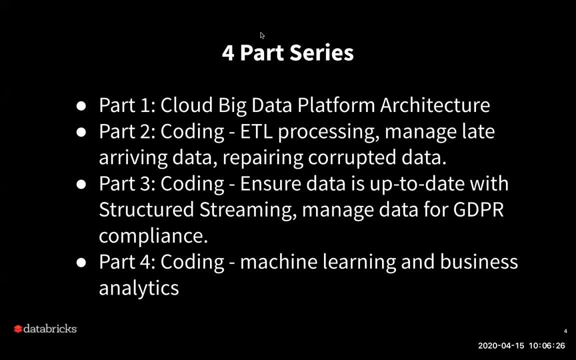 And then we'll also work with some of the capabilities of delta when it comes to accessing past versions of the data. and how would you scrub past versions of the data for GDPR compliance, GDPR being the European regulations for privacy? And then part four is where we're going to look. 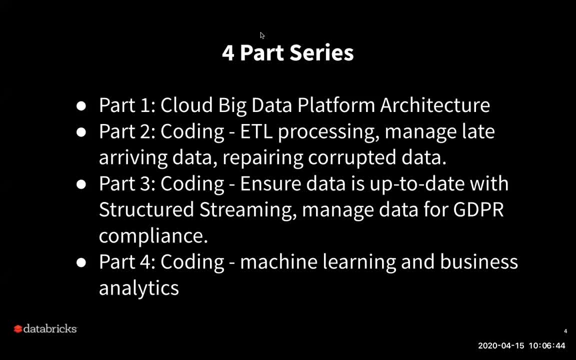 at downstream consumers. So I want to get into the data lake. So these people will be doing, for example, machine learning. So I want to consume the data lake that I've spent all this time doing ETL into, And now I want to build machine learning models and track my experiments using ML flow. 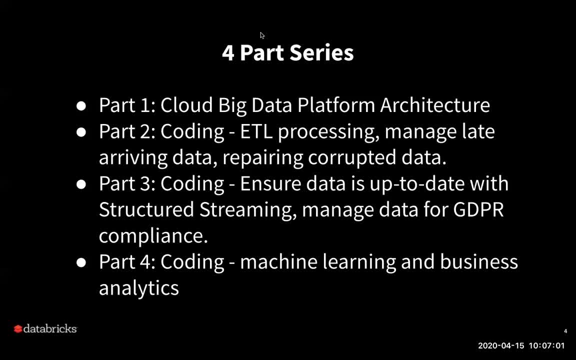 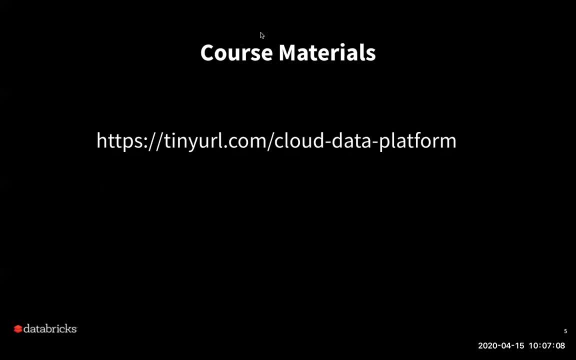 Or maybe I want to use a business intelligence tool to run SQL queries against my data lake, And so that will be part four of this four part series on Friday. Now a number of people have asked where can we go to get data? 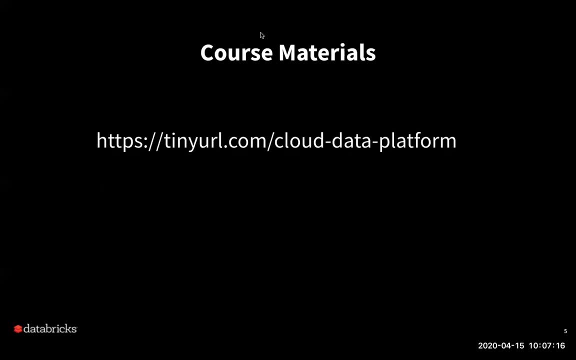 How can we get access to the materials that we are using for this course? And the answer is: we're uploading them to this website here, tinyurlcom- slash cloud dash- data dash platform, and if people ask in chat, That's the link that we're going to send you to as well. In fact, I'm going to hope I can't copy easily. 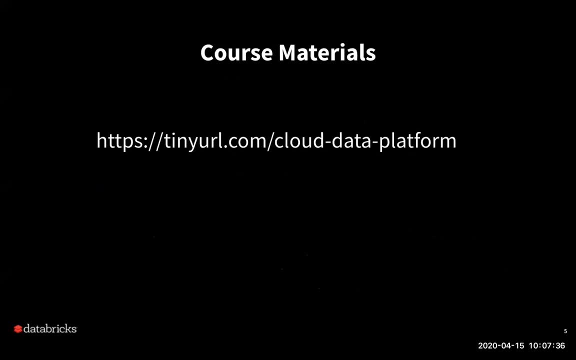 But tinyurlcom slash cloud dash data dash platform. Let me go ahead and type that into the chat area. It is. if I can successfully get access to the chat area, Here we go. I found out where it's hiding And you can go here to access the data at any time, And we will be. if I create notebooks and things of that nature, we will upload those there as well. So what does that look like exactly? 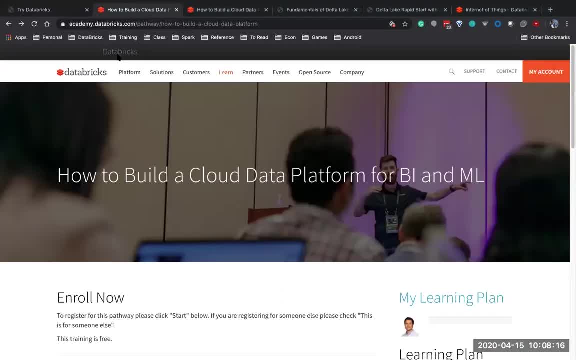 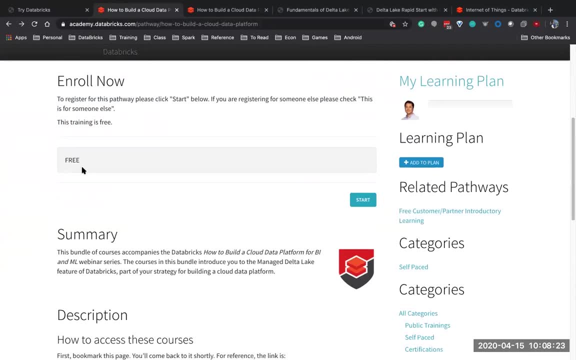 And the answer is: if you go to that URL, you're going to come here to academydatacom slash, pathway slash- how to build a cloud data platform, And we are making it available to people who attend the webinar. So this link is just for people who attend the webinar, That's you. 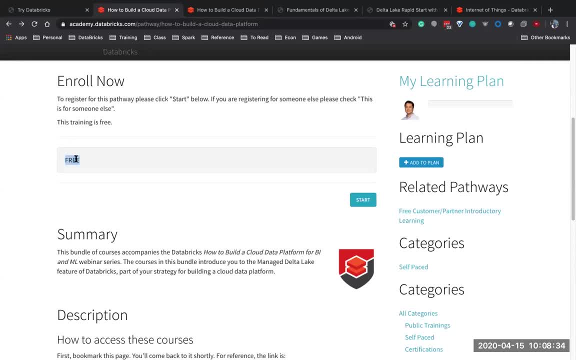 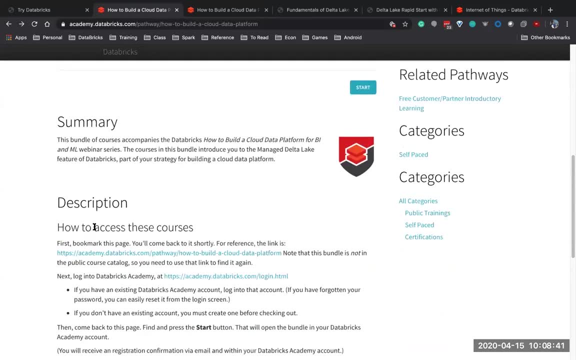 Or if you're watching this recording live or recording afterwards, then you come here and you can get access to what we would normally charge people for, but you get it free because you're here part of the webinar And you can access it for free. 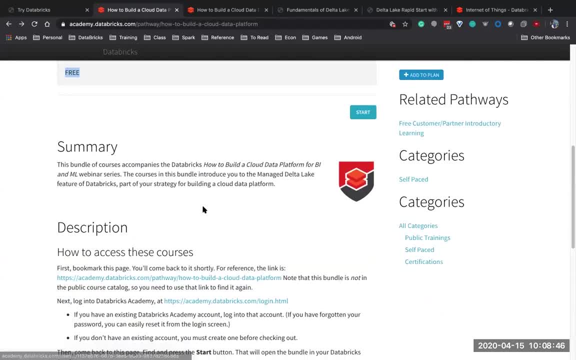 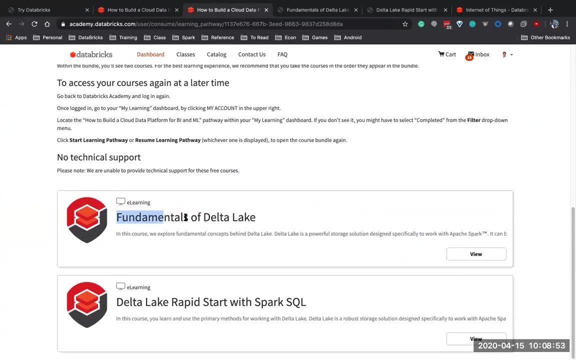 And you can actually sign up and enroll. So you would click Start and you'll be able to enroll in the course And at that point you'll be taken to a page where you have access to both the materials that we used yesterday, which was fundamentals of the Delta Lake. 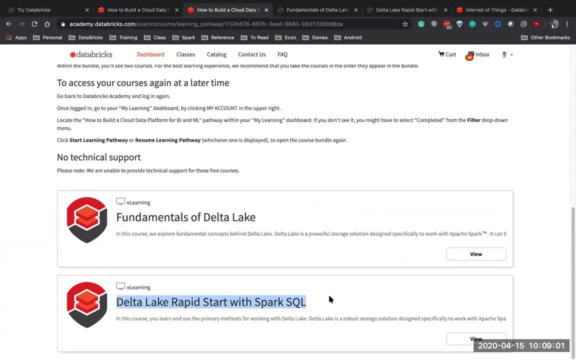 As well as the materials that I'll be using for the next two days here, which is the Delta Lake rapid start, And as we create additional materials, such as the demo notebook that we did yesterday, those will be uploaded to this page as well. So that demo notebook from yesterday- We're working on that. 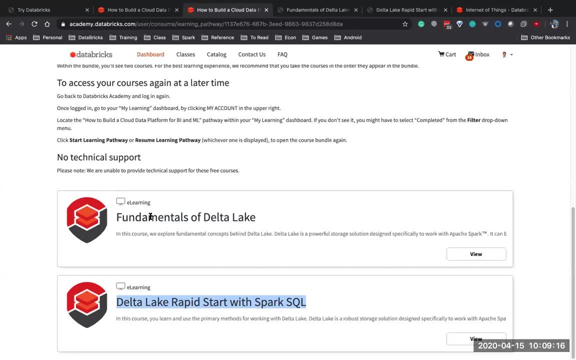 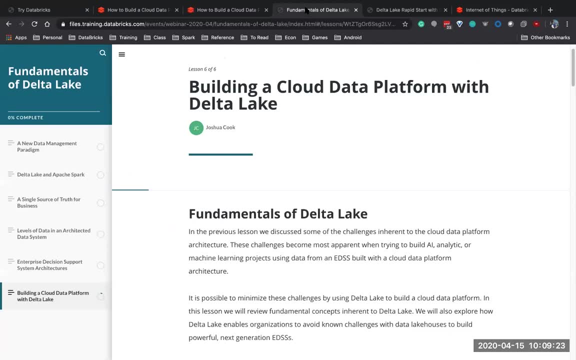 We're going to get uploaded to this website right now, So this gives you kind of an idea as to what's available, And yesterday, as you recall, we had worked with the fundamentals of Delta Lake And that's what you'll be able to get access to by going to this page. 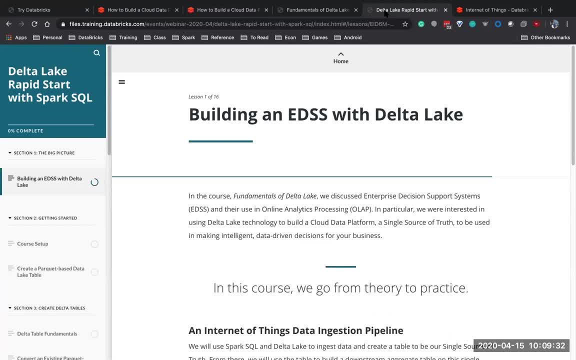 And, similarly, today we're going to be working on the Delta Lake rapid start with Spark SQL. So this is where we're going to be using Spark SQL to construct our Delta Lake. So we're going to be building our cloud data platform, And you're welcome to follow along or simply enjoy the show today while I'm doing the webinar and then come to this web page afterwards to try to do this yourself, which is what I would recommend, because it makes it a little bit easier to pay attention and follow along. 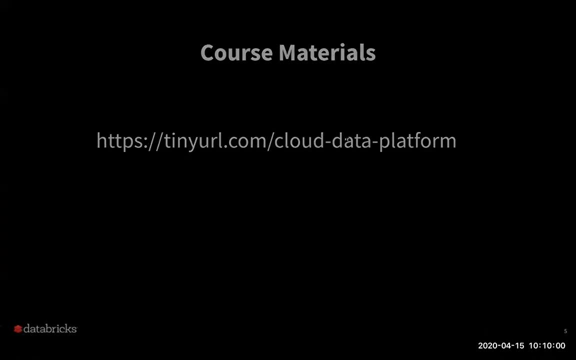 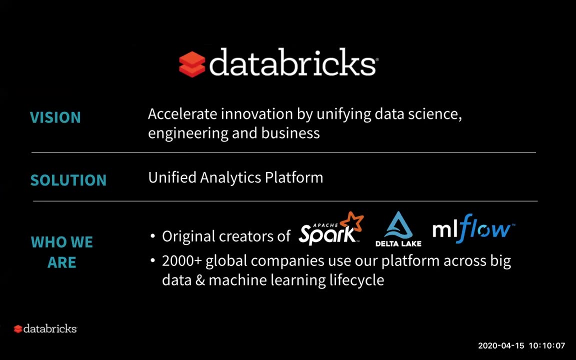 So, with that in mind, let's do a short recap of yesterday. So yesterday we introduced who is Databricks, So Databricks. we are really a big data company. We're the original creators of Apache, Spark, As well as the Delta Lake file format and MLflow. 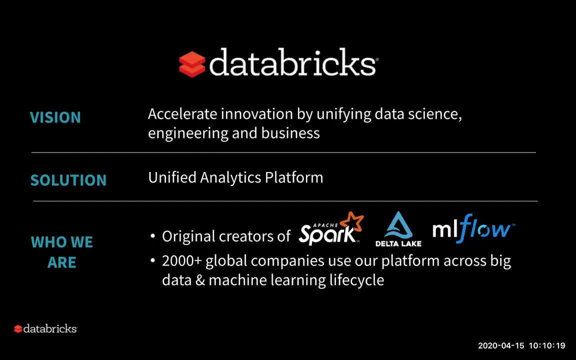 And these are open source projects that are now available to anyone on the internet, with contributors all around the globe. So we don't like to say we're the creators, but it's all the people on the world who have contributed any line of code to one of these projects. as a creator, 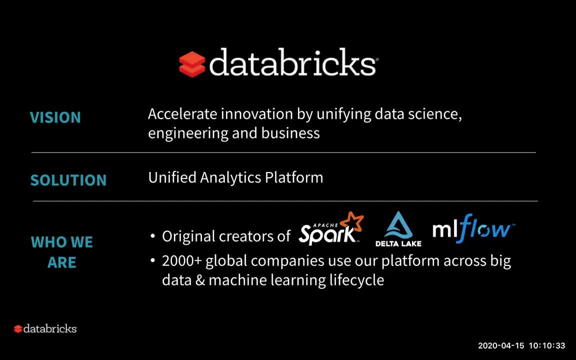 But we were the original creators who put it out there and available online, As we like to say. Spark, I am your father. Okay, that was my attempted humor For our Our morning webinar here. Now, of course, some of you guys are going to be in Europe, so it may not be morning where you are, but it's morning here in California. 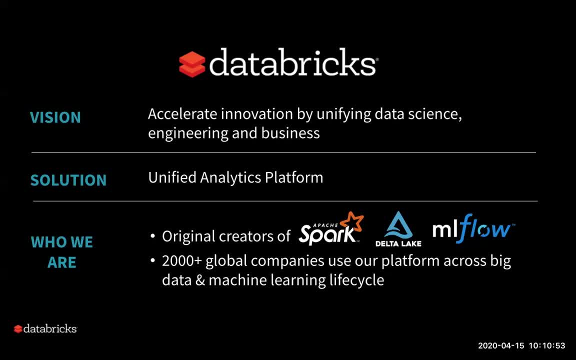 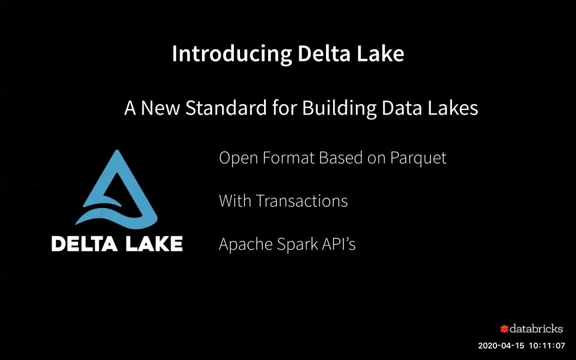 And we have thousands of global companies are using our platform across big data and machine learning, and it is scaling and growing, which is just really amazing, And our goal is to accelerate innovation by unifying data science, engineering and business using what we call a unified analytics platform. 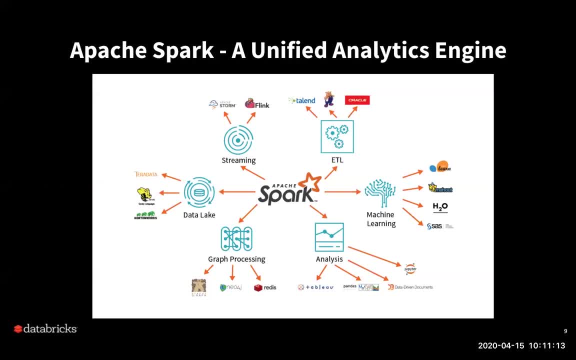 So what is a unified analytics platform? Well, we're going to be seeing it today, But it's this idea that you've got one platform that's able to do a variety of different workloads throughout the data analytics lifecycle. So that means ETLing the data into a data lake or our cloud data platform, which is what we were looking at yesterday on our presentation- the architecture for that. 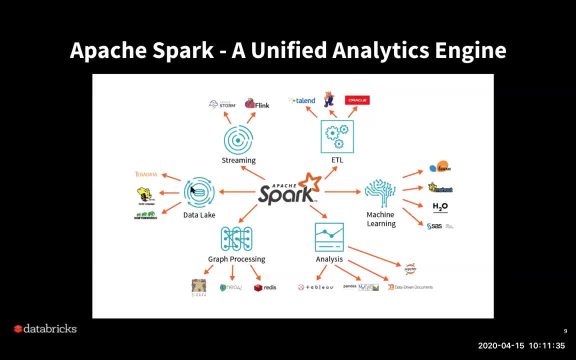 And we'll be doing today. So we construct our data lake that we can then query after we do ETL workloads. And then, once we've built that data lake, we want to be able to do exploratory data analytics. And then, once we've built that data lake, we want to be able to do exploratory data analytics. 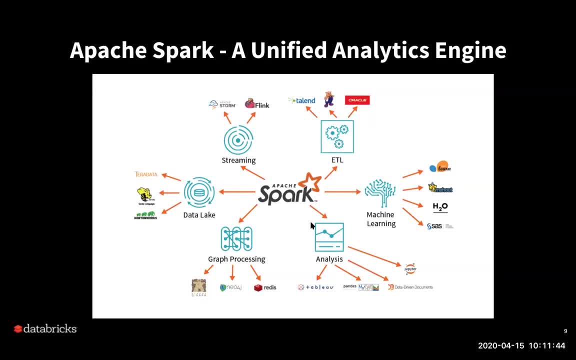 And then, once we've built that data lake, we want to be able to do exploratory data analytics. So you saw that we were able to use notebooks and make plots yesterday and our previous webinar in part one, And as well, you're able to do machine learning activities. 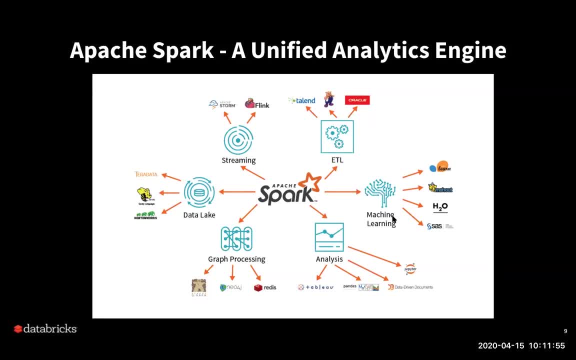 This is what will be a focus of the fourth part of our series doing machine learning, And there are other types of workloads that we can do, For example, updating the data in a continuous basis using live streaming, which is really really cool. 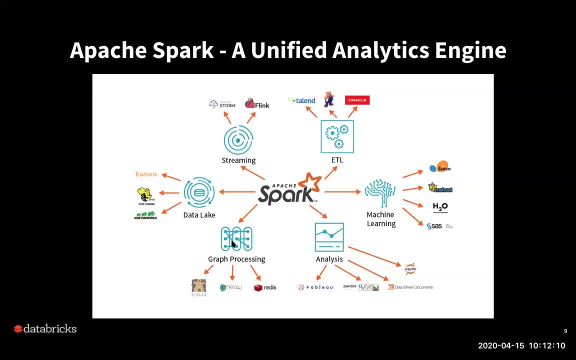 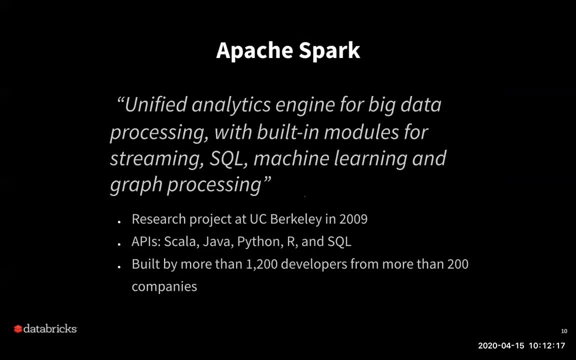 And then graph processing. That's where you have nodes and edges like flights and airports, And you're doing Some type of analytics that goes with that. So Apache Spark again was that unified analytics engine for big data processing with built in modules for streaming, SQL, machine learning and graph processing. 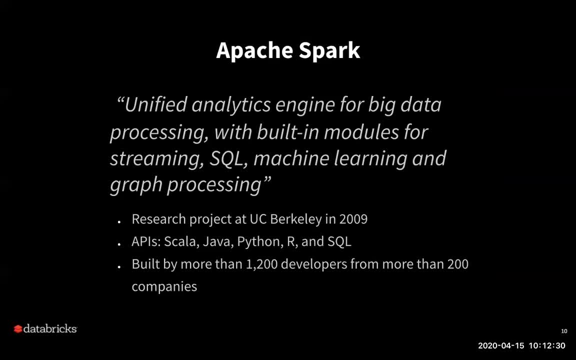 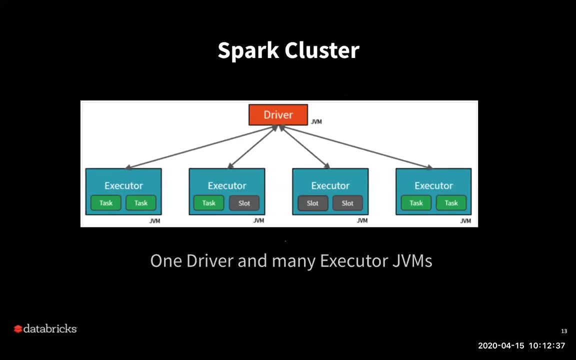 And it started out in 2009, and now it has really become a de facto technology for building our data lakes. We also reviewed just briefly yesterday the way in which Spark breaks up The Data. So Spark works by your code. Your application is running in the driver, and the driver then takes the queries that you write and comes up with an execution plan that, in turn, is divvied up amongst various cluster machines called executors. 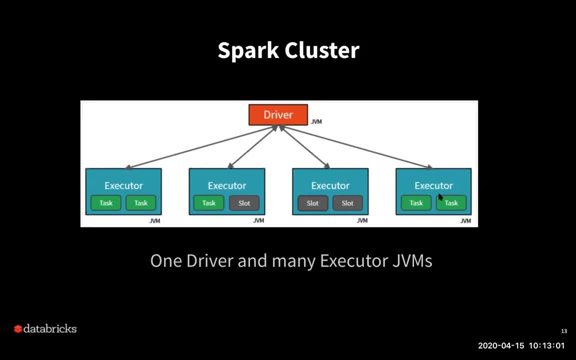 So a cluster consists of a driver and one or more executors that has been used to run our workloads. So one driver and many executors, And the Executors Are, In turn, each run on a piece of the data. So they'll read in some of the data from outside. 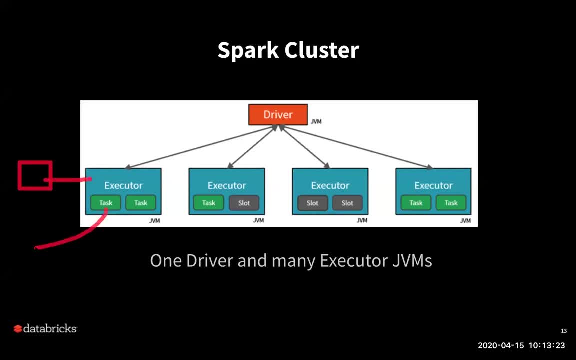 They'll read in data, Process it and write it back out to desk so that no one machine has to deal with all of the data. And this gives us scalability, where we can scale out when our data is too big to fit in a single machine. 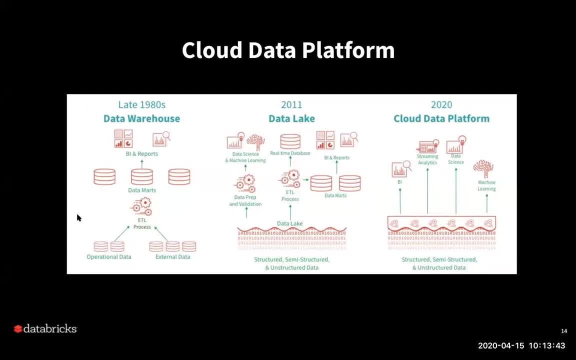 And then yesterday we talked about Where this really fits into the world. And so back in the 1980s people were using software systems and the field of data warehousing really became popular. Bill Inman had written whole books on the idea of data warehousing. 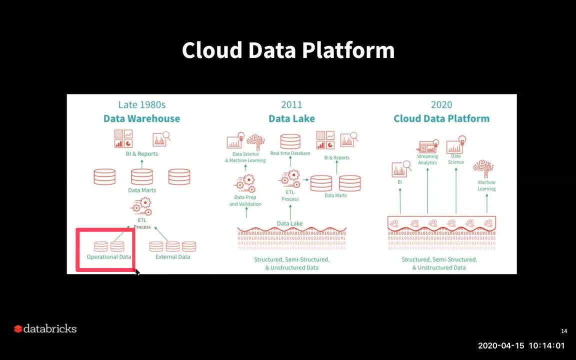 And this is the idea- that I've got all sorts of different data stores that contain my operational data And I may be pulling from other systems as well. So I may be doing snapshots of the operational data In my operational data store, but at some point I want to ETL that data into my data warehouse. 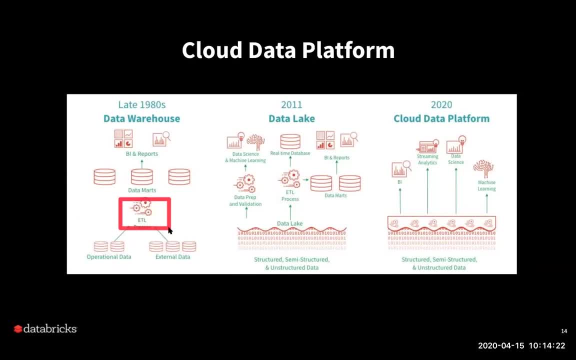 And so our data warehouse is pulling data from all across the enterprise with these ETL type workloads, And there's this entire process where you bring the data, you do load the data in, then you do some data cleansing And eventually you end up with these data marks that are used by departments to be able to do their business intelligence and reporting and the field of data. 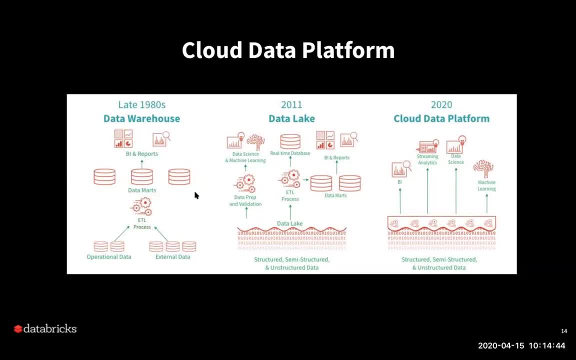 And that's what we call. data warehousing is incredibly popular when it comes to analytics, but there's challenges that we need to address, such as scaling up these software systems, As well as the diversity of file formats that we have to deal with. 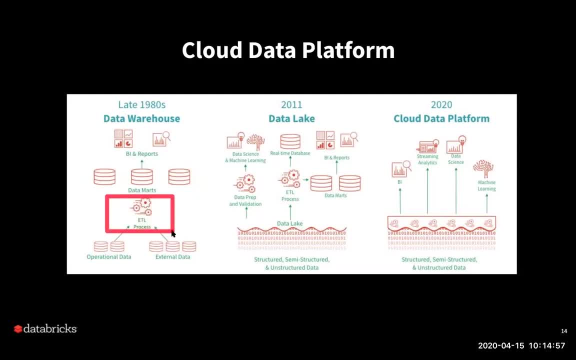 So a traditional data warehouse required that we set up our enterprise schema. It's highly structured And, as a result, there's a lot of work that was required to do the ETL upfront before we could start getting any types of insights. And so, with the advent of Hadoop, 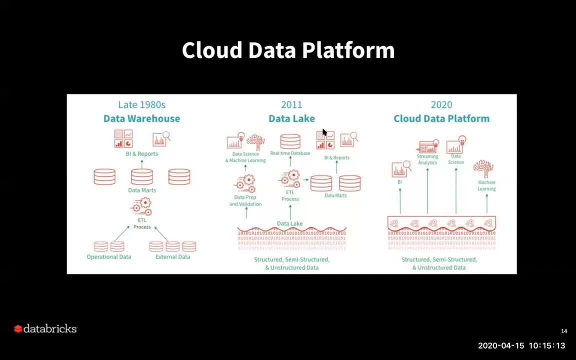 the data lake had become a really popular platform, And the idea of the data lake is that we simply store this data initially, as it's being exported into a really large storage bin. So we could be using cloud storage systems such as Amazon S3 or Azure Blob Store or Azure Data Lake Store. 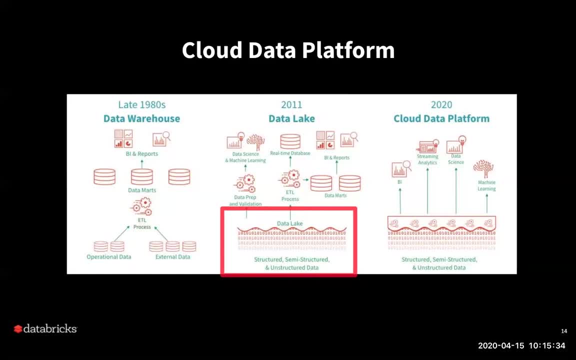 But what we're really doing is dumping this data out there so that it could be used and available for people, and we don't worry about cleaning it up front, We're simply capturing it. So we're getting it out of these systems and we're capturing it, but we delay the cleansing. 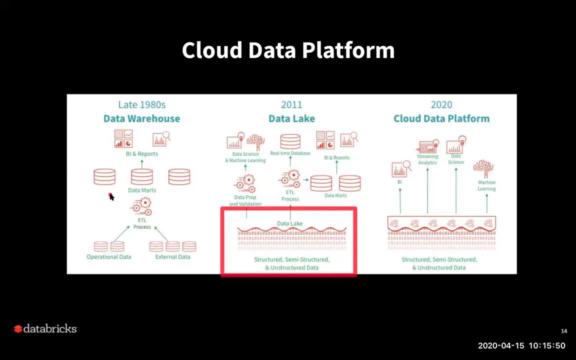 And the reason we delay the cleansing is that if we tried to do all the cleansing upfront, we would spend all of our time doing cleansing and people would decide that it was just too hard to use our data warehouse Because we spend so much time doing data cleansing and therefore we're just not going to bring in the data in the first place. So the idea is, no, let's just capture the data as it is. 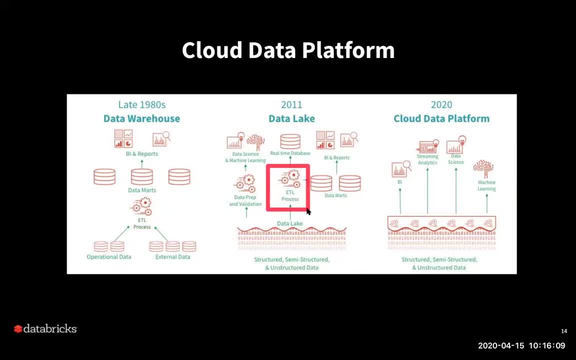 And then start doing ETL workloads On that data data later when we're actually interested in it. So you clean the parts of the data that you actually are interested in and you bring it into these data marks, which can be a data warehouse. 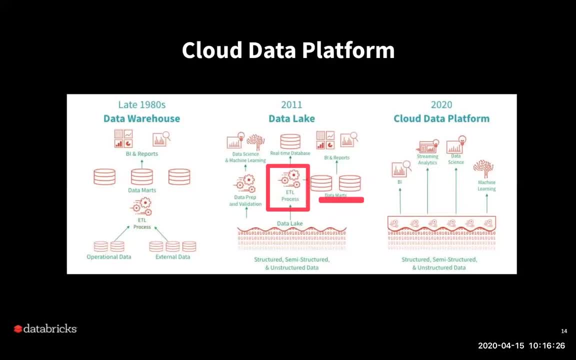 or it could simply be tables that are part of our cloud data platform And then you do your reporting and analytics on that. Now the cloud data platform takes this data lake paradigm from Hadoop and goes even further and says: let's use Apache, Spark and 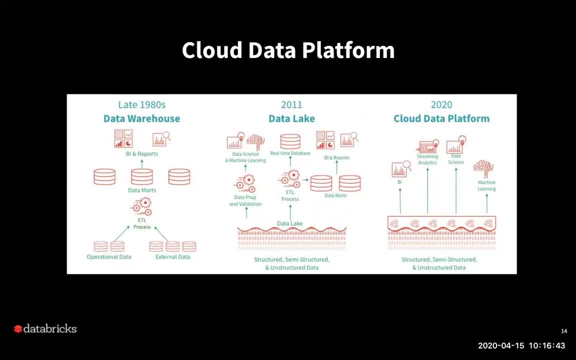 let's actually have our cloud data platform store all of the data And let's actually store it in the cloud where we've got this elastic compute and elastic storage. So we're going to have the cloud data platform keep everything And, in fact, when it comes time to do things like data marks, 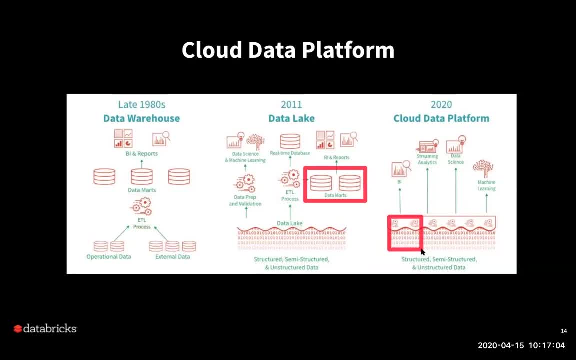 we'd really like to see if we can use Spark to be the data mark, that is, the consumer part of the data warehouse. But if I need faculty, I might still end up having a data warehouse in here as well. in terms of just reducing the response. 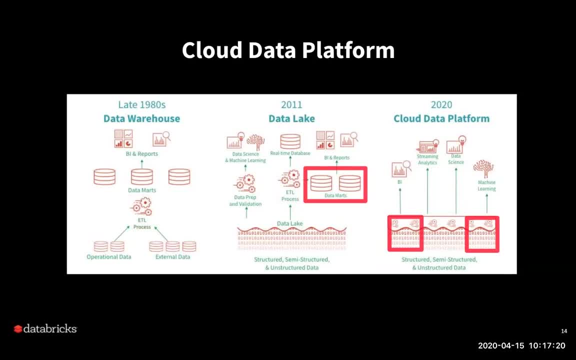 time for interactive queries, because there is a little bit of a latency when you're working with something like Spark and our cloud data platform. But for the bulk of the ETL, we really want to use the cloud to do this and host this using Apache, Spark. And so what does that look? 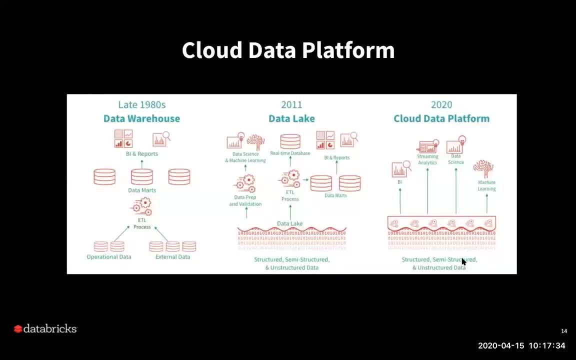 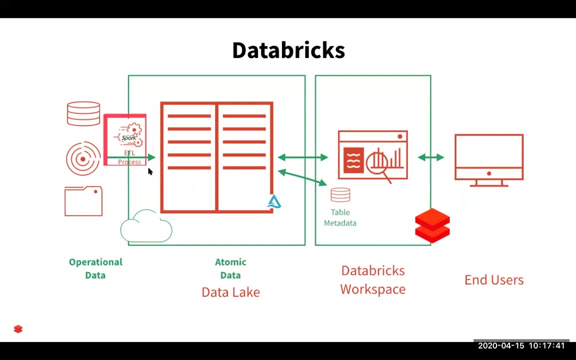 like exactly. So oops, there we go. So what this looks like is that we're using Apache Spark to do ETL workloads from all of our various sources of data. This could be our operational data store, where we've got snapshots and various systems, or this could be pulling from. 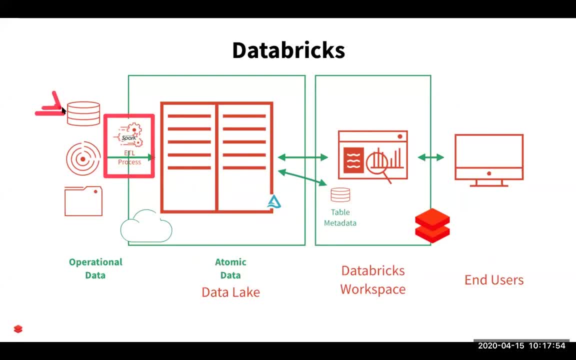 the actual systems themselves And as we pull data from the various systems, either by streaming or by reading from databases or just file formats that have been dumped into a directory. we're going to ETL that and we're going to talk about the layers again in just a moment. 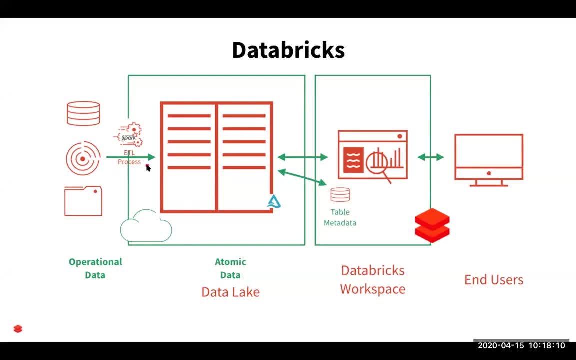 but we're going to ETL that into our data lake Using a really powerful query engine like Apache, Spark, And then we're going to use an interactive notebook environment like a Databricks workspace to be able to query that data and extract insights So our end users can log into the workspace, begin doing those types. 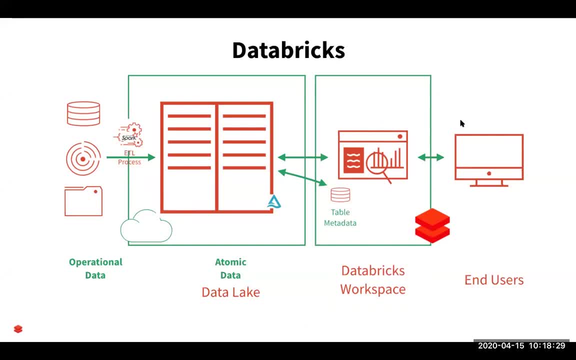 of queries. Additionally, an end user might prefer to instead use a tool like Tableau, And Tableau in that case would just be sending JDBC queries to Databricks which in turn would be servicing those queries from the actual database. So we're going to use an interactive. 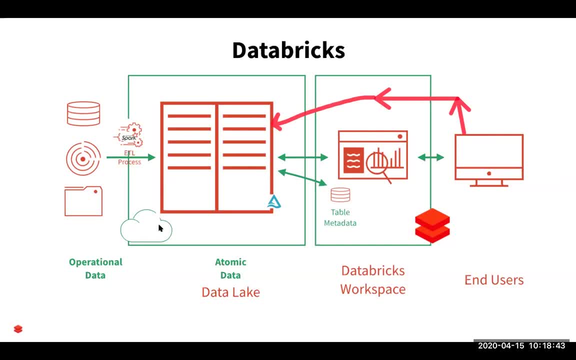 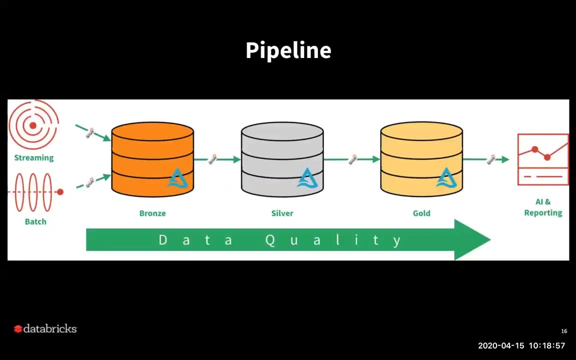 notebook environment called Data Lake, And the beauty is that we have really cheap storage for all of this data and we're only paying for the CPU cycles that are needed to run our workload for today. And then we shut down our clusters. And we had talked a little bit about this pipeline, The idea that when we do the ETL, 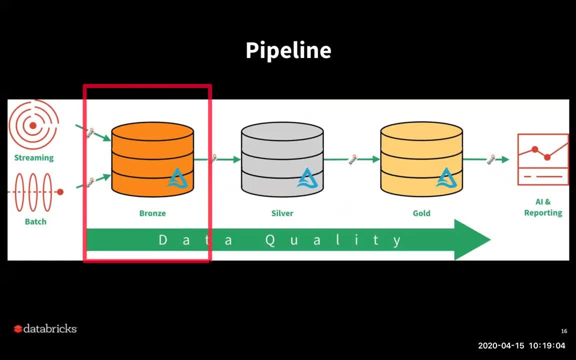 the first goal is just to capture the data as it's coming in, not do any cleansing. Some people call these their loading tables At Databricks. we like to think of it as kind of levels of data quality, So we tend to think. 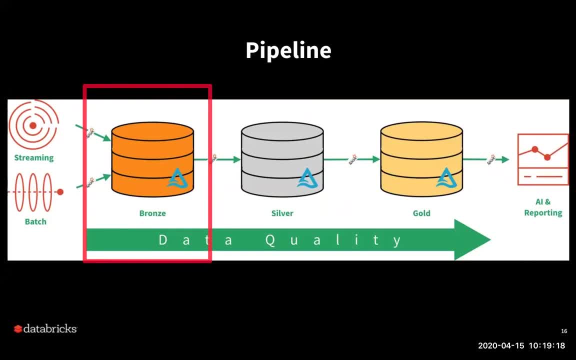 of it as our bronze layer. It's the data in its raw ugly format. It's everything. It's a lot of it, And the idea is: just capture it. Don't worry about cleaning it yet, Just make sure you don't. 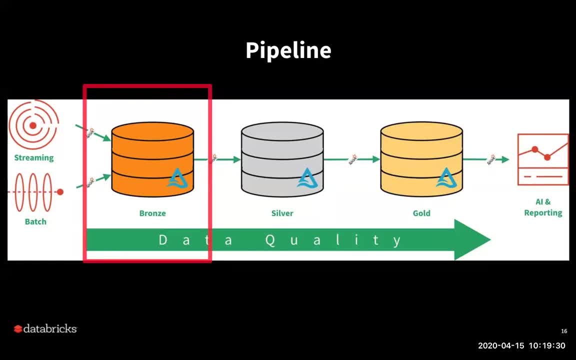 lose it, Store it in this cheap data storage. We'll come back and grab it later when we're interested in it. And then, as you start getting interested in the data, you're going to find that you need to do data cleansing. And that's where the silver tables come in. It says: what I'd really like to do is clean up this. 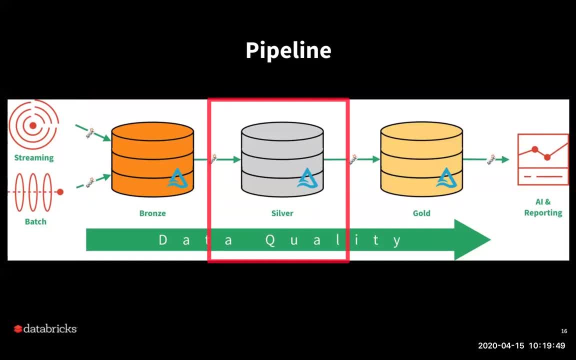 data. deal with late arriving records, corrupted records. put things into a flatter directory structure because it may have come in in JSON and it's a little bit tedious sometimes to query JSON as opposed to flat tabular structures, So I might move this into tables that are flatter. I might. 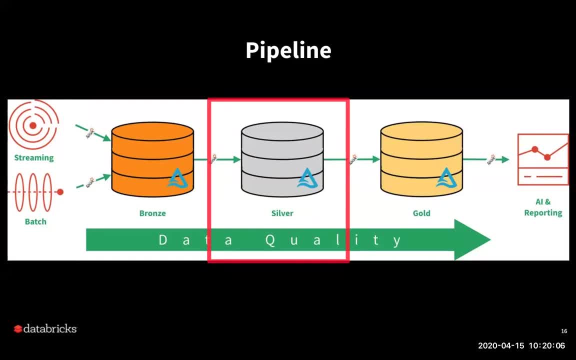 move this into something that's closer to a third normal form, although it doesn't have to be. And these are my query tables. Basically, my functional enterprise data warehouse And my data is here and people can go and query that data directly. But there's still a lot of data and we may want to do some types. 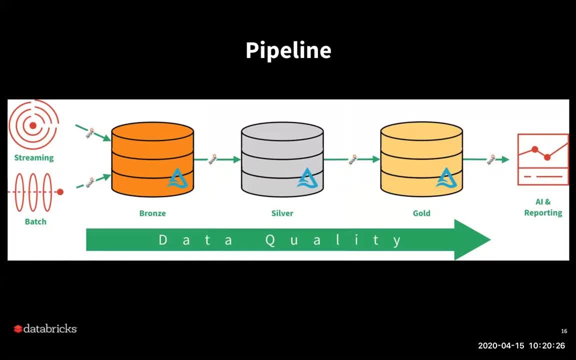 of aggregate roll-ups. So we may want to produce a star schema, for example, that really takes that data and does aggregations, And so we might have a nightly job that reads those silver tables, does various types of reporting on it and generates easier. 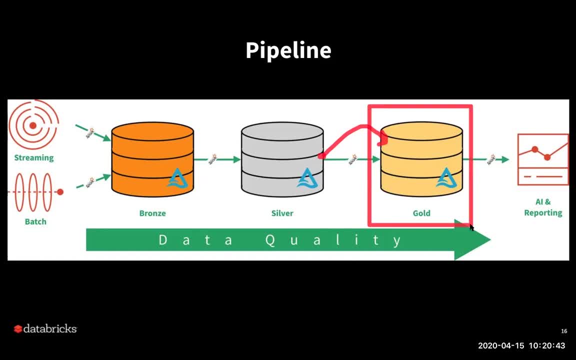 data, And then we'll create tables that are either featurized for machine learning or aggregated for reporting purposes and business intelligence, And we'll create an even higher what we would call a data mart in data warehousing lingo, or it could be featurized for machine learning. 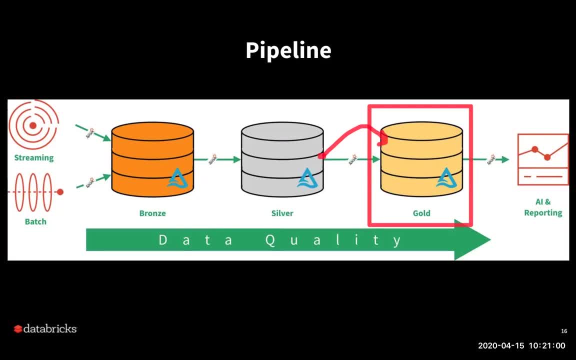 but are more refined data in terms of data quality. These are our gold tables and ones that we would really like our end users to be accessing. So most of the time, our end users who are doing reporting are really polished gold tables. On occasion they may say: oh, I've got a query. that's not. 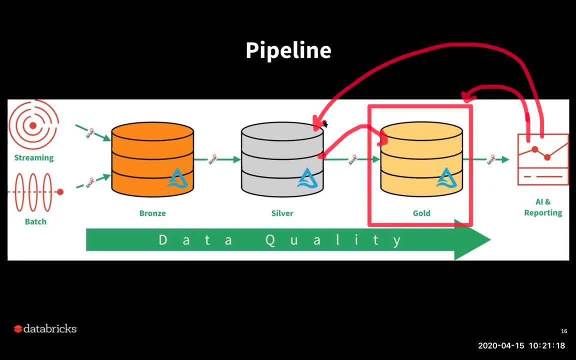 available in those gold tables because I'm trying to drill down and get more insights And they might access these clean data And then, on rare occasion, they may say, huh, there was data that nobody thought we would be interested in. but boy, I'm glad I saved. 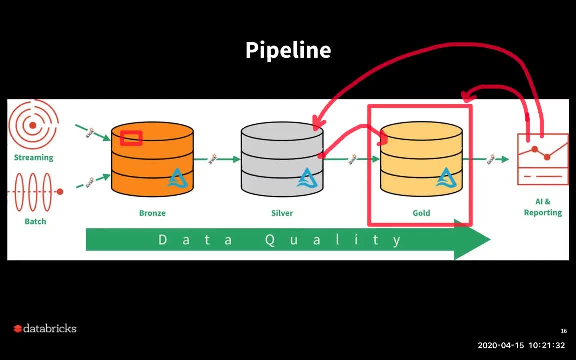 all that raw data. because I really am interested in this extra data point, Let me bring it into my system And you can in fact go and query the bronze tables. which you typically would do would just be to bring that extra data when you're interested in it. 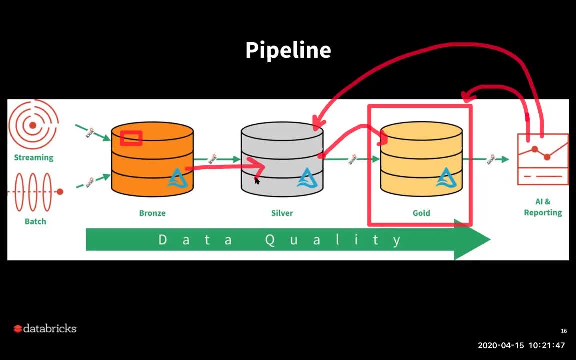 into your silver tables, So you're constantly improving your data pipeline. You've captured everything and now you're loading the parts that you're interested in, And this is what allows us to capture everything, which is the benefit of the data lake, while still getting data cleanliness. 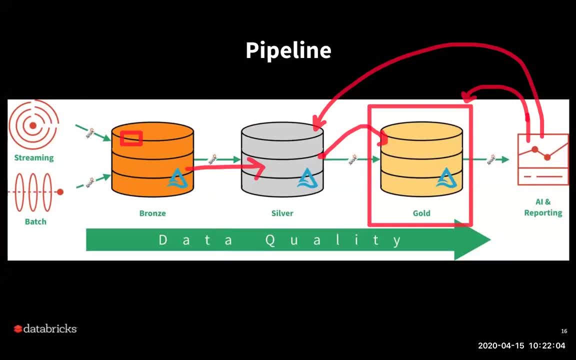 which was the benefit of a manicured data warehouse. But to do this, there are challenges that we need to overcome, And some of those challenges have to deal with managing this ETL pipeline, dealing with late arriving data, making sure that when I do one of these workloads, 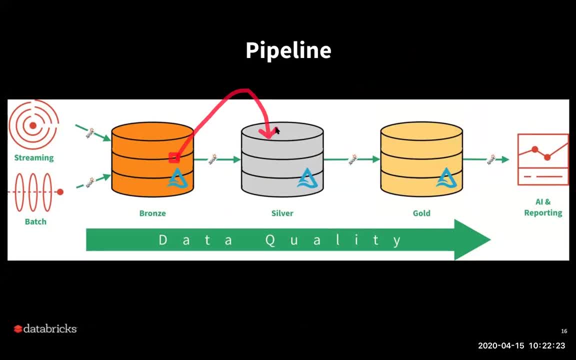 where I'm reading data from bronze to silver, that the job is reliable. So if it fails halfway through, I don't want half written data to my silver tables. I need an all or nothing. I want to be able to enforce data cleanliness constraints. 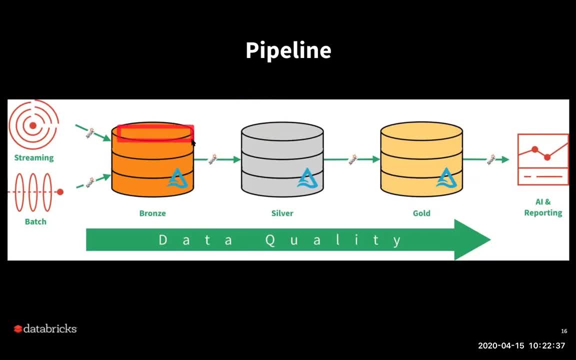 I want to be able to also work with. tell me what's new in my bronze data- And I'm going to do all of this jobs for myself by friend in the store- and ETL, just the new stuff. So is there an easy way where I could track the changes, the delta? 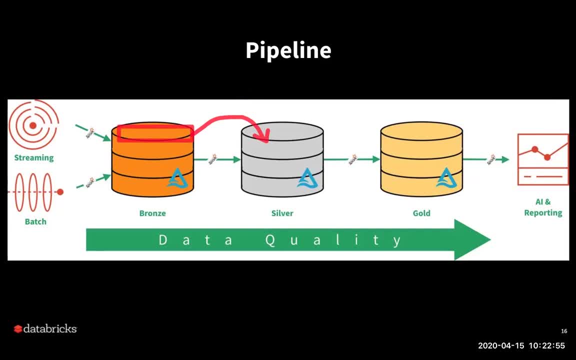 of what was in that table before and only work on what's new, And that's where streaming is going to come into the picture. So this is what we talked about in terms of the architecture in the previous webinar. So today, our goal is going to be to construct. 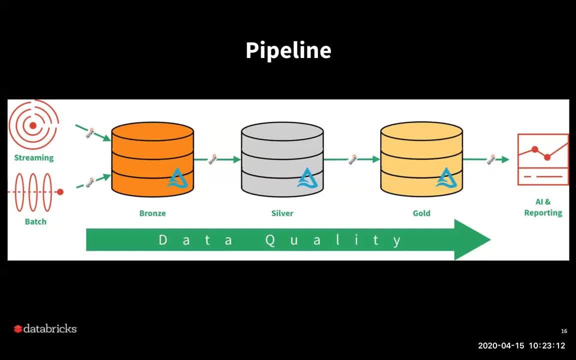 experience in our cloud data platform using Databricks. So we're going to drop down now and it'll go into the coding layer. Let's see here Before we do. I'm just going to take one question and answer it. Somebody had asked because we did a lot of our examples using Spark SQL. 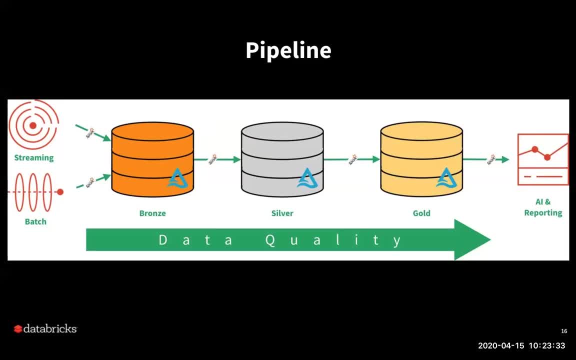 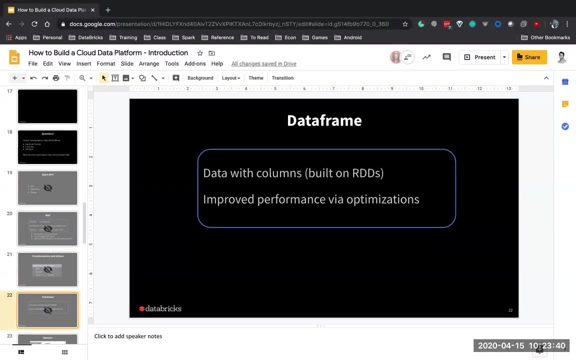 and somebody asked what's the difference between PySpark and Spark SQL, And I do actually have a slide on this. It was one that I wasn't going to cover, but I'm going to go ahead and bring it up now, because it will help address that question a little bit. So, first of all, let me just show 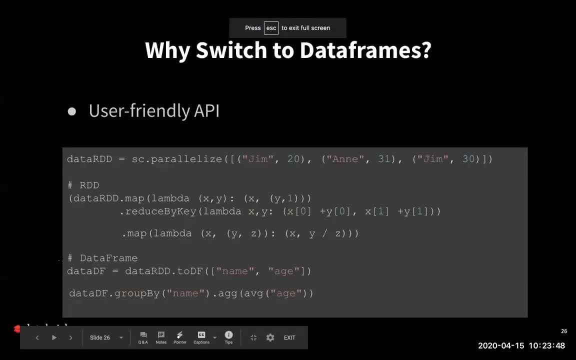 what PySpark looks like as opposed to Spark SQL. So in PySpark, notice I'm using Python as opposed to SQL to describe my queries, But at the end of the day, I'm simply describing my query, whether I choose to use SQL to describe my query or I use Python. 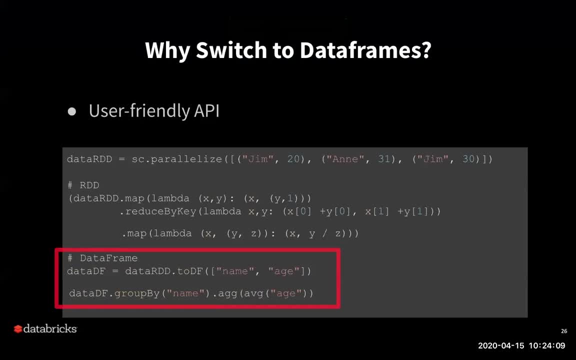 to describe my query. At the end of the day, I'm just describing a query. So in this case, my query is: I want to group this data up here by name and then I want to get the average age. But I'm just describing a query Now. this particular slide was really designed to be. 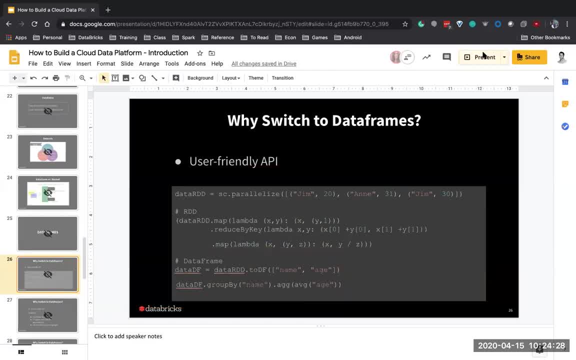 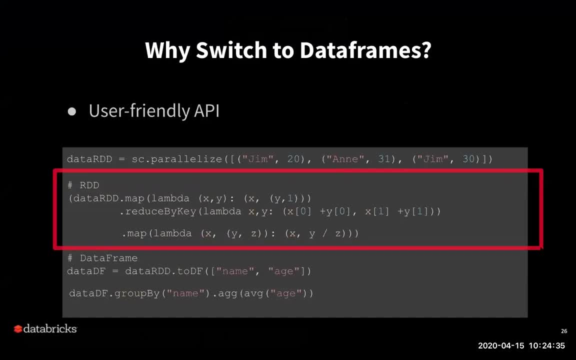 contrasting this data frames approach, where you're describing your query, to an older Spark approach called RDDs. RDDs are the underlying, almost like assembly layer. It's the low level in Spark that we don't often work at, And the reason we don't work at the RDD layer is: 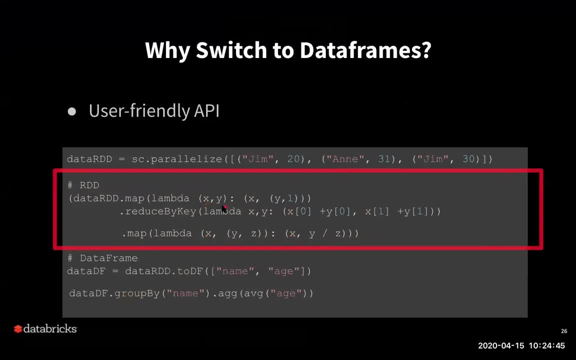 because it's not very readable. So if you look at this code, if I was trying to do this using functional programming, I'd be passing in a function here saying: grab that data, run this function, run this function and run this function, And it's really hard to know what that code is. 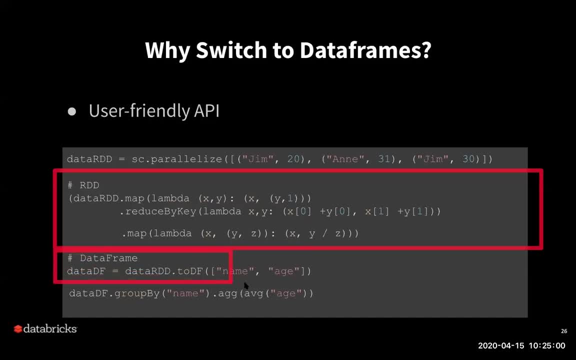 doing, compared to this code down here in PySpark, where it's really clear I'm grouping the data by name and averaging. So it's a declarative query as opposed to a functional oriented programming paradigm. So we really like working with data frames in PySpark as opposed to the RDD level. 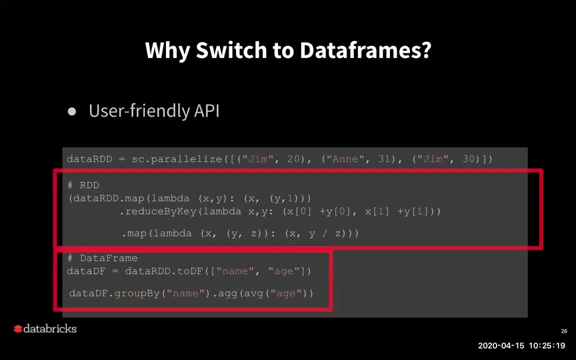 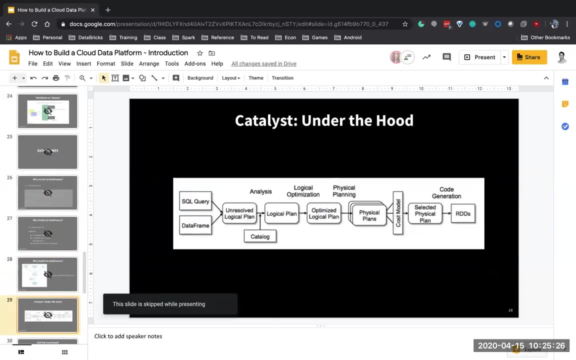 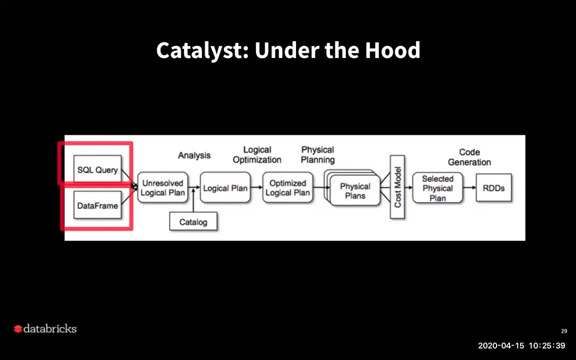 or if I'm using SQL. at the end of the day, I'm just expressing a query operation or a data operation. So I'm either doing data manipulation or data query, but I'm expressing in a declarative way what I want to do with this data. 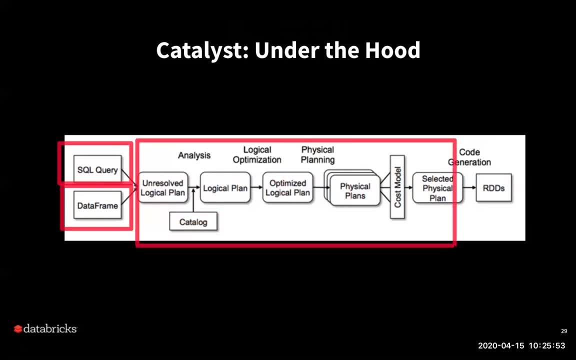 And then the driver takes all of this stuff and goes through a whole planning process where it generates code. So it's going to look at your query. whether you describe your query in SQL or in Python, it gets fed into the SQL. It's getting fed into the same process here. 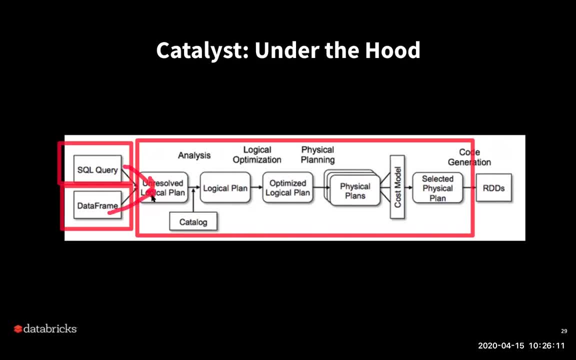 So there's really no difference as to whether I'm using SQL or Python. It's getting fed into the same query planning process, where it goes through a rule-based query optimizer And eventually a physical plan pops out on the other side. that Spark turns into an RDD and runs. 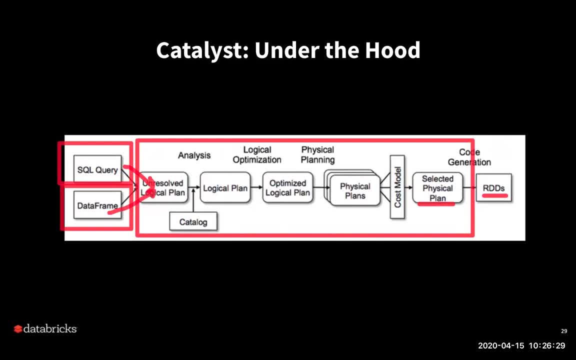 But this RDD that Spark generates is way more efficient than any RDD you could have written yourself, because it generates code. It's actually generating code on the fly that works on native biters, And you could just not. it would be incredibly difficult for you to write an RDD. that would be as 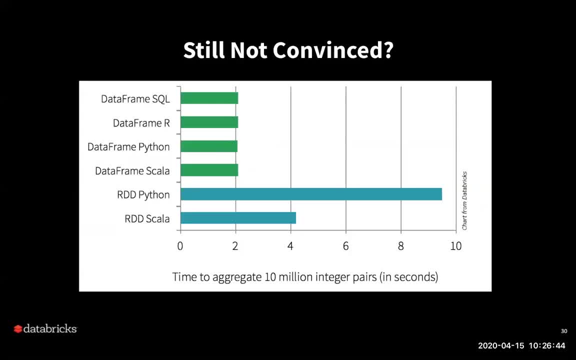 efficient as the stuff that Spark generates for you. Just how much more efficient. Take a look at this slide here. So if I was doing RDD programming, look how long it takes to run a job. And if I was doing RDD programming, Python would have been slower than Scala. 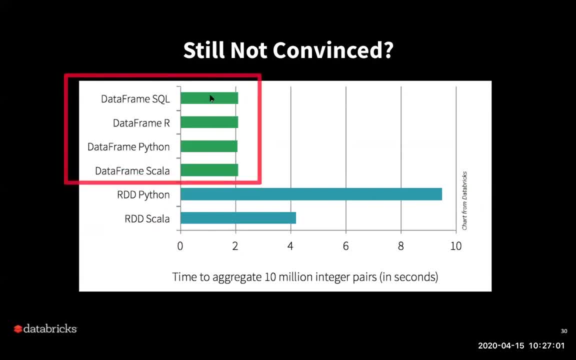 But when I go to using data frames, Spark is generating code, and it's generating code that's much more efficient. So it doesn't matter whether I use SQL or Python. I'm going to get all of the benefits of that query optimization process. 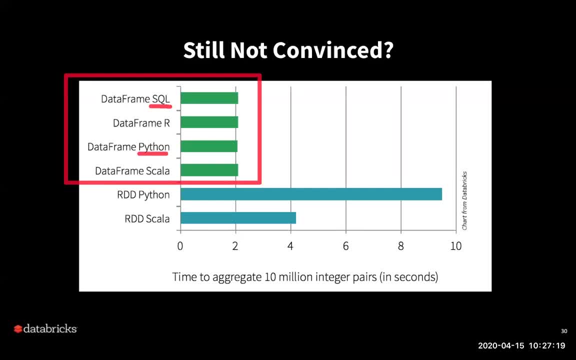 So the short answer is: choose SQL if SQL is comfortable to you. Choose Python if Python and PySpark are comfortable to you. In this series I'm going to choose SQL because it appeals to the broadest part of the audience. But when we get to streaming and to machine learning, we will drop the Python. at that point, 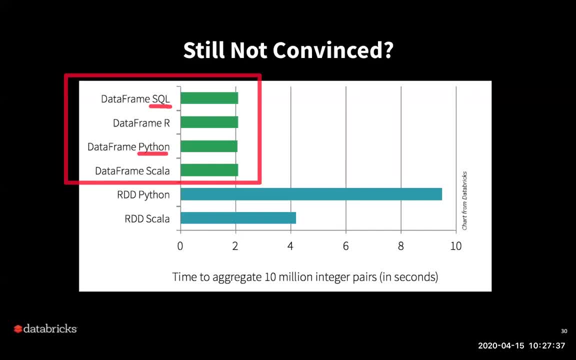 Because those APIs are not as efficient. Those APIs aren't available in SQL. The machine learning and the streaming APIs will require some Python, But for the rest of this I'm going to use SQL because it's just accessible and it's there and it's easy for people to work with. 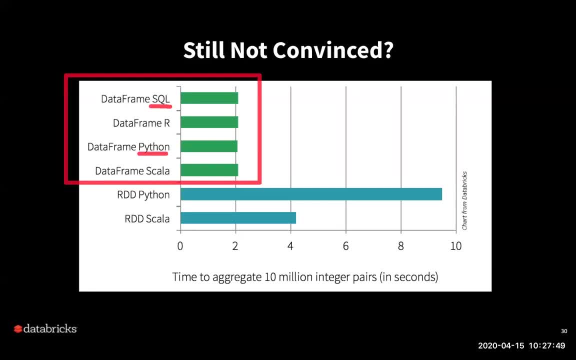 But notice that the performance is the same. And for those that are really advanced, I'll make a footnote. If you define a user defined function, User defined functions are the one place where there's now a cost associated with using Python because that user defined function is written in Python. 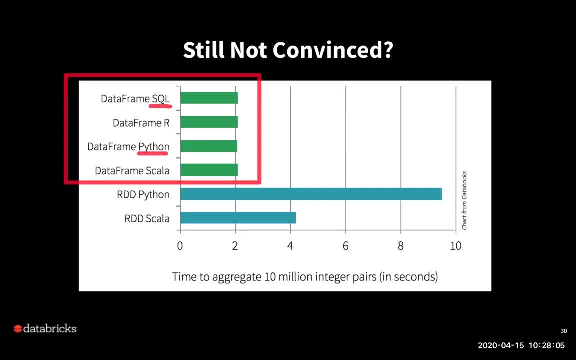 Now, if you write your user defined function in Scala, it will be faster Than if you wrote it in Python. We're not even going to be looking at user defined functions, but I wanted to make that footnote And if you wanted to learn more about user defined functions, I would encourage you to go to academydatabrickscom and take some of our SQL courses, where we really go deeper, especially our ETL series of courses in the academydatabrickscom, and you'll learn more about user defined functions. 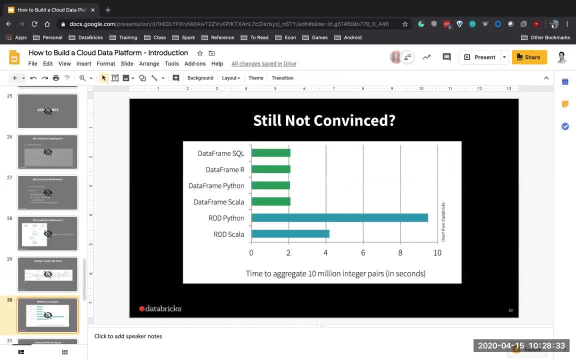 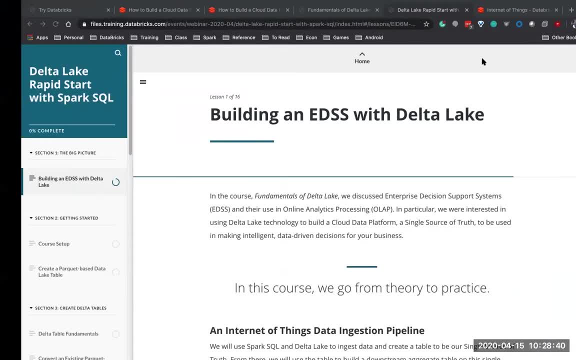 All right. so with that in mind, let's go ahead and start building our data lake here. I'm going to leave this slide up for a little bit later, All right. So remember, I told you you could go to that link. 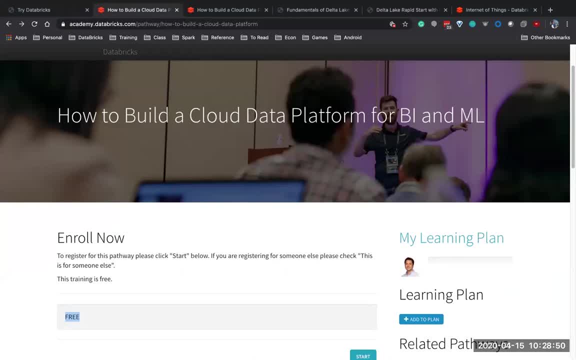 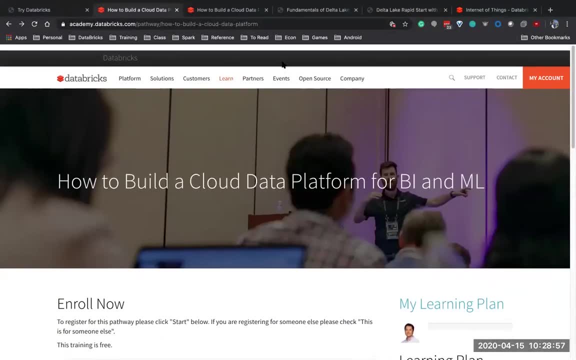 That tiny URL that we put up earlier. It's tinyurlcom. slash cloud dash data dash platform, and it's going to take you and make available to you access to the online course. At that point, you'll see the fundamentals of Delta Lake, which is what we covered yesterday. 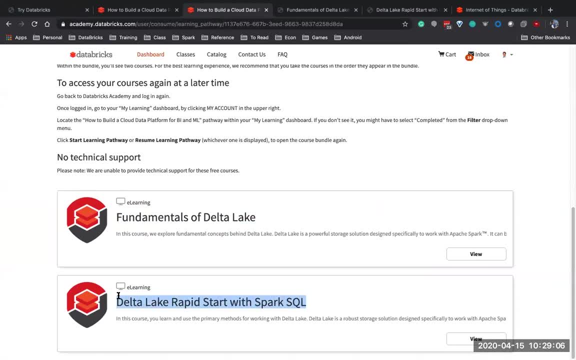 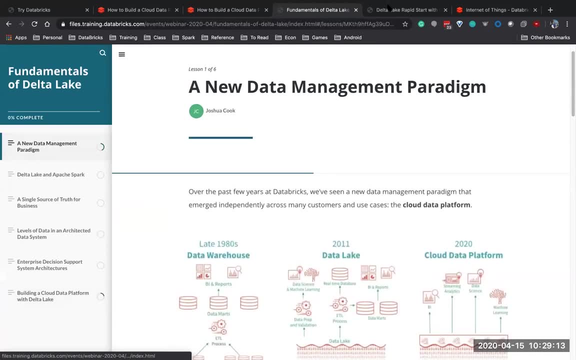 And for the next two days we're going to be working from Delta Lake Rapid start with Spark SQL. So in the Delta Lake, rapid start with Spark SQL. This is where we're going to be working today. we're going to actually be building our data pipeline. 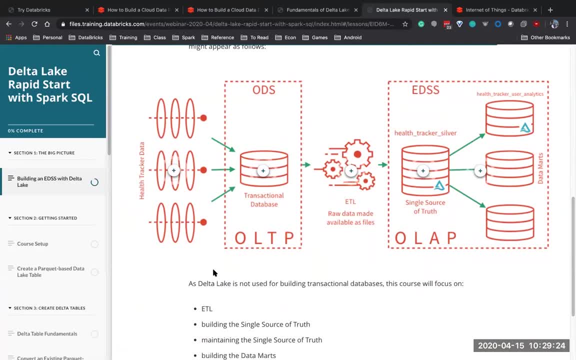 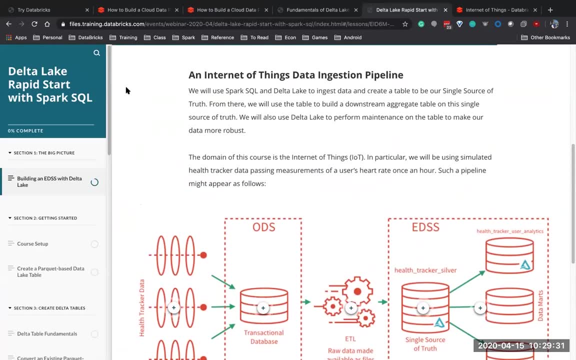 So, again, remember this picture that we had from yesterday where we might have. In this case we've got a scenario. we're going to be working in the Internet of Things, So our data set is going to be health tracker data. 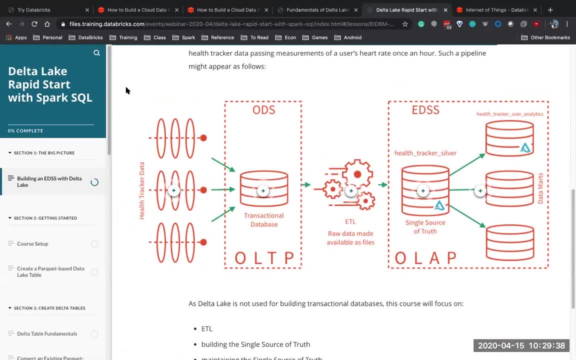 So we're going to be working in the Internet of Things, So we're talking little. you know: fitness watches that you might wear on your wrist. We've got health tracker data that's coming in from our Internet of Things. We've got JSON files being collected from a whole variety of different systems. 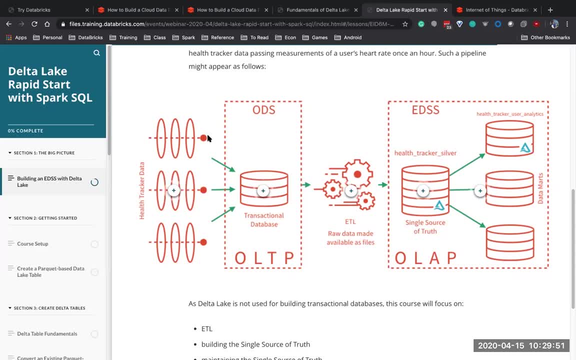 And our data is going to start out coming in as JSON files and this would be really what we would consider our operational data. So health- in this case the health tracker data- has been streaming in. somebody dumped it into our operational data store. This is using a traditional database, or what we call online transactions. 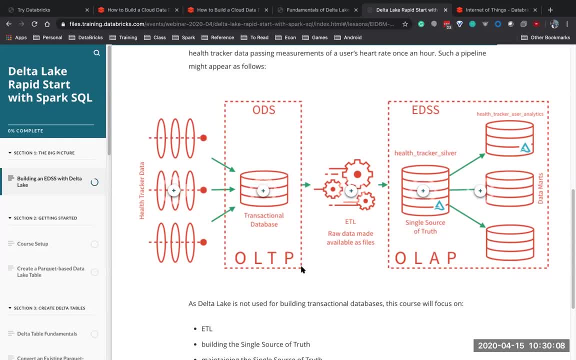 This is using a traditional database, or what we call online transaction processing. online transaction processing is where you are editing and modifying individual rows of a database, And we don't use spark for that type of workload. We use a regular database when we're when you're doing any type of workload where you just updating one or two rows, one or two records. 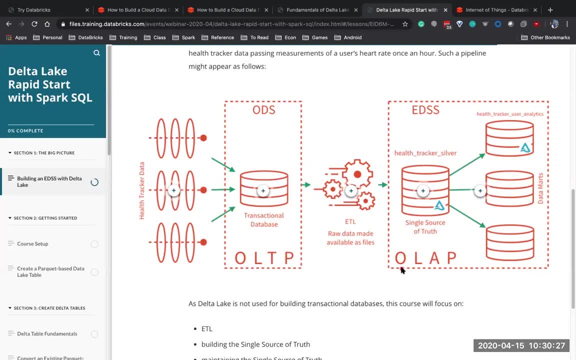 We would use a traditional database. where we're going to use spark is when we're doing the analysis, the online analytical processing from our data warehouse. We're running Huge Big data queries, So what we're going to want to do is ETL the data from that operational data store. 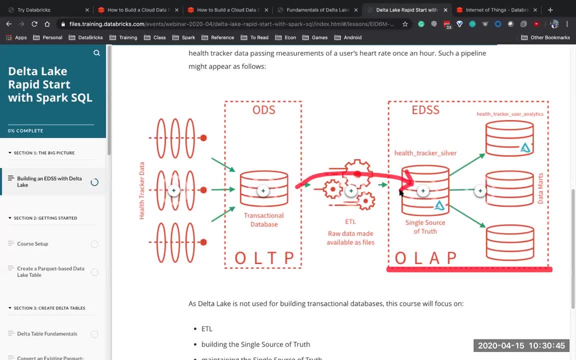 Into our data warehouse so that we could do this type of analytical query, as opposed to the individual row updates that are needed when I'm writing data to that operational data store. So this is the idea of ETL, and we're going to be using Apache spark to do this ETL and then we're going to go and build that single source of truth. 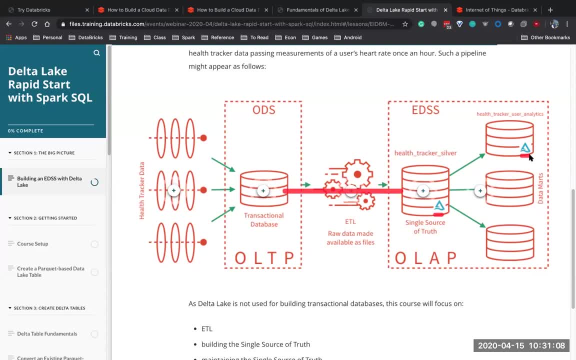 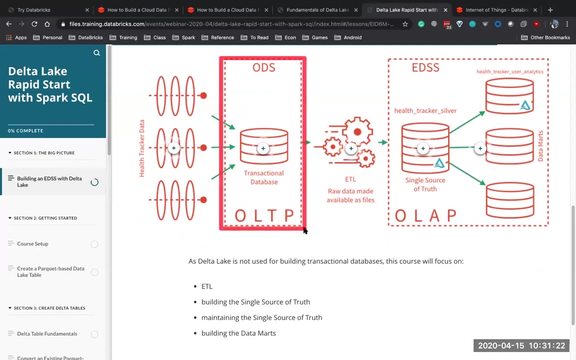 And eventually we're going to build out those data marks as gold tables for analytics purposes. So we'll have our silver tables and our enterprise data warehouse and eventually our gold tables doing analytics. And again, Delta Lake and spark are not used for transactional database. You're going to use my sequel or some other database for that type of work. 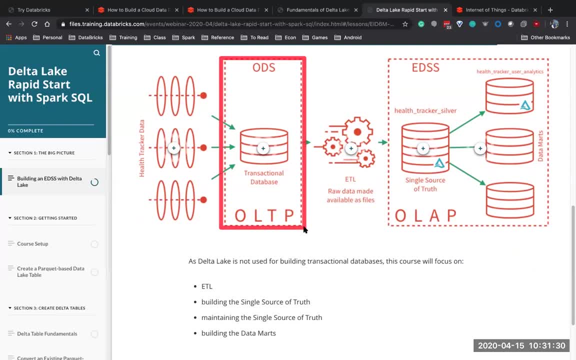 We're going to use spark to build the data warehouse or our data lake, in this case, our cloud data platform. So we're going to use Spark to do ETL: building out that single source of truth and maintaining it, keeping it up to date and building out those data marks. 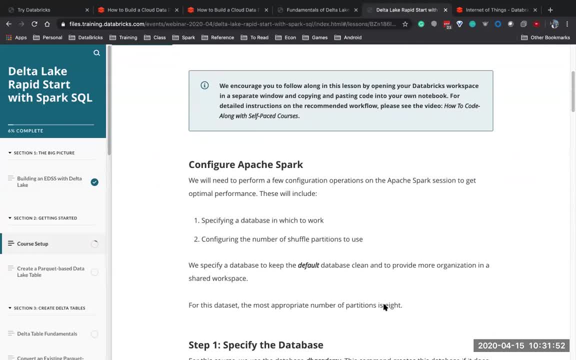 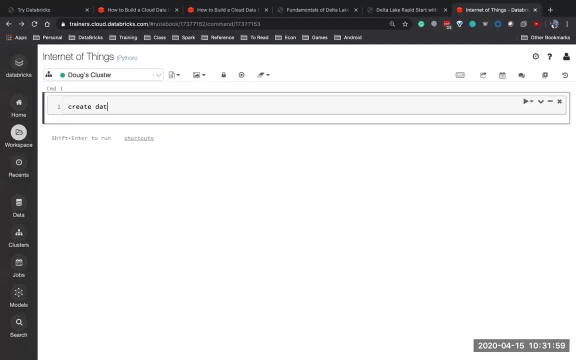 So, in this particular example, the first thing that we need to do is to create a database in our system. So I'm going to come over here. I'm going to say create. First of all, I'm going to remake this notebook. 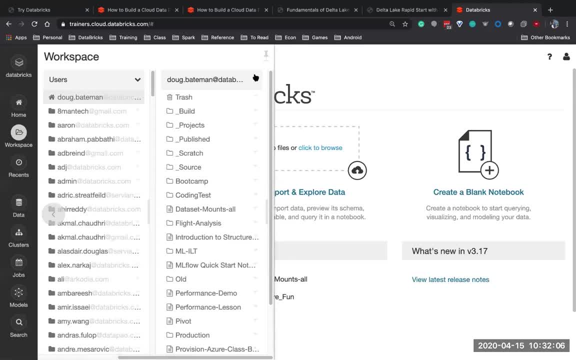 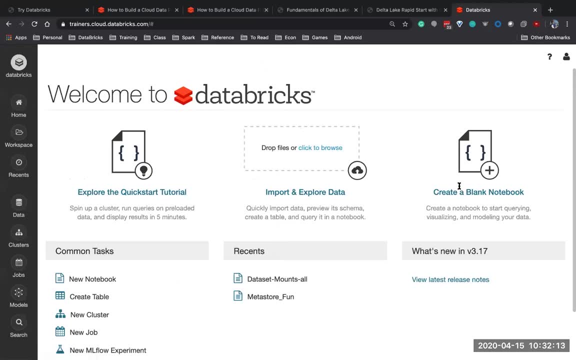 I had made this notebook in Python, and that was a mistake, because I'm going to use SQL as my primary language. So when I log into Databricks, whenever you first create your account, you're going to get a workspace a bit like this: 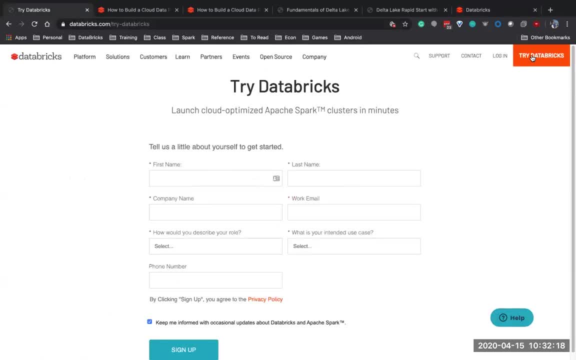 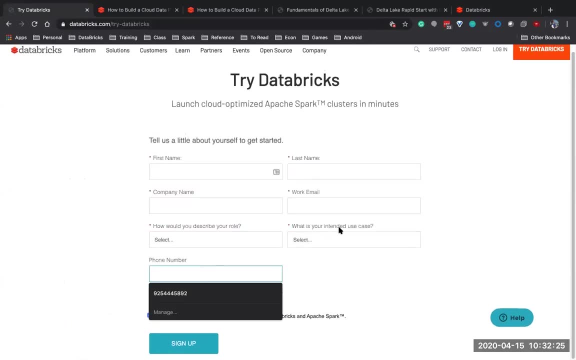 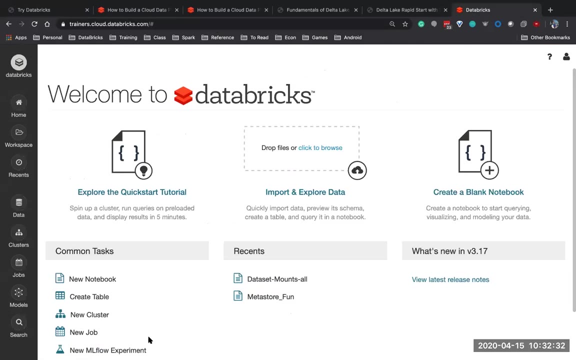 In fact, if you wanted to have your own workspace, if you go to Databrickscom and you click on the Try Databricks button, you're able to sign up for Databricks Community Edition And at that point you would log into communityclouddatabrickscom and you'd have a workspace that looks a little bit like this. 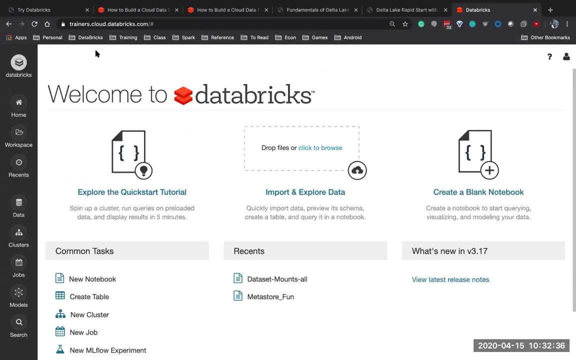 And if you want to make it look like mine, today I'm going to use not just the community edition of Databricks, but the full version of Databricks, because it's got additional features and allows me to launch larger clusters. that will reduce the latency of some of the jobs that we're about to run. 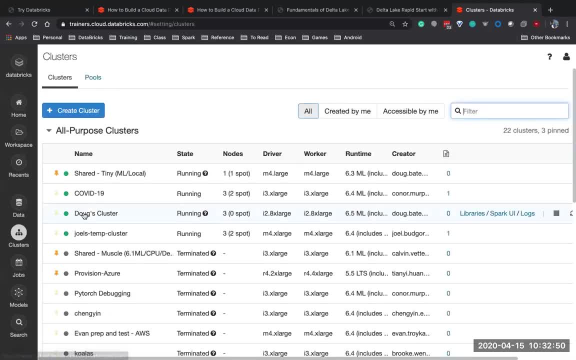 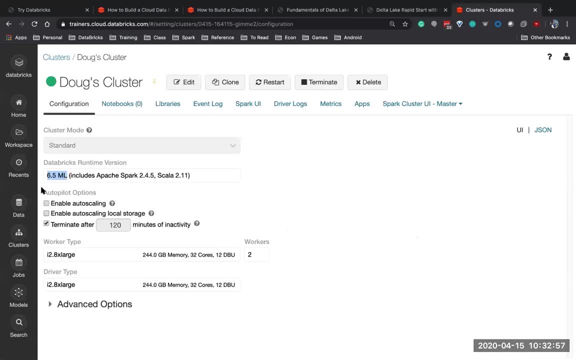 And you'd launch a cluster by clicking on the clusters tab. And in this case here's Doug's cluster And I'm running Databricks version 6.5 machine learning runtime. That means it comes bundled with a bunch of machine learning libraries. 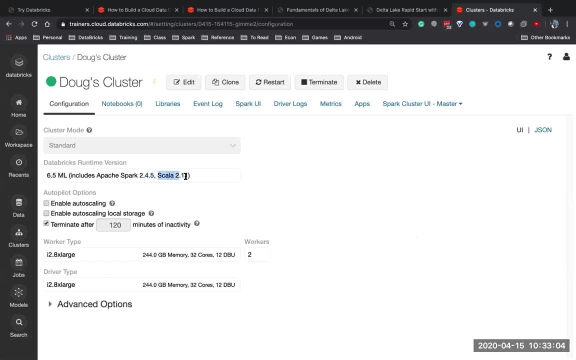 And that's running Apache Spark 2.4.0.. That's running Apache Spark 2.5 on Scala version 2.11.. So even though I might be using Python underneath, it gets compiled into Java and Scala code And I set my cluster to have two executors. 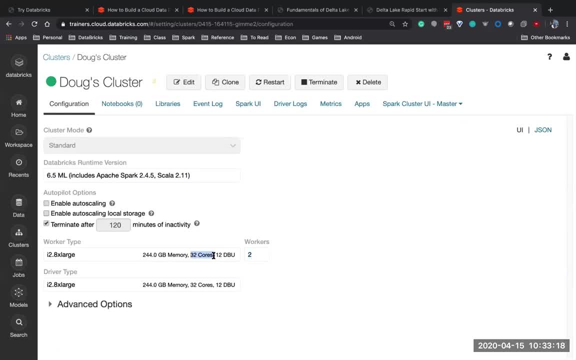 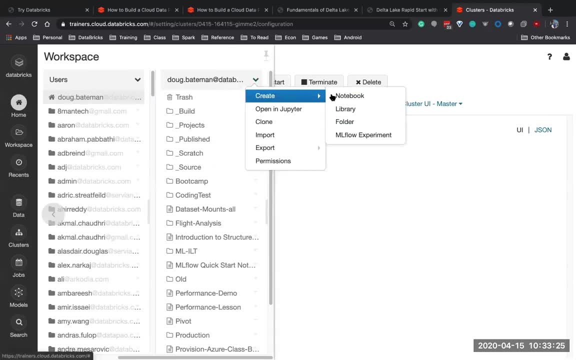 Each of these are going to be quite large, in this case a 64-core executor. And then I click on Home and I'm going to say: I want to create a new notebook, I'll create a new notebook, And I get to pick the programming language. 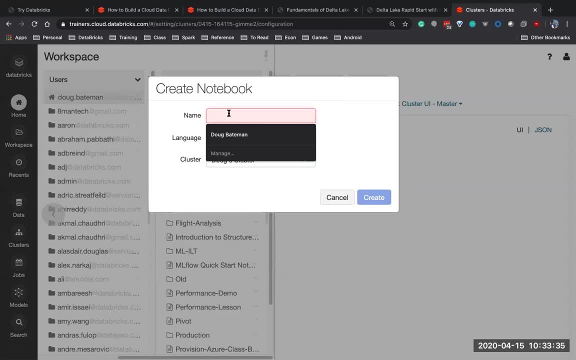 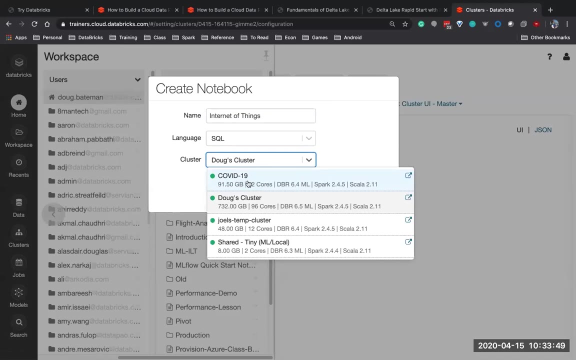 And in this case, the programming language that I'm going to be doing is SQL And this will be my Internet of Things project. Choose SQL for my default programming language and I choose my cluster And Databricks. has been doing a lot of contributions, trying to help do analysis of COVID-19.. 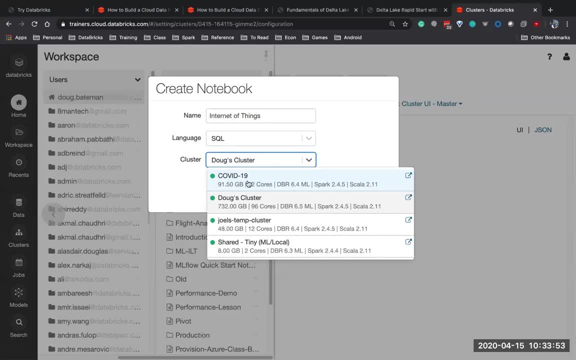 So you'll see that some other people at Databricks are running a cluster that's doing that type of analysis, But for now I'm going to just be creating my own cluster that I've not shared with anybody else and connecting to that. 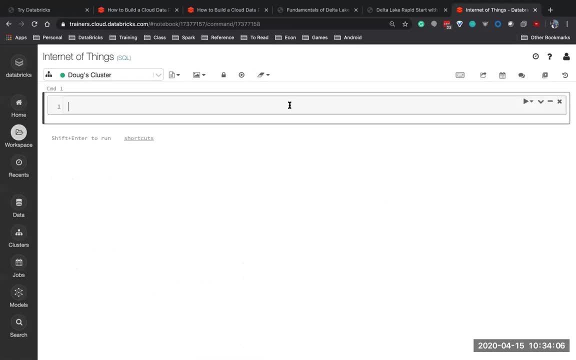 And now I want to start ETL-ing in my data. So the first thing I need to do is to create a schema where I can start uploading my tables. So I'm going to say, create database if not exists: dbacademy. 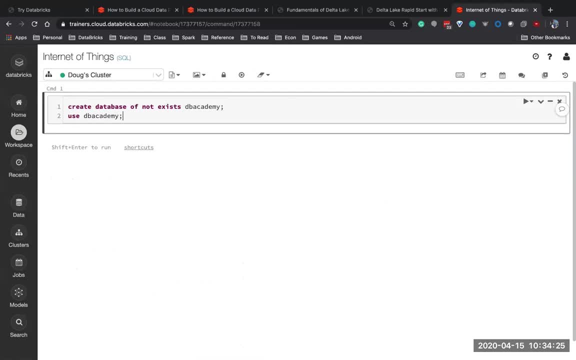 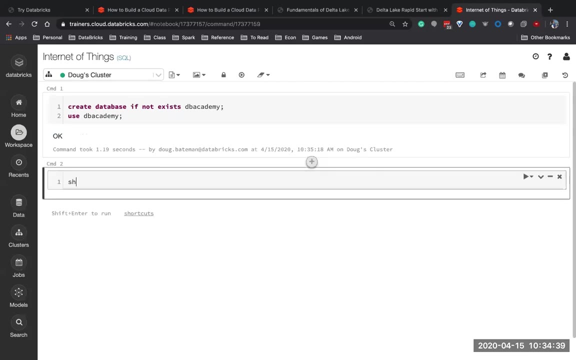 And use dbacademy for my tables. Let's see: create database. if not exists, There we go, And now I could look to see what tables I have in here. So show tables, dbacademy, Or just show tables in this case. 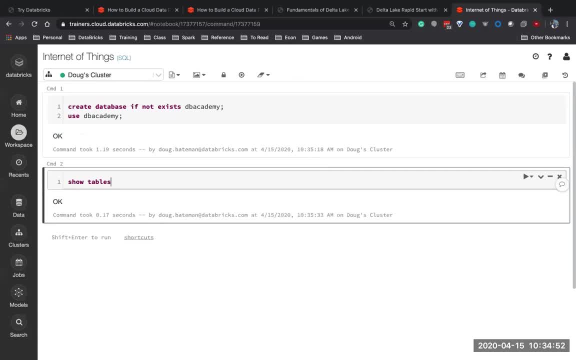 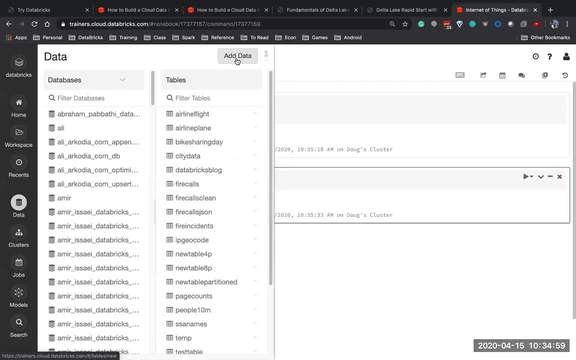 And currently I don't have any tables in the dbacademy schema, So we need to upload our tables. So I'll click over here on data and I'm going to click add data And I'm able to upload a file. 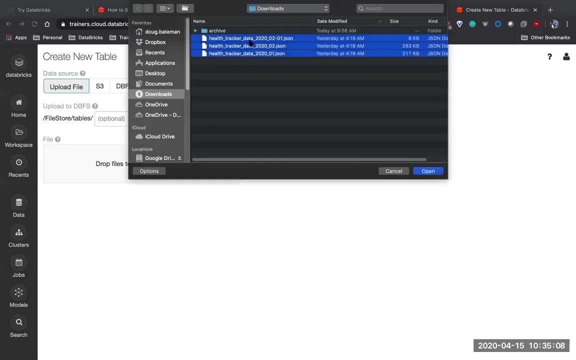 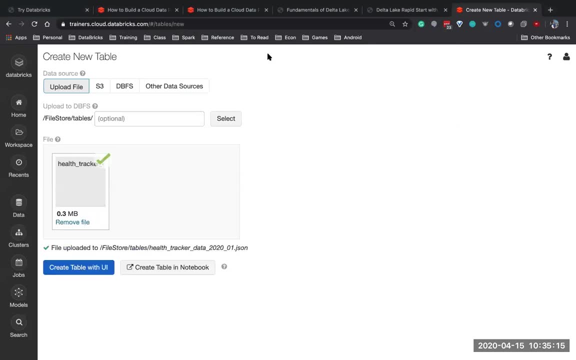 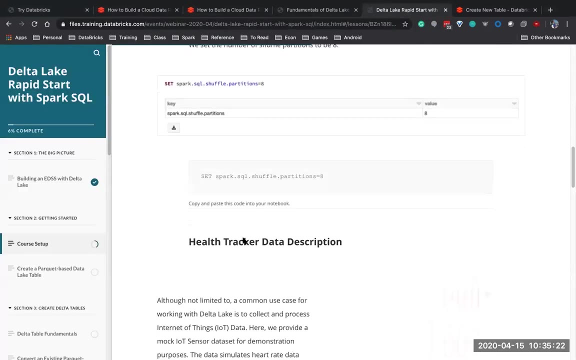 So I'll click browse And here's my health tracker data. So I'll upload my health tracker data 2020.01.json. And where do I get that data from? You may be wondering. So, if you're actually taking the course, so if you've got that course open, 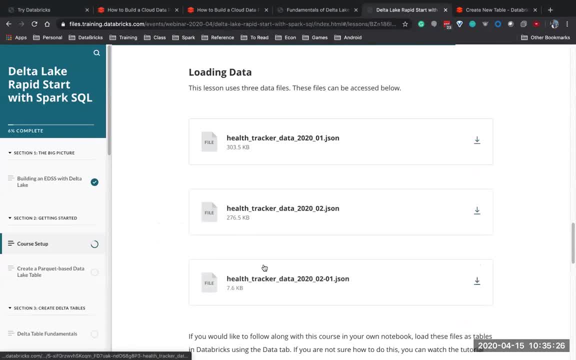 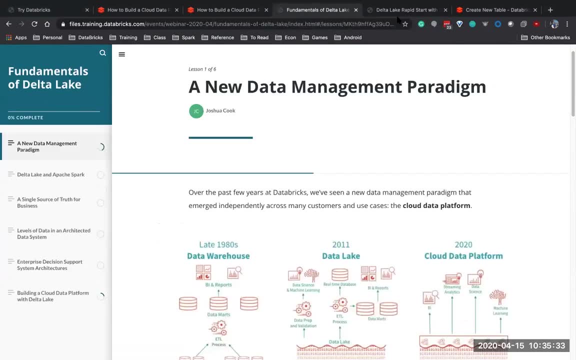 it's going to show you a place that you can actually download these JSON files that I'm using. So if you're doing this after the training, you're welcome to download those files. So I'm just going to upload them to Databricks. 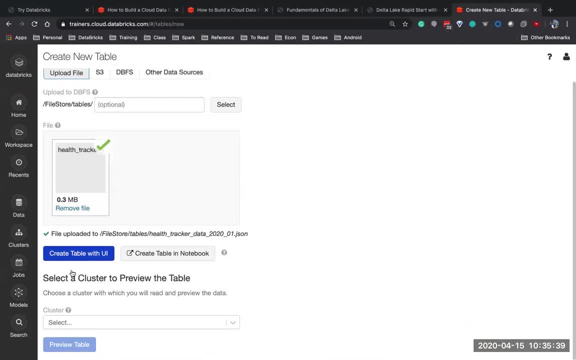 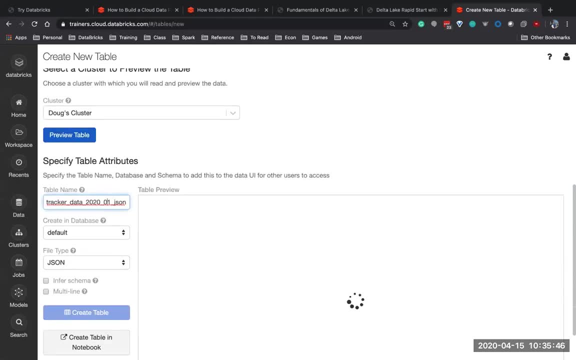 And then I say create table. with the UI. I choose my cluster, Doug's cluster preview table, And here's the file that I uploaded. It put JSON. because it's a JSON table, I'm going to strip off the name JSON just so that I can match the course. 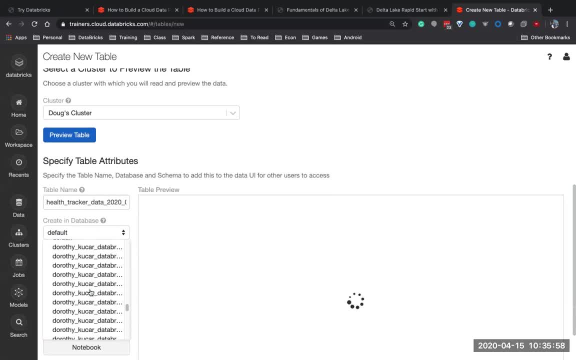 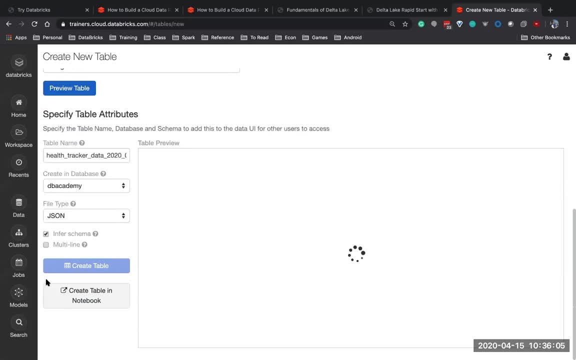 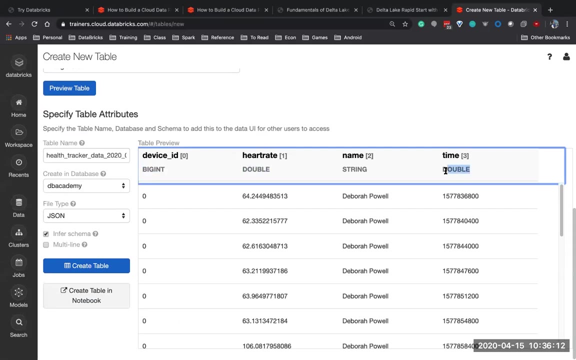 And I say create in database, And where is dbacademy? dbacademy, There we go, And then I check infer schema. So it's going to look at the JSON file and it figured out which columns are integers, which columns are doubles, which columns are strings, and so forth. 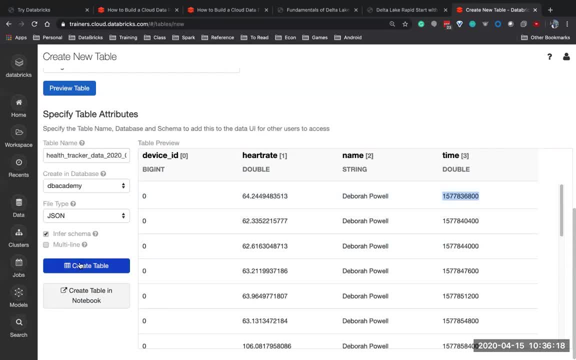 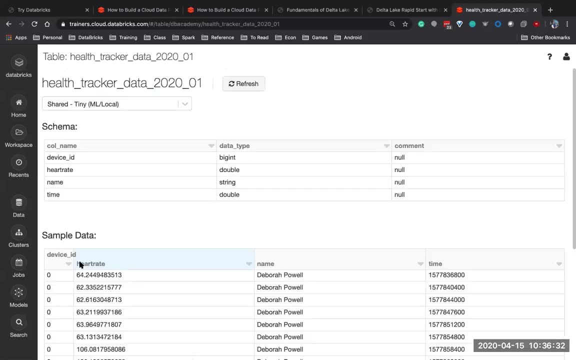 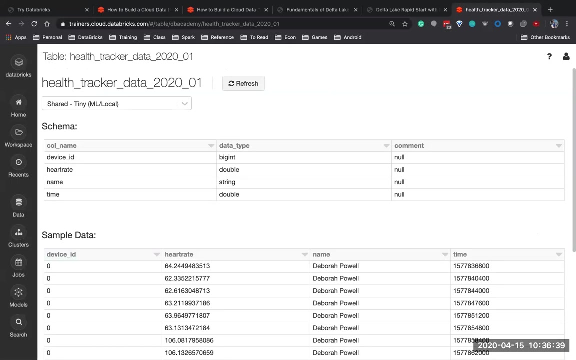 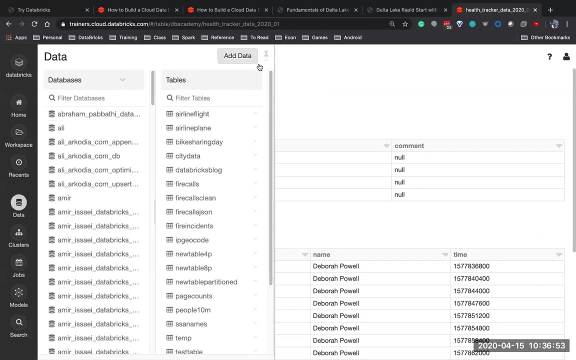 You'll notice the time it's decided to infer as a double And I click create table. All right, So now we've uploaded our first file, Let's upload the other two as well, just so that we're ready to go. So I click add data browse. 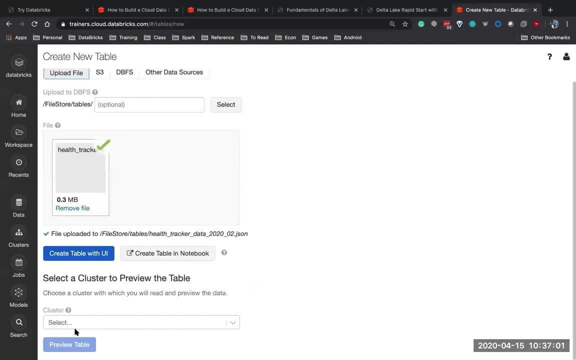 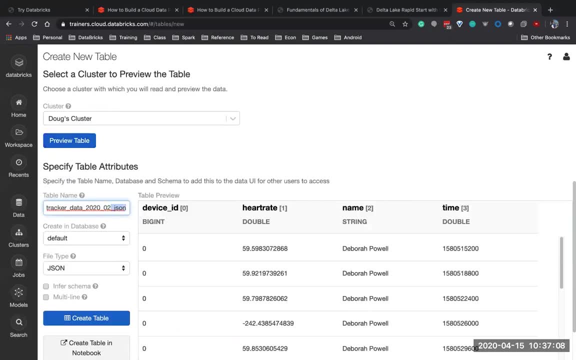 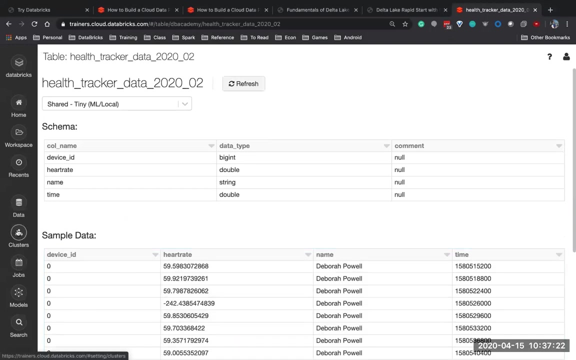 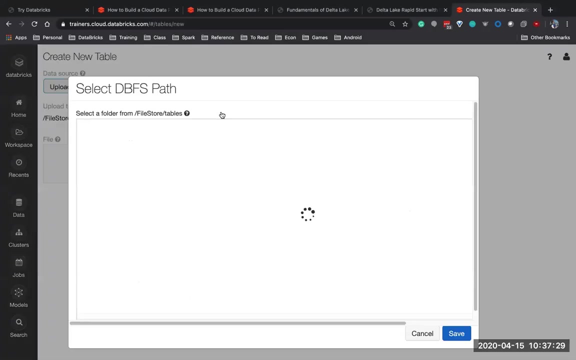 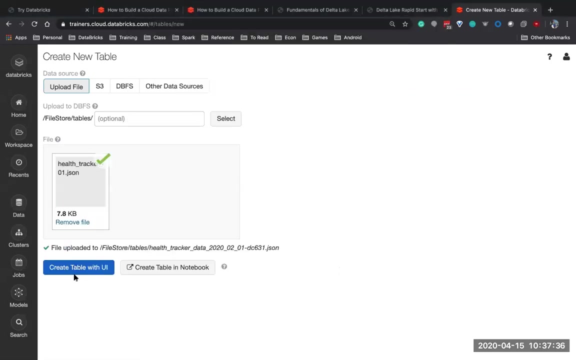 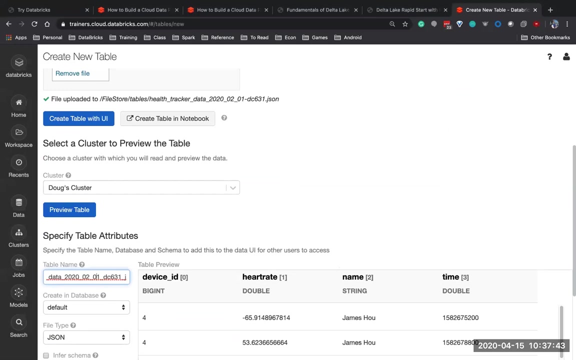 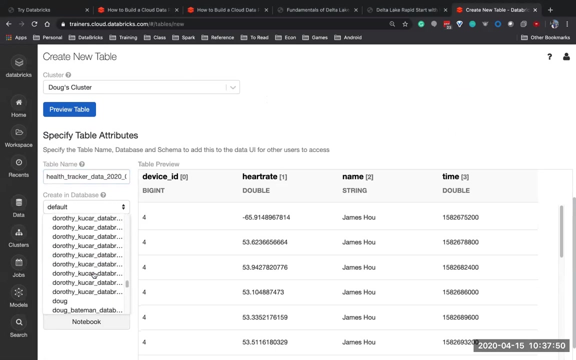 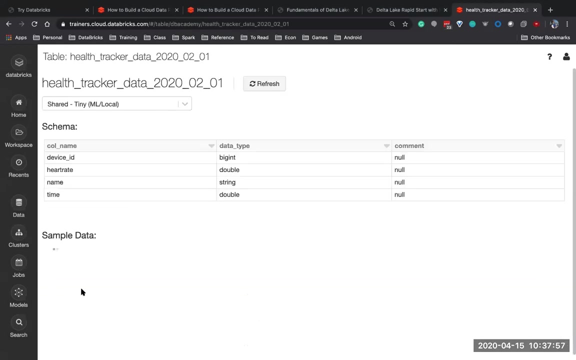 We'll grab the second month's worth of data. Create, Choose my cluster preview database, dbacademy, infer schema and I say create table And then, last but not least, create the last table. All right, So I've uploaded these tables. 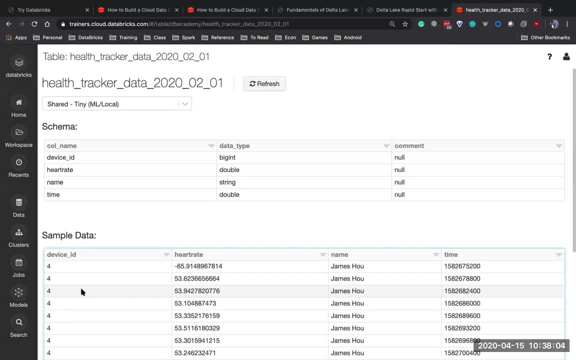 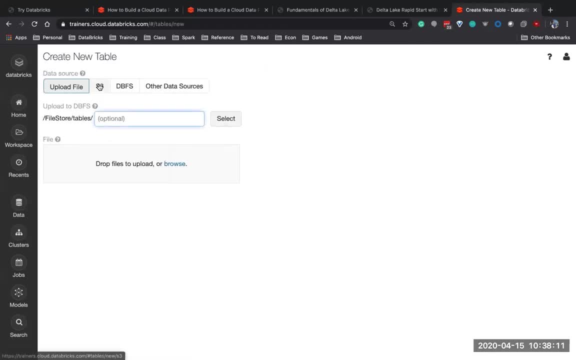 Now it's possible. It's possible that these tables were so big that I wouldn't want to upload them from my local machine. Maybe they're already out on the cloud. Well, in that case, instead of uploading a file, I could have pointed it to a file that's already out there on Amazon S3.. 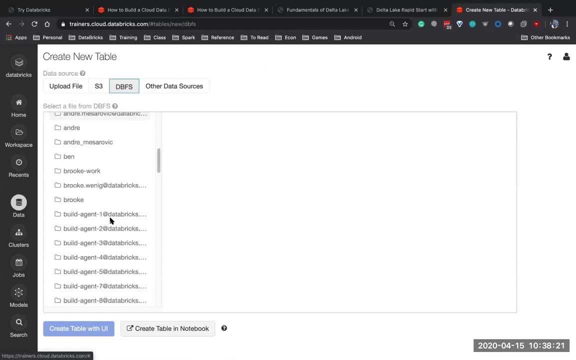 Or in the Databricks file system. So I can mount S3 buckets to the Databricks file system And I could have loaded the data that way as well, which is really really nice. All right, Now I've got my tables. 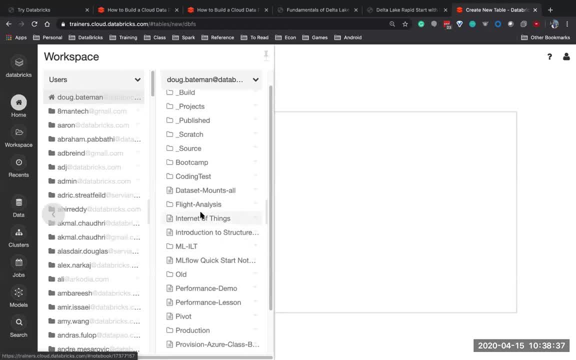 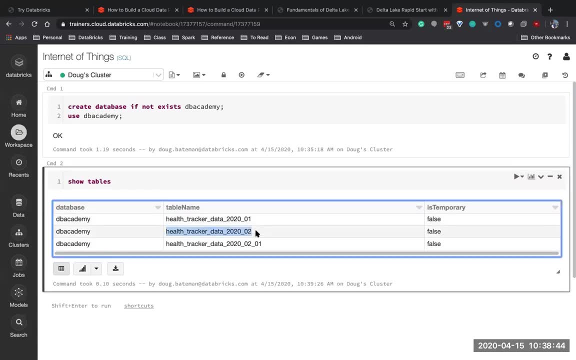 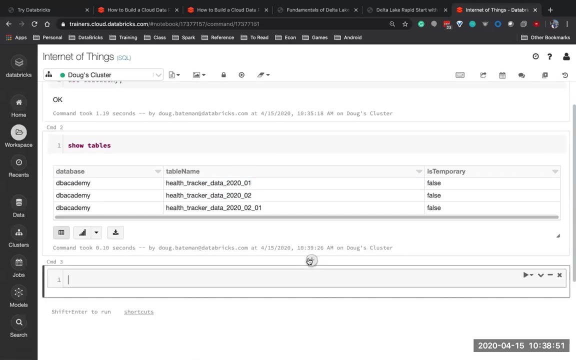 Let's go back to my notebook at this point. So we're going to find our Internet of Things And do show tables. And here are my three tables: Health tracker data 001, 002, and then 002, underscore 01.. 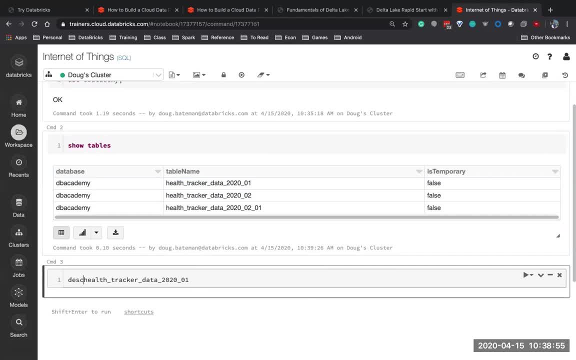 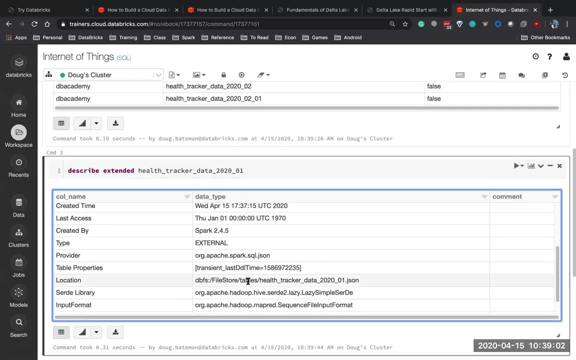 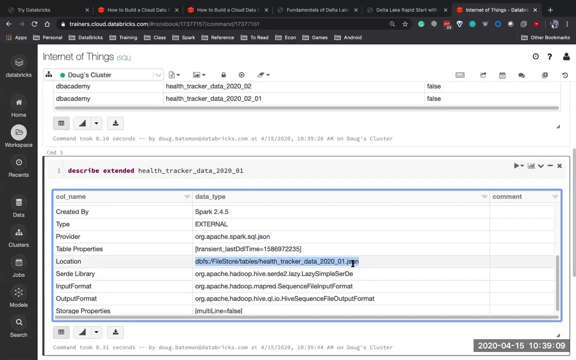 And I could do describe, describe, extended and the name of my table And notice that it tells me this table is JSON and it is located here in DBFS, the Databricks file system. And this Databricks file system is just a thin layer on top of my Blob store, whether it's on Amazon S3 or Azure Data Lake store. 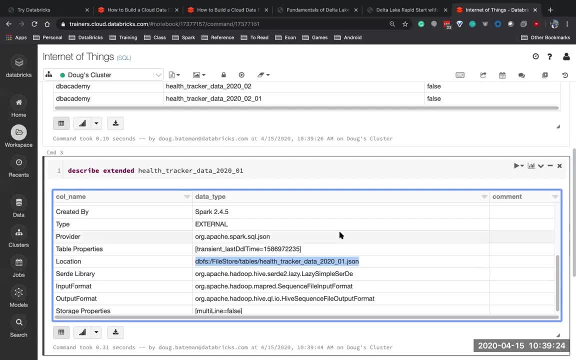 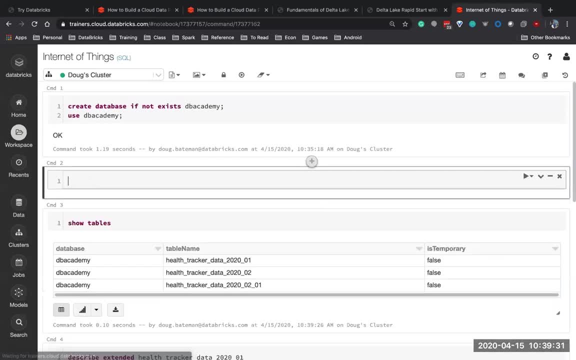 But here's my file, Here's a path to the file. So if I actually wanted to now that the file is actually in the Databricks file system, I could also have dropped it. So if I had dropped the table, I could say: drop table: health tracker data 2020- 01.. 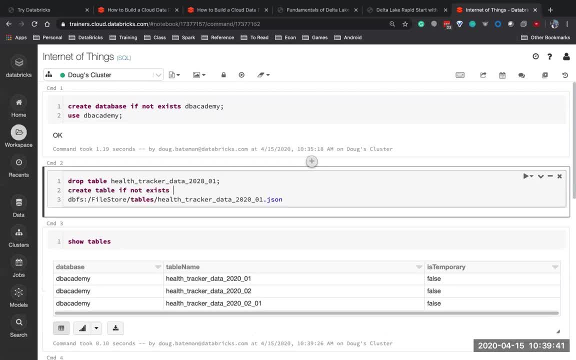 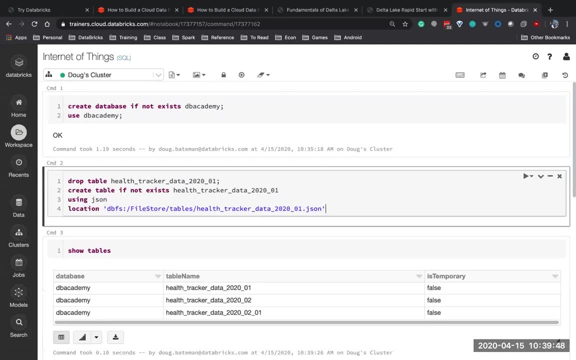 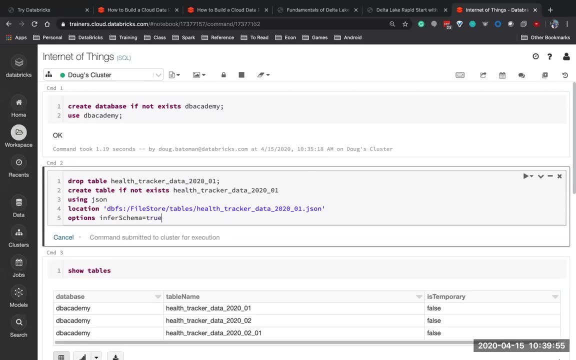 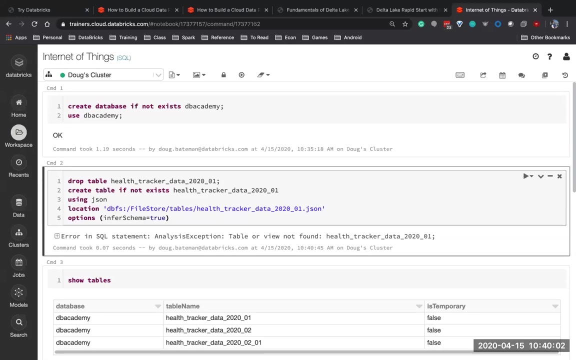 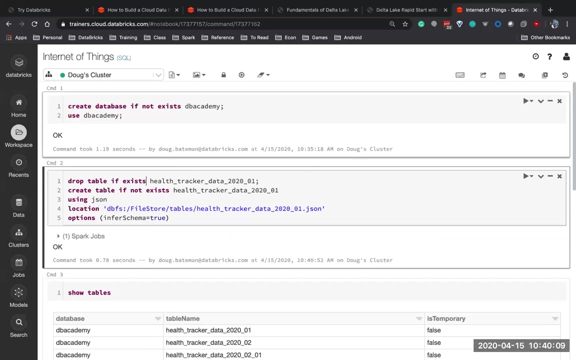 And then I could say: create table if not exists using JSON, location and options, And first schema is true And I could be creating the table using SQL instead. Drip table if exists. There we go And I've created the table using SQL. 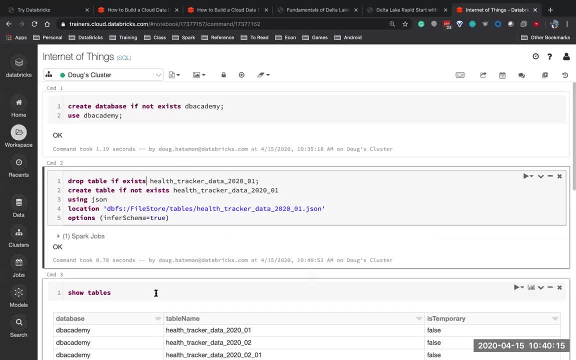 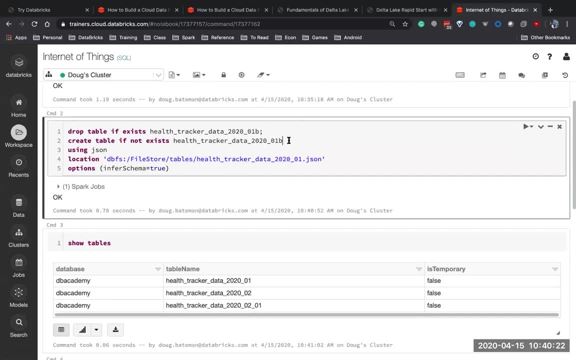 as opposed to using the UI. So I wanted to be able to show you both approaches to doing it. So I've got my tables. In fact, I will create the table a second time, just for demo purposes. I'll put a- B at the end. 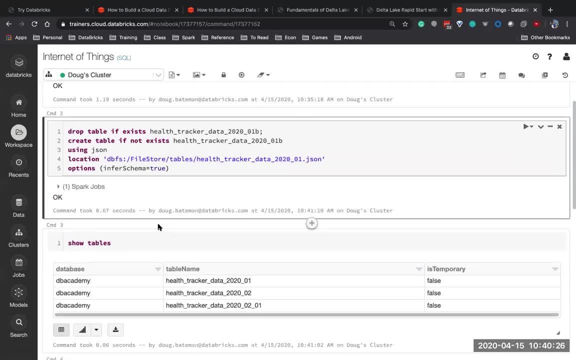 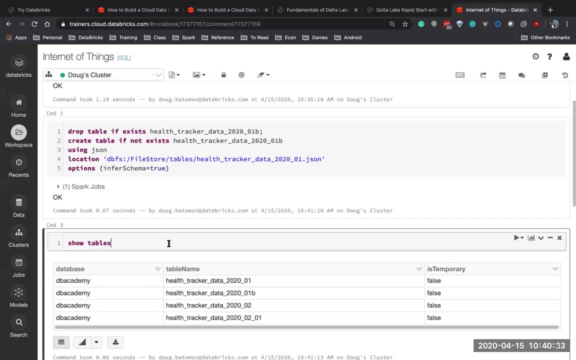 so that you can see that it's there. I'll do show tables And there's the table that I just created. It's just the duplicate, And then, if I no longer want it, I could drop table health tracker 001B. 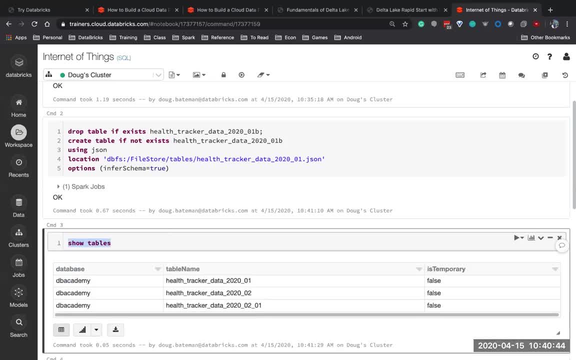 And now, if I do my show tables, it's no longer there. So this is how I get my data available to me as a table. Now keep in mind that this table is really backed by that JSON file, So if the JSON file changes, 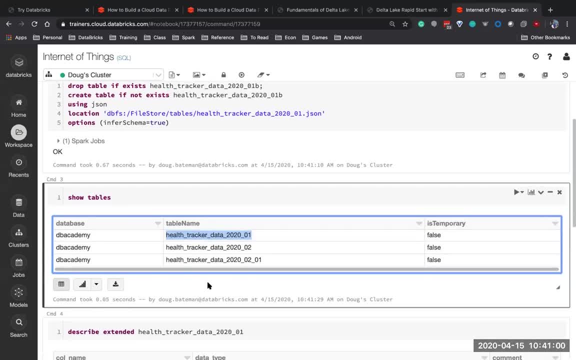 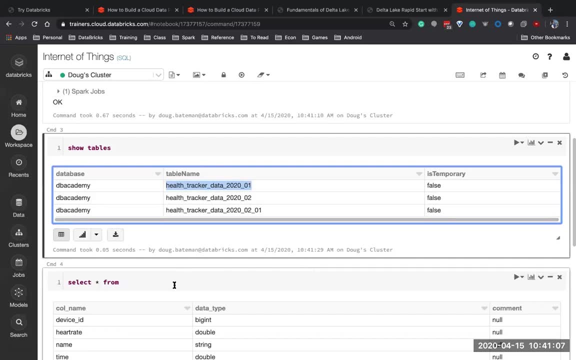 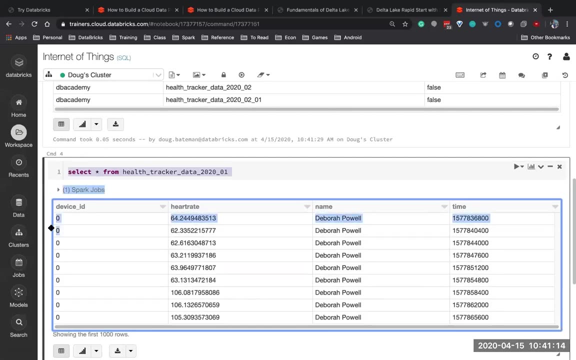 my table has changed And every time I read this table I'm really querying the JSON file. So let's do select star from health tracker 001.. And there it is. This is my data. I've got the device I'm looking at. 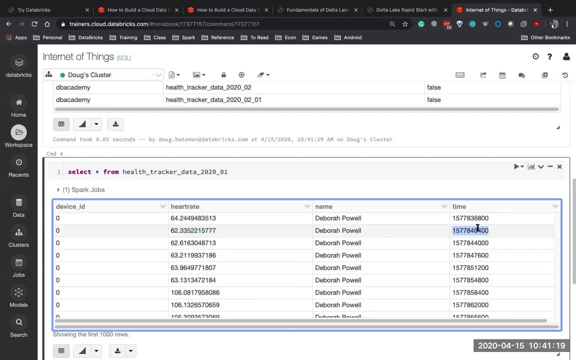 It's heart rate, who owned it? when did I capture this heart rate, et cetera. So this is my Internet of Things- data for a health tracker- And I brought it into to my Delta Lake And somebody asked me a question. 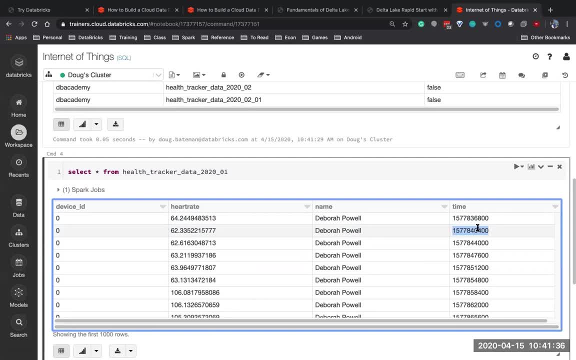 Does everybody have access to this Delta Lake or Delta layer? So this is Rohini's question. Rohini, the answer there is that the Delta Lake is the implementing technology for a data lake. So a data lake may include Delta files. It may also include JSON files. 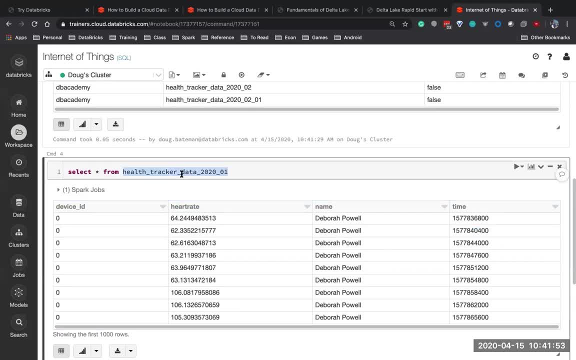 So in this case my data lake has got JSON files in it currently. This SQL table is not currently a Delta table. So that answers Shlomit's question. This is not currently a Delta table. It is in my data lake but it's backed by JSON at the moment. 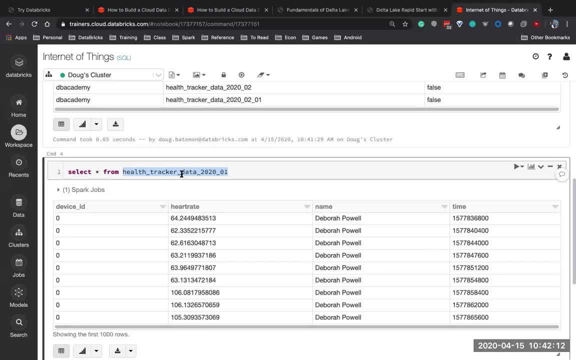 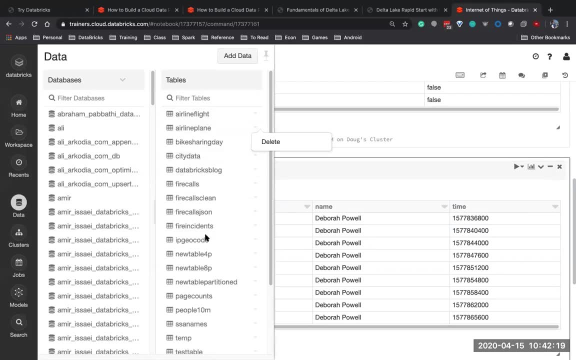 And. but notice that because it's registered as a table, people have access to it. Now, if you have the enterprise security package at Databricks, you can even attach ACLs- access control lists to individual tables in Databricks, which is really nice. So I'm going to go ahead and do that. I'm going to go ahead and do that. So I'm going to go ahead and do that. So I'm going to go ahead and do that. Other people are asking. 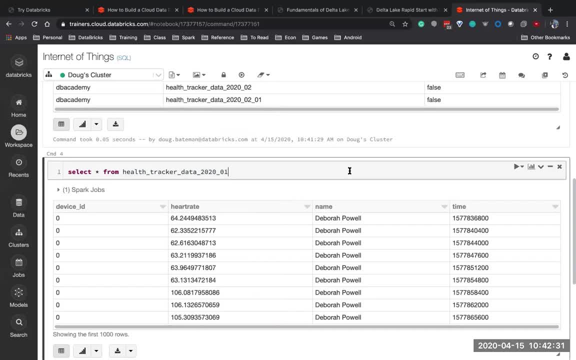 how do you refresh these tables on a schedule? We will actually dig into how do we go about refreshing tables on a schedule, because we're going to be doing various jobs to refresh them, But this is where the jobs tab in Databricks comes in. 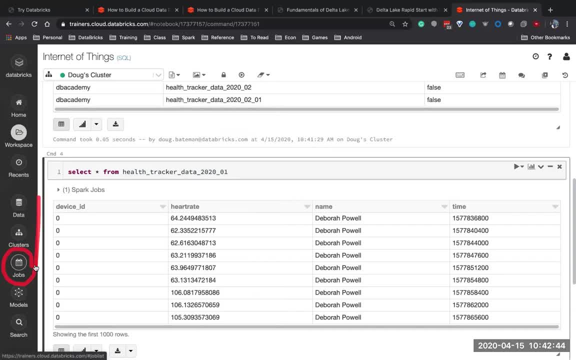 because you can set a schedule to run code that's going to be refreshing the tables. But keep in mind, right now this table is in fact a JSON file, So Databricks is not a and Spark is not a database. It's a query engine. 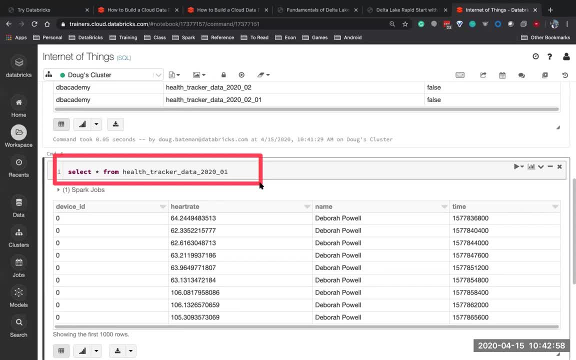 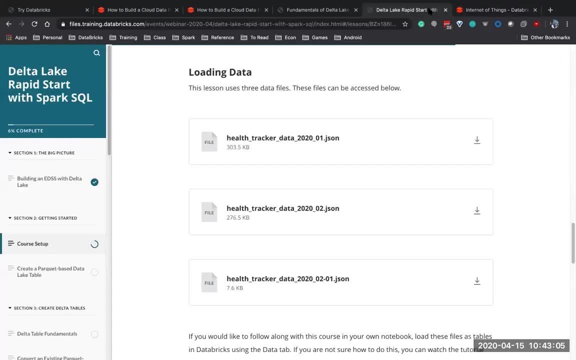 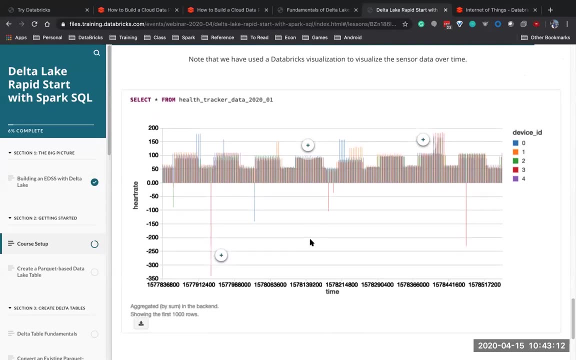 That's working on top of these underlying files in our data link. That's a really important distinction. All right, So let's keep going. at this point, We've uploaded our files, We've made this data available And we would like to just take a quick peek at it. 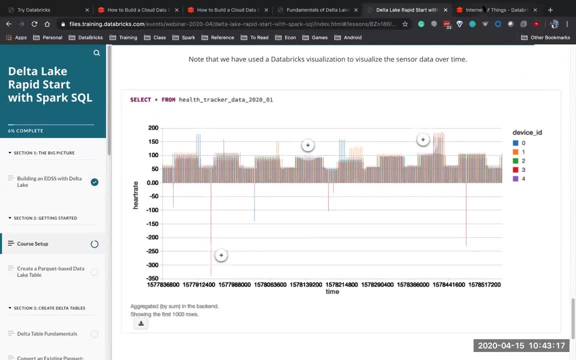 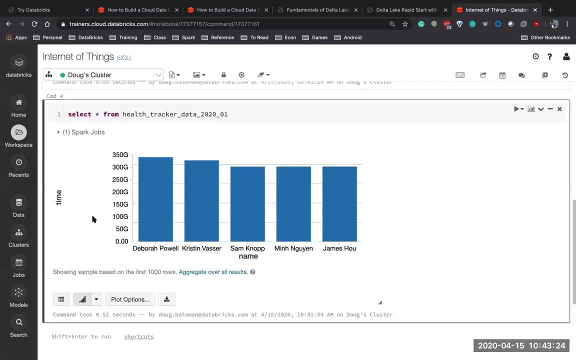 So let's do a plot: select star from health tracker data And let's make a plot out of it. So I've already done the select star, But I could come in here and do a bar chart And right now the bar chart. 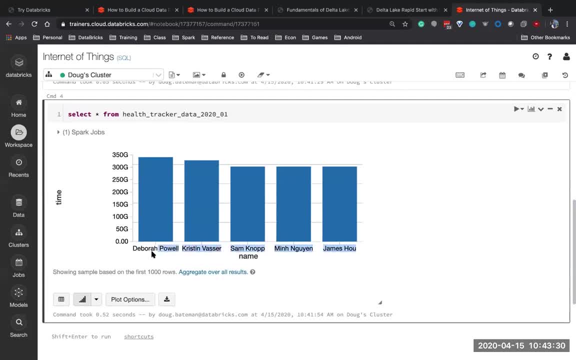 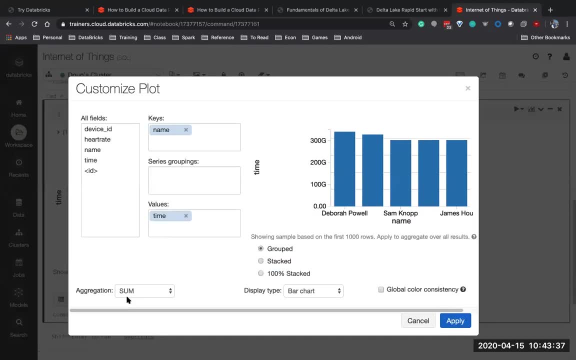 it just kind of pick which columns to use So we could see how much data I have for people, And in this case it's summed up the time column. Well, that's not at all the plot I want, So I come here to plot options. 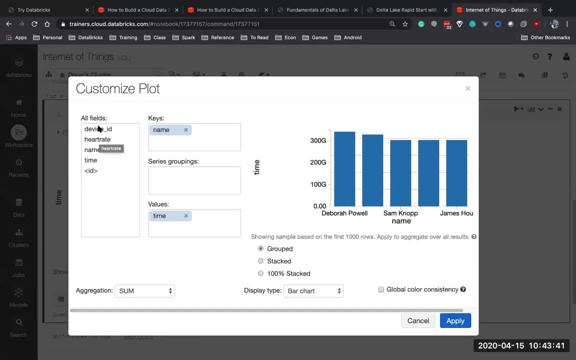 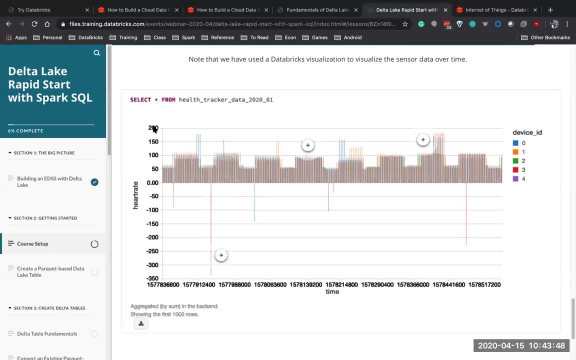 And what I really want to do is look at. let's see here, Let's look at the chart we're aiming to get. I want time along this axis and heart rate along this axis, And I want to split it up by device ID. 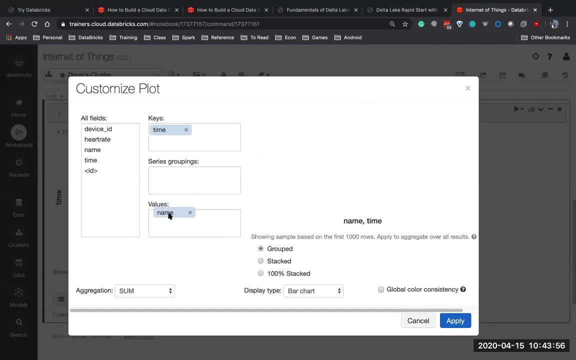 All right. So I'm going to Make the keys be time, I'm going to make the heart rate be the value And I'm going to split this up by device ID. And now I click And I want to look at the number of data points that I have. 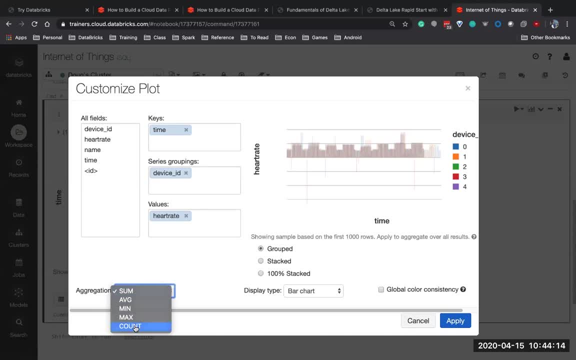 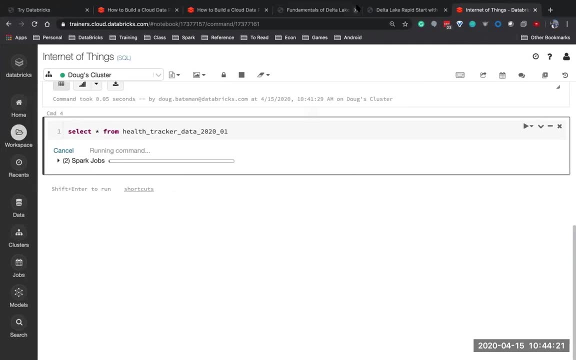 So I'll go to count, as opposed to summing up, your heart rate. I want to look at how many heart rate measures I have, And now I click apply. Let me just compare that here to the course. So the course looks like it was actually. 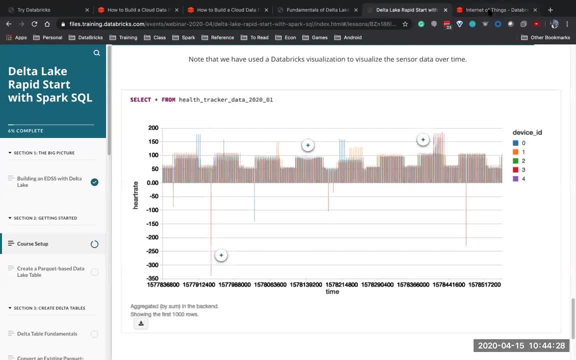 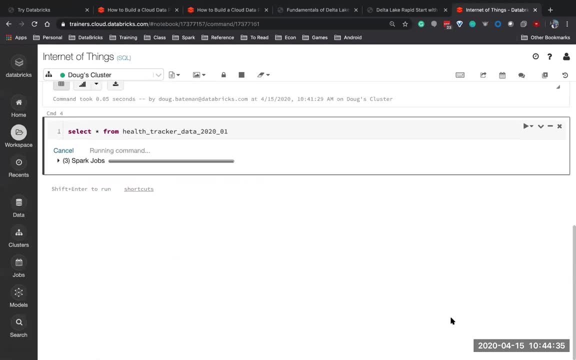 I'm looking at the average heart rate Now. it aggregated by sum in the course. So maybe instead of doing a count, I'm going to do average, And now I can look at people's average heart rates. There we go. 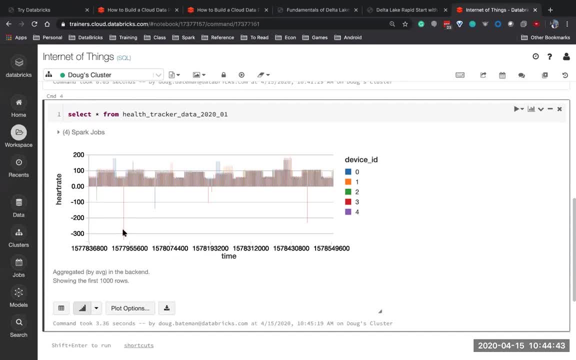 And this is a little disturbing. I've got some data points in here where I have a negative heart rate. I guess that means your heart is beating backwards. Well, clearly this is bad data that we're going to have to clean up as part of our data cleansing process. 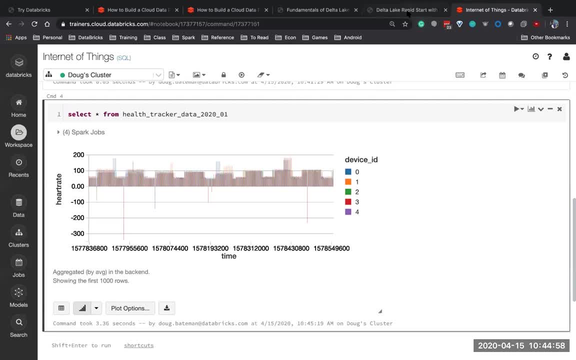 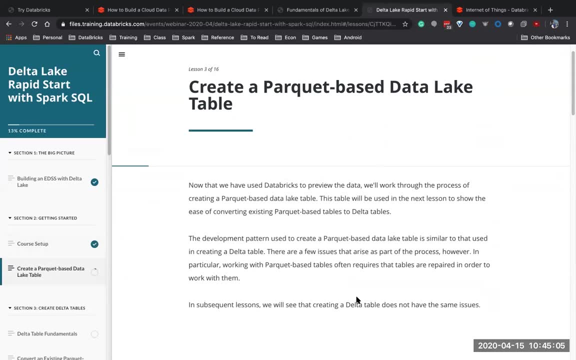 So let's continue on here. I'll click continue. So the first thing we want to do is keep in mind: JSON is fine for our ingest process, but it's a very slow file format to read, because every single time I run this query. 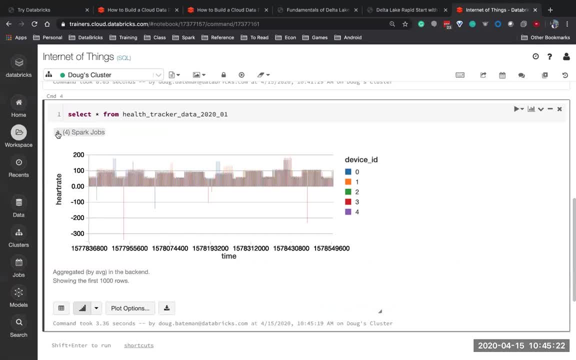 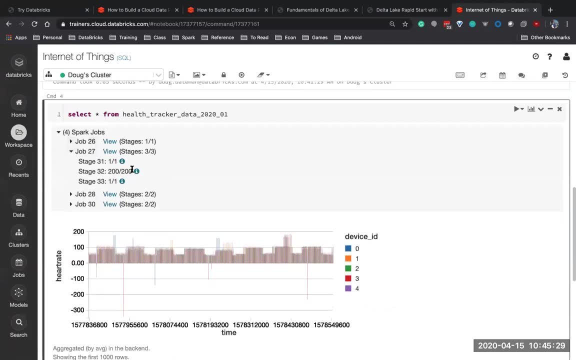 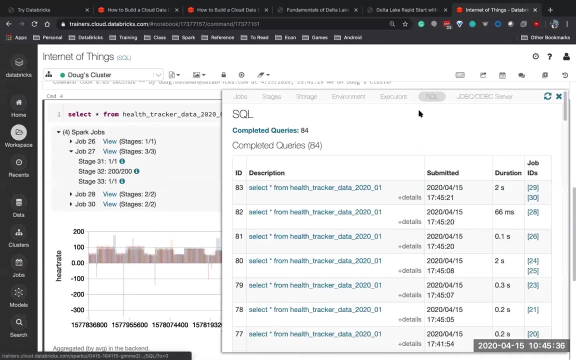 I've got to parse the JSON file Just to illustrate this. let me expand the Spark job And let's come here to the second Spark job and take a look at what this looks like. Actually, I'm going to come to the SQL tab and I'll look at this query that we just ran. 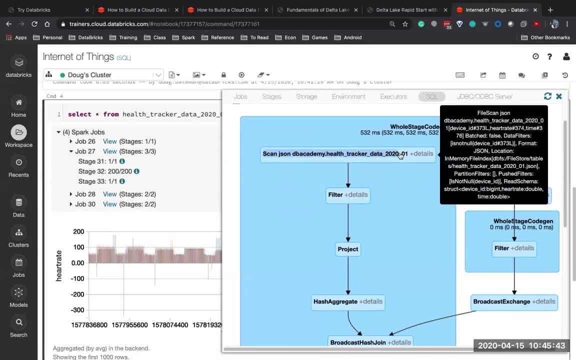 And notice that here it's scanning the JSON file. So it's reading a JSON file every time I run a query, So it's got to parse that file every time I run a query, which is nice. So it's not very fast at all, but then you could see I'm filtering out data. 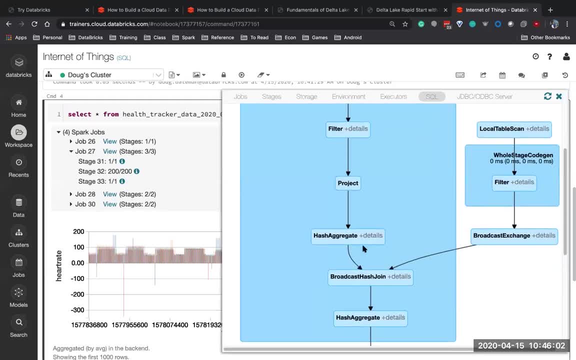 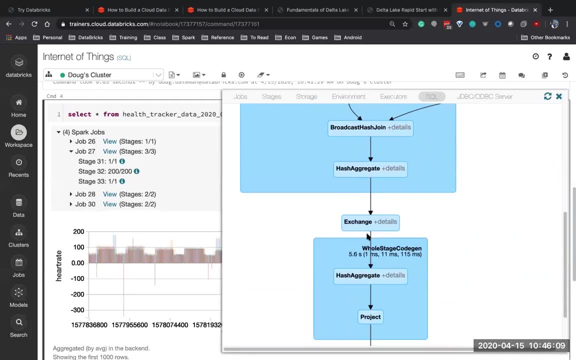 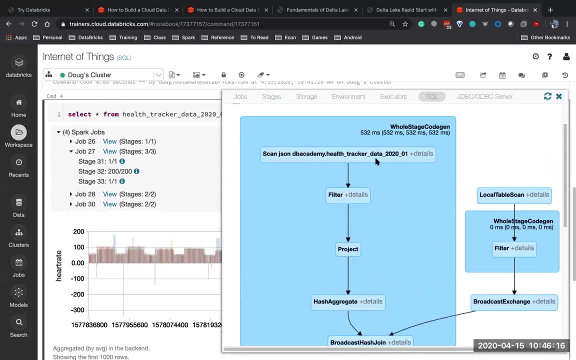 I'm selecting only the device ID, the heart rate and the time. I'm then doing a group by operation so that I could do the average heart rate And eventually I get my final result that I'm displaying in this plot So you can actually view the physical query plan. 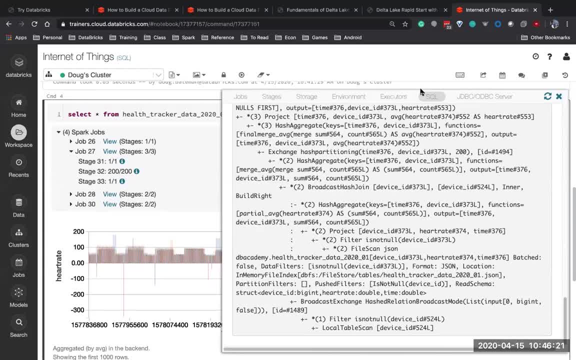 You could also view that query plan as text down here and that's all available inside of the SQL tab when I view the JSON file. And you can also view the job details. And somebody who wants to learn how to do performance optimization will need to learn how. 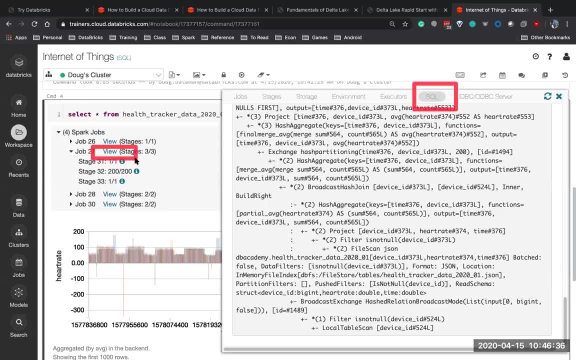 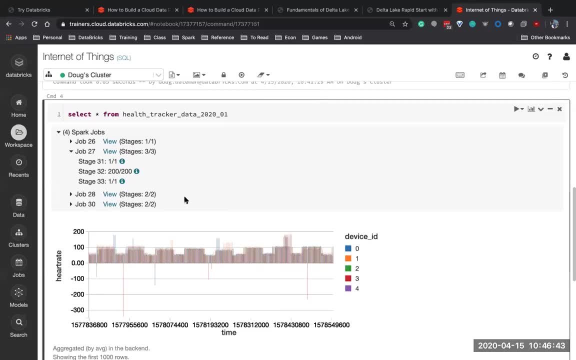 to read these query plans to figure out what is taking so long in your query, And you could do performance optimization using that part of the UI. That's beyond the scope of what we're talking about today, All right, But this is my query and you could see that I was able to successfully run it. 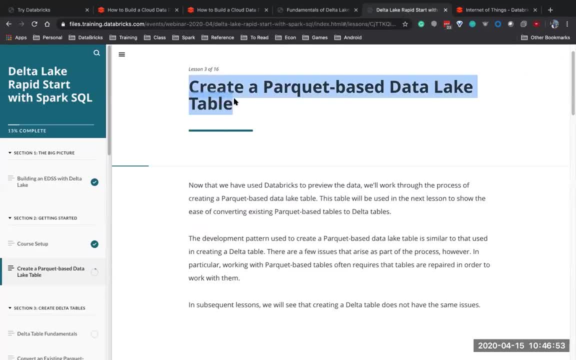 But I'd like to. the first thing I'd like to do would be to get it into a faster file format. Now, just for the benefit of making a narrative, we'd like to first turn this into a Parquet file. Now, in Truett, I would rather use a Delta file format. 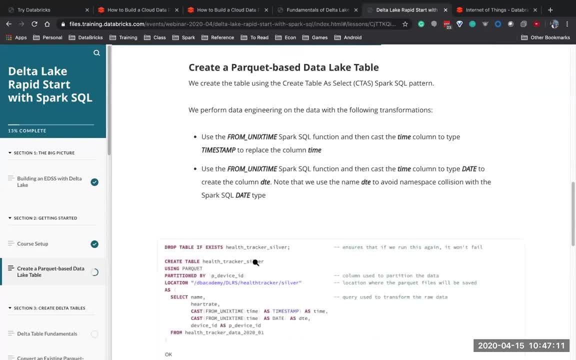 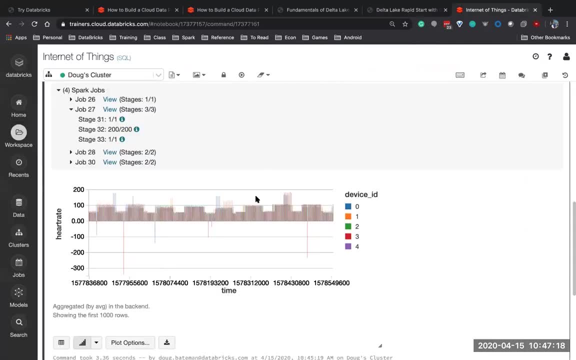 But a lot of people already have their data out there in Parquet. So what I'm going to want to do is convert this data from JSON into Parquet. So I'll come in here and I'm going to say: drop table, if exists. Well, I don't have it. So I'm going to say drop table if exists. Well, I don't have it. So I'll come in here and I'm going to say drop table if exists, Well, I don't have it. 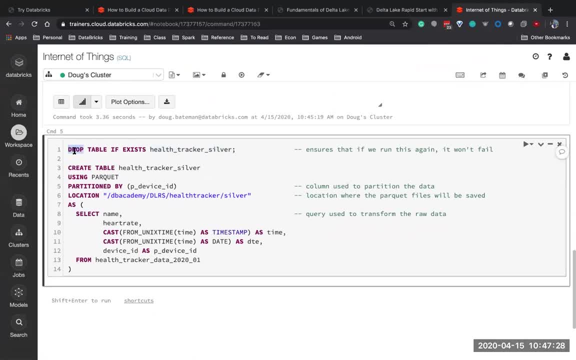 have the table yet. but this is just to make it so that if I run my notebook a second time it would drop that table and rerun this code. so the first time this is actually kind of a no-op, because the table doesn't exist. but then I'm going. 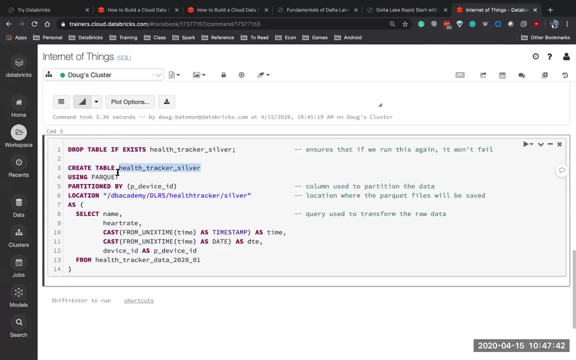 to say, create table health tracker silver using parquet and I give it a location to put that file using parquet. I'm gonna have it break up the data on disk by device ID. I don't have to, but you're able to partition the data by different parts if you needed to. 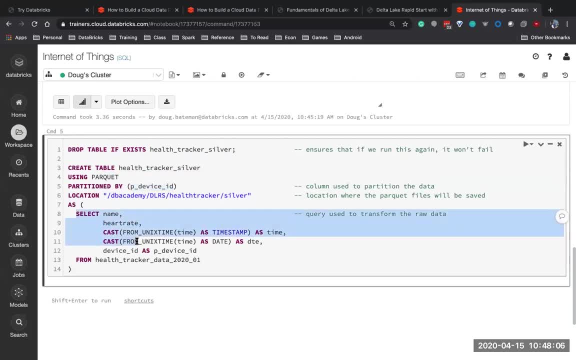 on disk to make the file smaller and then I give it the query that I want to run to populate this parquet file and we're going to read the original JSON data to do that and we're gonna read that timestamp that was coming in as a. 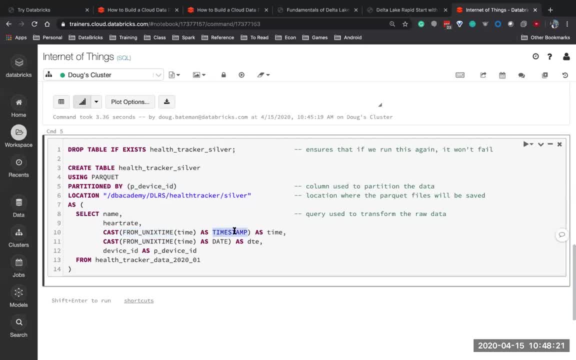 double and we're going to come in and we're going to come in and we're going to convert this to be a Unix timestamp and we're also going to grab the date. so we're going to grab the Unix timestamp and the date. so we're doing some data. 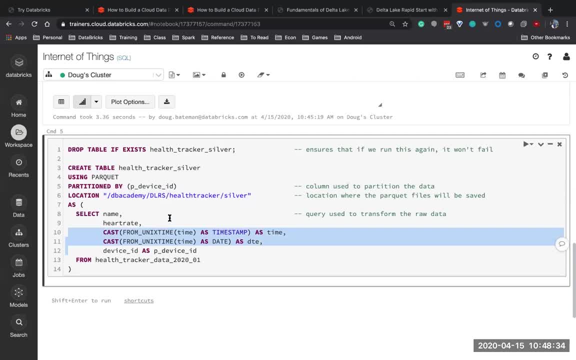 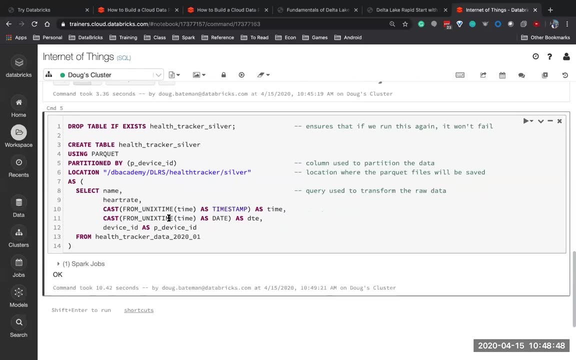 cleansing as we go and putting it into a better file format suitable for reads, and parquet and Delta are by far the better file formats. now a lot of data lakes already have parquet, and parquet and delta are by far the better file formats. now a lot of data lakes already have parquet. 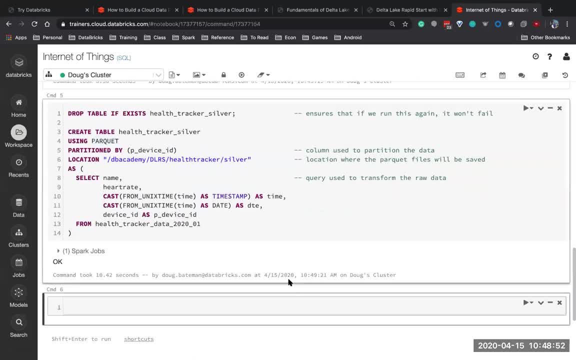 which is why we started by making this be a parquet is just to show you how you would do it if it was a parquet. but we're really interested in using Delta. Delta is an improvement on the parquet file format, so let's convert this to be. 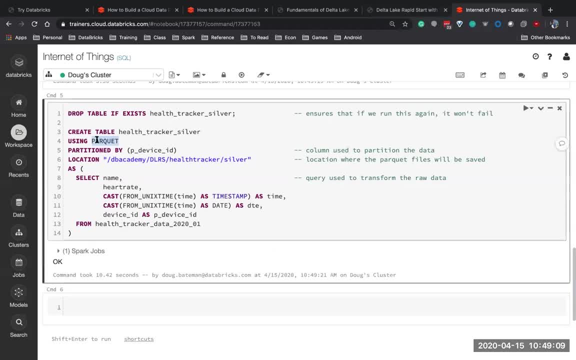 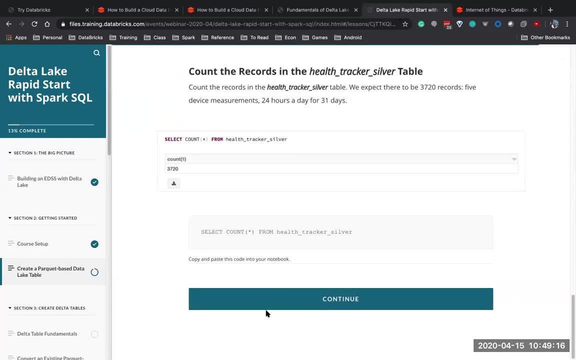 a Delta table instead. so let's say that I already have a data lake that's using parquet. could I convert this to be a Delta table instead? and there are a variety of different ways to do this here. I'm going to go ahead and jump ahead. 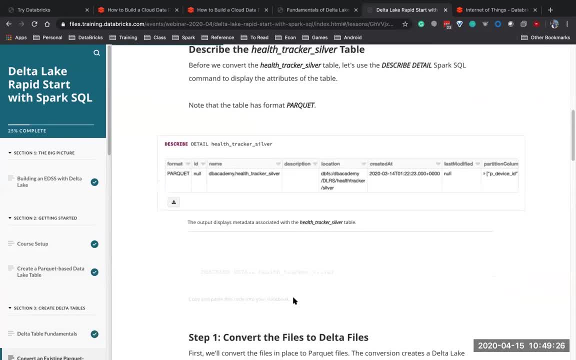 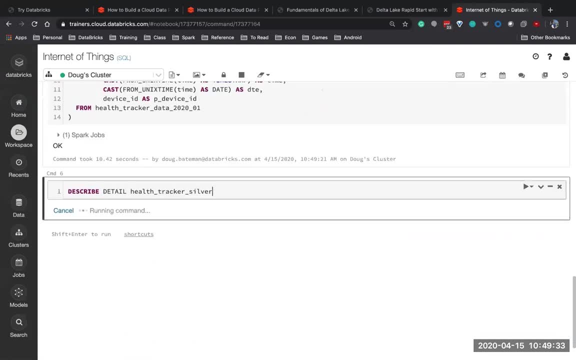 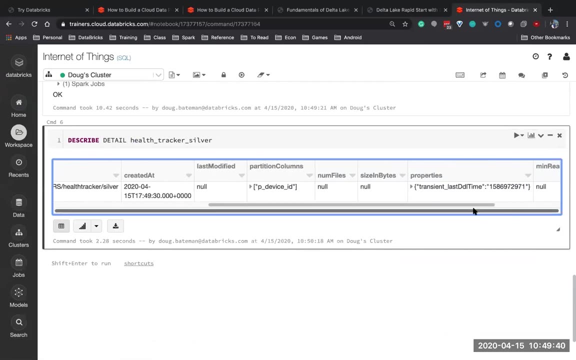 I'm going to go ahead and jump ahead. so first let's look at it and we're going to see that it is in fact a parquet file: describe, detail, health tracker silver. and let's see what we find in here. it is located here and here and 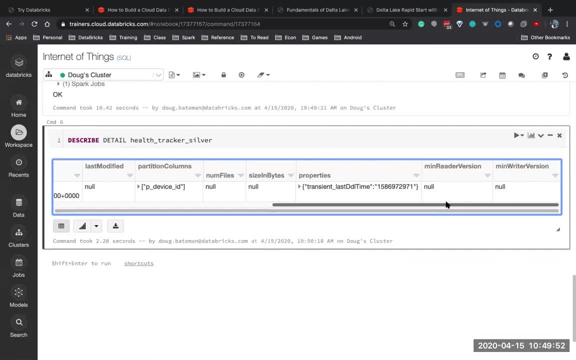 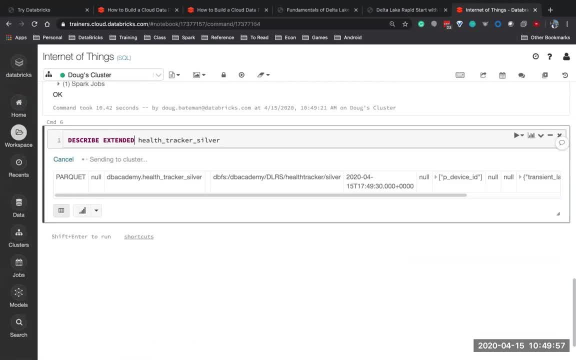 tell me the file format. so I'm gonna go tell me the file format. so I'm gonna go describe extended instead of describe, describe extended instead of describe, describe extended instead of describe detail. and this lets me scroll down and detail. and this lets me scroll down and 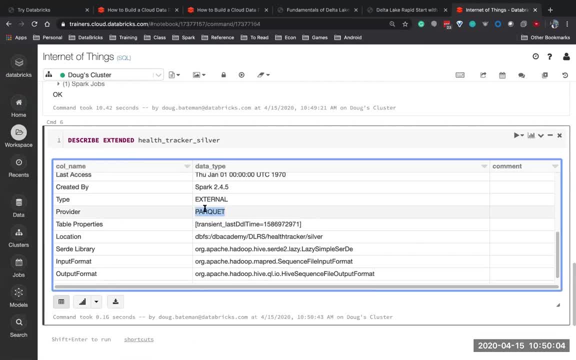 detail. and this lets me scroll down and see- yes, in fact it is a parquet file. see, yes, in fact it is a parquet file. see, yes, in fact it is a parquet file. and I want to convert this, Oh somebody. and I want to convert this, Oh somebody. 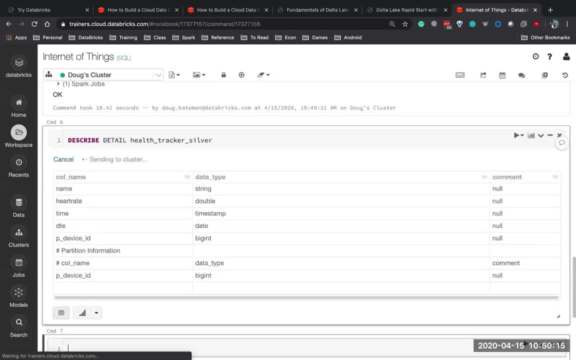 and I want to convert this. Oh, somebody says I missed it. apparently the says I missed it. apparently the says I missed it. apparently the described detail did tell me the file described detail did tell me the file described detail did tell me the file format. let's go back up. there it is. 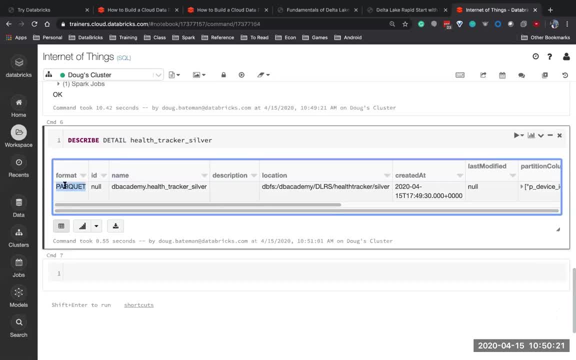 format. let's go back up there. it is format. let's go back up there. it is first column. it was there. I was just first column, it was there. I was just first column, it was there. I was just blind because I saw the name over here. blind because I saw the name over here. 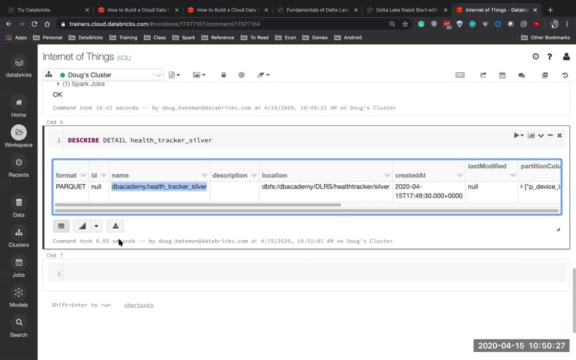 blind because I saw the name over here instead perfect. so I could you describe instead perfect. so I could you describe instead perfect. so I could you describe detail or describe extended- all right, so detail. or describe extended: all right, so detail. or describe extended- all right, so we know it's a parquet file. how can I? 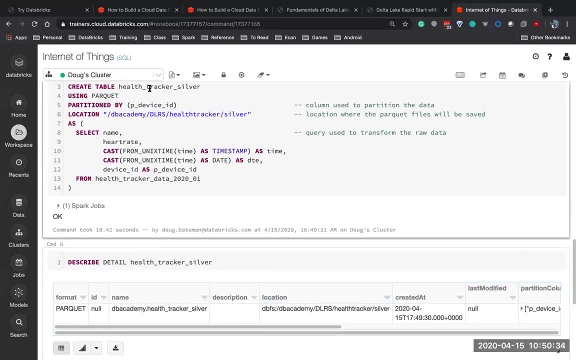 we know it's a parquet file. how can I? we know it's a parquet file. how can I convert a parquet file? well, there's a. convert a parquet file. well, there's a. convert a parquet file. well, there's a couple of options. I could a leave the. 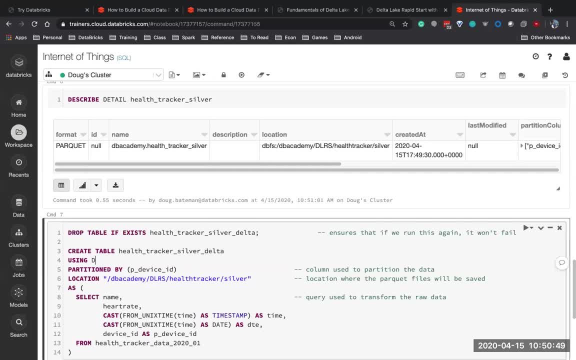 couple of options. I could a leave the couple of options. I could a leave the. I could make a new file and leave the. I could make a new file and leave the. I could make a new file and leave the original one alone if I wanted to, and I. 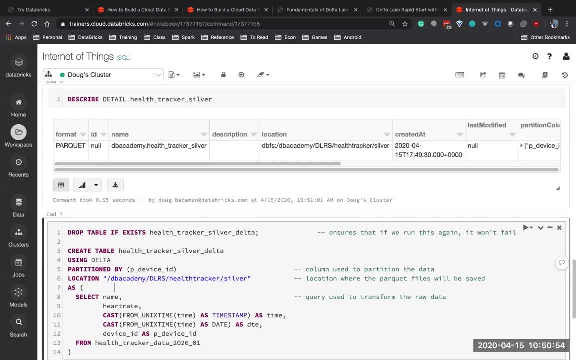 original one alone if I wanted to, and I original one alone if I wanted to, and I would just change it to say use using. would just change it to say use using, would just change it to say use using Delta, and then do a query, just like we. 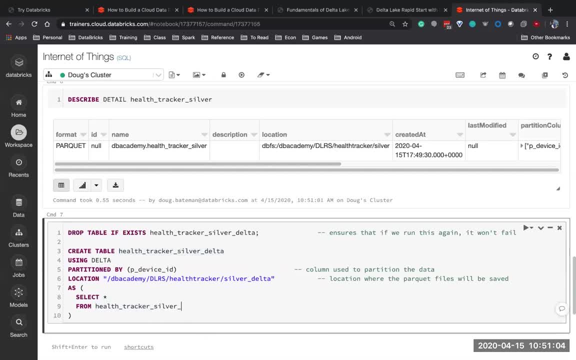 Delta and then do a query just like we Delta, and then do a query just like we did before select star from the old one, did before select star from the old one, did before select star from the old one. I could query and make it and this works. 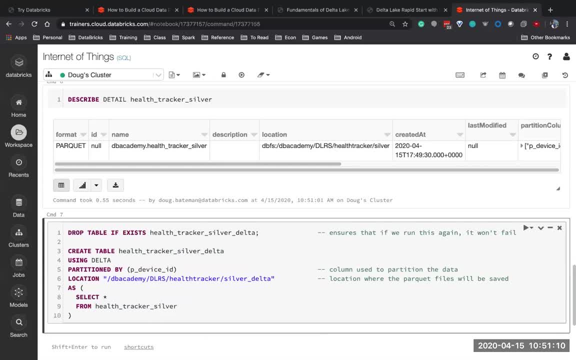 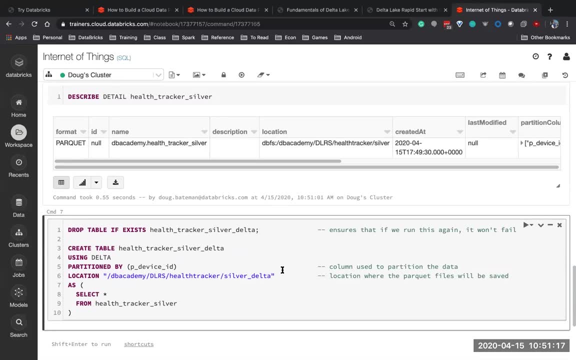 I could query and make it, and this works. I could query and make it, and this works. if I'm willing to make a copy, so this. if I'm willing to make a copy, so this. if I'm willing to make a copy, so this is the parquet, or should be the parquet. 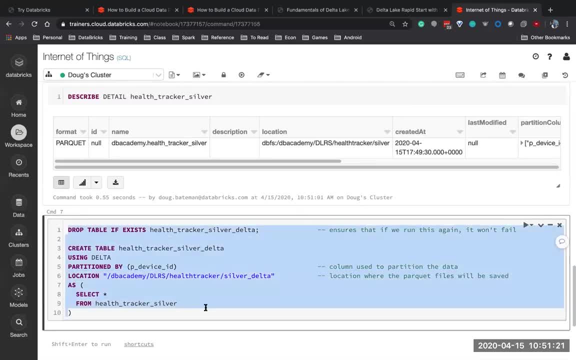 is the parquet or should be the parquet? is the parquet or should be the parquet? table to a Delta in place without table to a Delta in place without table to a Delta in place, without actually making a copy at all? so let's actually making a copy at all. so let's. 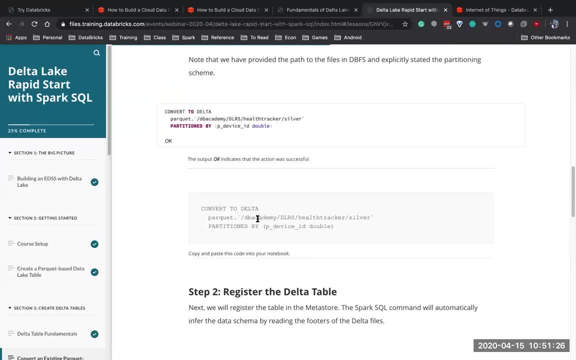 actually making a copy at all, so let's do that instead. so I'm gonna come down, do that instead. so I'm gonna come down, do that instead. so I'm gonna come down here and I'll say: convert to Delta, let's here and I'll say: convert to Delta, let's. 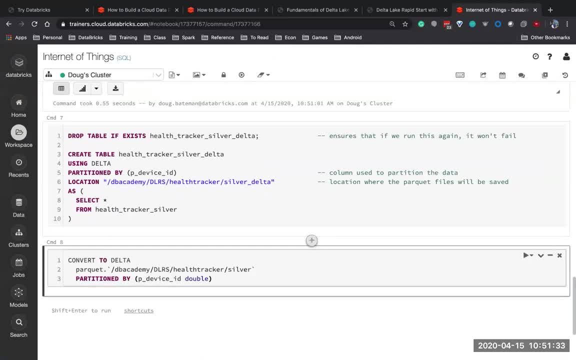 here and I'll say: convert to Delta. let's take a look at what that looks like. take a look at what that looks like. take a look at what that looks like. convert to Delta and I give it the path. convert to Delta and I give it the path. 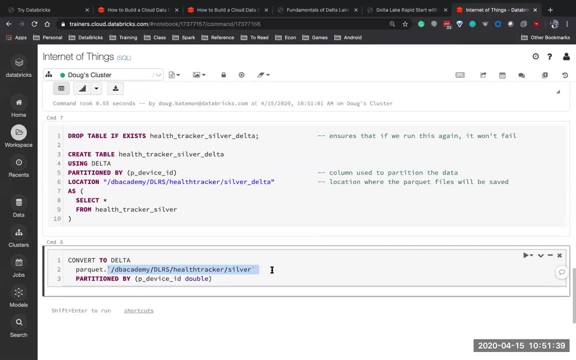 convert to Delta and I give it the path to the file and this is going to go to to the file and this is going to go to to the file and this is going to go to that directory on disk and this is that directory on disk and this is. 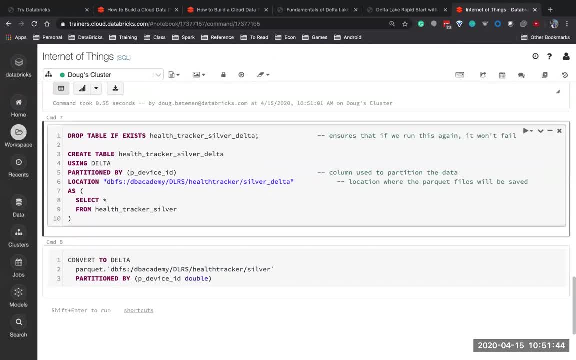 that directory on disk and this is inside of DBFS. if I don't put the inside of DBFS, if I don't put the inside of DBFS, if I don't put the prefix DBFS, it assumes it's DBFS. I'm prefix DBFS. it assumes it's DBFS I'm. 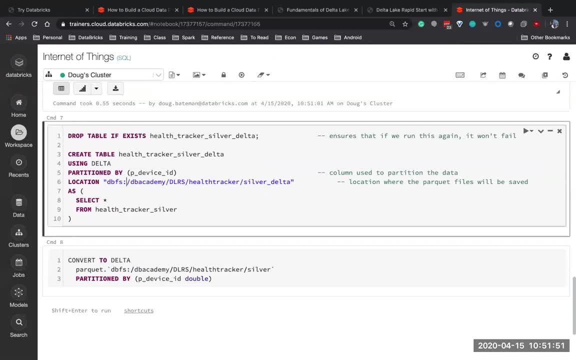 prefix DBFS. it assumes it's DBFS. I'm getting an alert that you can't hear me. getting an alert that you can't hear me. getting an alert that you can't hear me? is anybody else having trouble hearing? is anybody else having trouble hearing? is anybody else having trouble hearing me? just send me a chat message and let. 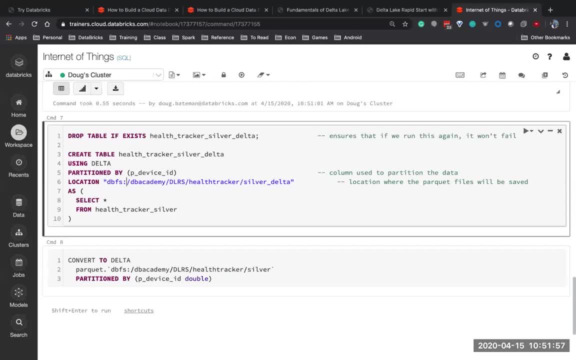 me just send me a chat message. and let me just send me a chat message. and let me know you're able to hear me sometimes. me know you're able to hear me sometimes, me know you're able to hear me. sometimes there's internet issues. no issues. 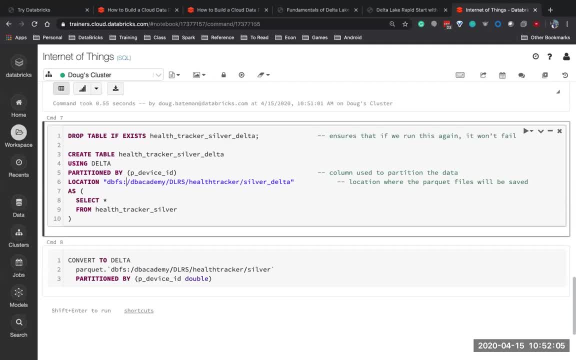 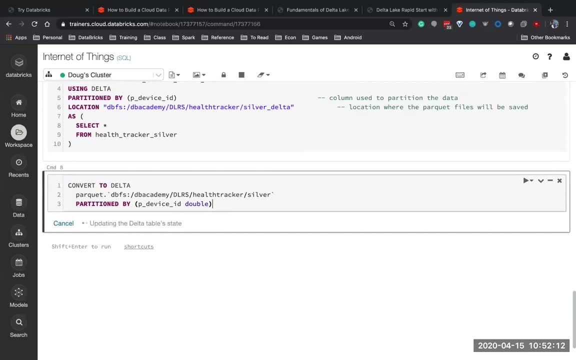 there's internet issues- no issues. there's internet issues- no issues. perfect, thank you everybody, all right. perfect, thank you everybody, all right. perfect, thank you everybody, all right. so I could convert this to Delta on disk. so I could convert this to Delta on disk. so I could convert this to Delta on disk rather than copying the data. I'm just 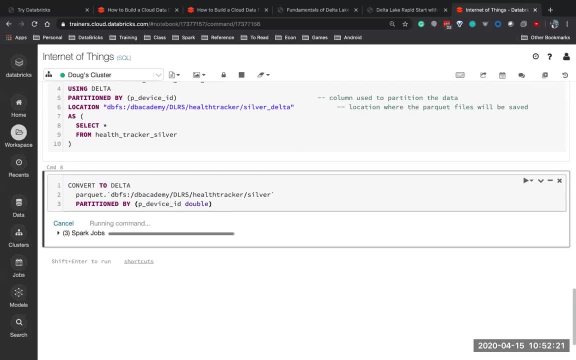 rather than copying the data. I'm just, rather than copying the data, I'm just going to convert a parquet directory to going to convert a parquet directory to going to convert a parquet directory to Delta in situ in place. so it's going to Delta in situ in place. so it's going to. 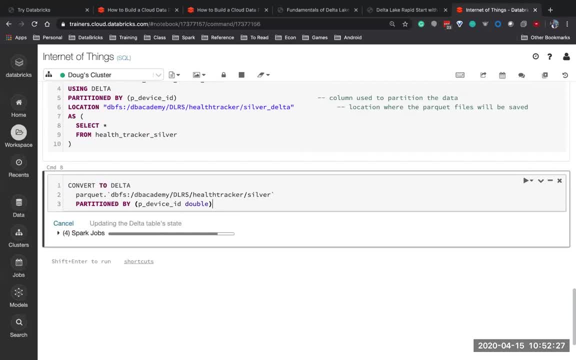 Delta in situ in place. so it's going to do that directory in rewriting it to be do that directory in rewriting it to be, do that directory in rewriting it to be a Delta directory instead, and once I've a Delta directory instead and once I've a Delta directory instead, and once I've done that, what I'm going to need to do. 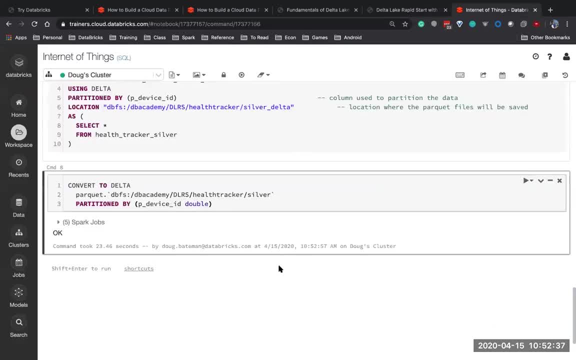 done that, what I'm going to need to do. done that, what I'm going to need to do is to reregister our table to be a Delta is to reregister our table to be a Delta is to reregister our table to be a Delta table. so I'm going to come in here now. 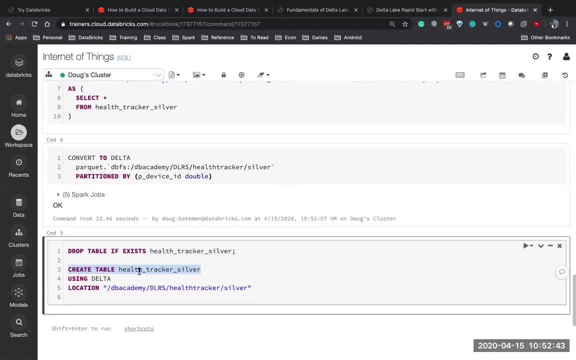 table. so I'm going to come in here now. table. so I'm going to come in here now. drop the old table. remake the table and drop the old table. remake the table and drop the old table. remake the table and I'm pointing it to where those files are. 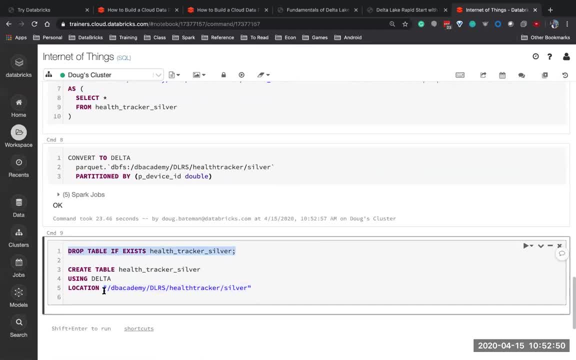 I'm pointing it to where those files are. I'm pointing it to where those files are because the fight, even if I drop the, because the fight, even if I drop the, because the fight, even if I drop the table here, because I'm told it where the 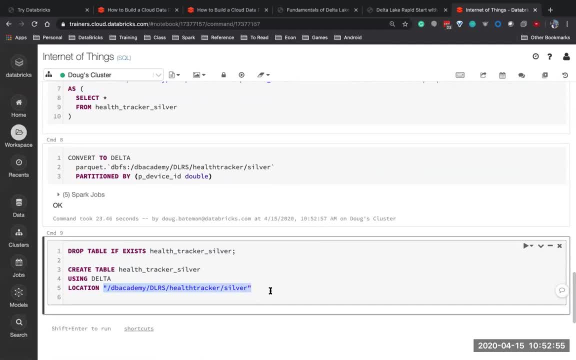 table here because I'm told it where the table here, because I'm told it where the files are. it's actually not deleting files. are it's actually not deleting files? are it's actually not deleting the files on disk? it's just removing the, the files on disk. it's just removing the. 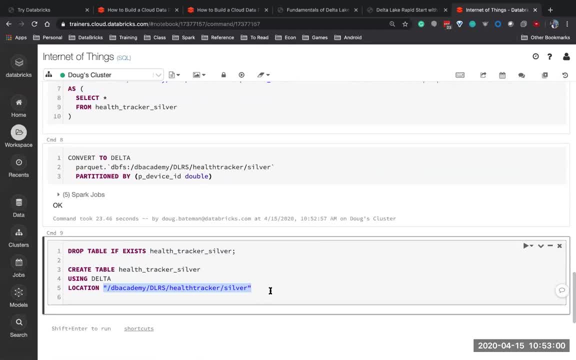 the files on disk. it's just removing the table registration in that Metastore. we table registration in that Metastore. we table registration in that Metastore we talked about the other day. it's just talked about the other day, it's just talked about the other day. it's just removing the identifier for the table. removing the identifier for the table. removing the identifier for the table, it's not actually deleting the files on. it's not actually deleting the files on. it's not actually deleting the files on disk. in this case, it's what you call an disk. in this case, it's what you call an. 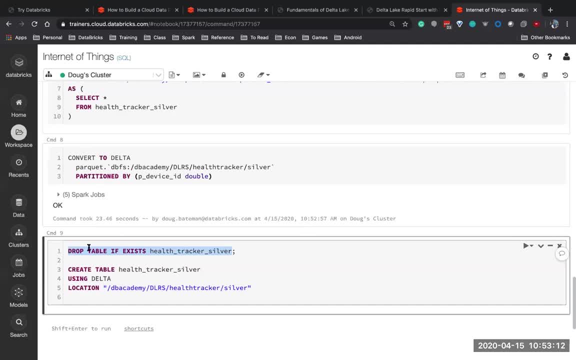 disk. in this case it's what you call an external or unmanaged table. and so I'm external or unmanaged table, and so I'm external or unmanaged table, and so I'm just going to remove it and then just going to remove it, and then 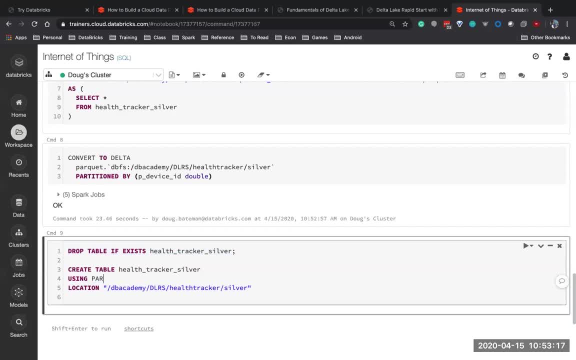 just going to remove it and then recreate the table. telling it that this recreate the table. telling it that this recreate the table. telling it that this table, instead of being a parquet, I have table. instead of being a parquet, I have table. instead of being a parquet, I have officially turned it into a Delta table. 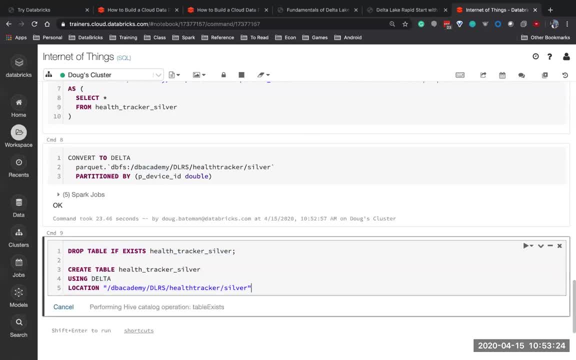 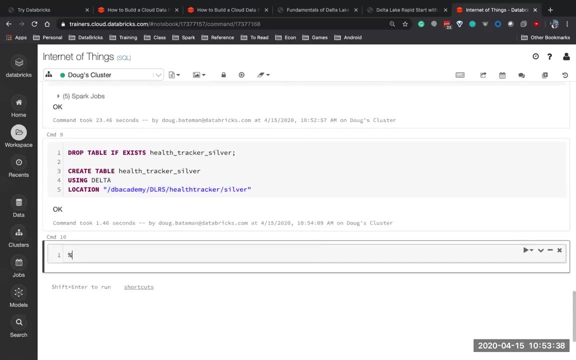 officially turned it into a Delta table. officially turned it into a Delta table. so I say using Delta, so I say using Delta, so I say using Delta. directory look like before and after, but let directory look like before and after, but let directory look like before and after. but let me go ahead and just do this right. 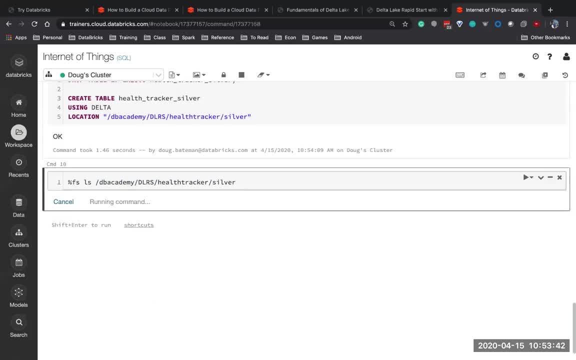 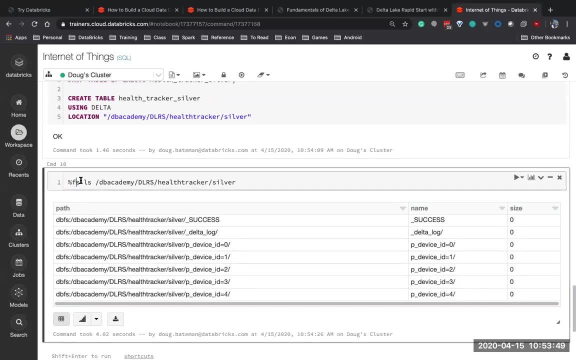 me go ahead and just do this, right me. go ahead and just do this right now. let's take a look at this directory now. let's take a look at this directory now. let's take a look at this directory. so percent file system that says I'm. 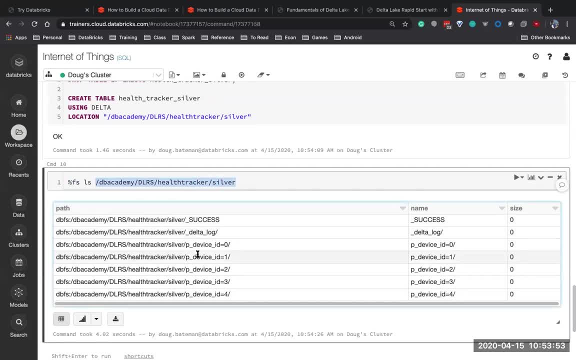 so percent file system. that says I'm so percent file system. that says I'm doing a file system command, and then I'm doing a file system command, and then I'm doing a file system command, and then I'm gonna list this directory and notice. gonna list this directory and notice. gonna list this directory and notice that it's still the same content that I, that it's still the same content that I, that it's still the same content that I would have had if it was notice it's would have had if it was notice it's. 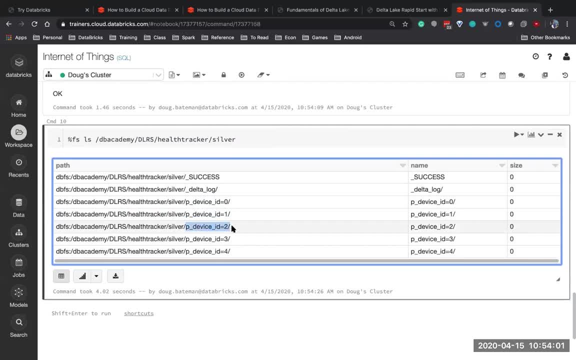 would have had if it was. notice it's partitioned by device, just like a partitioned by device. just like a partitioned by device. just like a regular parquet directory would be. but regular parquet directory would be, but regular parquet directory would be. but when I converted it to Delta it added: 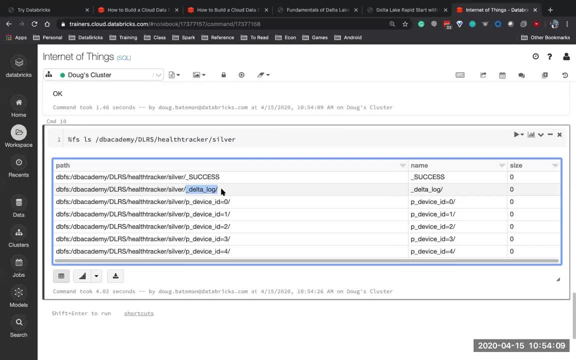 when I converted it to Delta, it added: when I converted it to Delta, it added this subdirectory here called Delta log, this subdirectory here called Delta log, this subdirectory here called Delta log, and the Delta log serves as this and the Delta log serves as this. 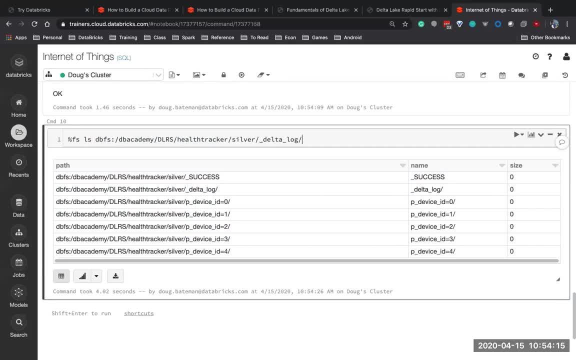 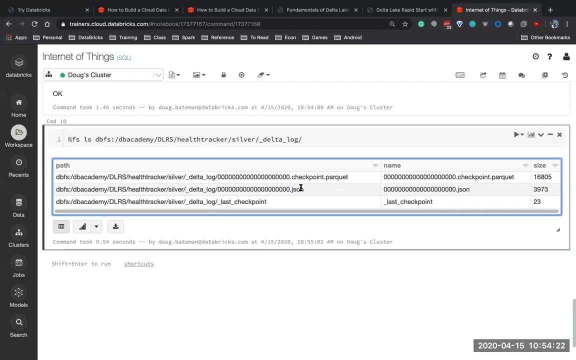 and the Delta log serves as this: transaction log that lists which files. transaction log that lists which files. transaction log that lists which files contain the latest data. so it's really contain the latest data. so it's really contain the latest data. so it's really a JSON file in the Delta log and it lists. 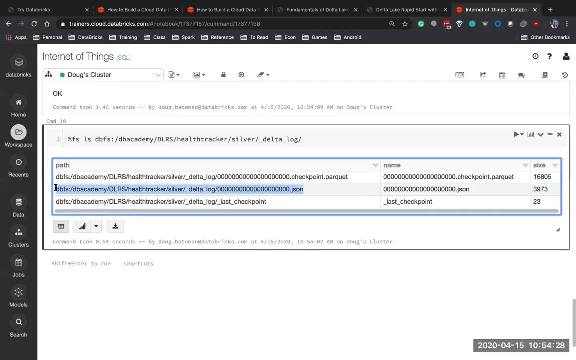 a JSON file in the Delta log and it lists a JSON file in the Delta log and it lists which files contain the latest version, which files contain the latest version, which files contain the latest version of the data. and I'm just going to of the data and I'm just going to. 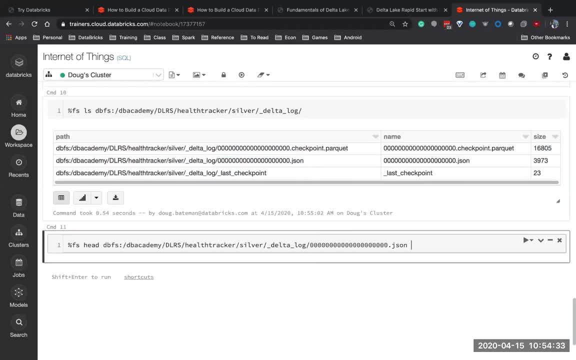 of the data and I'm just going to showcase what that looks like here. percent. showcase what that looks like here. percent. showcase what that looks like here. percent FS head and I'll point out that FS head. and I'll point out that FS head and I'll point out that transaction log notice. it's just a big. 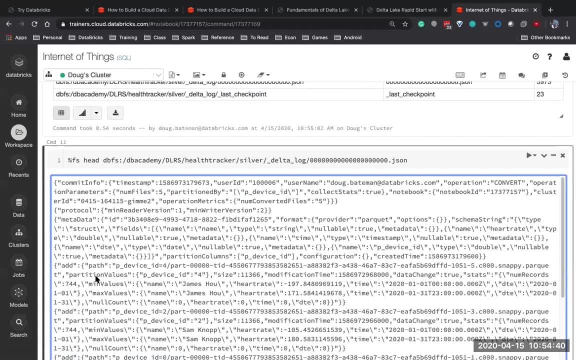 transaction log notice. it's just a big transaction log notice. it's just a big JSON file and it's going to list for JSON file and it's going to list for JSON file and it's going to list for each partition what's the minimum and each partition what's the minimum and. 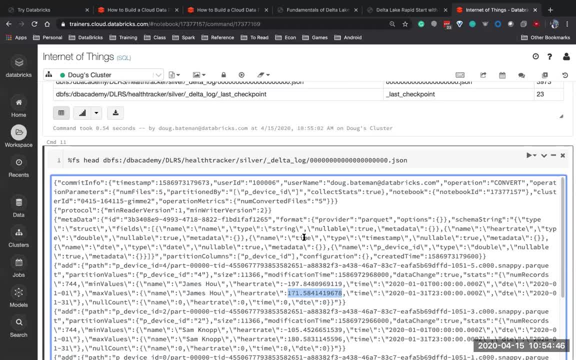 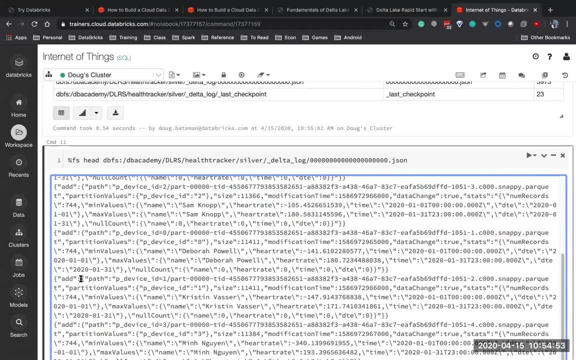 each partition. what's the minimum and maximum value of the heart rate? you can maximum value of the heart rate. you can maximum value of the heart rate. you can individual files like this one, that individual files like this one, that individual files like this one that represent the data having a transaction. 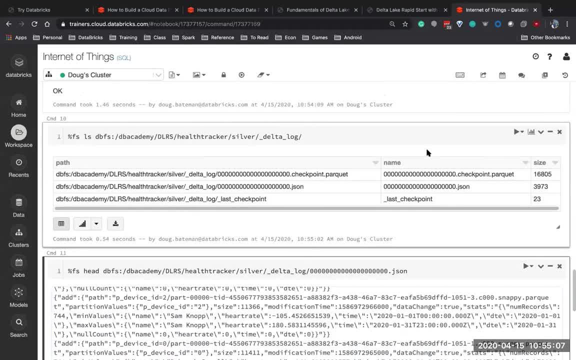 represent the data. having a transaction represent the data, having a transaction log is incredibly powerful. because if I log is incredibly powerful, because if I log is incredibly powerful, because if I go to do an update what it's going to do, go to do an update what it's going to do, 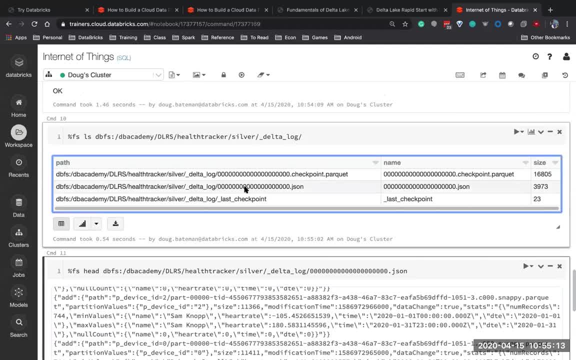 go to do an update. what it's going to do is write out new files and then change is write out new files and then change is write out new files and then change the transaction log. it'll make a new the transaction log. it'll make a new. 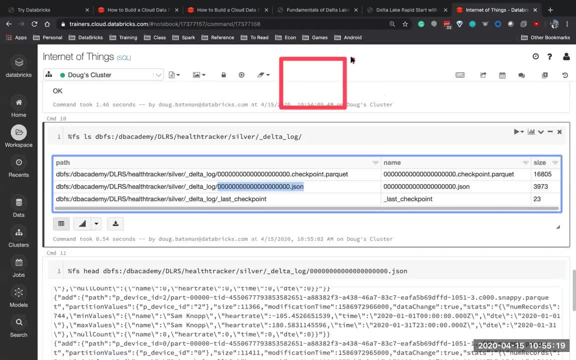 the transaction log. it'll make a new entry in the transaction log saying you entry in the transaction log, saying you entry in the transaction log saying you know, maybe your old data set was these know, maybe your old data set was these know, maybe your old data set was these four files. but you've just done a. 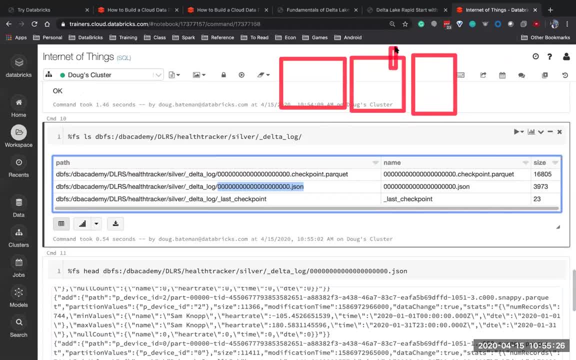 four files. but you've just done a four files, but you've just done a modification to this one. so I'm gonna modification to this one, so I'm gonna modification to this one. so I'm gonna rewrite this file out as a new file and rewrite this file out as a new file, and 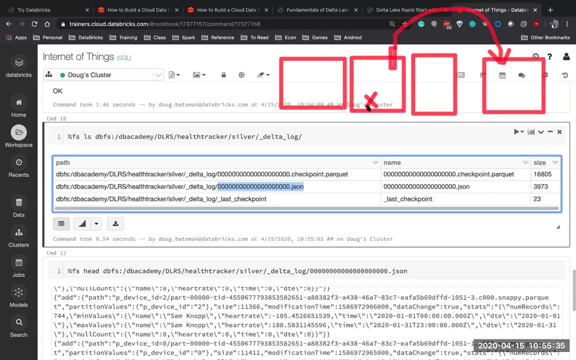 rewrite this file out as a new file and I'm not going to delete the old file. I'm not going to delete the old file. I'm not going to delete the old file, but I'm gonna mark it old. so now my data. but I'm gonna mark it old. so now my data. 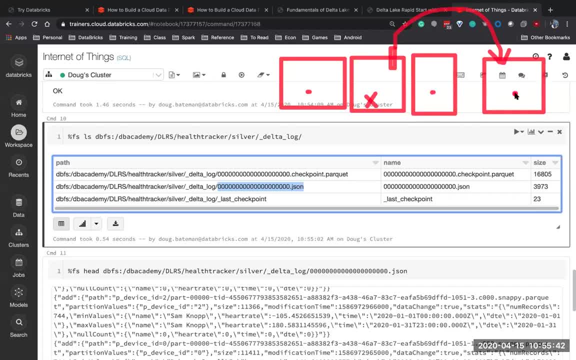 but I'm gonna mark it old. so now my data will be this file, this file and this will be this file, this file and this will be this file, this file and this file on disk. so I'm able to access old file on disk. so I'm able to access old 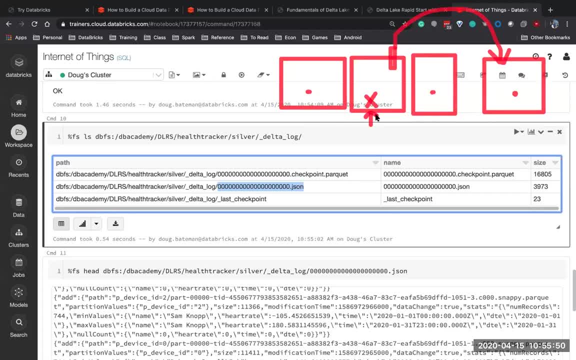 file on disk, so I'm able to access old versions of the data- that's known as versions of the data, that's known as versions of the data that's known as time travel- and I'm also able to start time travel and I'm also able to start. 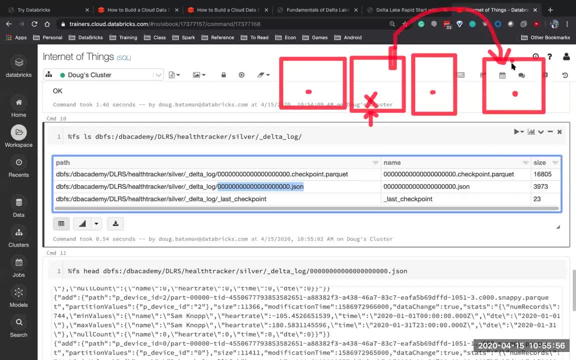 time travel and I'm also able to start writing new files, and only when the new writing new files and only when the new writing new files and only when the new file was written successfully does the file was written successfully. does the file was written successfully? does the old file get marked old in the 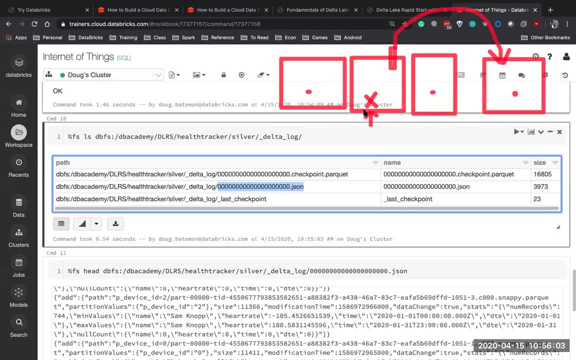 old file, get marked old in the old file, get marked old in the transaction law, and so I'm able to transaction law and so I'm able to transaction law, and so I'm able to achieve versioning as well as atomic, achieve versioning as well as atomic. 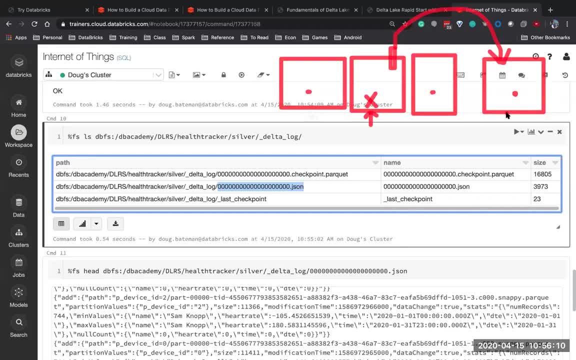 achieve versioning as well as atomic updates. so if in the middle of a write updates. so if in the middle of a write updates. so if in the middle of a write this failed- I would just never mark this. this failed. I would just never mark this. this failed. I would just never mark this file as good and I would never mark this. 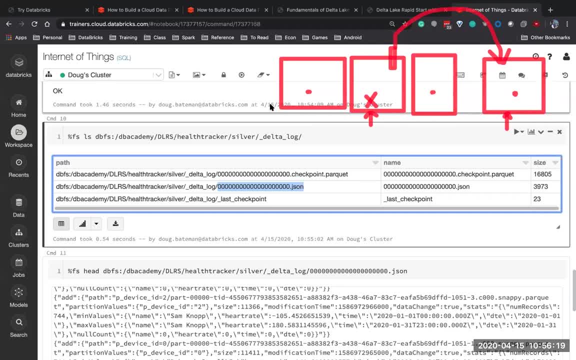 file as good and I would never mark this file as good and I would never mark this file as old. so I get transactionality file as old. so I get transactionality file as old. so I get transactionality because I've got this transaction log in, because I've got this transaction log in. 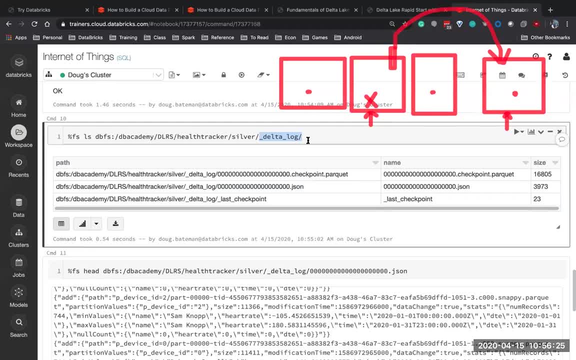 because I've got this transaction log in Delta. it's a critical feature that Delta, Delta. it's a critical feature that Delta, Delta. it's a critical feature that Delta adds on top of parquet but if you look, adds on top of parquet, but if you look, 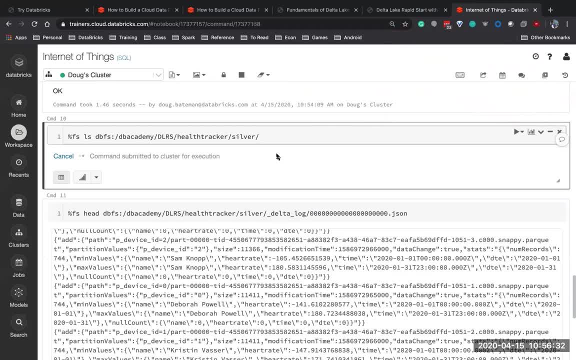 adds on top of parquet. but if you look at the actual files themselves, so let's at the actual files themselves. so let's at the actual files themselves. so let's go in here again and look at the files. go in here again and look at the files. 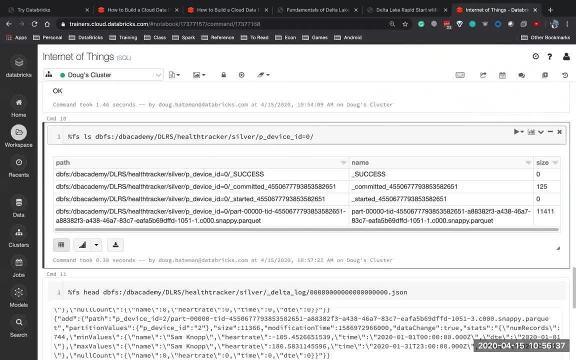 go in here again and look at the files themselves. the file format under the themselves, the file format under the themselves, the file format under the hood is still parquet. what Delta is hood is still parquet. what Delta is hood is still parquet. what Delta is adding is that transaction log and that 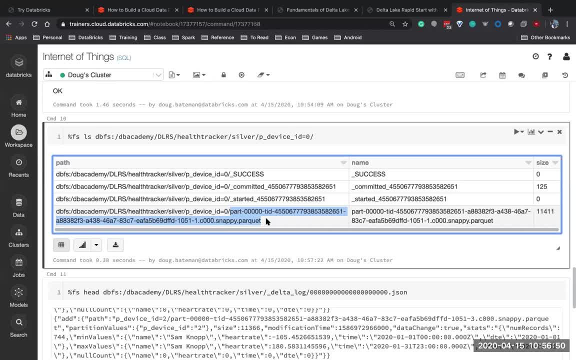 adding is that transaction log and that adding is that transaction log, and that is a critical piece to a cloud data, is a critical piece to a cloud data, is a critical piece to a cloud data infrastructure. now somebody was asking infrastructure. now somebody was asking infrastructure. now somebody was asking: where did the DBS files get stored? so 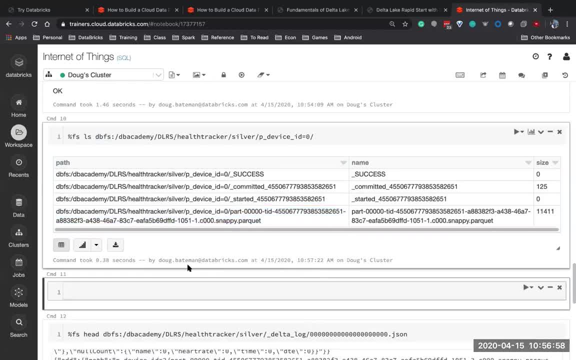 where did the DBS files get stored? so where did the DBS files get stored? so where is this DBFS? so to answer that I. where is this DBFS? so to answer that I. where is this DBFS? so to answer that I could do, for example, percent of mounts. 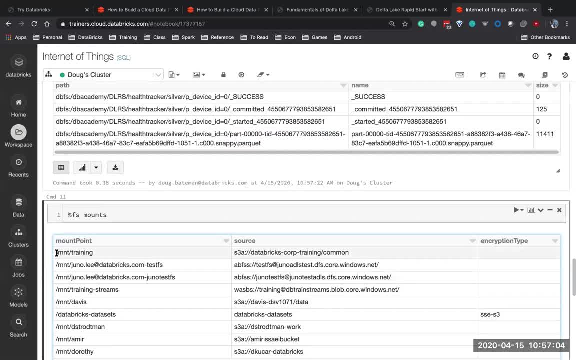 could do, for example, percent of mounts, could do, for example, percent of mounts, and I can see different mount points and I can see different mount points and I can see different mount points, paths and DBFS, and what bucket are they? paths and DBFS and what bucket are they? 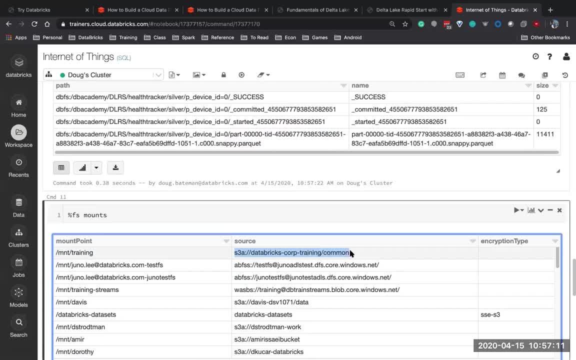 paths and DBFS. and what bucket are they pointing to? so it could be pointing, pointing to, so it could be pointing, pointing to. so it could be pointing here to a s3 bucket or to an azure blob. here to a s3 bucket or to an azure blob. 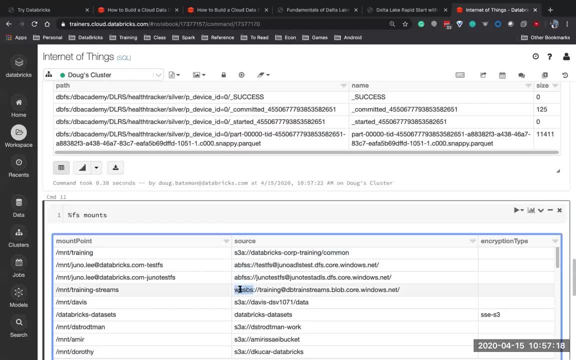 here to a s3 bucket or to an azure blob store bucket. so when does as your blob store bucket? so when does as your blob store bucket? so when does as your blob store? when does as your data lake store store? when does as your data lake store? 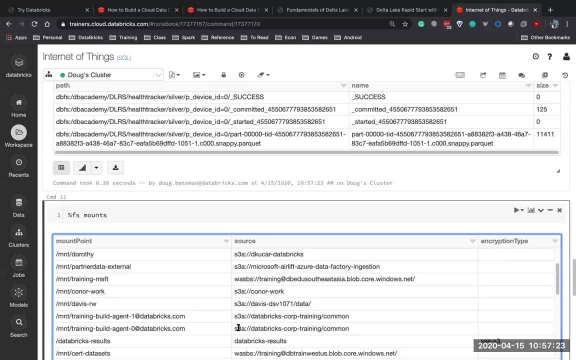 store when does as your data lake store or s3. I'm able to point to a variety of or s3. I'm able to point to a variety of or s3. I'm able to point to a variety of different types of buckets. in this case. 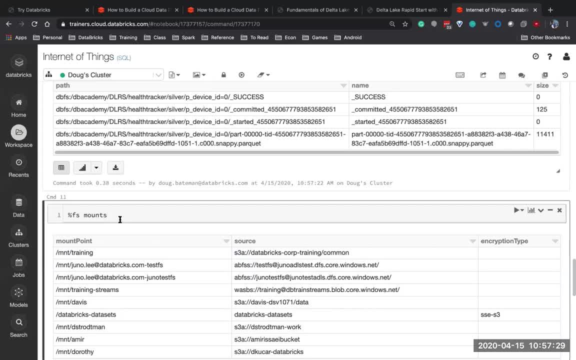 different types of buckets, in this case, different types of buckets. in this case, I'm not actually in the mount directory. I'm not actually in the mount directory. I'm not actually in the mount directory, so there's what's known as the root. so there's what's known as the root. 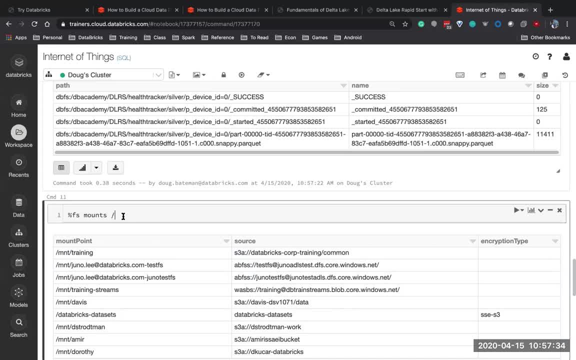 so there's what's known as the root bucket. that would correspond to the top bucket, that would correspond to the top bucket, that would correspond to the top, and again because this particular and again, because this particular and again because this particular workspace is deployed in AWS that itself. 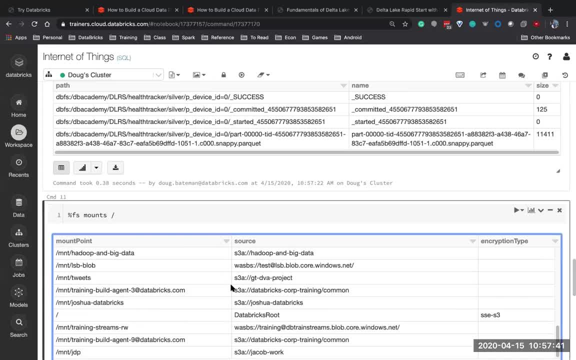 workspace is deployed in AWS, that itself workspace is deployed in AWS. that itself would map to an s3 bucket. so the root would map to an s3 bucket. so the root would map to an s3 bucket. so the root bucket. you see, if it even shows up here. 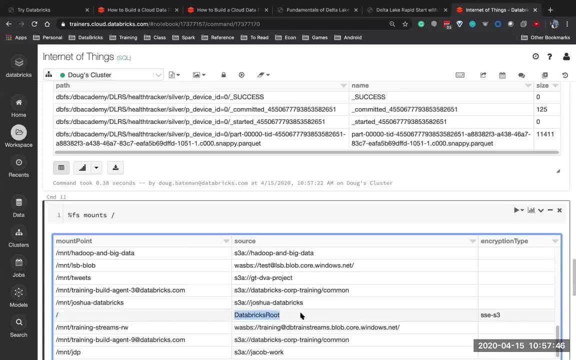 bucket. you see if it even shows up here. bucket. you see if it even shows up here. it is databricks root is itself a bucket. it is databricks root is itself a bucket. it is databricks root is itself a bucket in s3. now Corinne asked what would 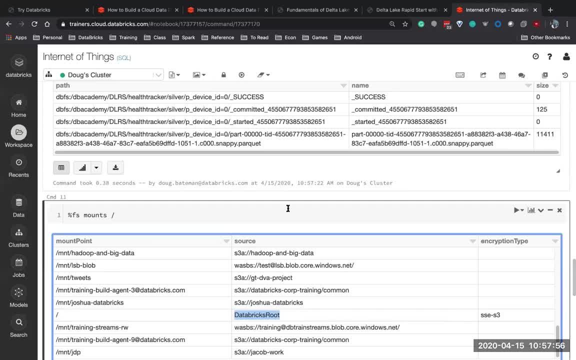 in s3. now Corinne asked: what would in s3? now Corinne asked what would happen if the table wasn't converted to happen. if the table wasn't converted to happen. if the table wasn't converted to Delta- well, if the table had not been Delta. well, if the table had not been 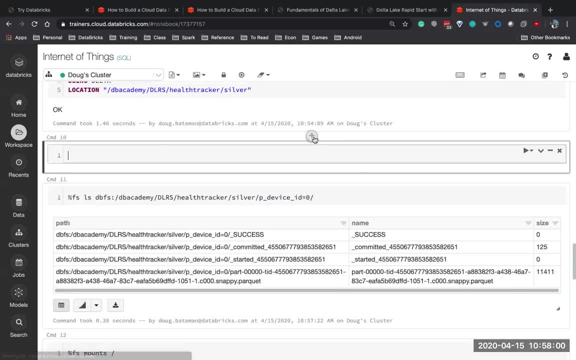 Delta. well, if the table had not been converted to Delta, it's no big deal for converted to Delta, it's no big deal for converted to Delta, it's no big deal, for example. I can continue to query the example. I can continue to query the example. I can continue to query the original health tracker table select. 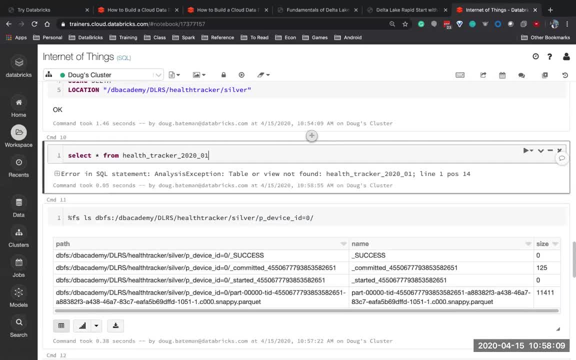 original health tracker table. select original health tracker table. select star from health tracker 2020-01. what star from health tracker 2020-01? what star from health tracker 2020-01? what was it called file name so I can query. was it called file name so I can query. 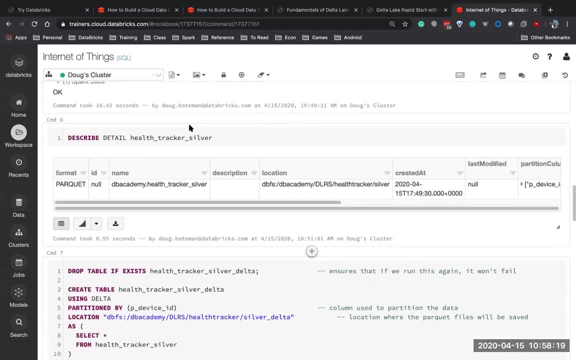 was it called file name, so I can query the original JSON file and in fact I the original JSON file and in fact I the original JSON file and in fact I could have queried the original parquet, could have queried the original parquet, could have queried the original parquet file. so I'm able to use file formats. 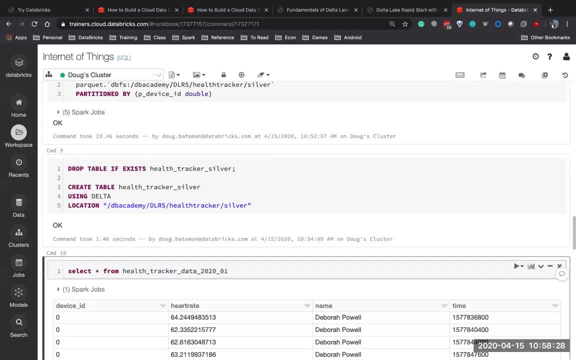 file, so I'm able to use file formats. file, so I'm able to use file formats that aren't Delta. if I wanted to Delta, that aren't Delta. if I wanted to Delta, that aren't Delta. if I wanted to Delta simply adds that versioning and 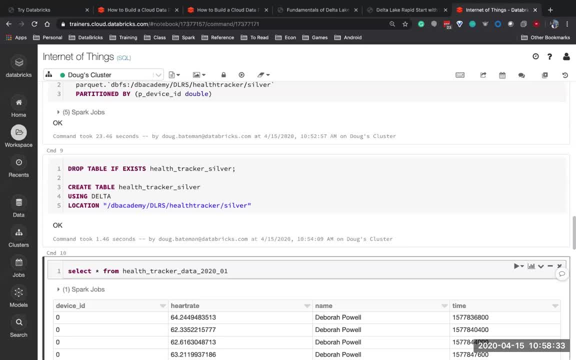 simply adds that versioning and simply adds that versioning and transactionality and a bunch of indexing transactionality and a bunch of indexing transactionality and a bunch of indexing capabilities to make things faster. so we capabilities to make things faster, so we capabilities to make things faster. so we like Delta because it's more robust and 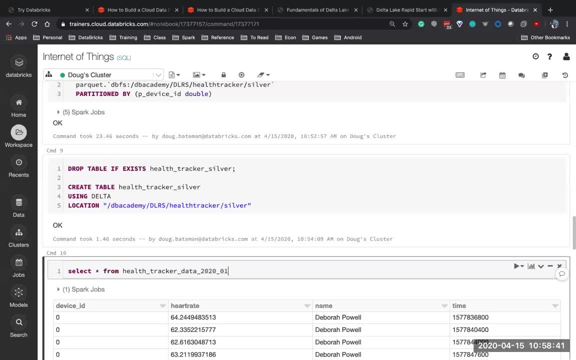 like Delta because it's more robust. and like Delta because it's more robust and faster, but spark is able to work with faster. but spark is able to work with faster. but spark is able to work with parquet. it's able to work with other parquet. it's able to work with other. 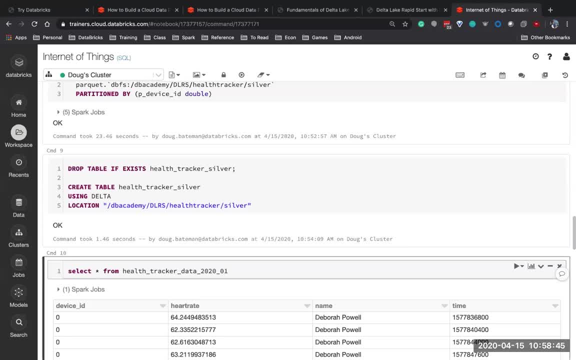 parquet, it's able to work with other things. I absolutely can be using other things. I absolutely can be using other things. I absolutely can be using other types of technologies out there now. some types of technologies out there now. some types of technologies out there now. some people are asking: is there like? 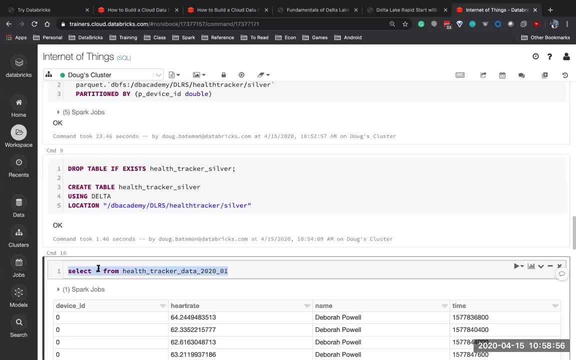 people are asking: is there, like people are asking: is there like intelligent dots to this notepad? does intelligent dots to this notepad, does intelligent dots to this notepad? does this work? for example, like toad does for this work, for example, like toad does for. 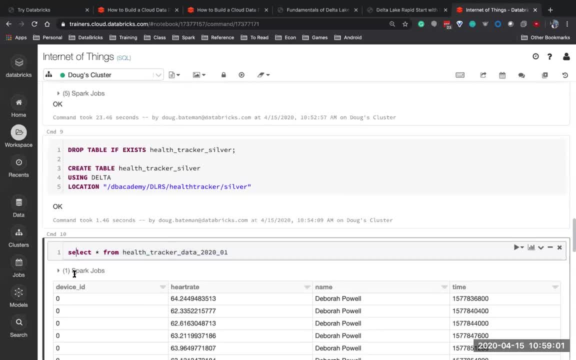 this work, for example, like toad does for Oracle, it doesn't have as many features Oracle. it doesn't have as many features Oracle, it doesn't have as many features as some of those other sequel work pads. as some of those other sequel work pads, as some of those other sequel work pads do, for example, I have to run all of a. do, for example, I have to run all of a do, for example, I have to run all of a cell or none of it. but the secret there- cell or none of it, but the secret there- cell or none of it, but the secret there- is that if I want to run part of a cell, 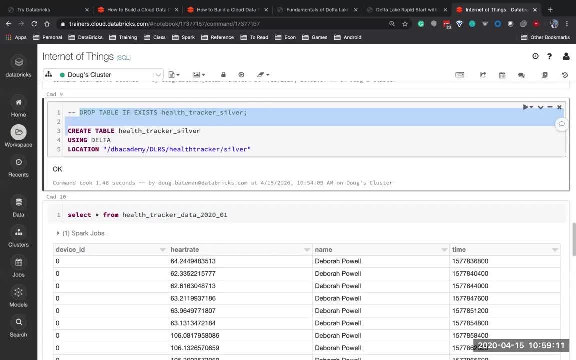 is that if I want to run part of a cell, is that if I want to run part of a cell, I comment out the part of the cell that I comment out the part of the cell that. I comment out the part of the cell that I don't want to run. and there's little. 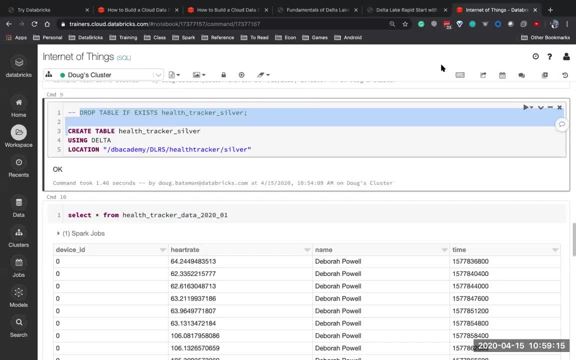 I don't want to run and there's little. I don't want to run and there's little shortcuts for that, like control slash and shortcuts for that, like control slash and shortcuts for that, like control slash. and if you want to see the keyboard, if you want to see the keyboard. 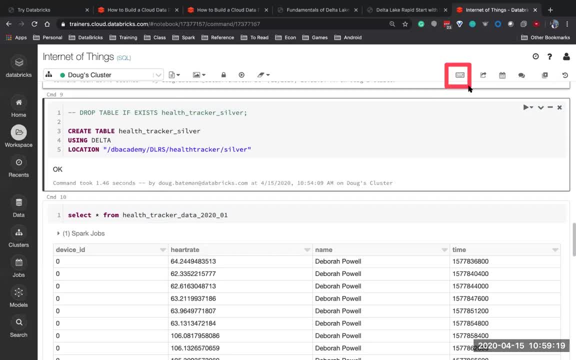 if you want to see the keyboard shortcuts, you would just click on this shortcuts. you would just click on this shortcuts. you would just click on this keyboard icon up here. and yeah so, Karam keyboard icon up here. and yeah so, Karam keyboard icon up here. and yeah so Karam is mentioning if I'm doing change data. 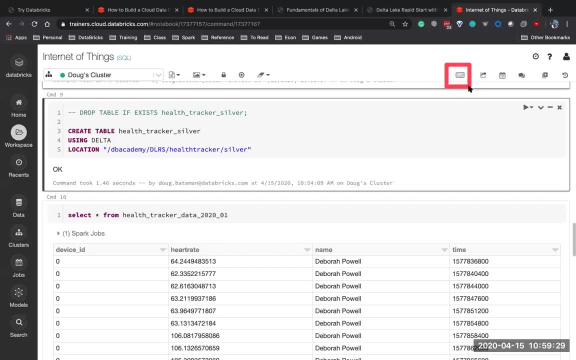 is mentioning if I'm doing change data is mentioning if I'm doing change data. capture Delta has a lot of benefits. capture Delta has a lot of benefits. capture Delta has a lot of benefits because I can look at what's changed, because I can look at what's changed. 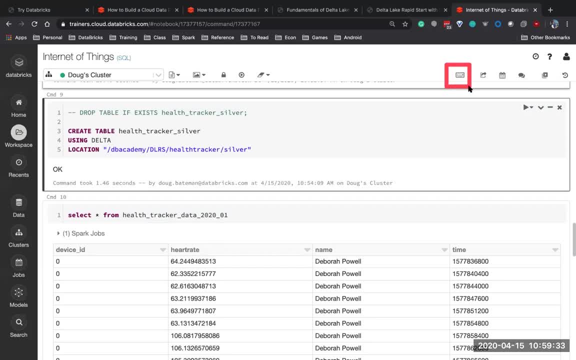 because I can look at what's changed between each version of the table. so between each version of the table, so between each version of the table. so there's actually a lot of ways to do. there's actually a lot of ways to do. there's actually a lot of ways to do that. somebody else asked: could I convert? 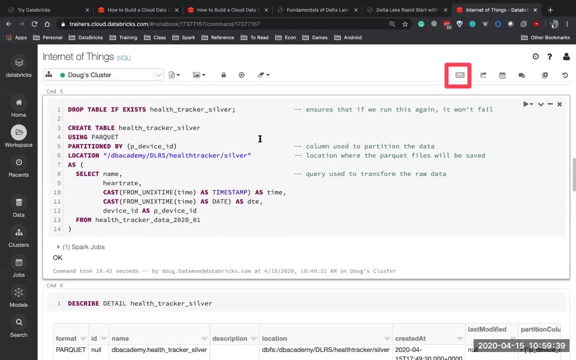 that. somebody else asked: could I convert that? somebody else asked: could I convert this directly to Delta and not go this directly to Delta and not go this directly to Delta and not go through the parquet step? absolutely through the parquet step, absolutely through the parquet step. absolutely let's do that. in fact, I'm gonna drop. 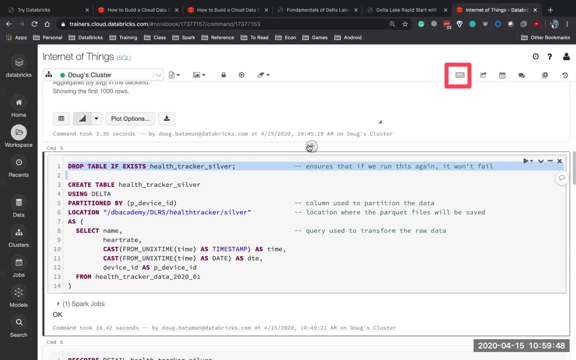 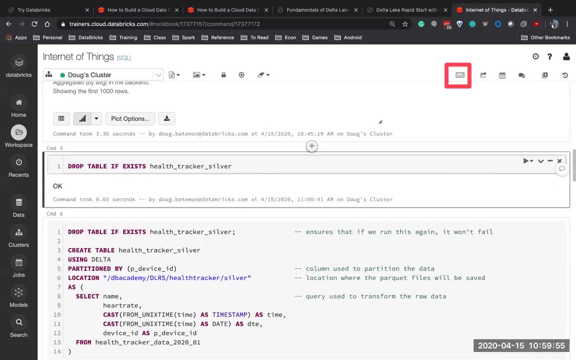 let's do that, in fact I'm gonna drop. let's do that, in fact I'm gonna drop the table. the table health tracker, silver, just to emphasize. i don't have to go through this parquet step, and i'm going to delete it on disk as well, just for demo purposes. 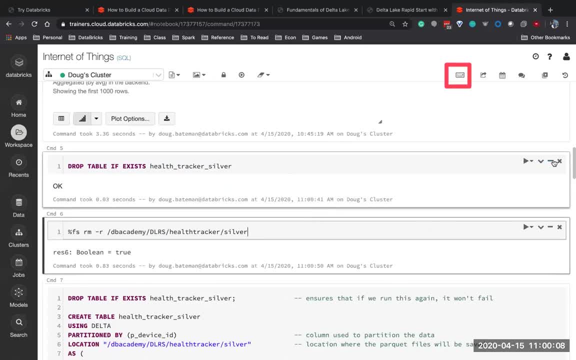 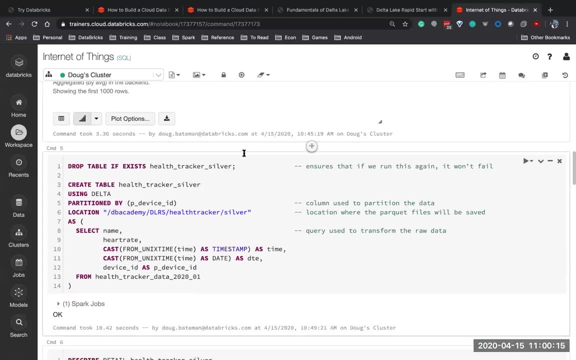 i'll delete the files on disk so that table doesn't exist. they said: do i have to go to parquet first to get to delta? and the answer is absolutely not. in fact, normally you wouldn't go through parquet. so instead of saying create table, silver using parquet, i could just say create table. 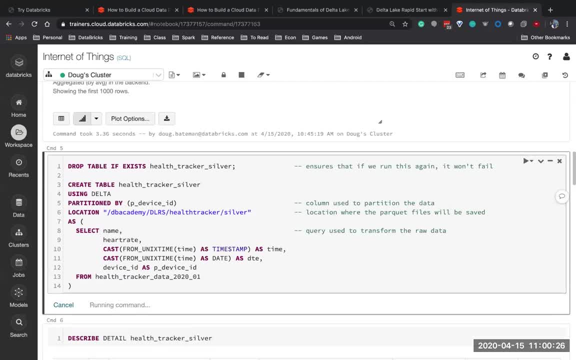 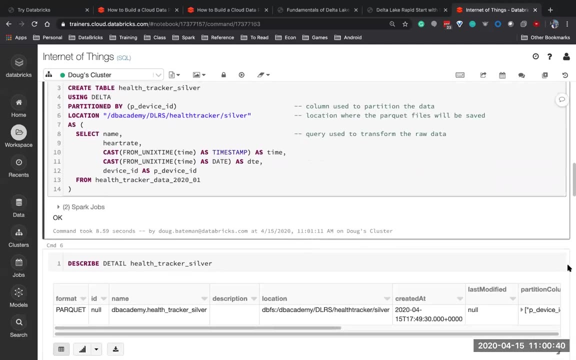 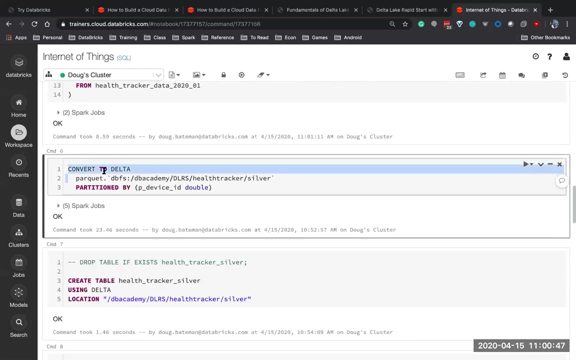 silver using delta and it's going to make this immediately be a delta table, and i'm not even going through parquet first. the only reason in this demo i made it parquet first is so that i could demo the command convert to delta. that's the only reason i had actually made it a parquet file first so i could. 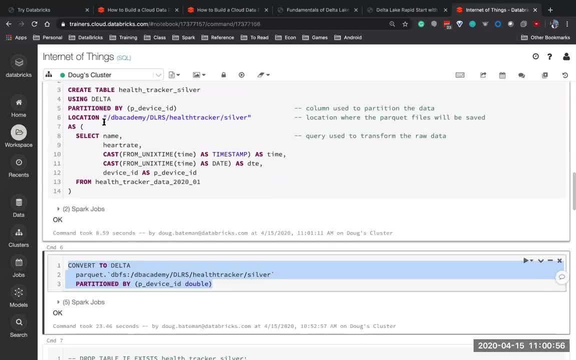 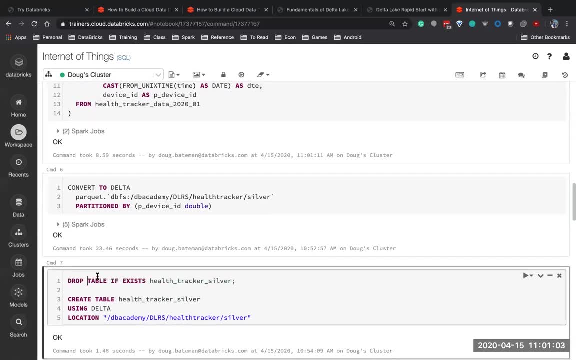 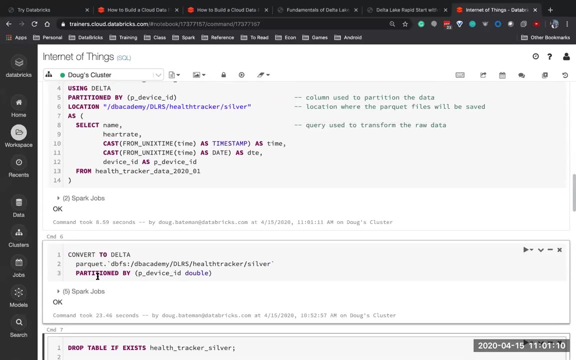 showcase this convert command. but you would probably go straight from json to delta, as i did here. all right, so at this point we have a delta table, whether we went through parquet first or not. um ravi asked what happens if the json doesn't have a standardized schema. some of them have more columns, some of them have other columns. 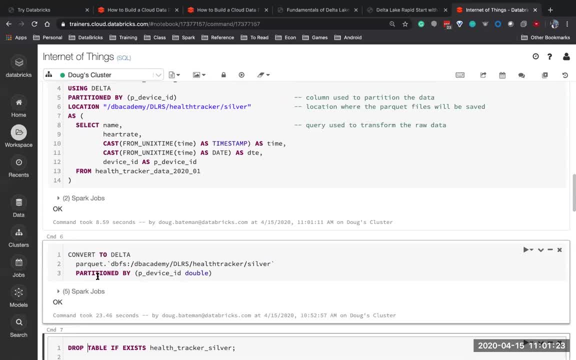 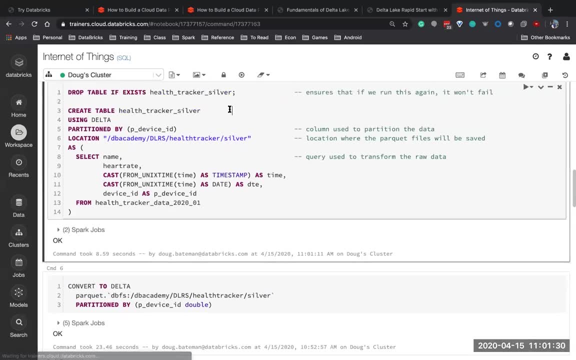 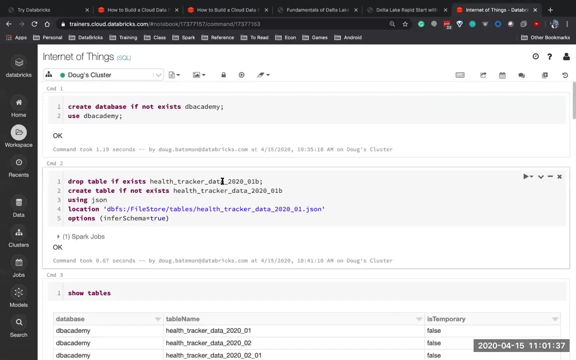 yes, you can still convert it to delta. it'll infer a unified schema. but, ravi, in a case like that, sometimes it helps to actually provide the schema in your create table statement. so one thing i did here is i did i told it to infer the schema in the json that we did up above. here we go. i told 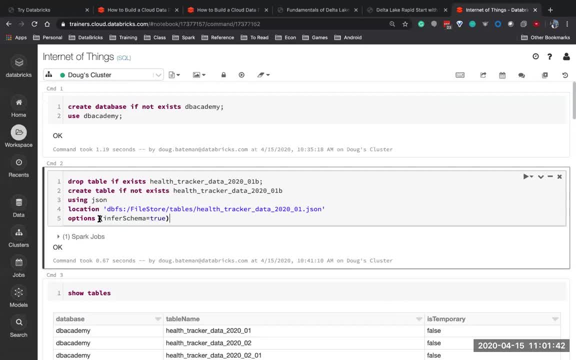 it infer schema. if you don't want to infer the schema, because maybe the schema is too erratic and changing, you could provide the schema manually instead of inferring it, and that would help you. with data- json data that's sparse, where the schema varies by row. you would manually provided the 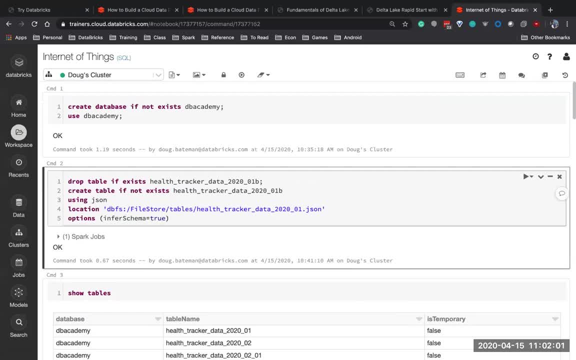 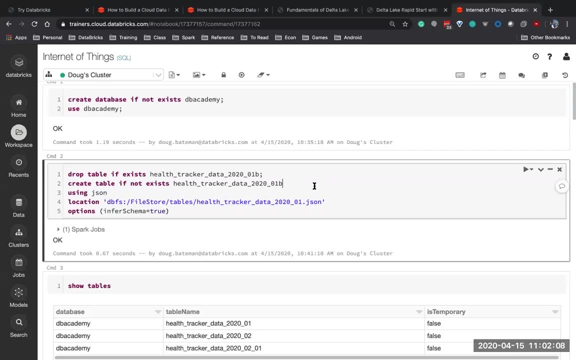 schema and that would address that concern and i'll leave that to you. to look at our etl course. we talk about how to provide the schema. if you go on to our databricks academy and look at etl part one and two, you'll see how to provide schemas manually. 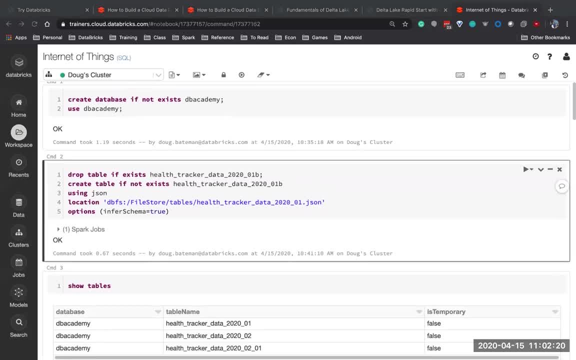 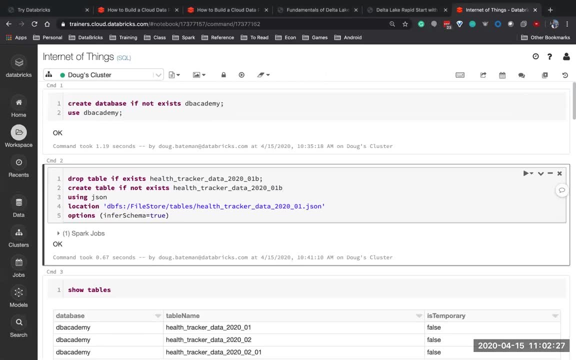 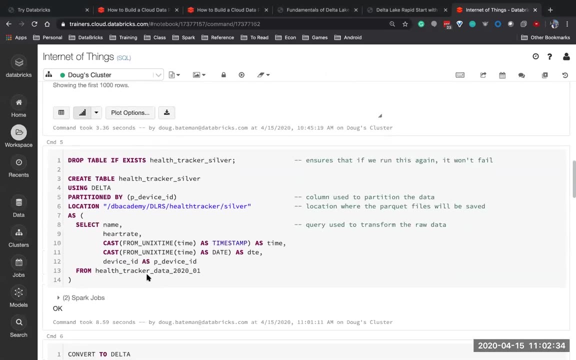 all right. uh, daryl, i'll get you to submit your question to the q a, since it's a little off topic here, as opposed to the direct chat. um, so rajesh asked: could we have created delta without even mounting the json file? yes, we could. so let's say i didn't even want to mount the json file. 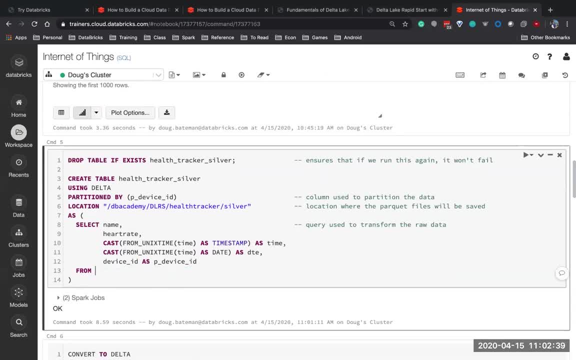 so let's say i don't even have a pointer to a json table. i could go json dot and give it the path to the health tracker data. so you know my json. i could give it a path that way to a json file and never even make a bronze table go straight to the silver table. you could definitely do that. there are. 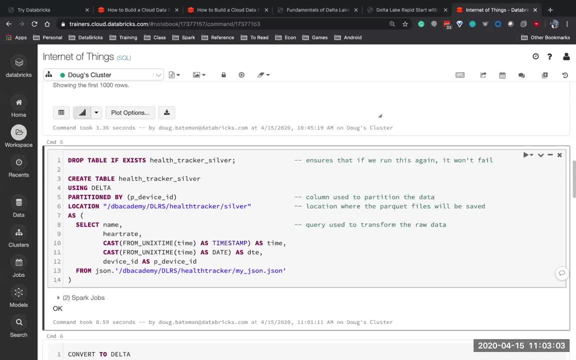 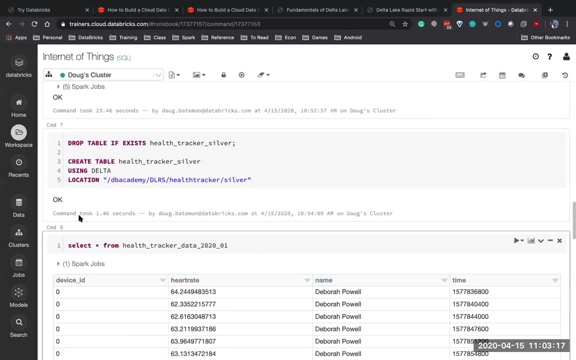 some benefits, though, to having the bronze data available under a table name, because then, if people need to get to the bronze data, they still can't. all right, so at this point, what we've just done is we've created a table for query purposes, and at this point it is a delta table, and I'm able to, in turn, query that table. 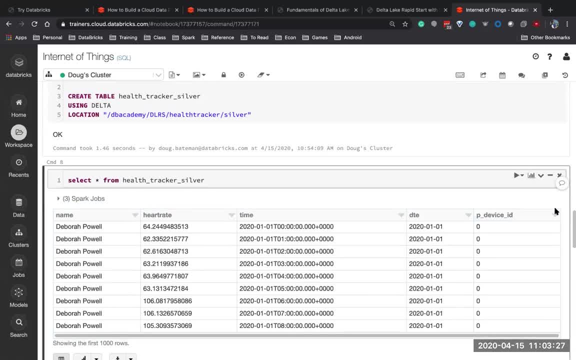 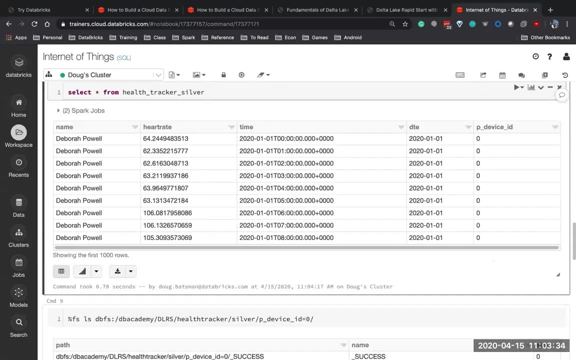 and one thing that you'll note is that it queries a lot faster than it used to query if it was a JSON file. So now notice I'm getting sub-second query times because delta and parquet are much faster than parsing JSON. Now, in the interest of time, I do want to keep moving forward because we 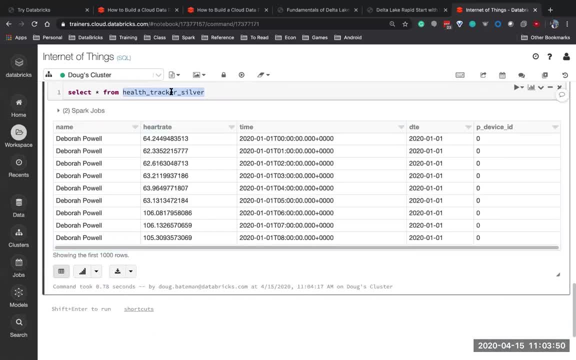 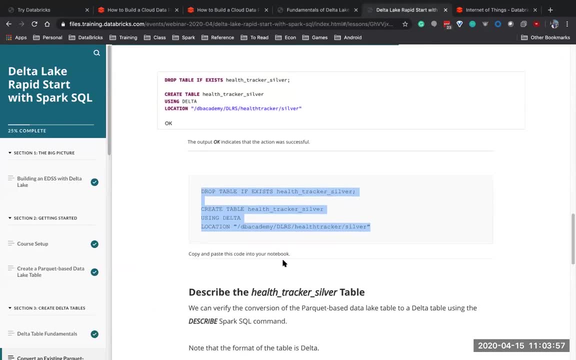 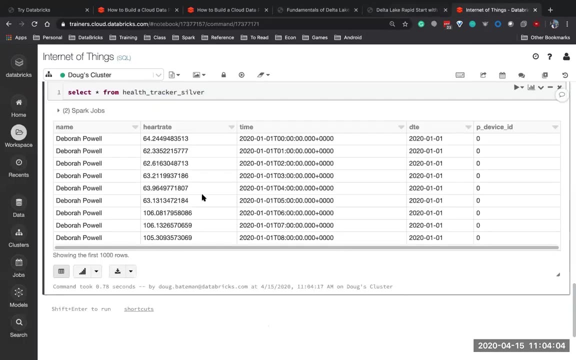 have a lot more work to do. Just because we've got a silver table doesn't mean we're done, So let's go ahead and continue on. First of all, let's use the describe command- Describe, detail or describe- extended on our silver, so that we can see that in fact it is a delta table. 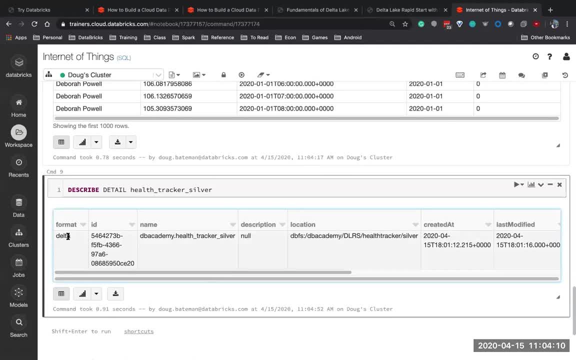 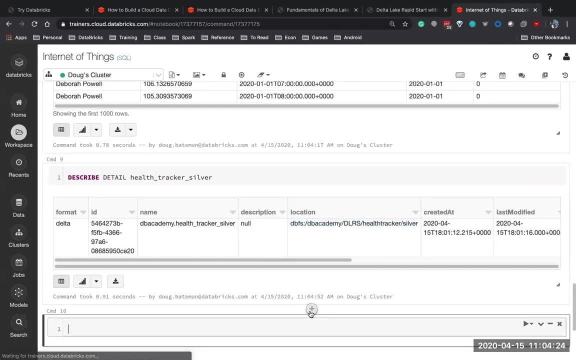 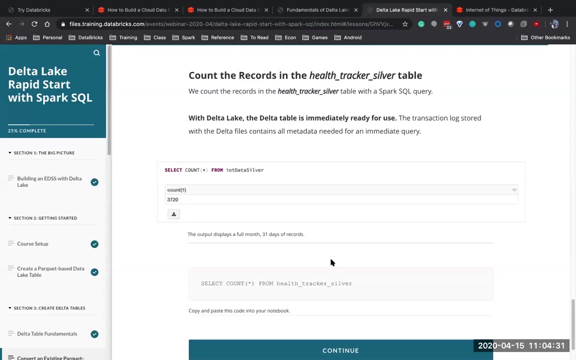 So describe, detail, Notice. this time it says the file format is delta, and again it tells me where it's located on disk. Now let's keep going. So let's do a more interesting query. I'm going to just steal it. It's not that much more. 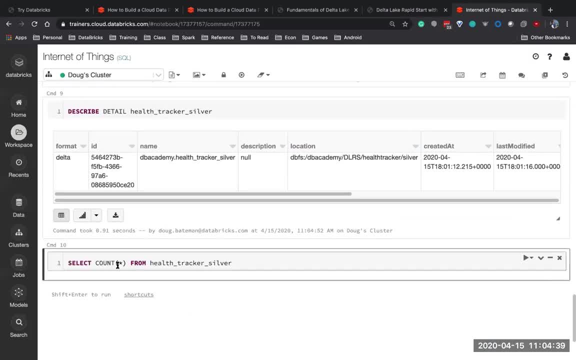 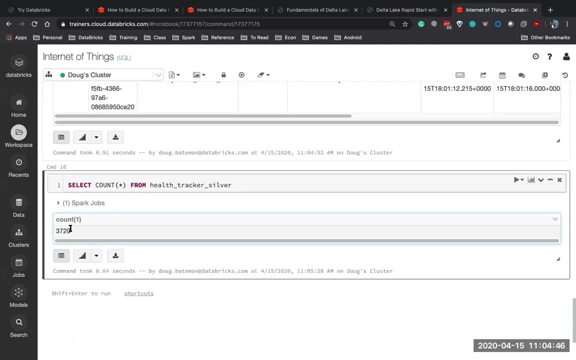 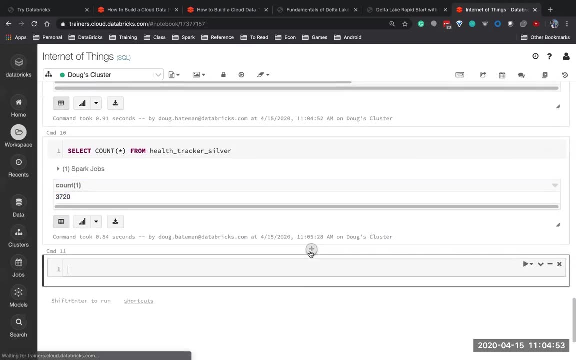 interesting. but instead of just describing it, let's do an aggregation: Count star From health tracker silver. Here we go: Count star from health tracker silver. Now somebody had asked: could I do this in Scala? I'm going to just showcase that. yes, if you wanted to use Python or 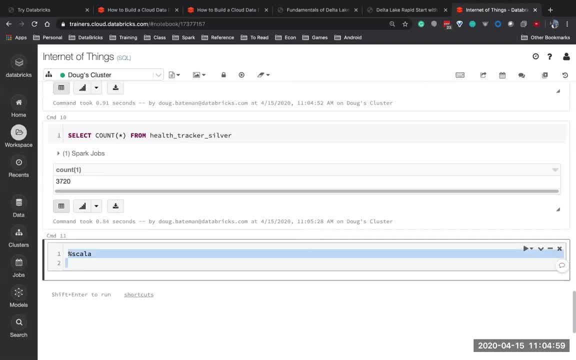 Scala. you could, I'll do Scala. I'm going to run Scala code. Notice, the default language for this notebook is SQL. So if I want to run Scala code, I have to say it's Scala. but then I could go sparkreadtable. 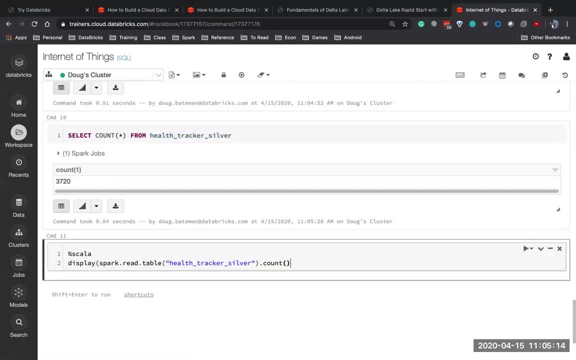 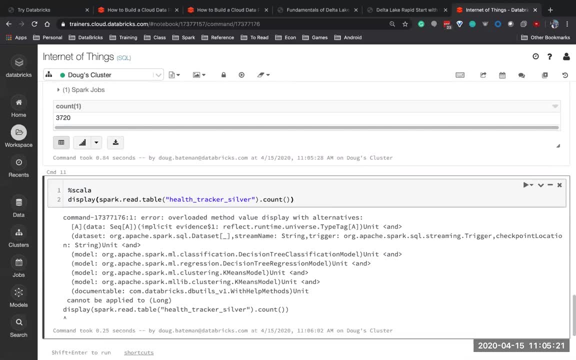 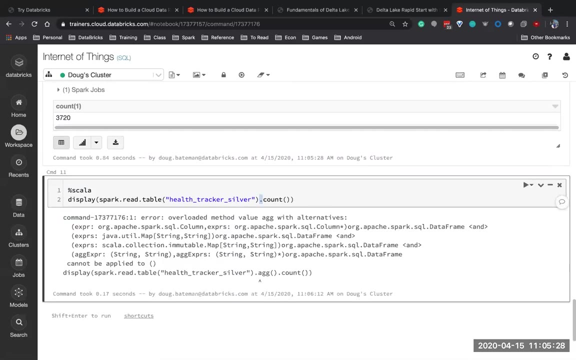 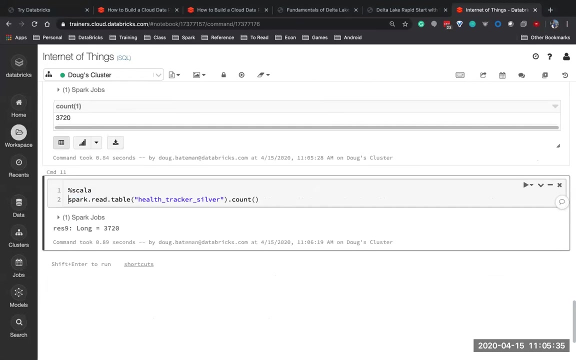 Health tracker, silver dot count, and I could display that And I could write the exact same code in Scala. And why is he complaining? Oh Well, count in this case is coming back as a single row. So we'll do this And I get my count back. 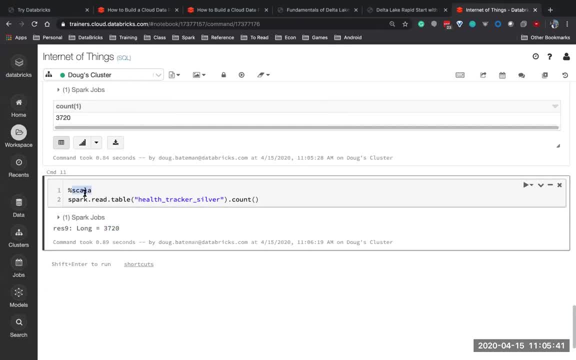 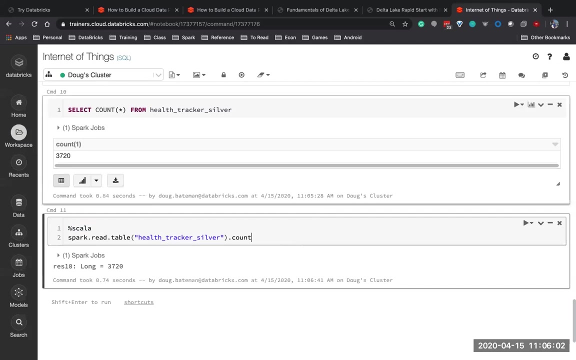 Three thousand seven hundred and twenty. I could do this in Python. In this case, the Python would look exactly like the Scala. There it is in Python. If it was Scala technically, I don't need these parentheses. There you go, So just showcasing that, yes, I could mix in Scala if I wanted to. We're going to stick with SQL for the bulk of this particular one. 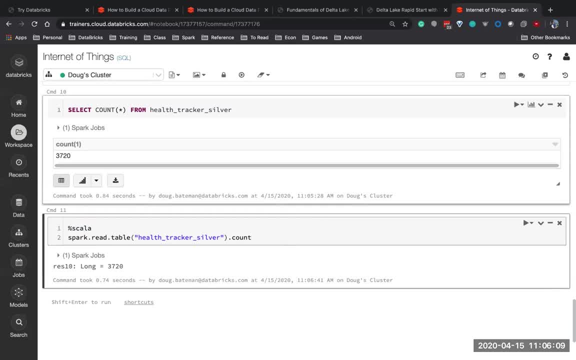 But if you want to learn how to do this stuff using Python and Scala, I really do recommend you go to Databricksacademycom and get the ETL course series. ETL is part one, two and three and they use Python and Scala to do this type of work and you get to choose your programming language. 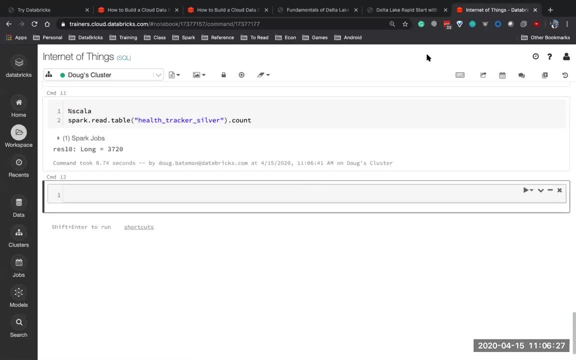 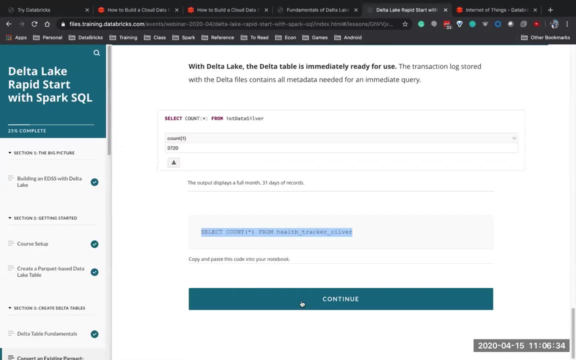 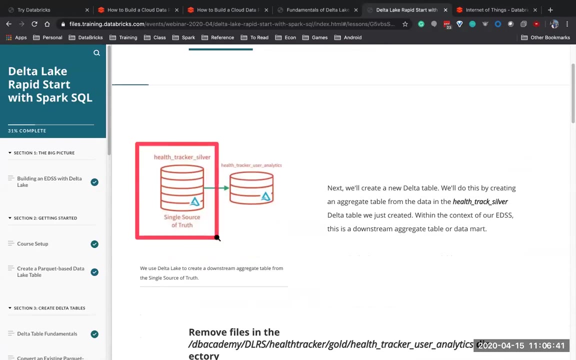 For this series. we're going to focus on SQL for today. We'll have a little bit of Python, tomorrow on session three and quite a bit in session four. All right, let's continue on now. So at this point we have loaded our silver table, which serves as that single source of truth. 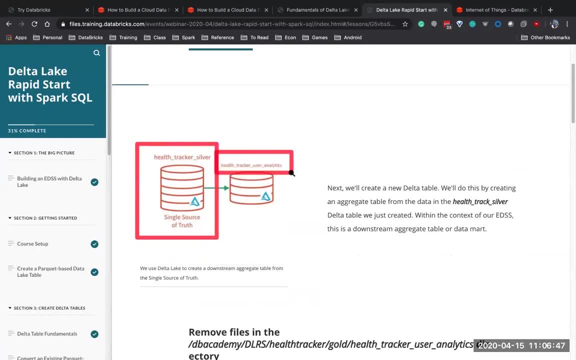 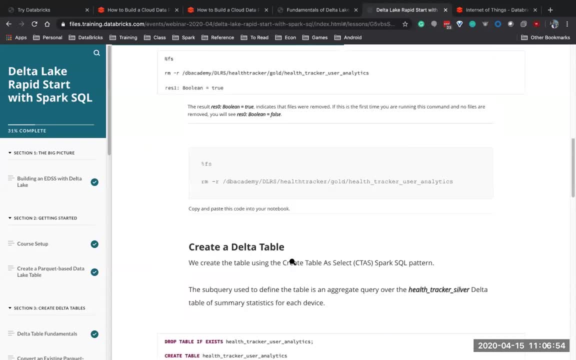 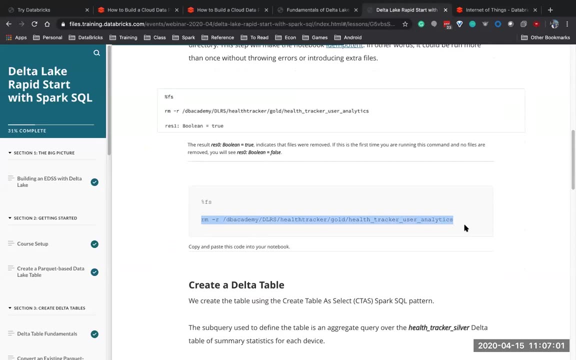 And now we want to try to create an analytics table that does some degree of aggregations. So let's go in here and create a delta table Now. if you're running the course yourself, you'll notice that they recommend you delete old files if they exist on disk. 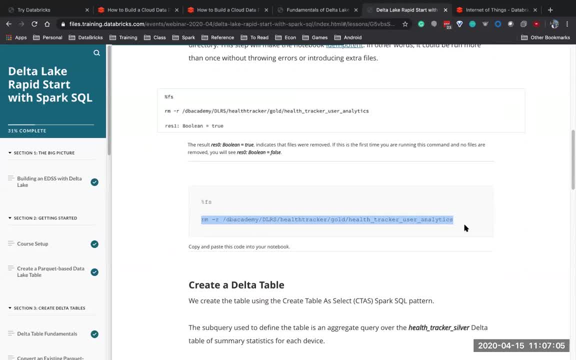 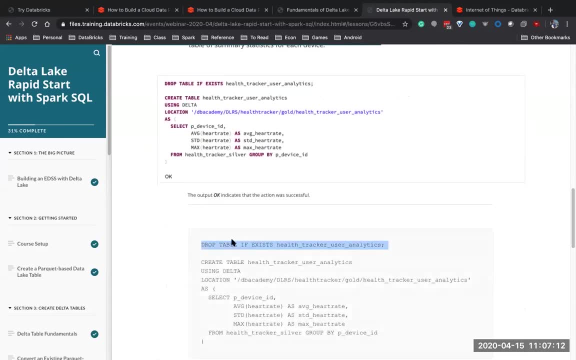 This is just to ensure that if you run the notebook twice, there's not old files laying around. I don't have that problem because I don't have old files laying around, so I'm going to go straight to this command here, where we're going to create a table that does aggregations. 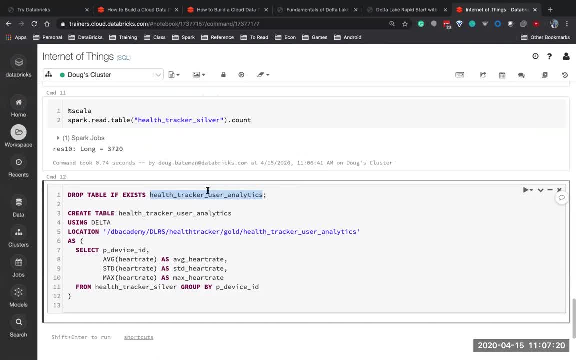 So this is my gold table. it's the Data Mart table, So I'll drop it if it already exists. in this case, it does not exist and I'll create the table using delta. I can tell it where I want to put the table. on DBFS. 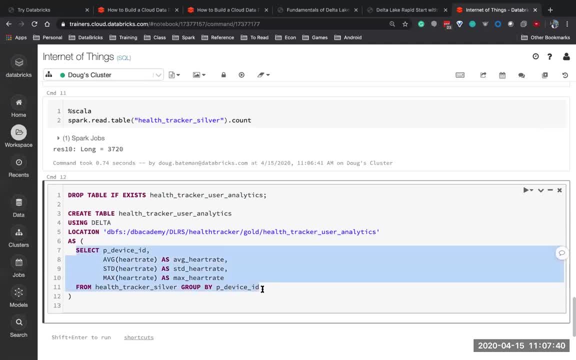 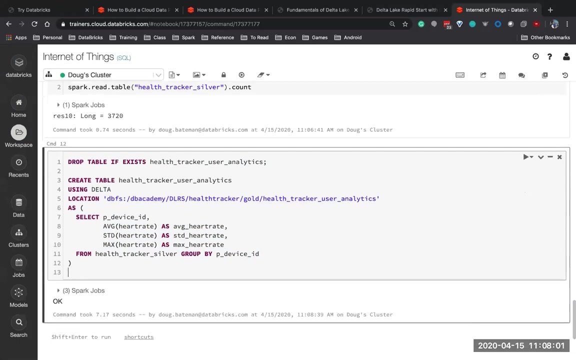 and then I give it the query to use to make that table. so in this case I'm going to get the average, the standard deviation and the max of my heart rate and I'm going to group by device ID. so I'm making this gold table and let's take a look at it. 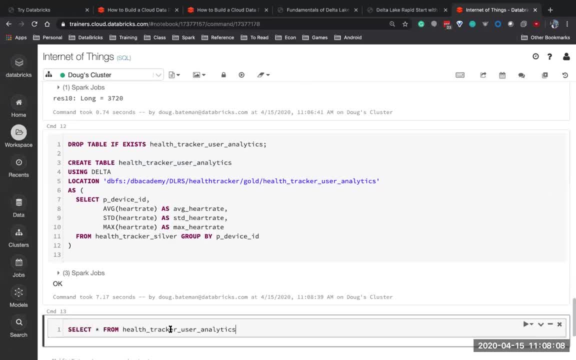 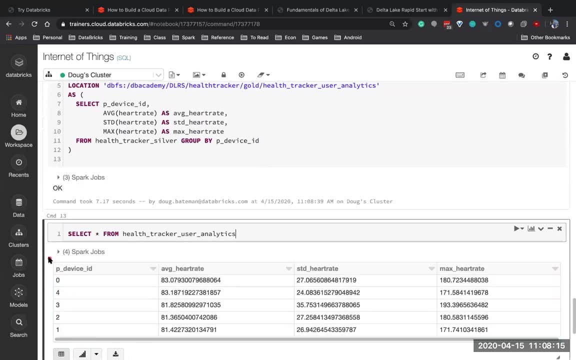 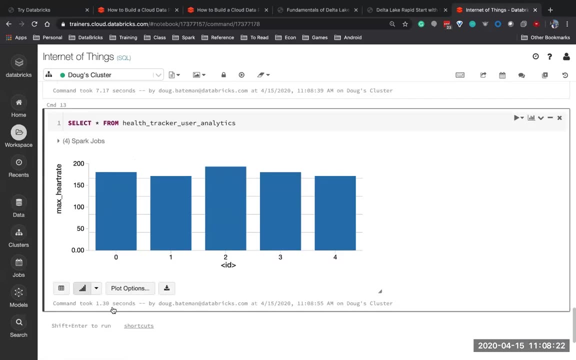 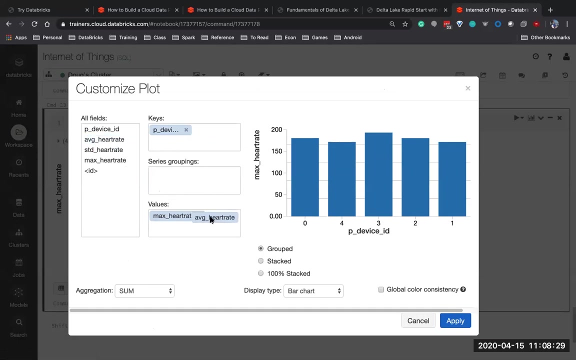 select star from health tracker user analytics. and there it is and notice that of course the device IDs didn't come out sorted in any particular way. so when I go and make a bar chart for this, let's see here, if I make a bar chart I want to use device ID and I want to look at max. 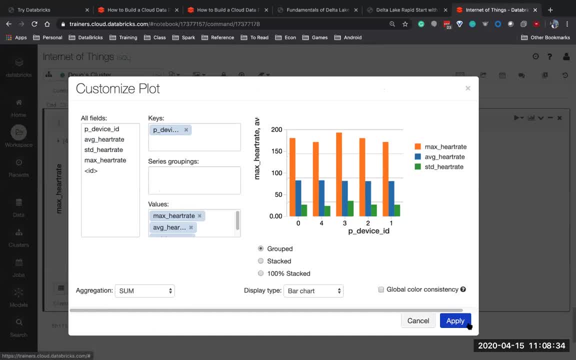 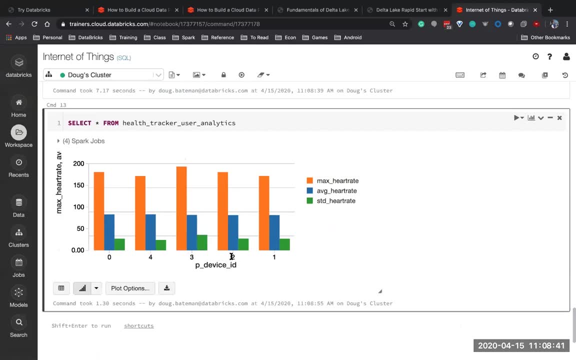 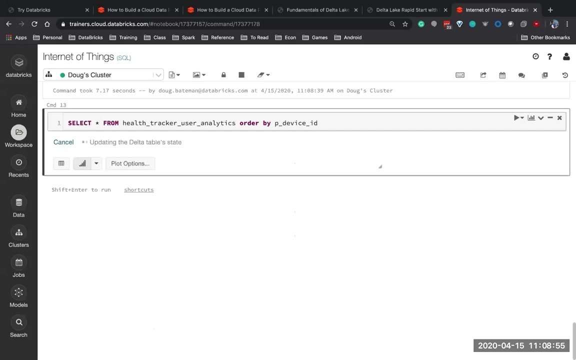 heart rate, average heart rate and standard deviation here and I click apply, girl notice that these keys came out in a weird order: zero, four, three, two, one. I don't like that, so I could come in here and go order by P device ID and sort as part of my query, and now they come out ordered. 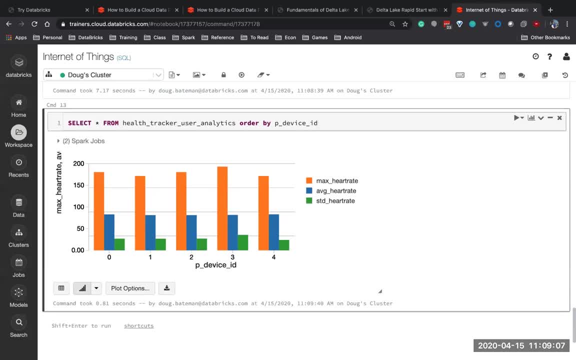 very good, cool, and this is my gold table that my end users might want to hit as part of their exploring the data. so first I read in those bronze JSON files, I then did clean up, I fixed the schema and I brought in the data, and that's my silver. 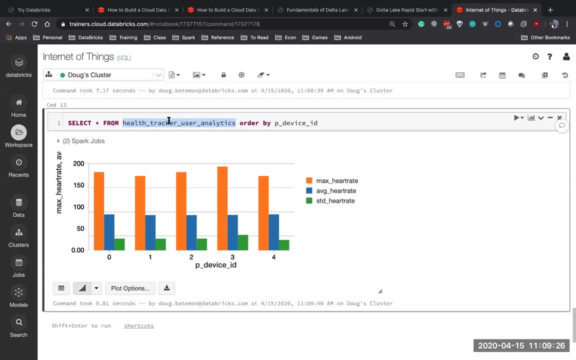 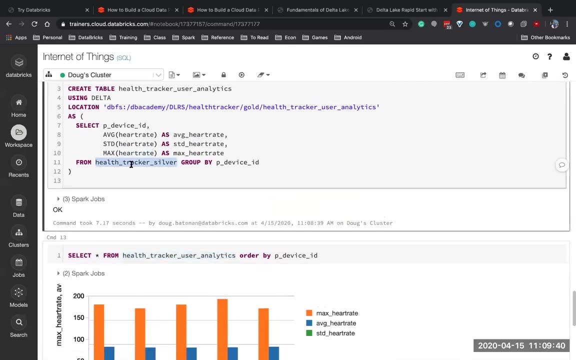 table. although we still have some cleanup to do, we're gonna be doing that soon enough. and then I was able to build my gold layer, which is these reports and roll-up analytics. and somebody asked: why is the gold table table not created directly from the silver? and it is. take a look. I made the 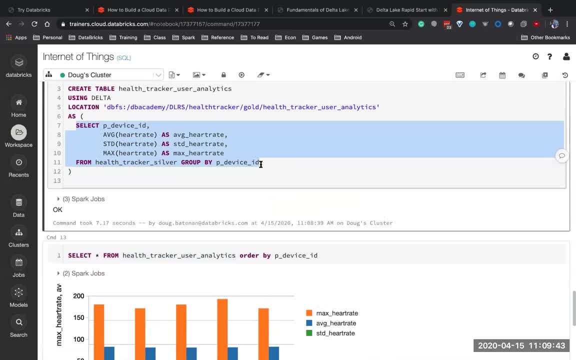 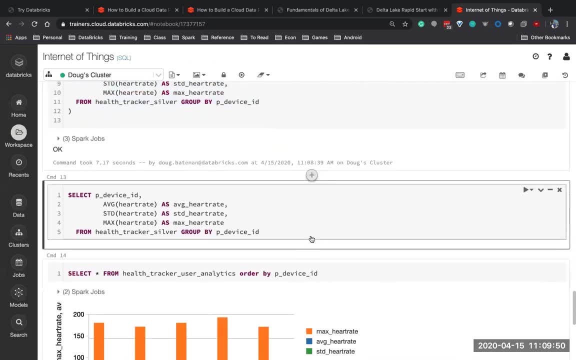 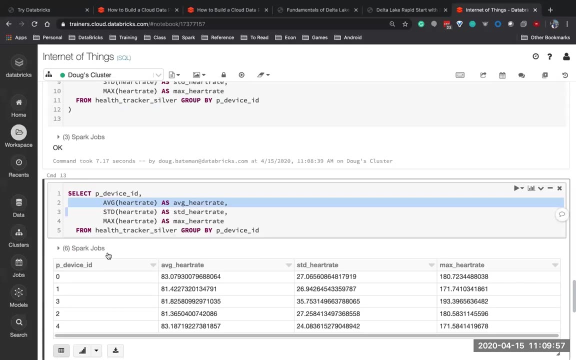 gold by running a query off the silver table. now, if I wanted, I could actually run. that is just a sequel query and not write it out as a table. but that means that every time I run this query I've got to do that computation over again, which, for really big data, could take. 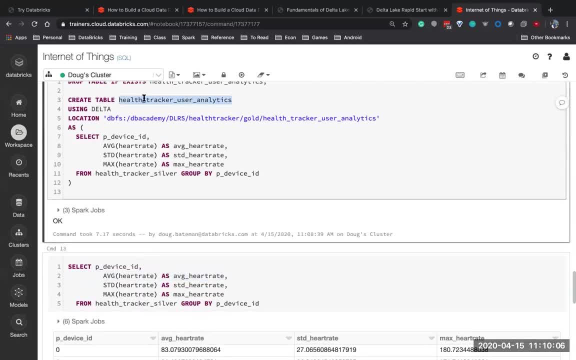 hours, so that means that can be a lot of work, so part of the goal of this is to So by saving the results off as another table, I'm now able to hit that table and view pre-computed information for my exploratory data analytics. 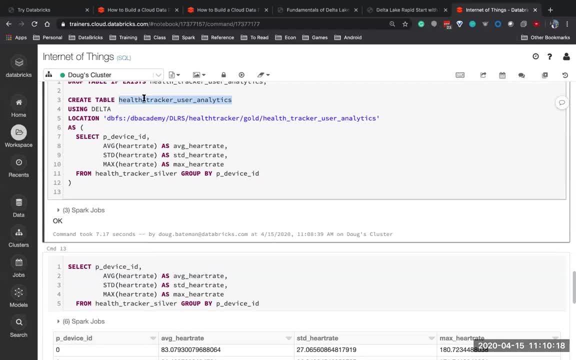 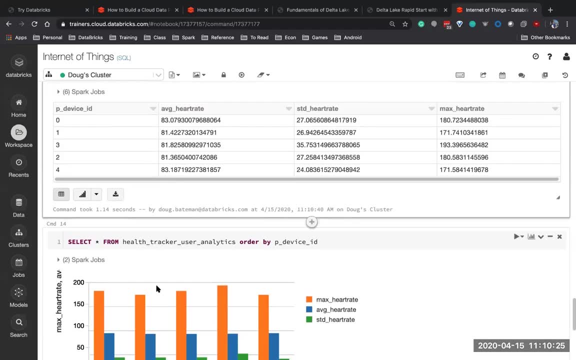 So the benefit of writing a gold table is speed. It takes a little while to write out the results. but now let's say that gold table had millions of records in it. I could query the gold table directly and not have to recompute all those aggregations every time. 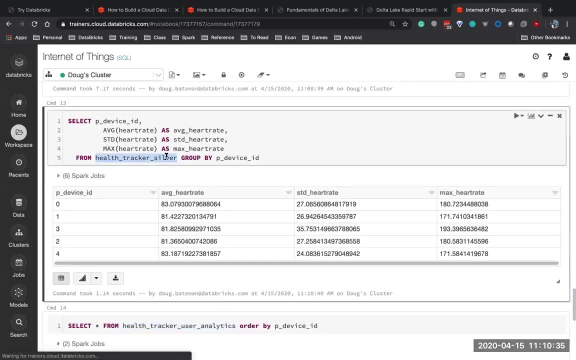 So, yes, they could query the silver table directly, but at that point they've got to run those analytics over and over again. So if these are analytics that they're reporting on frequently- for example, if I'm building a star schema and I'm creating a cube, a data cube- for a star schema- I likely will want to write that out as a table so that people can query it much more quickly than they could query by recomputing the aggregations on the raw data. 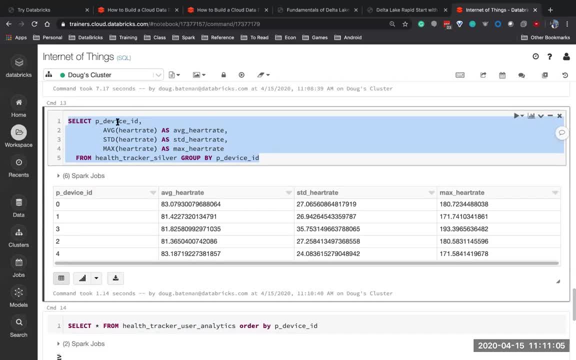 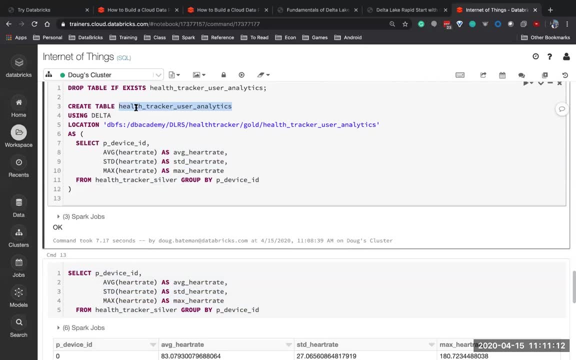 But you have a choice. It depends on your use case as to whether or not you want to query the silver table directly or you want to write that out to a gold table so people can look at the roll-ups more quickly, based on pre-computed aggregations. 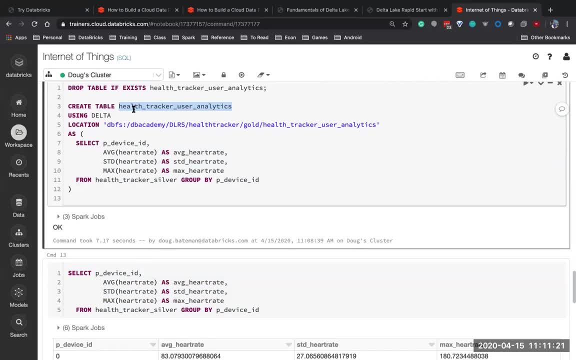 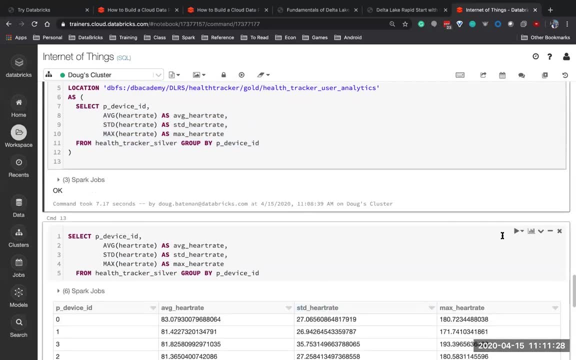 And that's a choice that depends on your use case as to whether you need this gold table layer, But the more data you have, the more benefit you get from having some pre-computed gold data. All right, let's continue on here. 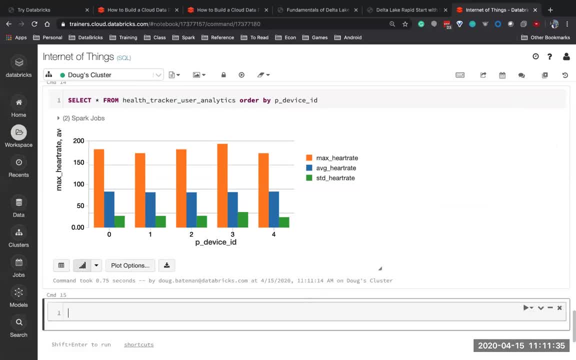 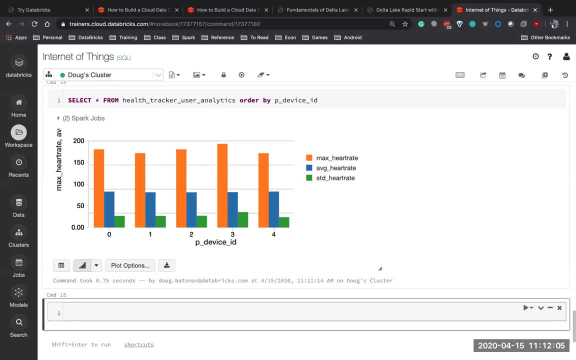 You can also use ETL tools integrated with Databricks, And then, if you're in Azure, there's something called the Azure Data Factory that you can also use. But notebooks are a really nice interactive way. You can also use Airflow. 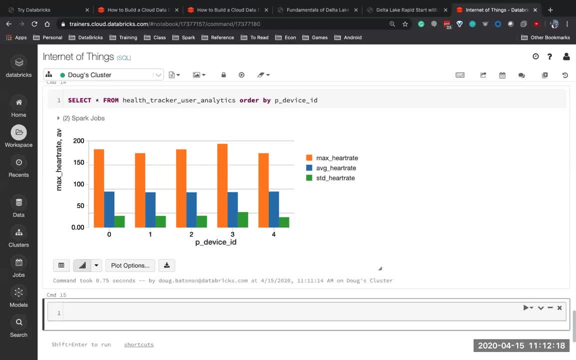 That's right. Somebody just mentioned you could use Apache Airflow to kick off those ETL jobs. But what we like to do a lot of the time is to describe the ETL in a notebook and then have Airflow. call the notebook Or Azure Data Factory. 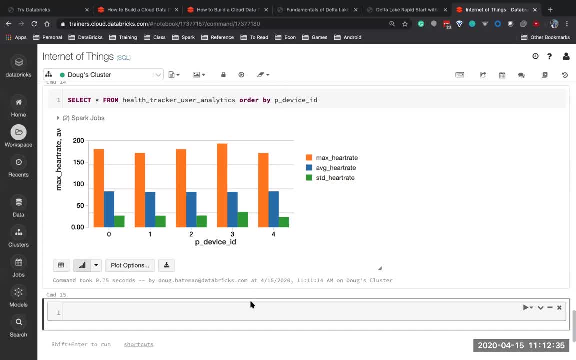 Or Azure Data Factory call the notebook. Or if you have a file like a library you want to use, you could upload the library to the cluster and then have the notebook call that library. So there's lots of options that come with that. 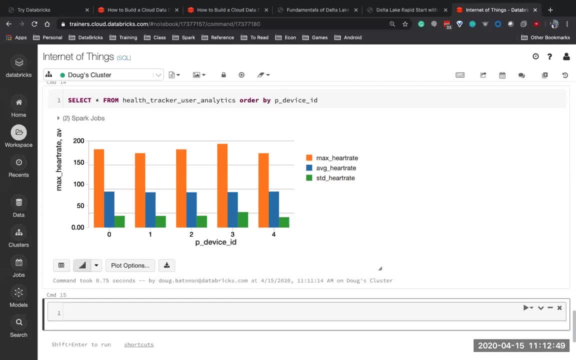 And Saeed, I see earlier you would ask: can you define a schema for JSON? Yes, you can. I'll let you look at that ETL course for examples of defining schema for JSON. Or, if we have time, I will try to pull up an example where I defined a schema for a JSON. 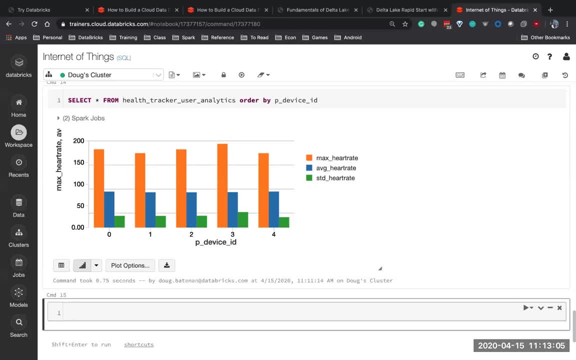 I'll let you look at the JSON file at the end of the course. Let's see here. I'm just going to skim down to some of the newer questions. Somebody asked: could we use this with structured streaming? Absolutely, All of the things that we're doing can be used with structured streaming, and that will be something we showcase in Seminar 3.. 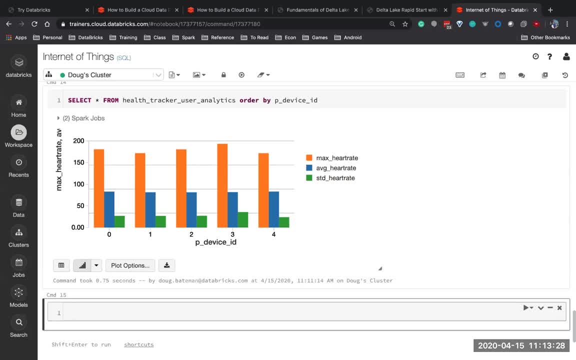 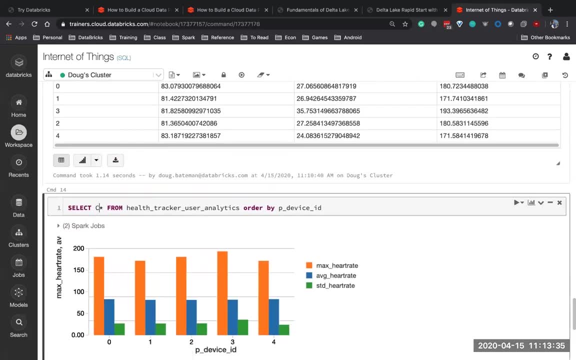 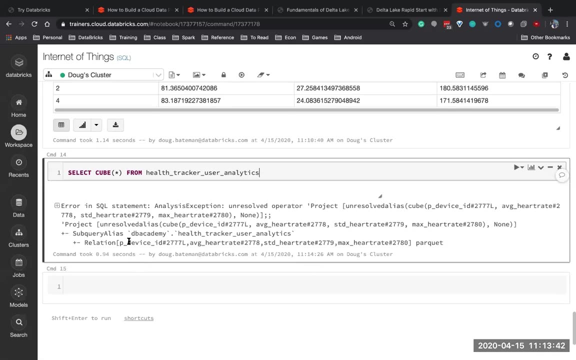 And then Nimesh mentioned: could we create a multidimensional cube on top of a data lake? Absolutely So. there is in fact a cube function that I could run. I may have to look up the syntax for cube because I'm not using it right. 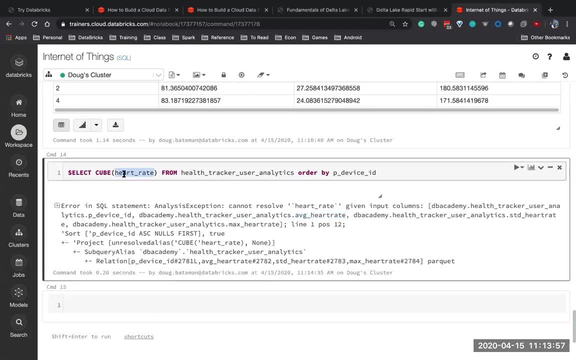 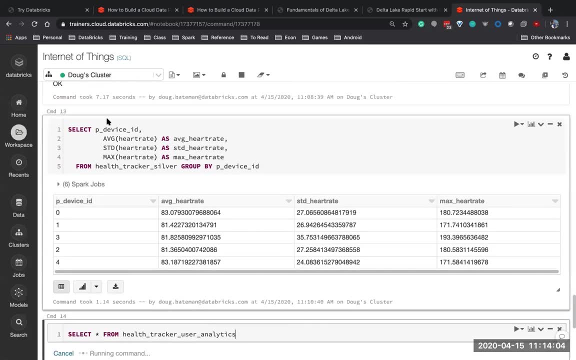 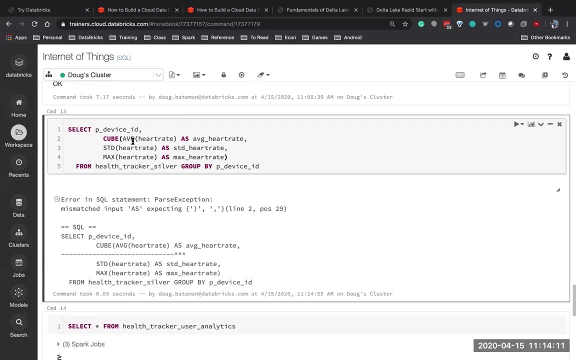 It is average heart rate. Oh, I know why That was my gold table. Go back to my silver table. I could, for example, do a cube, And I just have to remember the syntax for doing a cube, so I may be in trouble here. 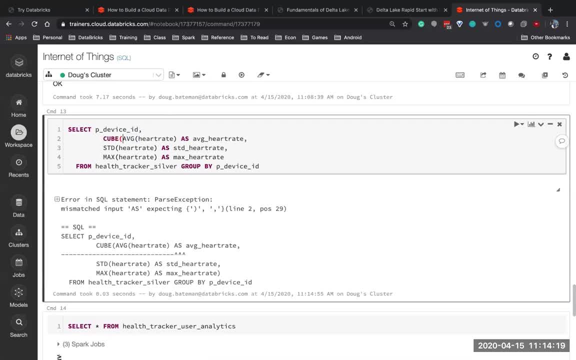 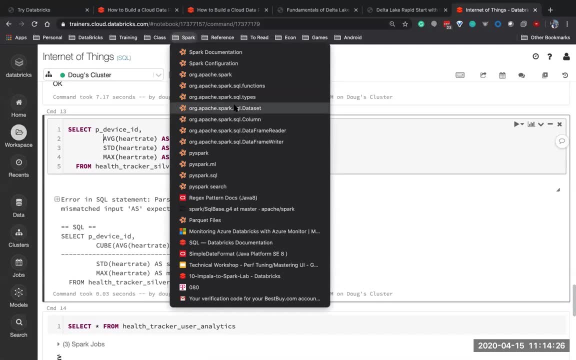 I don't remember the syntax off the top of my head but I can use cube functions inside of my SQL to roll up a cube And if you really want to know what functions there are, I have a bookmark to it. If we go and look at the functions that are out there, there is a cube function. 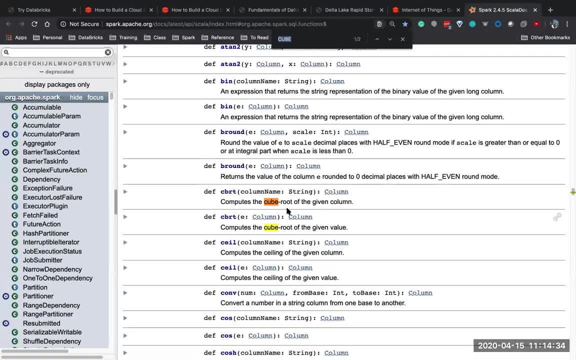 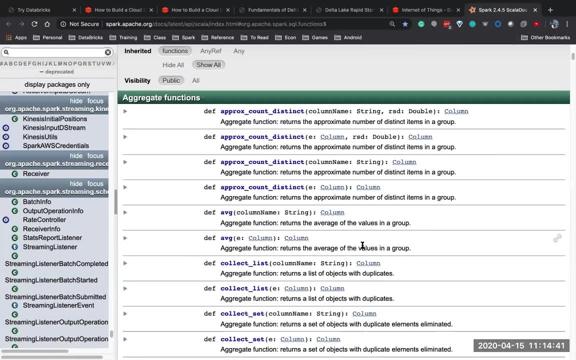 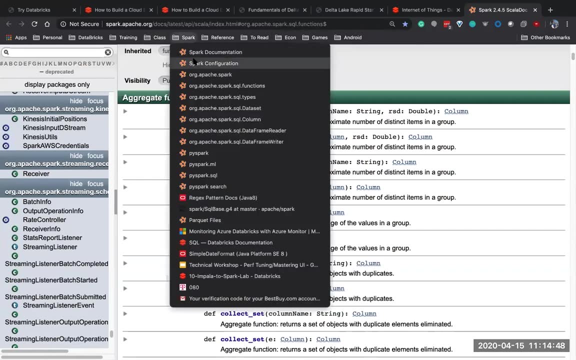 And it's a function for building cubes and rollups. Oh, it's called, let's see rollup. Why is it not showing up? Oh, I'm looking in the wrong place. That's why it's on the data frame itself. 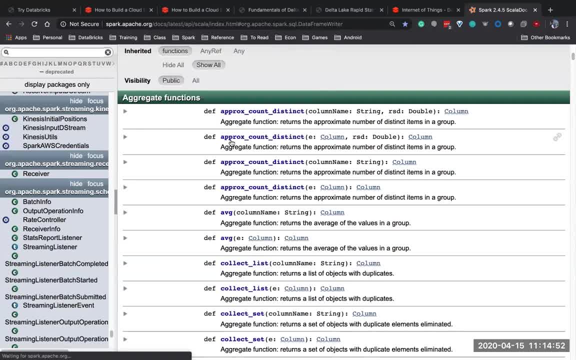 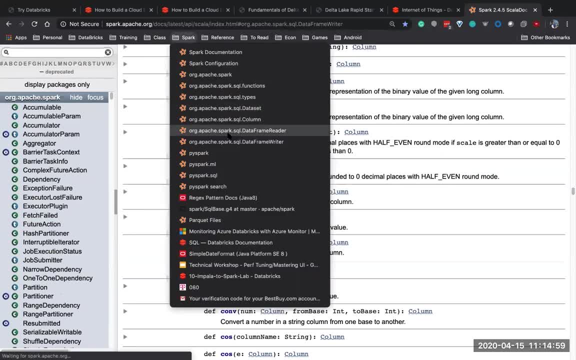 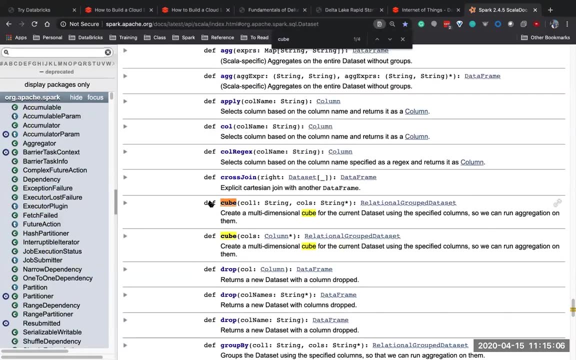 So we have to go to the data frame API and we look at cube Shoot. This is what I get for answering questions live. But let's see here Spark data set, cube- There it is. There are functions that we can use and you could do it in SQL as well. 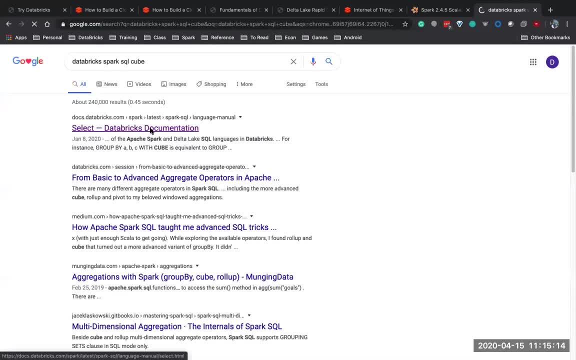 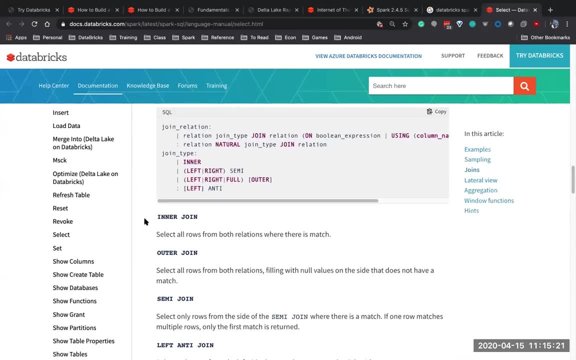 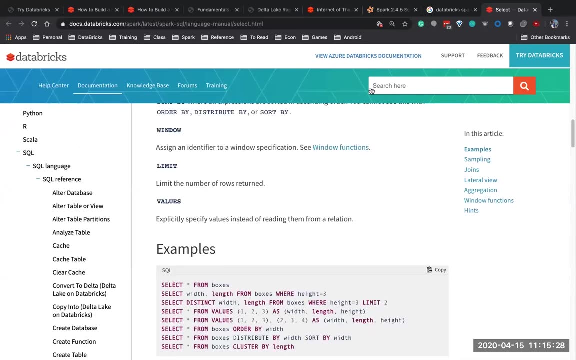 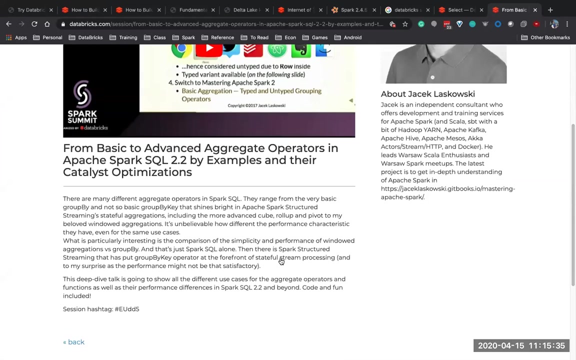 Databricks, Spark, SQL, cube, And in here let's see if we can find where cube is mentioned. Hmm, I will have to look and answer that offline Where we find the cube Cube operators inside of Spark. I believe we have an online presentation in fact. 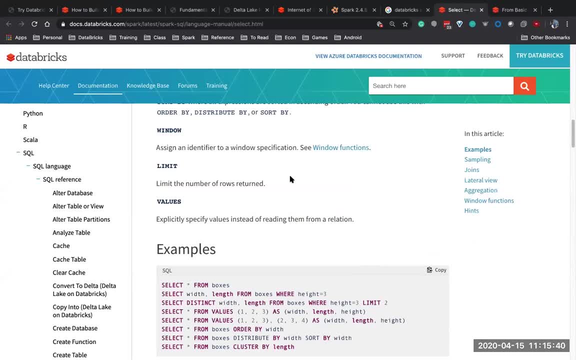 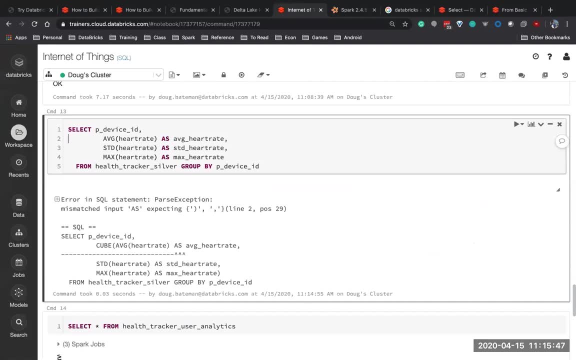 where people are using the cube operations inside of aggregate in Spark. Let's go ahead and not get sidetracked by using cube for right now, because we do have a lot to cover today. But the answer to your question is yes, I could do cubes in my rollups. 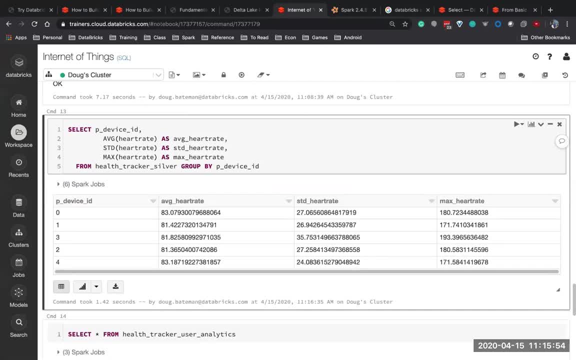 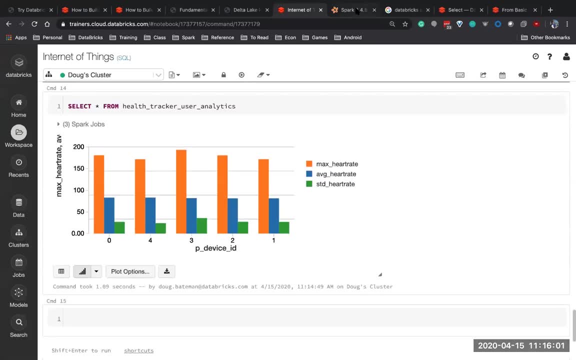 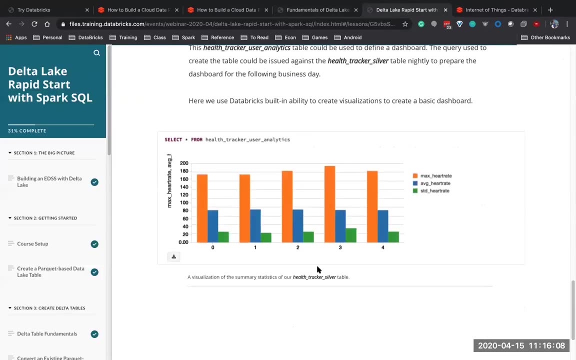 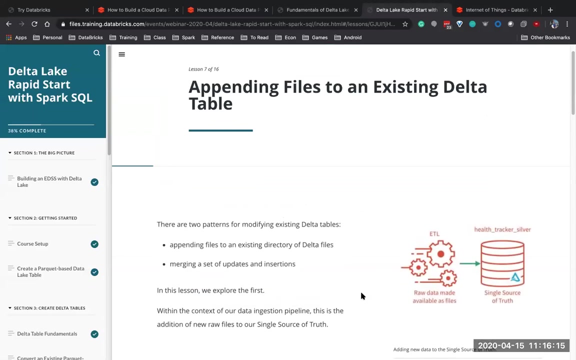 All right, Let's continue on. Okay, And we've created our dashboard. I already showed you the dashboard where we got to look at our various user analytics, So let's continue on now and start dealing with newly arrived data. So I've already got my bronze JSON file, my silver query table and my gold aggregation. 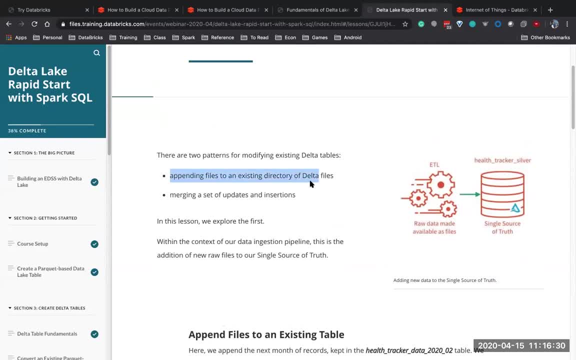 And now I want to deal with appending new data to an existing and I want to deal with my silver and gold tables. So I need to be able to insert new data into this, Because it's rare that you would just be done once you've built your silver and gold tables. 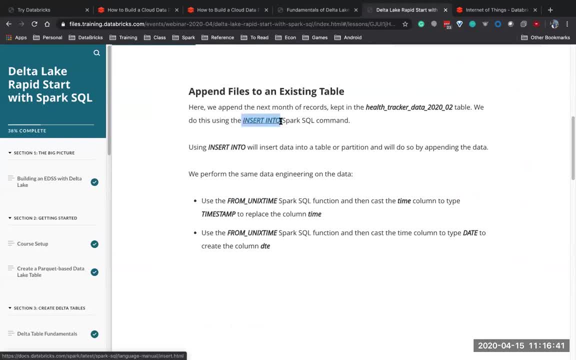 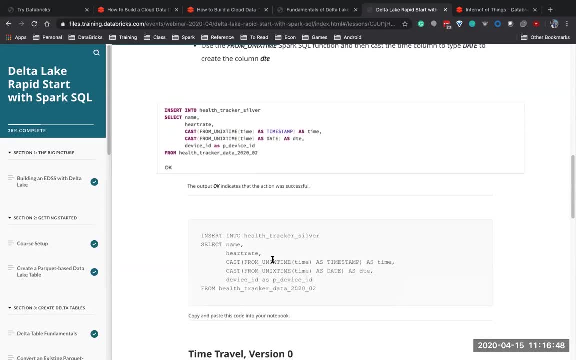 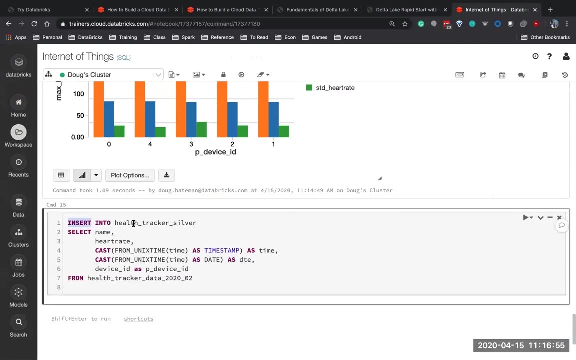 So I need to be able to insert new data into this. In this case I want to insert data for February. So I'm going to need to say: insert into my silver table. So let's come down here and actually do that. I'm going to insert into health tracker silver. 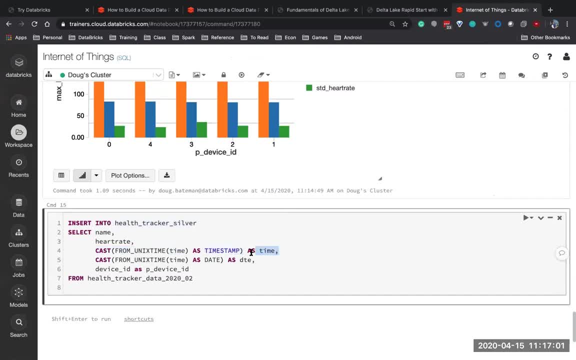 I'm going to need to again take that bronze data that we had before, make sure that I'm making it match the schema and doing the cleanup. So I'm going to grab the bronze data for February and insert it into my silver table. 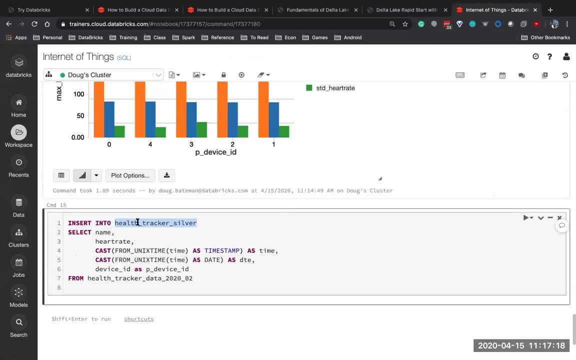 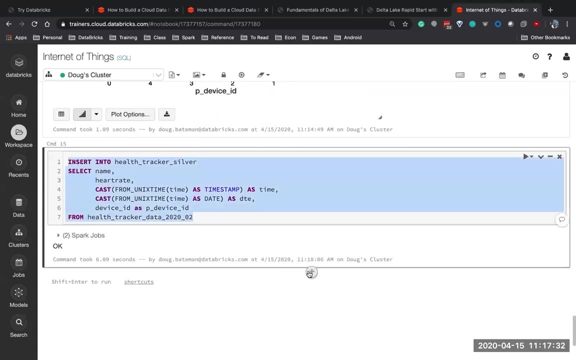 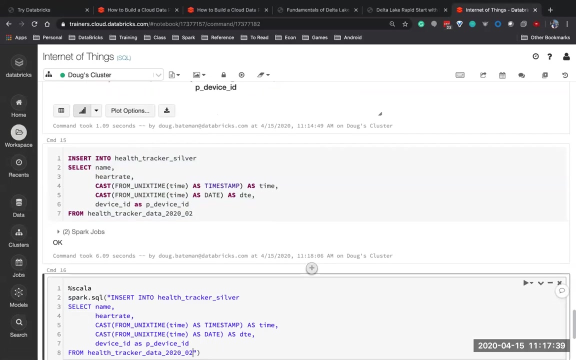 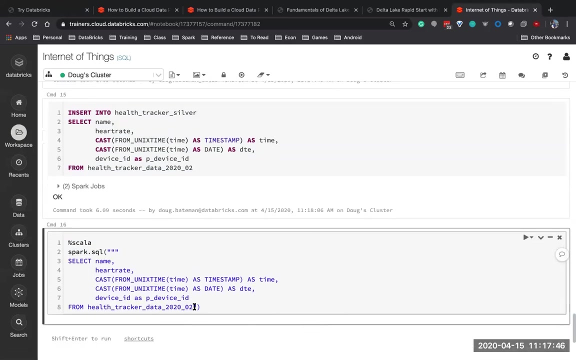 by using the insert into delta command. Okay, Okay, Okay. Now, if I was doing this as Scala, for example, Do this, I'll write my query. Then what I could do is go writemode, append and tell it that I want to write to my 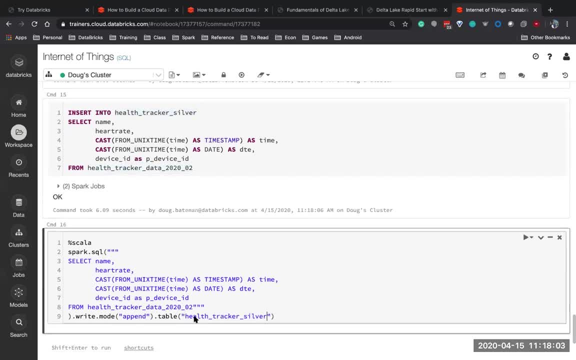 my silver table So. but if I'm using SQL, I just get to use the insert into command to be adding data to my file, which is really really nice. So I've added it in here. I now have more data in this file. 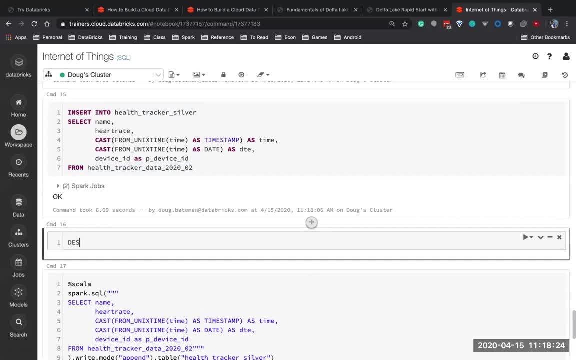 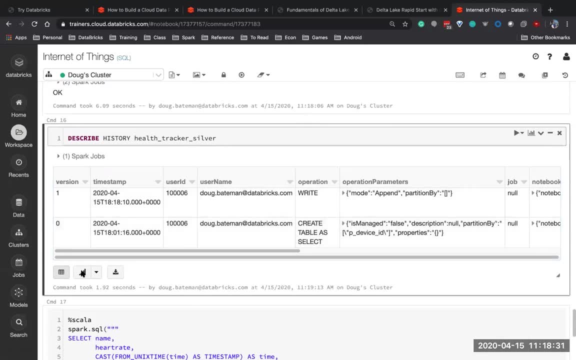 Let's take a quick look at my thing here. So let's go describe history, health tracker silver, And you could see that I have a new version of the table That's been written out as a result of a write operation And it's written out new files to disk. 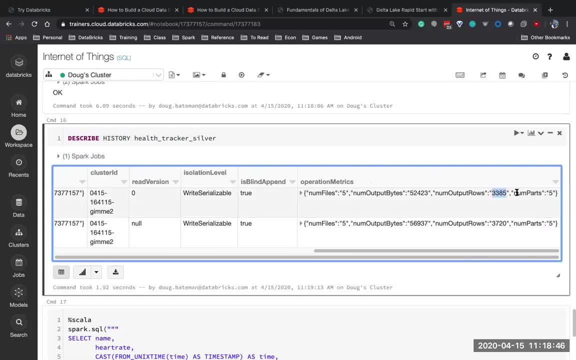 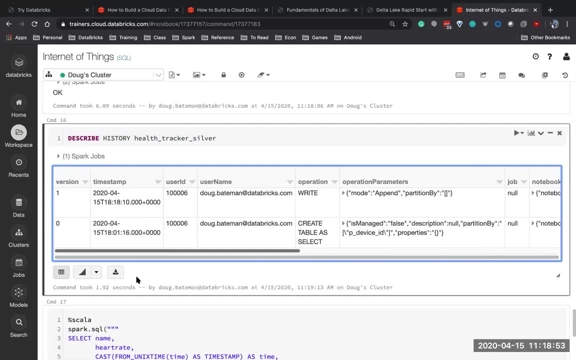 So, um, and let's see here the total number of rows, Let's see which one was version zero, Which one is version one, version one: Okay, That's the newer data, And I could see, for example, how many files were added, how many bytes are there, and so forth. 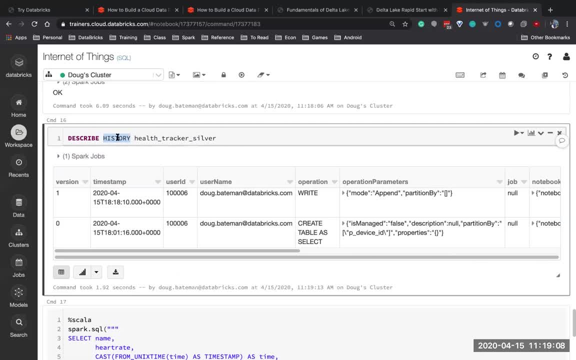 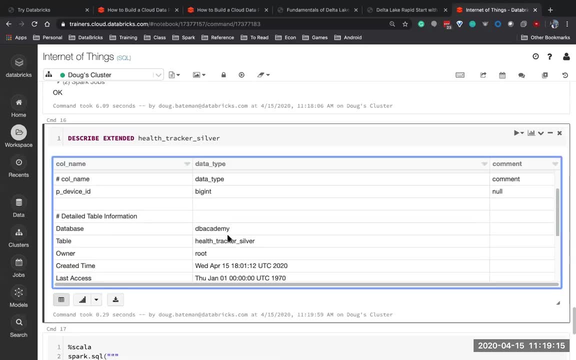 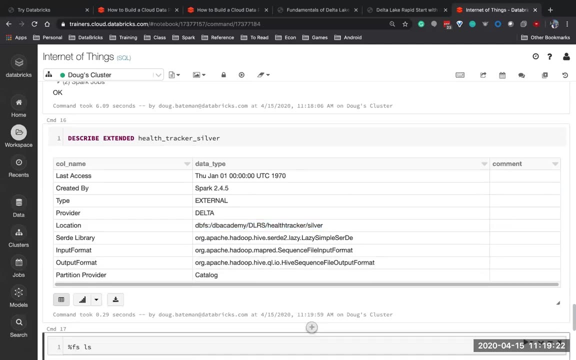 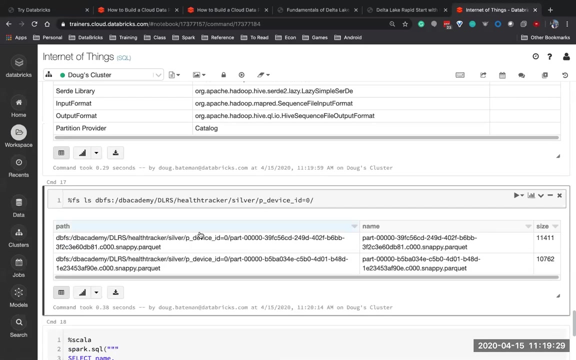 And I could even go and look at the directory. Let's go to the directory for my silver table And let's look inside of one of these partition folders And you see That it's written out another file part. It's appended a second file to the first and now we haven't deleted anything. 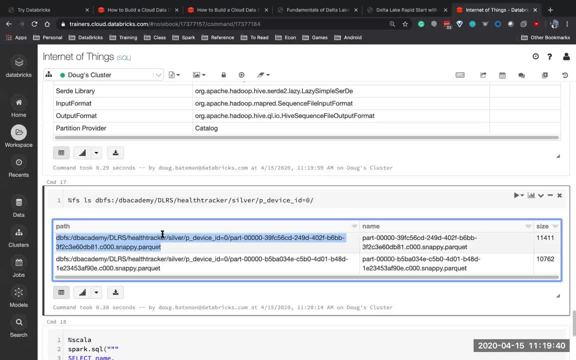 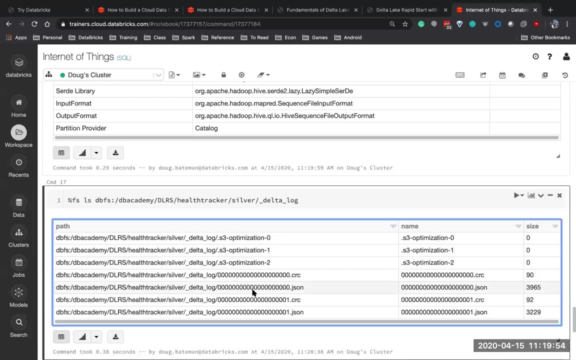 So both of these files are considered good. None of them have been marked in valid yet, but if they were marked old, that would have been marked in that metadata directory that we talked about The JSON log or the Delta log. So if I look at the Delta log you see that I've written out a new record to the Delta log that says: 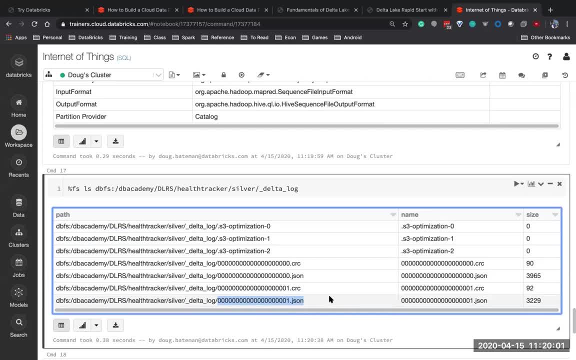 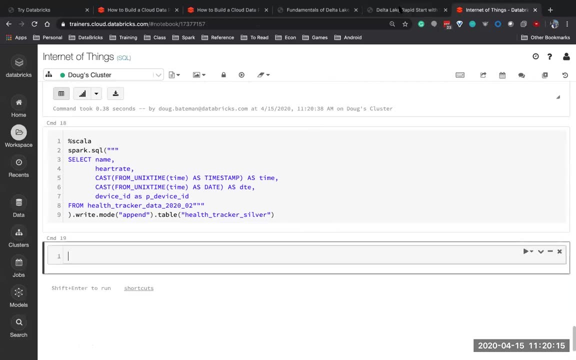 what's the new state of the files on data- And this is constantly being appended to- to let me see the state of files on disk as I add new files or delete files from the table. All right, let's continue on here. That was an insert into what if I wanted to view the old version of the table? 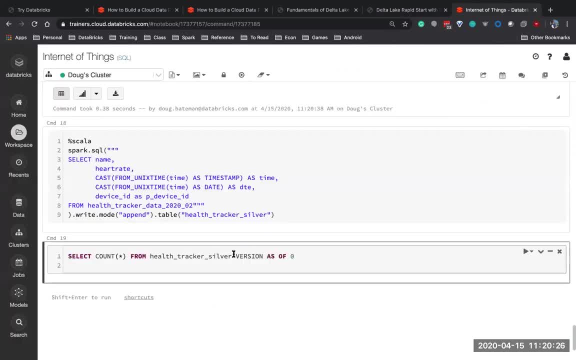 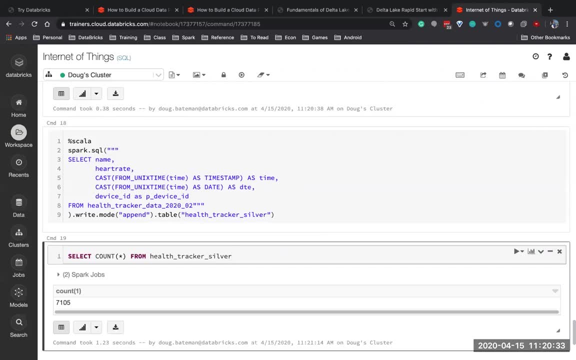 So, right now, what I want? to run a query. Let's just run a query on it and not do time travel. I want to view the current state of the table. There we go. The current state is 7,105.. If I wanted to view, though, the earlier version of the table, I can say version as of zero. 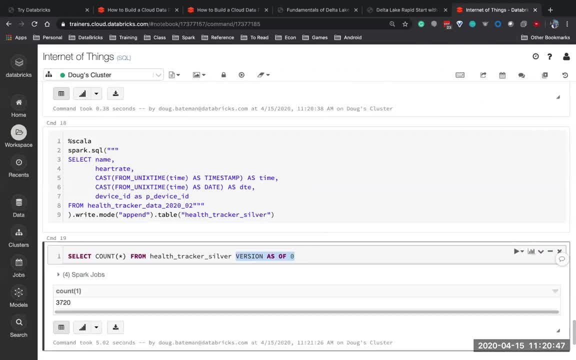 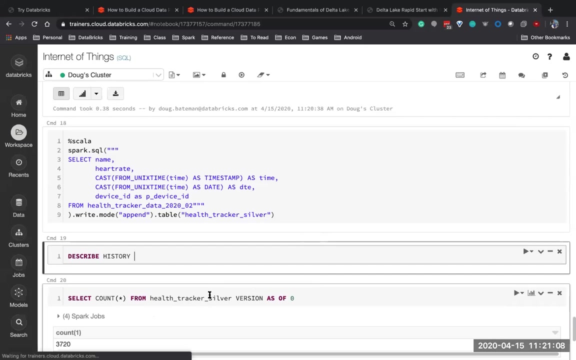 And I get to view the original version of the file: The 2720 versus 7105.. So that had quite a bit of new data, So I'm going to go ahead and add that to my file. Now let me go back again and do describe history. health tracker silver. 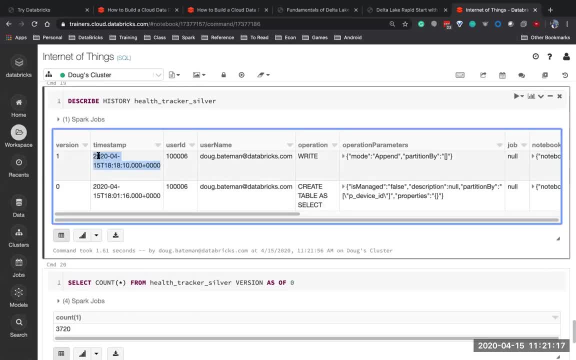 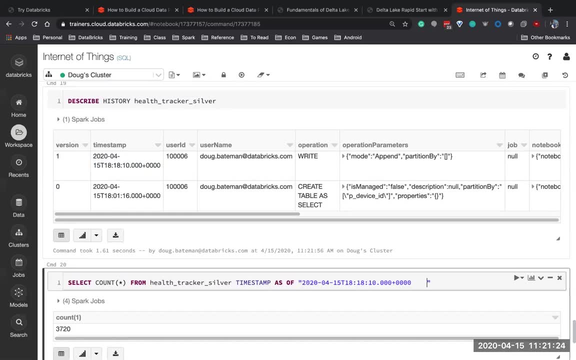 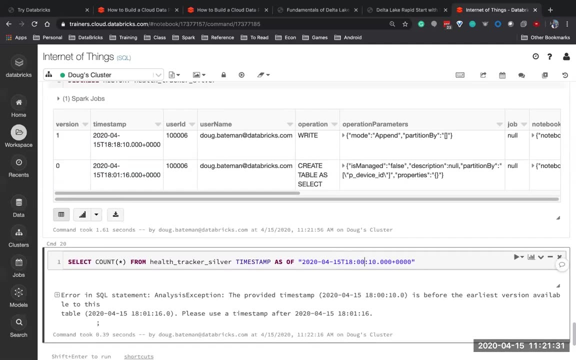 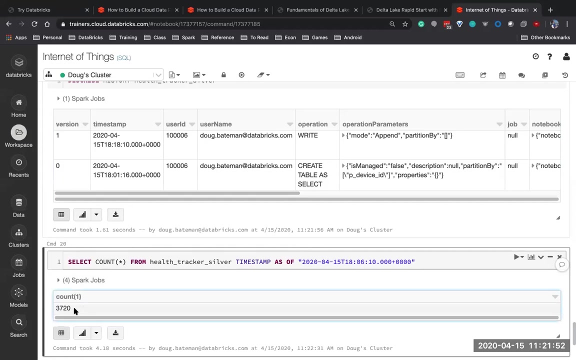 And let's grab this timestamp. I could also do timestamp as of and give it a specific time, So let's go to a time that was a little bit earlier. Ah, there we go, And this time is between the two, So it'll automatically figure out that it should show me version zero. 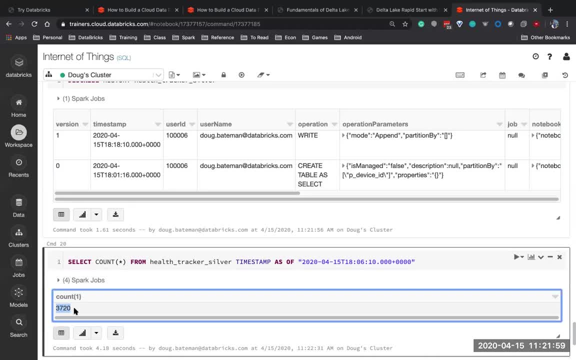 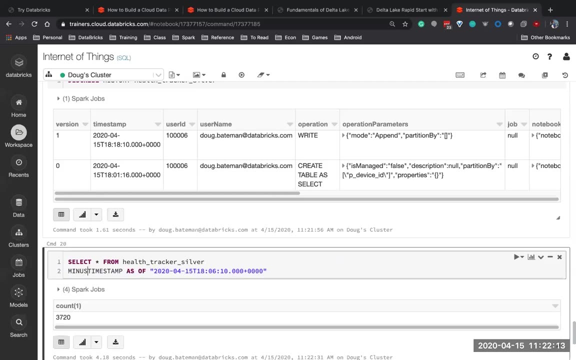 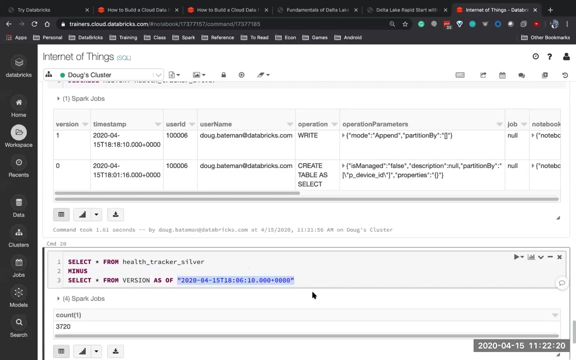 So I'm able to view previous versions of this data. I can even do a query where I get to see what's changed. So I could say select star from health tracker silver minus, select star from health tracker silver version as of zero And see what's changed between the two. 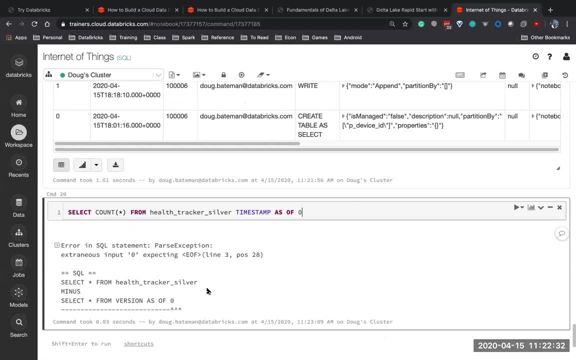 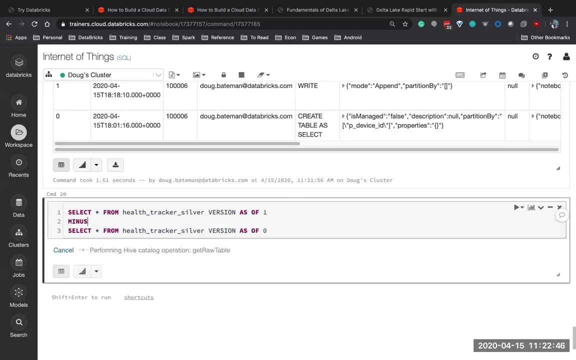 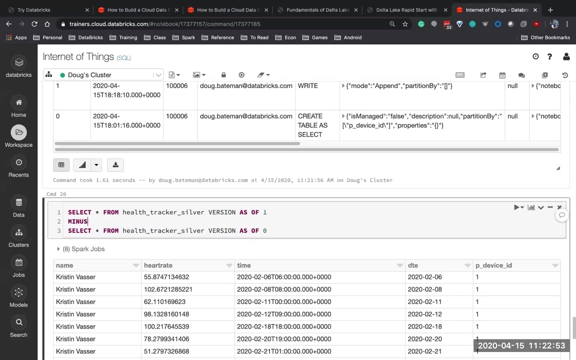 What did I do wrong with my version as of Fix? that Version as of zero should be working. There we go, And I could see what changed between the two versions, which is really cool. Ah, somebody had noticed in the courseware. 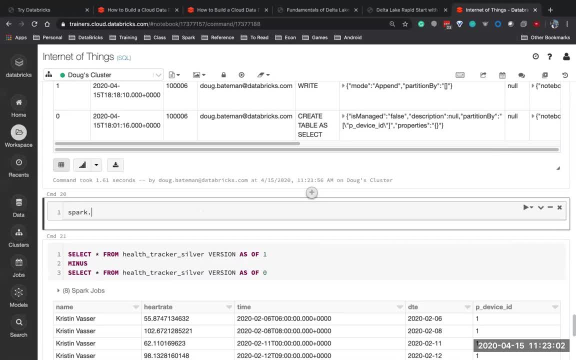 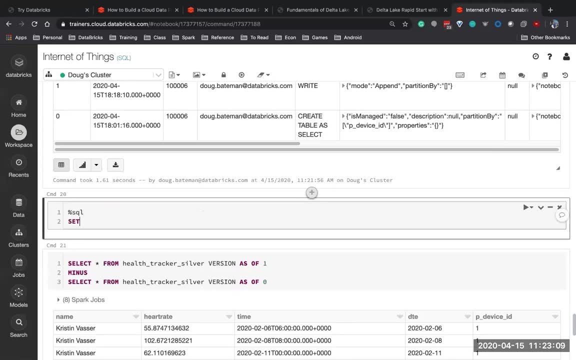 the course has this tip. They say you could go sparksqlcomp and change the number of shuffle partitions. So you go percent SQL, set comp or set sparksqlshufflepartitions and change the number of shuffle partitions. That's a performance tuning option. 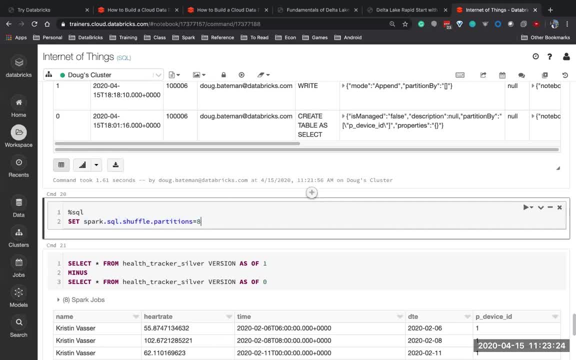 If you have a small cluster, you'd set this to eight. I actually have a much bigger cluster with 64 cores, Depending on the size of your cluster and the size of your data. this is a setting that you can change. I deliberately did not go into this. 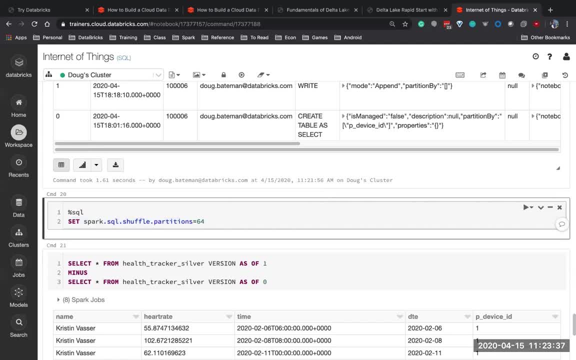 but somebody noticed that it was in the written courseware And I didn't go into this because I didn't really want to explain what this setting is all about right now. It's a performance setting thing, People. the course suggests that you set it lower for your smaller clusters. 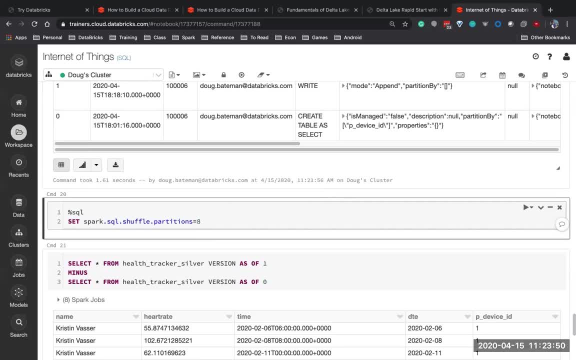 to make things run a bit faster. We're going to just sideline that discussion because it's really a performance tuning topic. The default is 200, and it works very well for both small and large datasets. We don't really don't recommend changing the default. 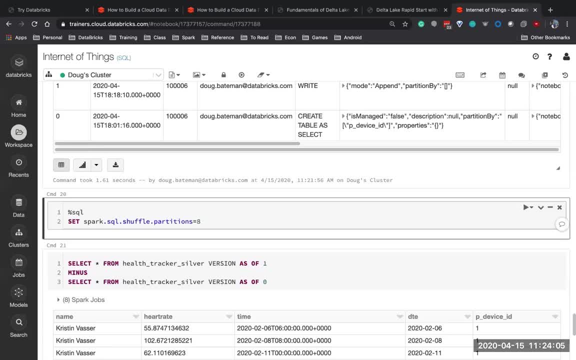 unless your data is truly small enough that you can afford to go smaller, And in our case our data is in fact small enough. But I'm not going to go in any more detail than that. It's just somebody had asked a question several times, asking what happened to that. 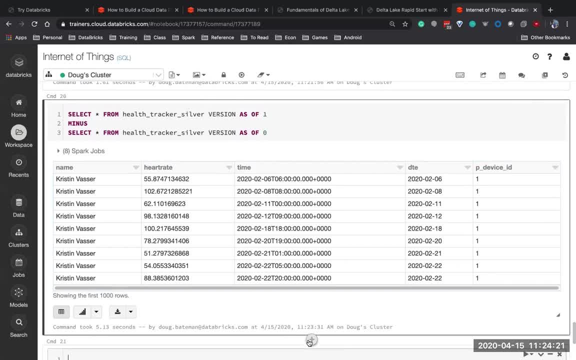 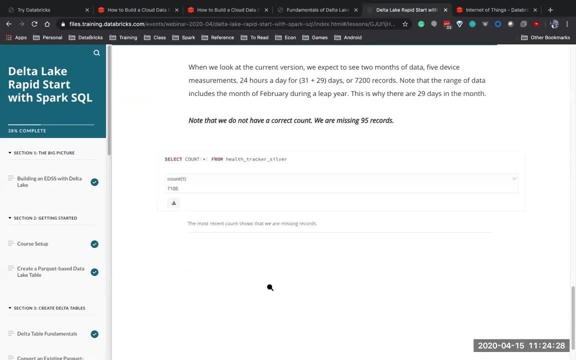 and I just skipped it intentionally. Let's continue on. So at this point we are able to do time travel to view earlier status of the table, which is really nice, And if we don't tell it a version, then we're seeing the most recent version of our table. 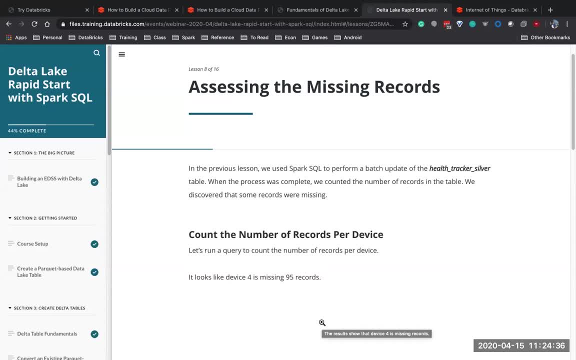 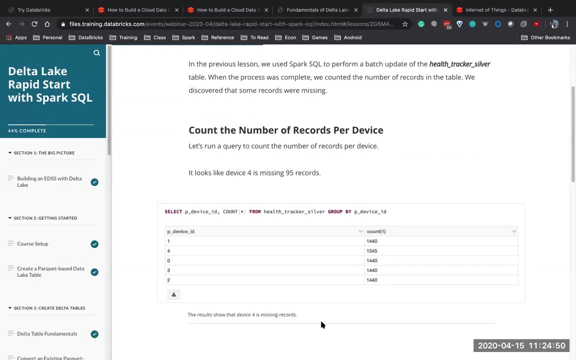 So at this point in the previous lesson we had done a batch update to the silver table And we were able to count things, But there are actually some missing records in our data. And to discover that we've got missing records, let's run this query. 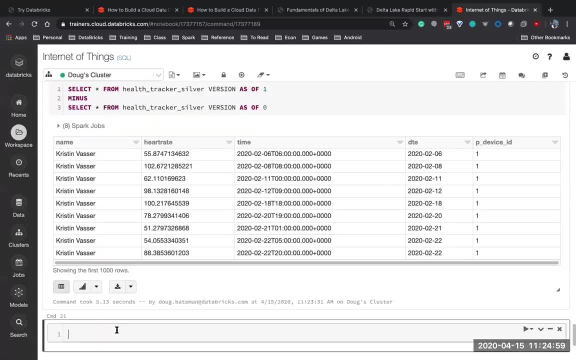 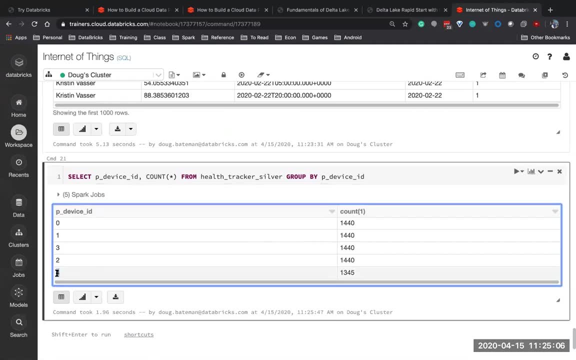 Because during ETL sometimes you didn't ETL correctly. So here's an example. Let's just run a query on our silver table and notice that one of the devices has significantly fewer records than the other devices deal Here. I'll even order by P device ID. It's in order And you can see that row four has fewer. 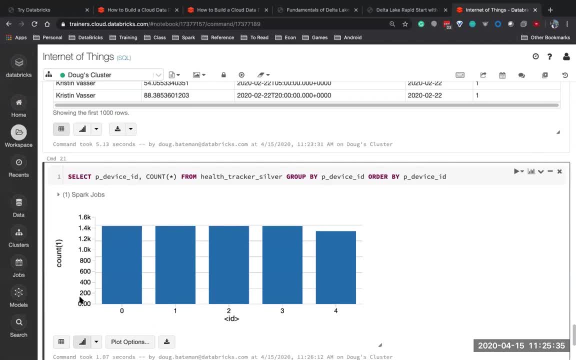 records than the other device. They could even do this as a bar chart And I see that I've got fewer records And this is not unusual. that you do an ETL and you discover that you have fewer records than the other device And you can see that row four has. 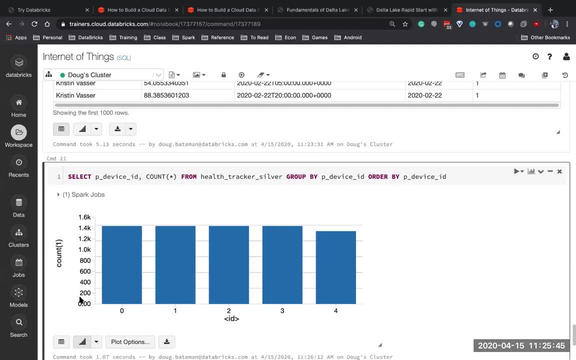 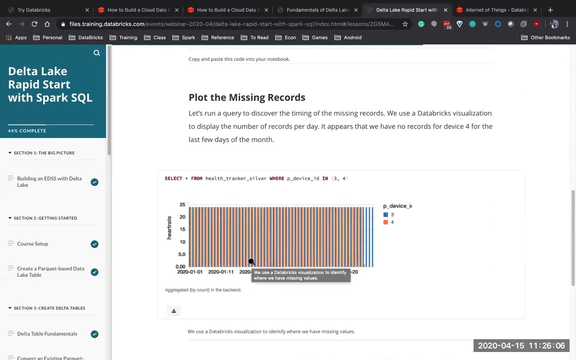 fewer records than the other device, And you can see that the data that I used when doing the ETL is out of date. So or it was wrong, And now I've got to go back and do some corrections. So that's what we're going to deal with next. So we could try to do a plot here to get a sense. 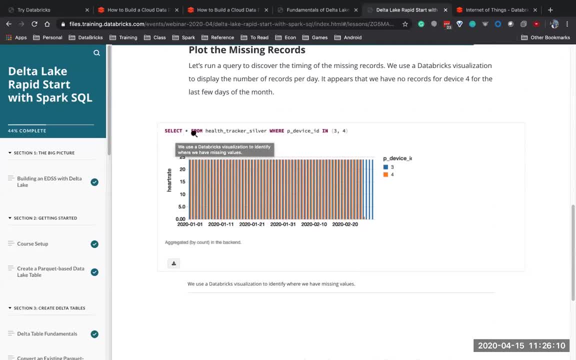 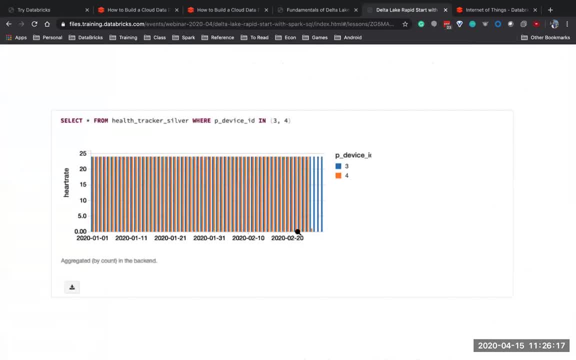 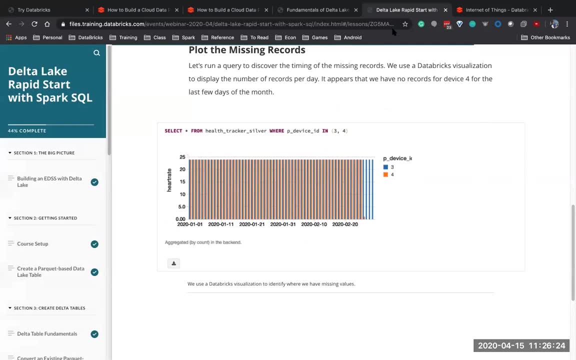 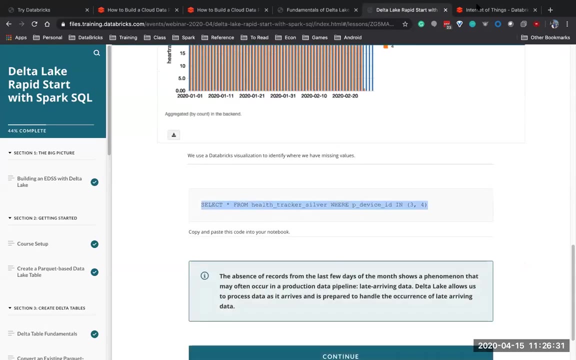 just look at devices two and three And in this case it's not going to show up in a really pretty plot because I'm not grouping by date. Well, let's see. Let me come back. If I go select, let's run this query. I may have to tweak it a little bit, Because when I run this query initially, 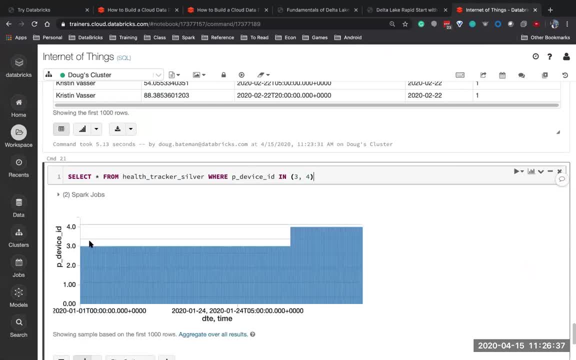 it's going to be a little bit cluttered. Oh, there we go. It's actually not too cluttered. You can see that I am missing some data. So I'm going to do select star from health tracking software And I could do select star from health tracking software And in this case it's not going to show up in a really pretty 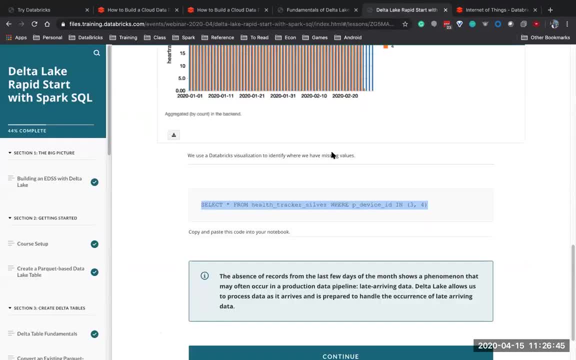 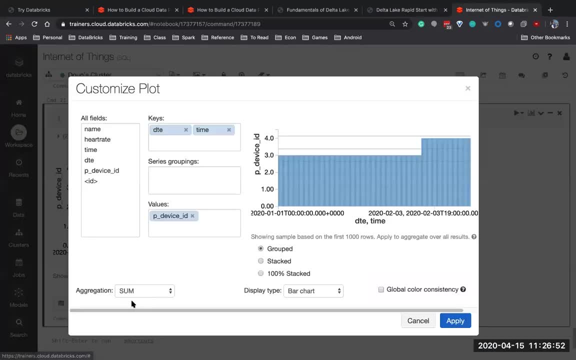 data for certain dates And let's try to make it match a little bit. So I want to look at the date and the count of the records. So I'm going to come in here plot options. I'm going to look at the. 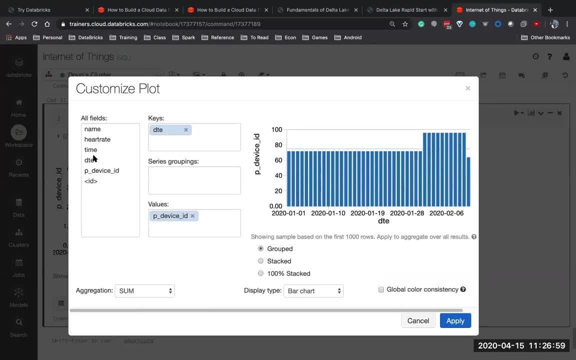 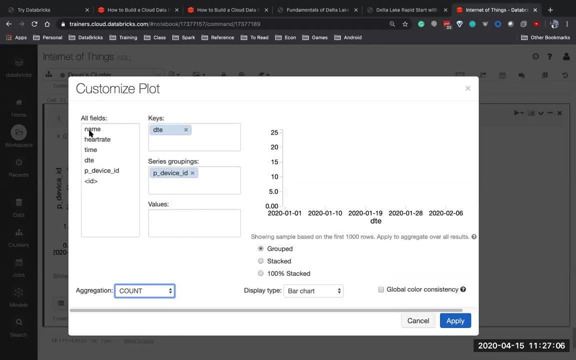 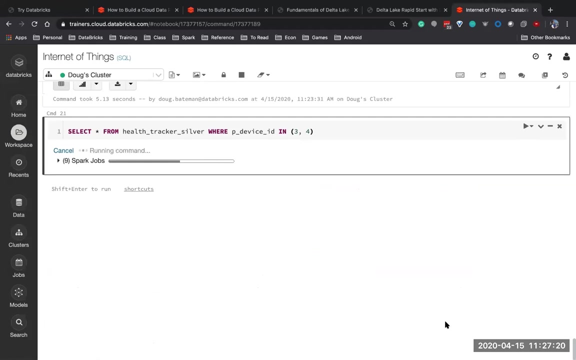 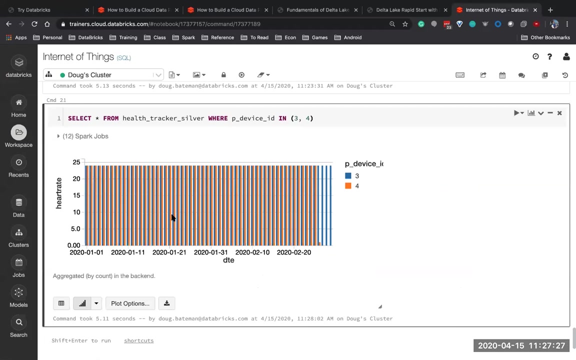 date And I'm going to look at the count And I'm going to group by device ID And I'm going to look at just the count of the heart rate records And what I see here is that I've got most of the data but I'm missing device for starting at a. 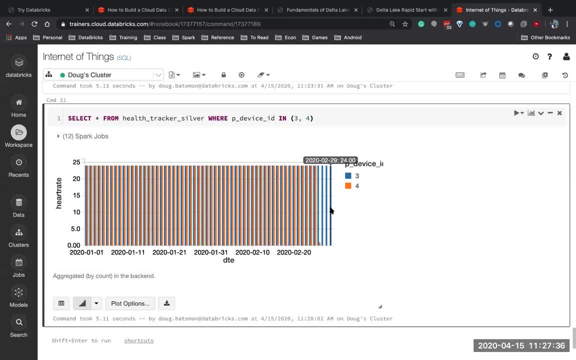 certain date, Because the input data that I ETL'd was missing it. I didn't have it, So we're going to have to need to go and back load it And I'm going to go ahead and do that And I'm going to 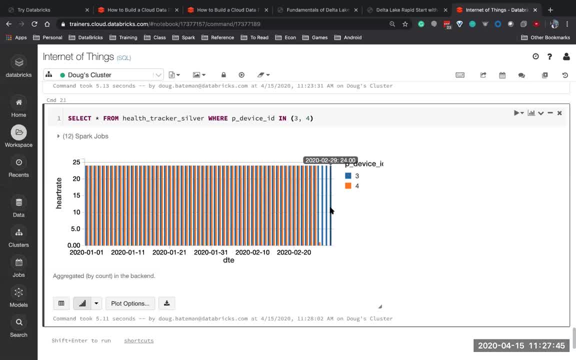 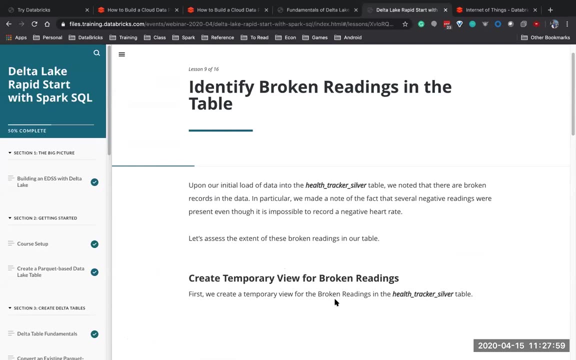 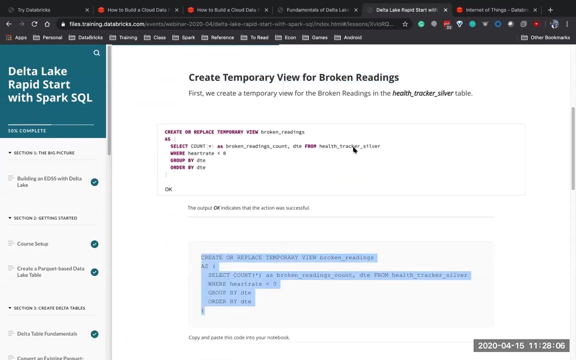 go ahead and load some data and update our table to have this new missing data, And that's an incredibly common type problem, So let's address it. We have clearly some broken readings, So we're going to first create a temporary view to identify our broken readings. So let's talk about what a 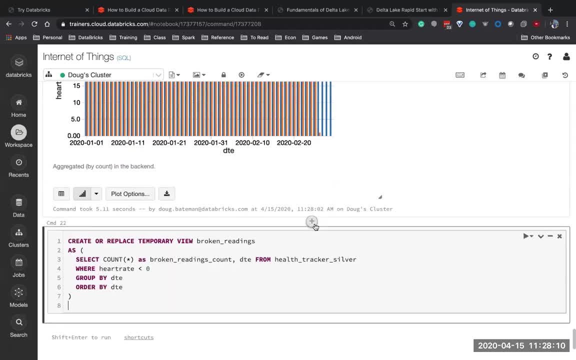 temporary view is, So I'm going to create a view. A view is nothing more than a stored query, So, unlike creating a table which would be written to disk, a view is just a query that whenever I query the view, I'm really 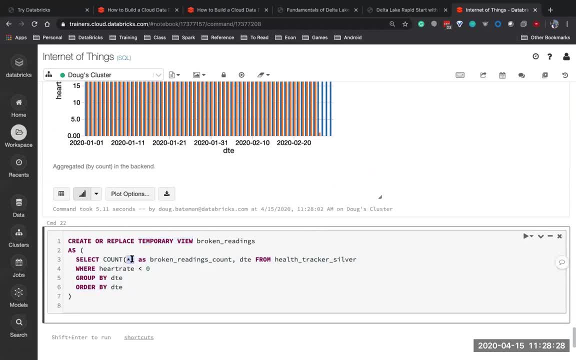 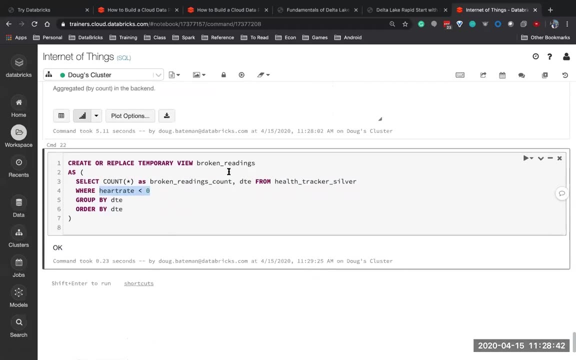 running this underneath query And I'm going to count how many of these exist where the heart rate is less than zero, Because those are some broken records here where I had these negative heart rates And let's query this table now. So I created a view that I could turn around and query And the view 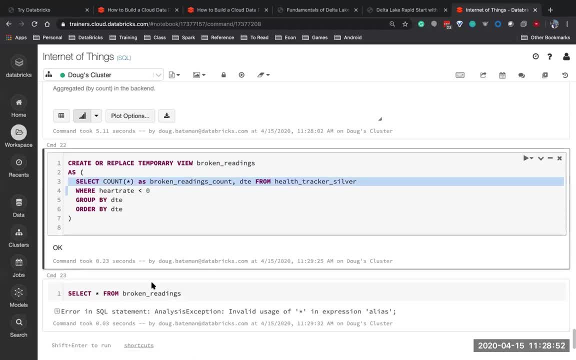 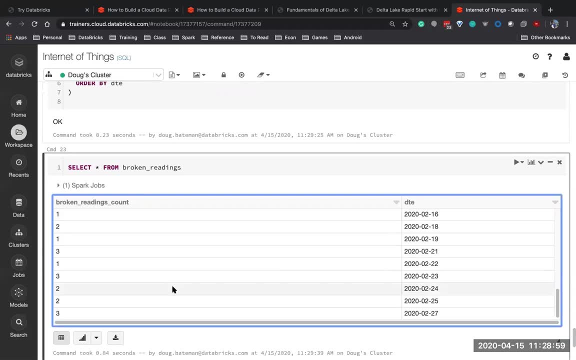 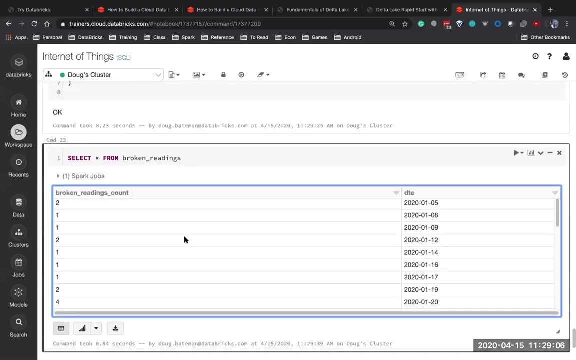 is not written to disk. It is really running this query underneath every time And, sure enough, I have quite a few readings where I've got negative heart rates And this is leading to some data corruption, So there's a lot of problems in my data. 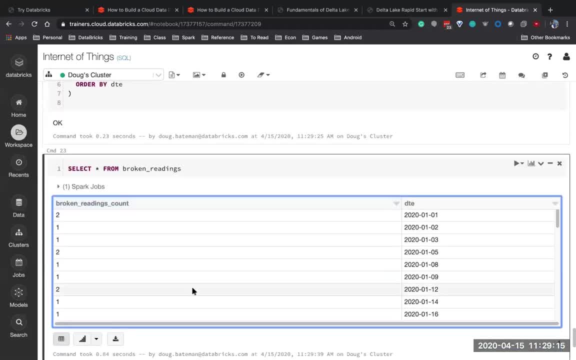 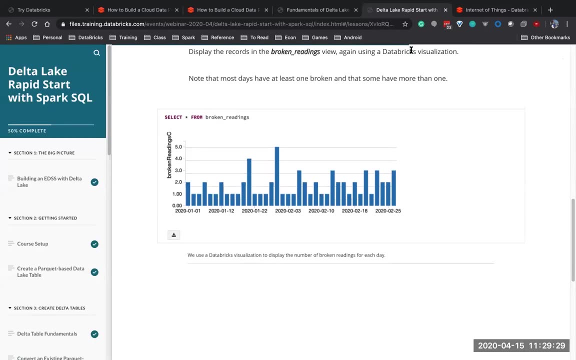 I've got missing data And I've also got negative heart rates. that's dirtying my ETL And I need to go back and fix this. So let's first display them So we could run just a little plot here. That's what we did down here. 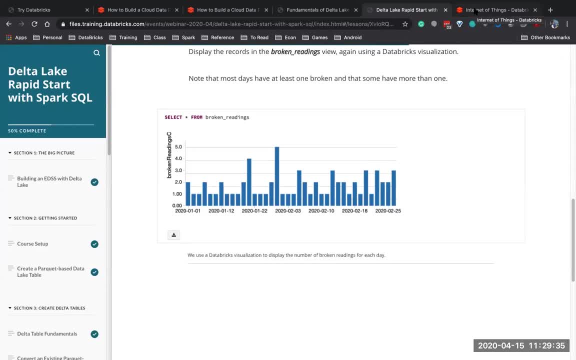 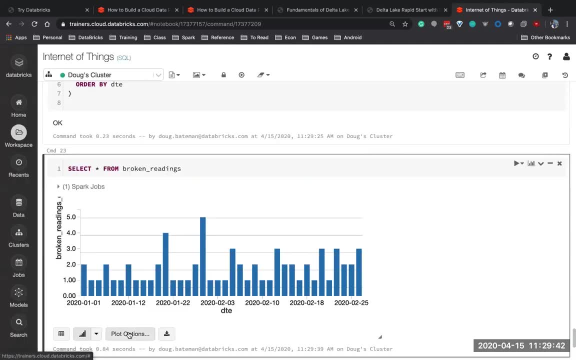 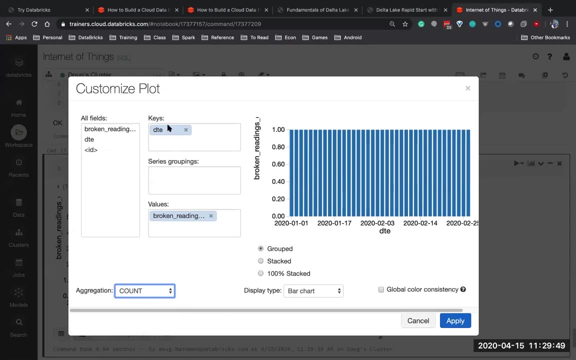 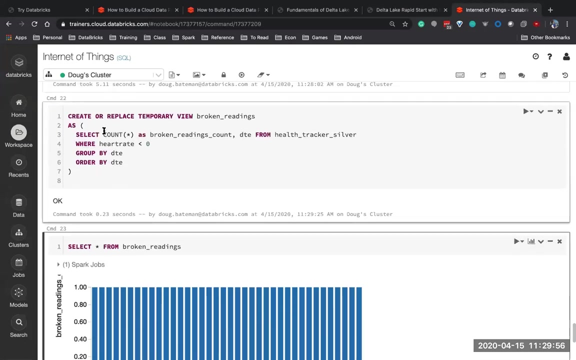 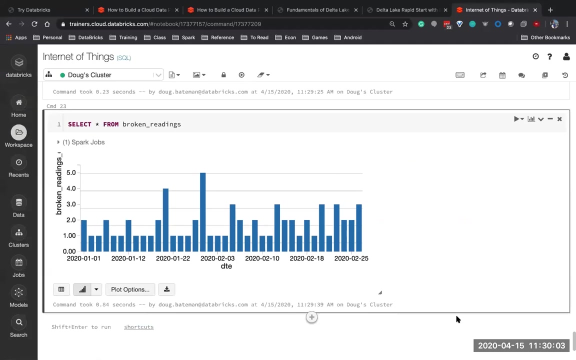 But let's turn this into a plot, because I think plots say a lot more. So let's do it by date. So I'm going to come in here, do a bar chart by date. So I go, plot options. I want to look at the count of the broken readings grouped by date, And let's see here: Oh, I've already got the count. My bad, I don't want the count, I want the actual values. There we are, And because I already had grouped them by count up here, I didn't want to count the count. That wouldn't have worked. 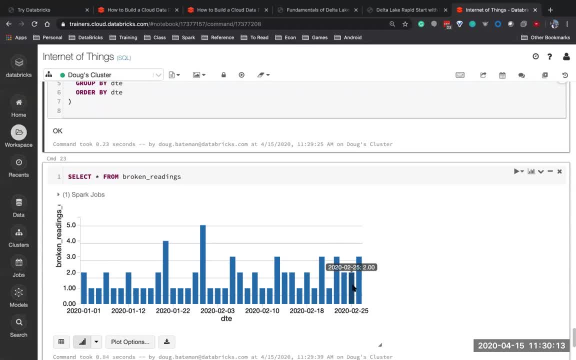 And you can see: yes, indeed, I have broken records for some of our data that I need to go back and correct, And this is a typical thing to happen in people that are maintaining a data lake is that dirty data gets in there. you discover it later and you've got to go and do corrections or updates to your existing table. 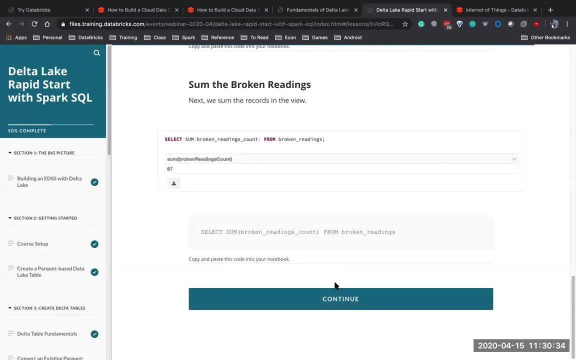 So how do we go about doing that? We could also get a count of how many total broken records there are. I could sum them up: There's 67.. I'm going to skip doing that. Summing up the counts for a total of 67 broken records. 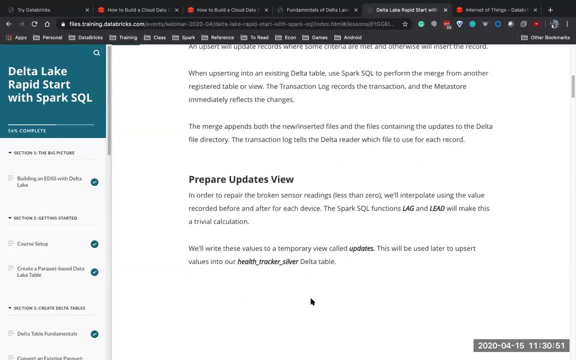 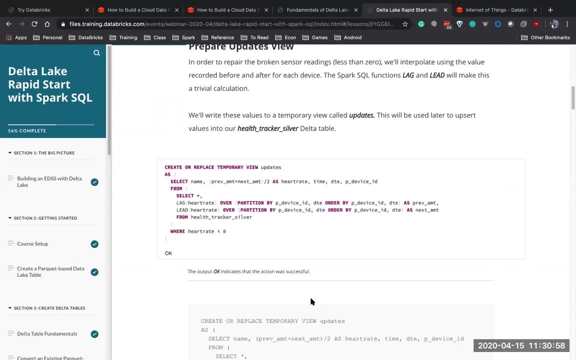 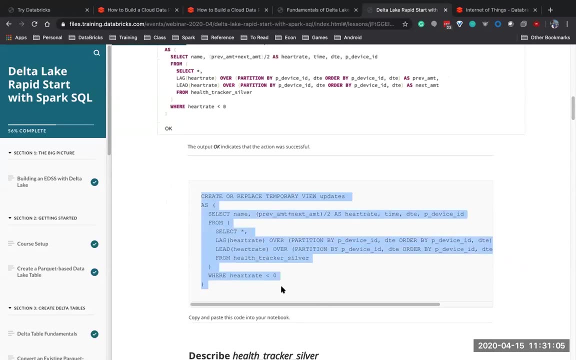 Let's repair them, And the way we do a repair in Databricks is we're going to use what's called an upsert, And an upsert allows us to merge in corrections to our existing table. So to do that, the first thing I need to do is to grab the data that I want to do corrections on. 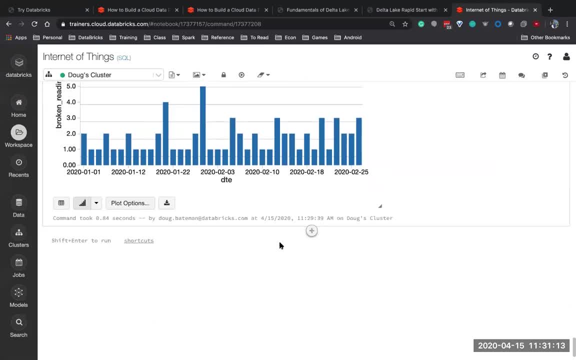 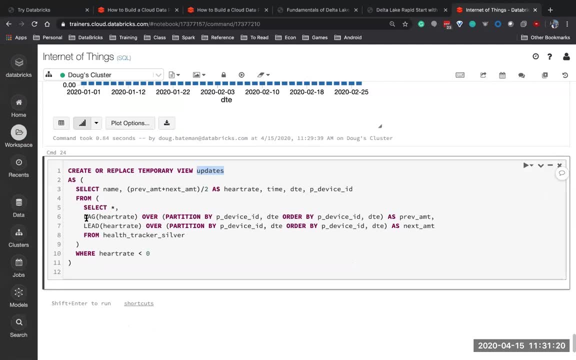 So let's grab the data that we want to do corrections on. So we're going to make a temporary view updates. This is just a query here. I'm going to Look at the each partition. So this is actually using what's called a window function. 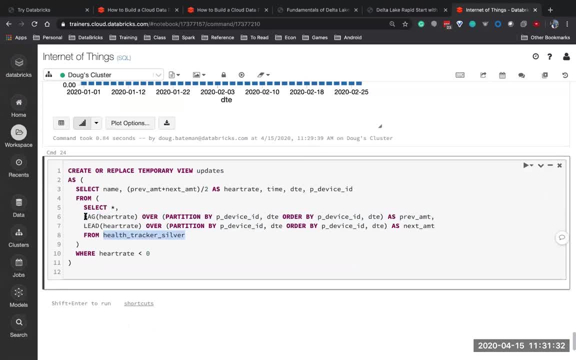 And we're querying the silver table and we're looking at what is the first and last heart rate in a window of time. So we're looking at the first and last heart rate. So we're looking at the first and last heart rate. So we're looking over- in this case, over the device and the date, and we're trying to get the first and last heart rate and we're going to average the two. 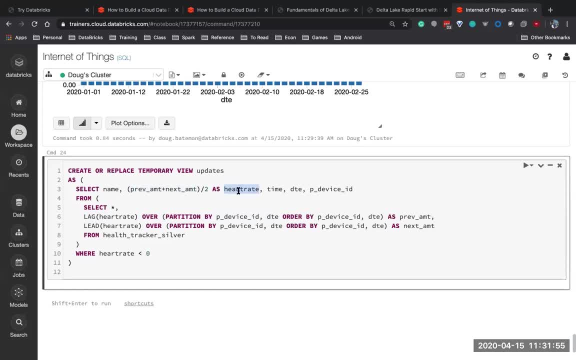 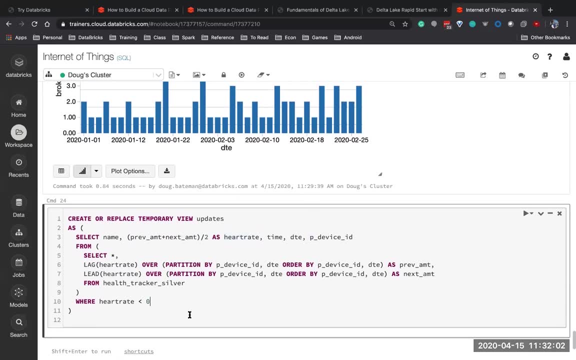 The minimum and the maximum. We're going to average the two to make it a heart rate, because what we had was the duplicate data and some negative data. So we're just going to write a really fancy query that's going to average the two, but only in cases where the heart rate was less than zero. We're going to instead average them and get something better than zero. 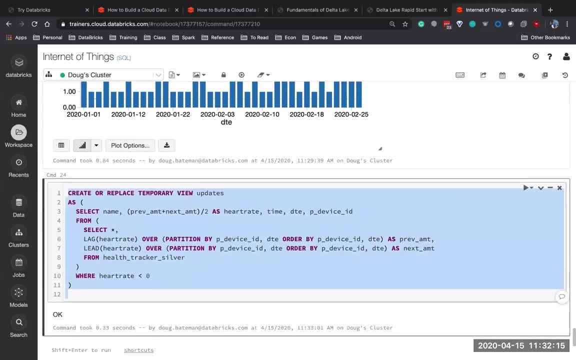 So we're just going to write a really fancy query that's going to average the two, but only in cases where the heart rate was less than zero. Just a way of doing analysis to correct for bad data. And let's just take a quick query of our updates table. 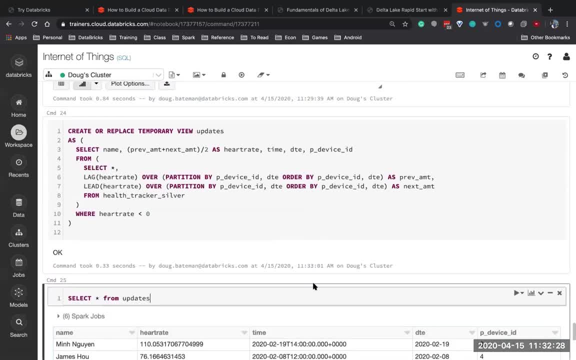 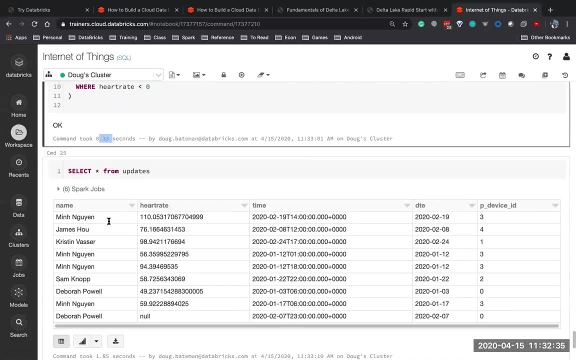 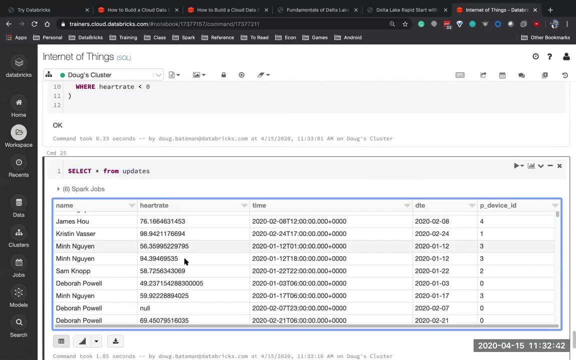 Or updates view, I should say. Notice, defining the view took no time at all because it didn't actually run anything. It just defined this as a query. It's actually doing the math when I query the view. It's lazy, But now notice that my heart rates are positive, although I have a few nulls in here. 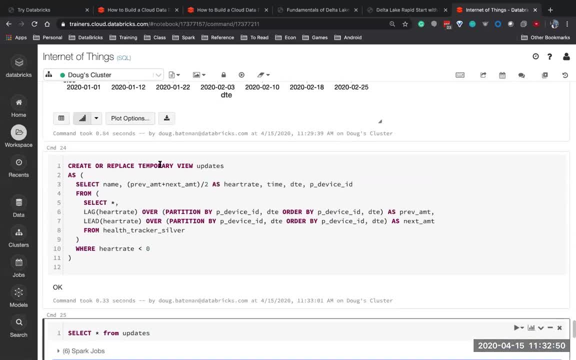 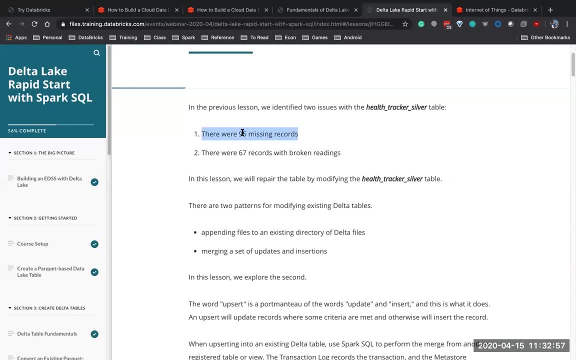 Otherwise, my heart rates are positive. This is a way of correcting for bad data, So I just want to go back and talk. So there was a bunch of missing records- 95 missing records and 67 records with broken negative readings. So there's things that we could do. We saw that we could append files. 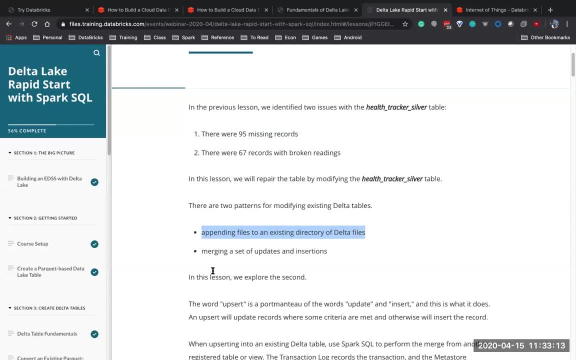 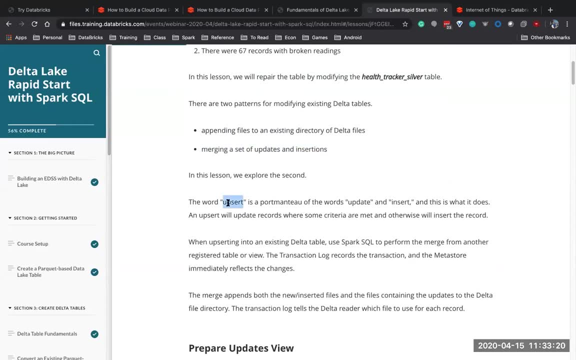 But in this case I want to go back and modify existing records, And this is where we're going to use merge to modify existing records using a process known as an upsert, which means I'm going to update the data if it's there, insert the data if it's not there. 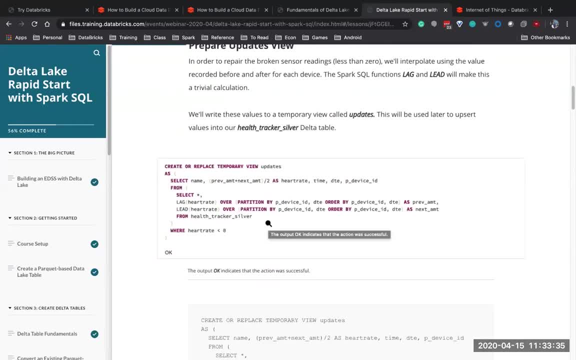 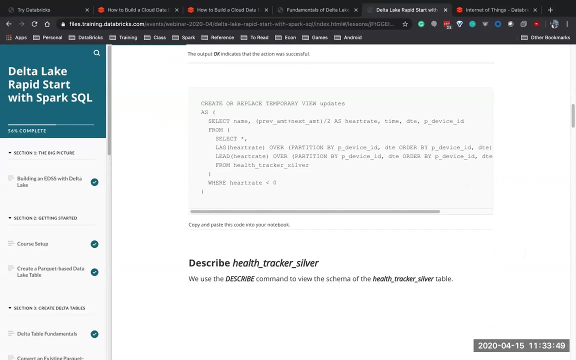 And to do that we ran this query to simply compute a replacement by averaging the good data. We're going to replace the good data. We're going to replace bad data with the average of the good data. Just taking a quick peek at questions Looks like we're good for the moment. 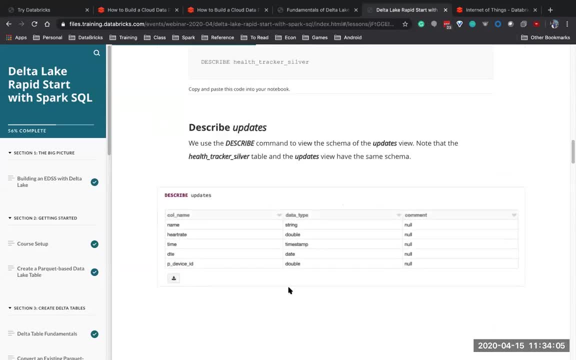 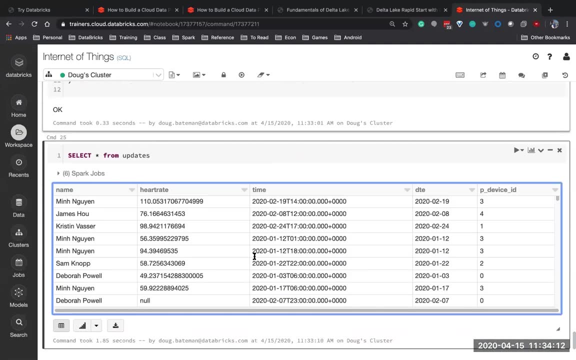 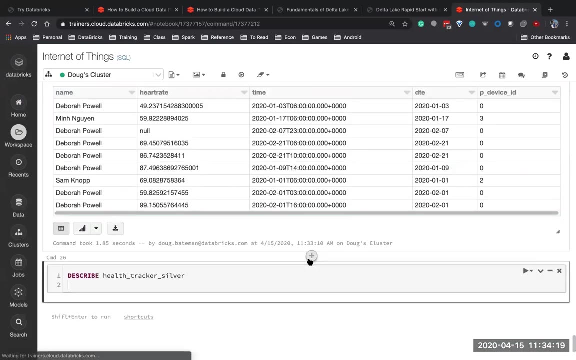 All right. So we want to do updates here And let's just compare the schema for HealthTracker Silver and HealthTracker Updates. Let's make sure that the schemas match So we have name, heart rate, time, date and device ID. We could actually do describe to look at the two schemas And we want to make sure that they match in order to be able to do this update. 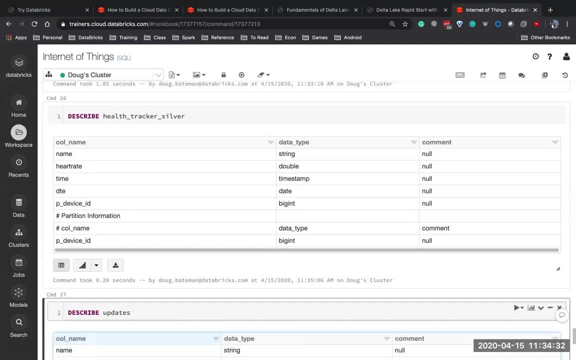 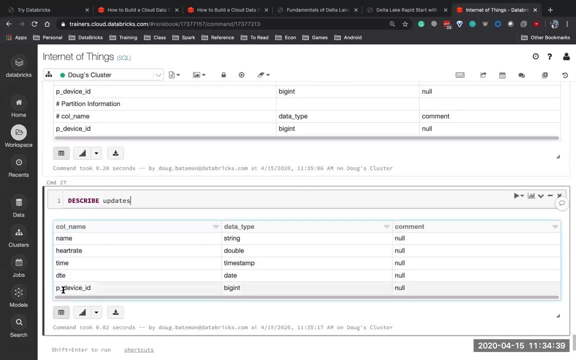 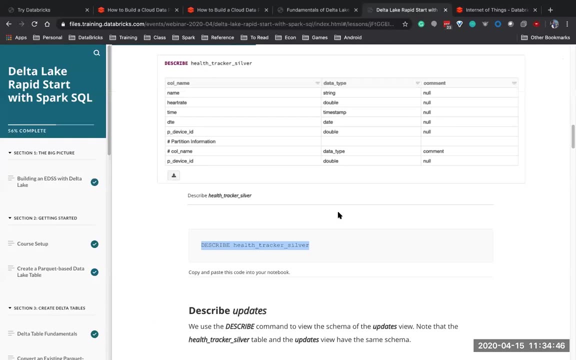 Updates And let's see, we have name, heart rate, time and date and device: Name, heart rate, time, date and device, So our schemas match. That is a very good thing, So we'll be able to do a merge operation. 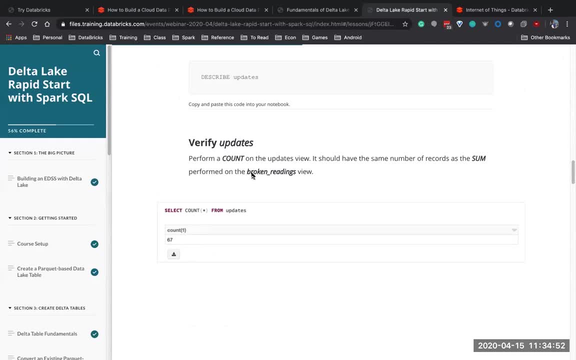 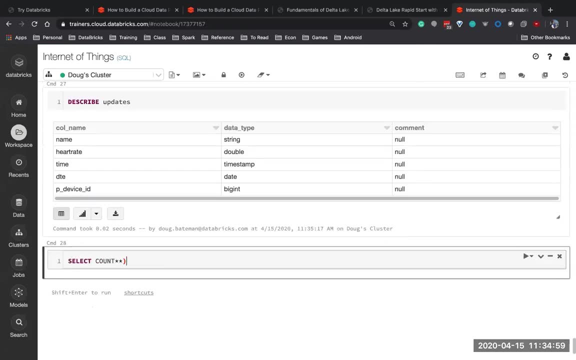 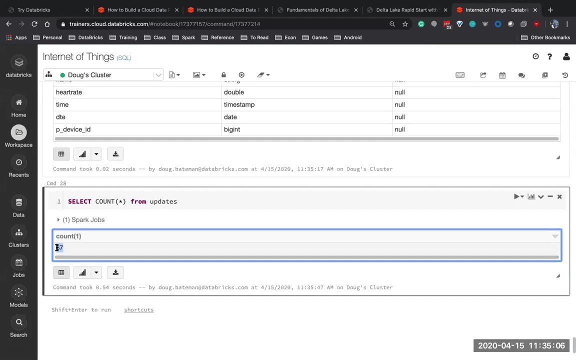 The other thing we might want to do is make sure that the new readings- So if I do a count star from updates- Notice that I'm putting in 6070 records, which matched the number of broken readings We had before, And this is the type of thing that a data engineer or a data scientist needs to do. We spend a lot of our time cleaning broken data, So a robust data platform needs to be able to clean broken data. 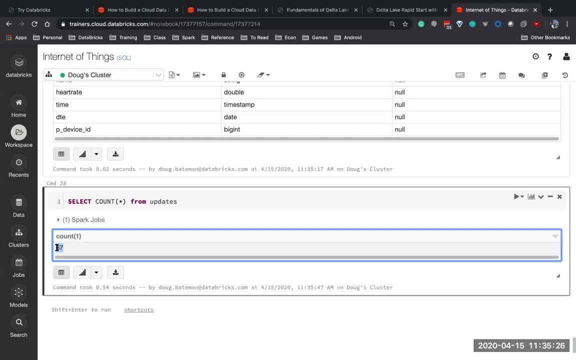 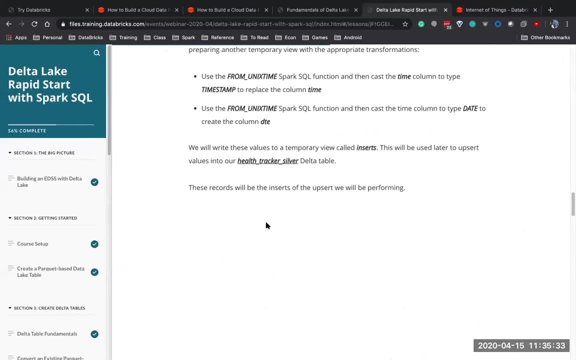 And the upsert operation we're about to do doesn't work on Parquet, but it will work on Delta tables. So let's get to where we do this upsert. So, first and foremost, let's make a table that's going to describe all the data that we're going to be using. 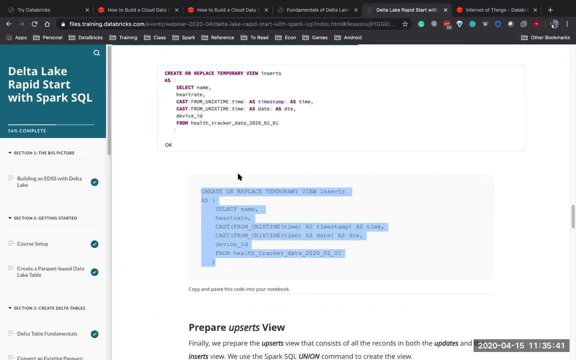 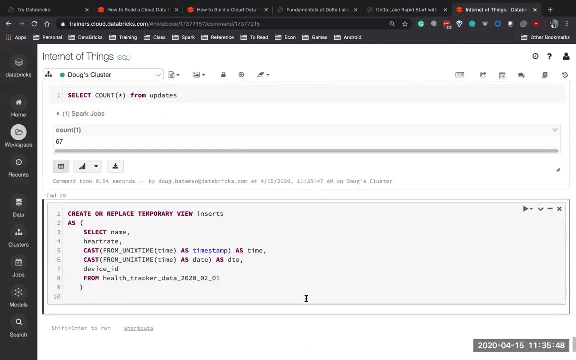 So, first and foremost, let's make a table that's going to describe all the data that we're going to be using, All of the tables that we want to insert. That's the new data and all the tables that we want to update. That's the updates table. We're going to make one table that's got the new records I want to insert. 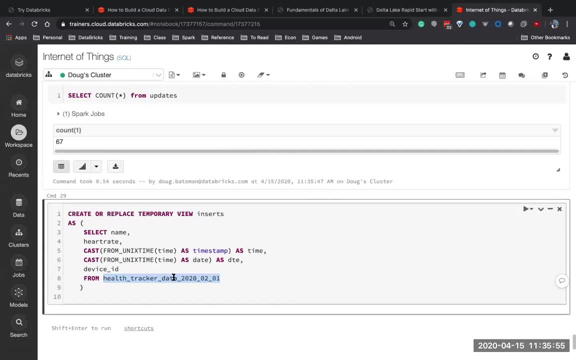 This is coming from this new file that represents our missing data, whereas update is the data that was broken because we had negative values. So we have a table for inserts- That's the data we want to insert- and a table for updates- That's the data we want to change. 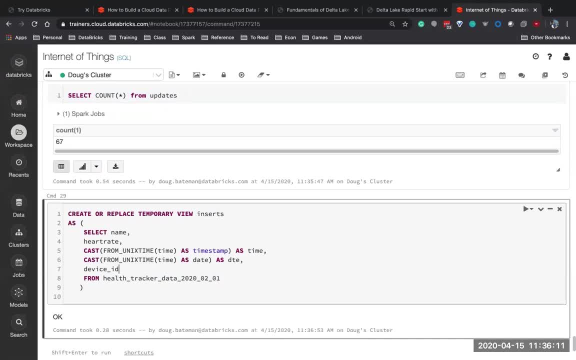 Let's make a view for each of these. Let's make a view for each of these So that we can then get to the command I'm really interested in, which is this merge command. I'm going to insert this data. I'm going to be updating this data. 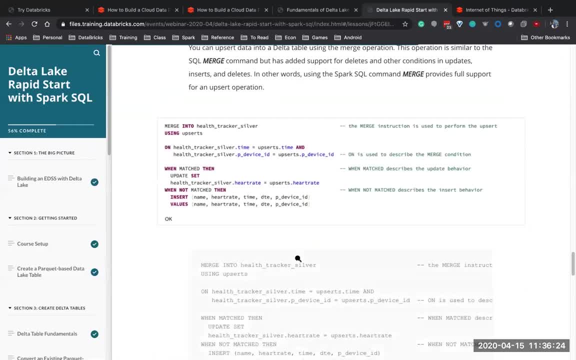 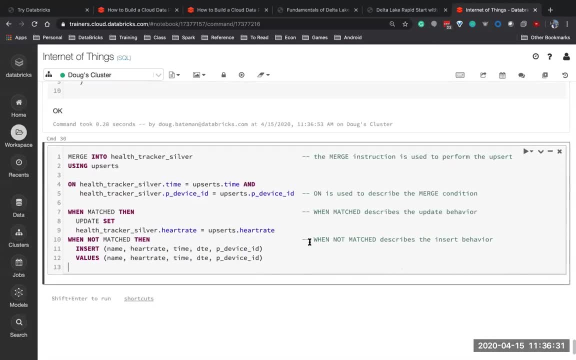 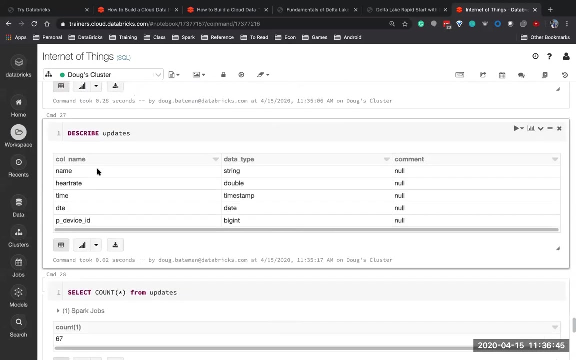 How do we do that? This is the secret sauce, The command I've really wanted to get to Merge. So I want to merge into my silver table. I'm going to grab things. Where's the upsert table? Hang on here. I miss a step. I may have missed a step. Let me look. 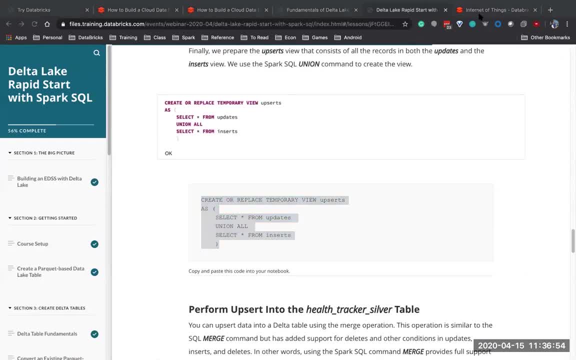 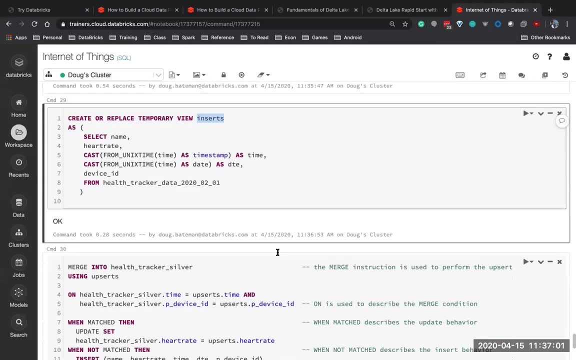 Ah, Yes, I did miss a step. So I told you we had the things we wanted to update. We had the things we wanted to insert. for the sake of it, Let's pretend like we just got a data of corrections. We could call this corrections. 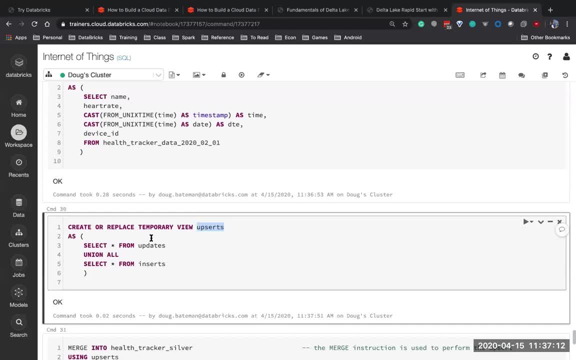 In this case we're going to call it upserts, but it's a table that's going to represent all the rows We want to change as well as all the rows We want to insert. We're just putting them together into one new data set that we want to upload. 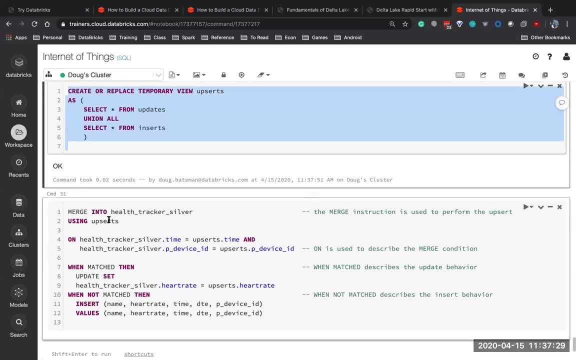 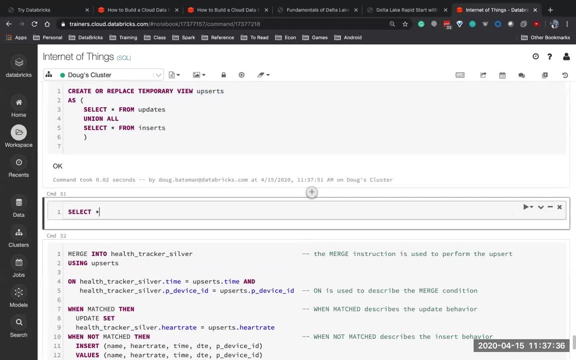 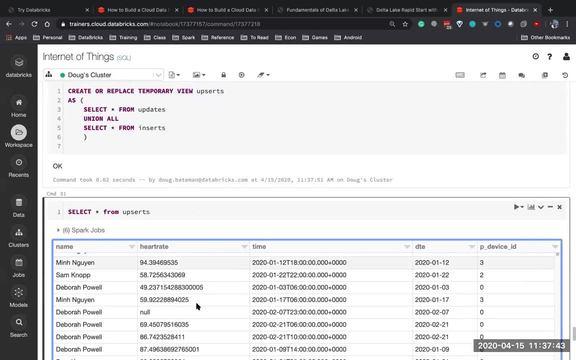 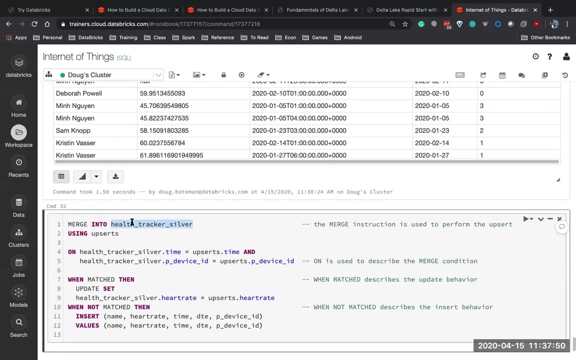 So now I want to merge this new data into my table. So let's just do a quick query, select Count or just select star from upserts, And this is all the data that I want to add. some of the data is going to be an insert, other data is going to be an upset update. So I want to go to the silver table And if there is a record that matches the device. 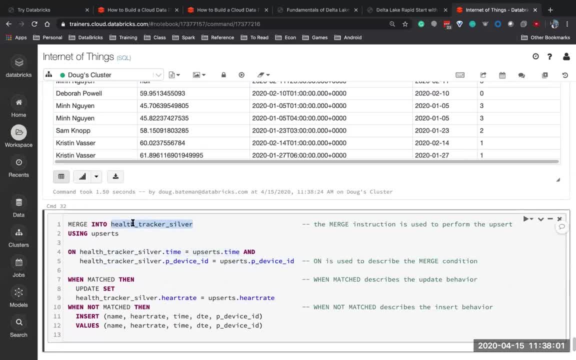 And the time If it's already in the silver table. So when it's matched, because it's already in the silver table that I want to do an update, command Update and change the heart rate for that timestamp so that it's no longer negative. But if it's not in the silver table, that is when it does not match. 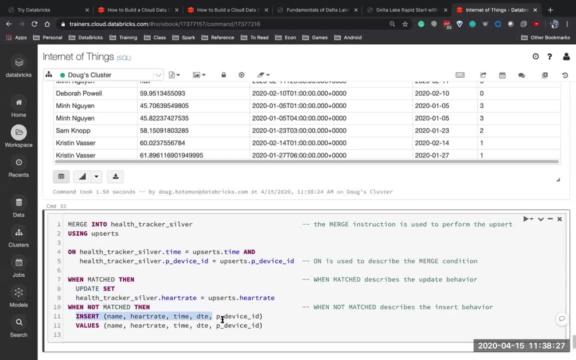 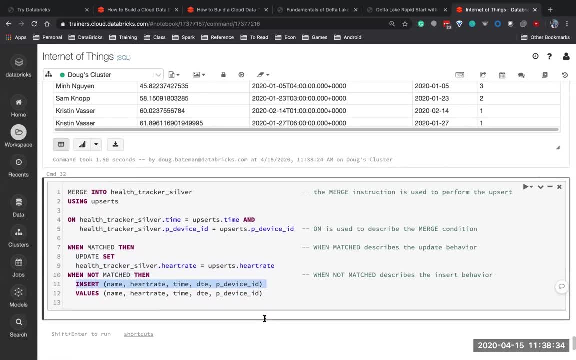 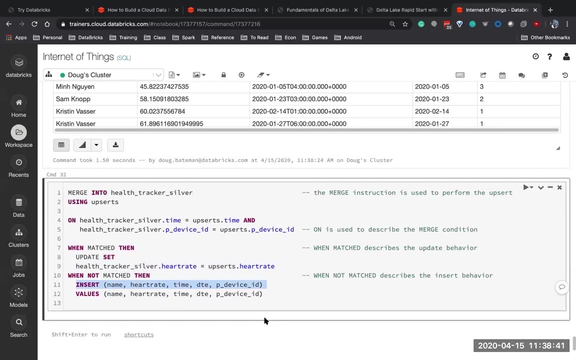 Then instead of doing an update statement, I want to do an insert statement and I'm going to insert this new data into my table Merges. how we do this update or insert in spark In a data or delta way. and merge only works on delta tables. So I can't use the merge command on JSON. I can't use the merge command on parquet. I need to be working on a delta table to use the merge command. 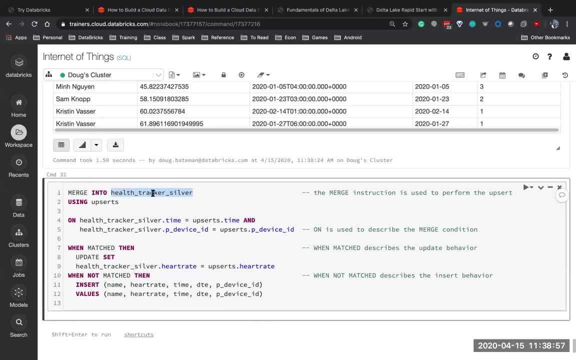 But it's going to let me merge in fixes to my data. If the data matches record that's already there, I'm going to change the record that's already there. If it's not already there, The data is already there, Then I'm going to add it to my table. 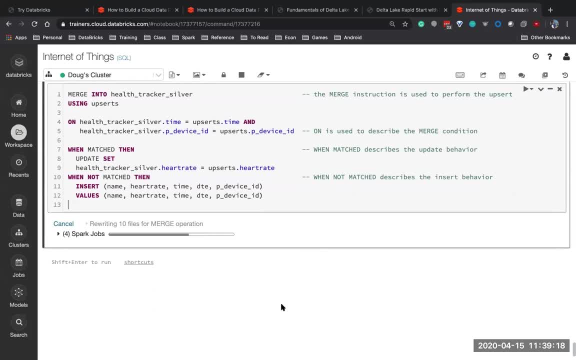 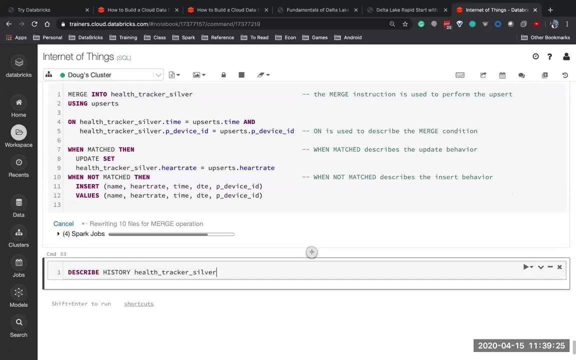 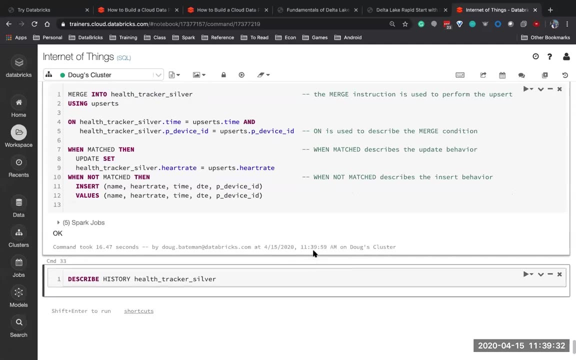 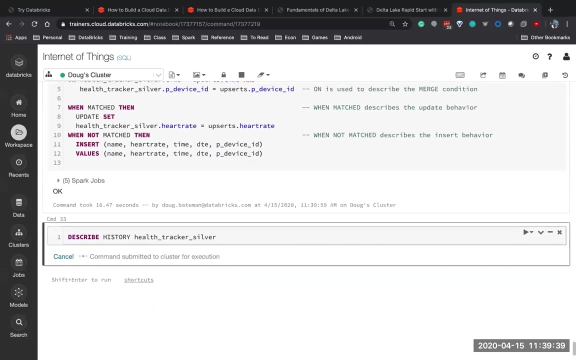 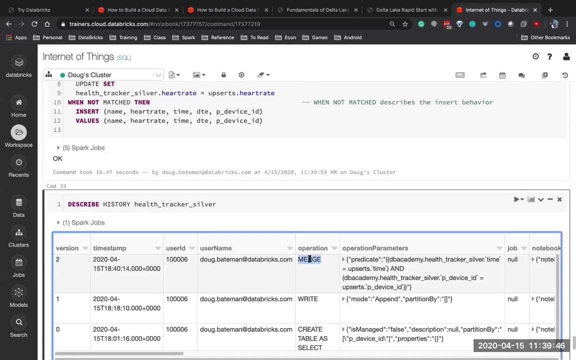 So let's run this And then let's do describe history. and look at my silver table. This absurd, this merge operation is how you are going to repair broken data in a table. So here we go, Let's describe the history now and we could see- I have version two now available- That was the result of a merge operation. 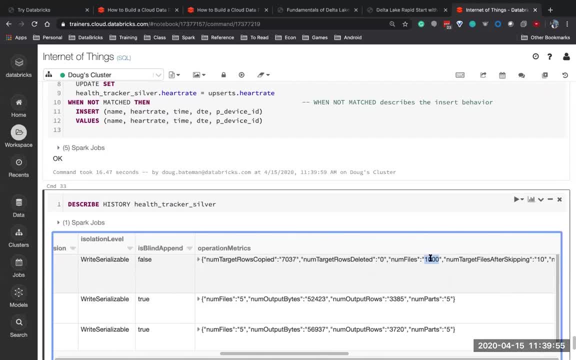 And, uh, looks like we've got a bunch of files that actually got out of this part of this process. a bunch of small files got out of this part of this process And you can see some of the files were deactivated. Here we go. Here's how many rows I inserted. 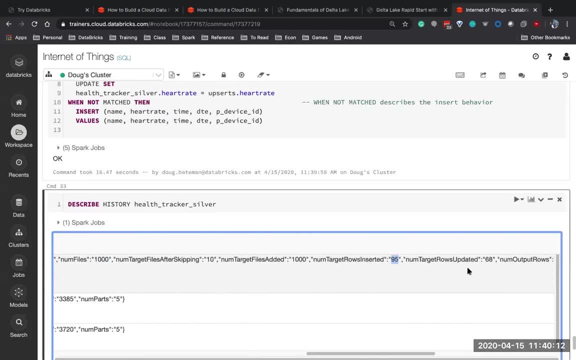 I inserted 95 rows. It looks like I updated 68 rows for a total number of rows in my table. that are 7000 rows split up into 1000 different files. Now somebody asked: is a view of a delta table also a delta table? The answer to that is: a view is not a table at all. It is a query result and it's not stored anywhere, It just gets. 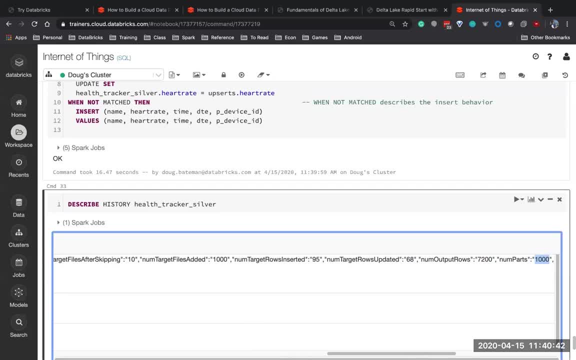 Reputed when you query the view. So views aren't really physical files at all, so that you wouldn't call them delta, you wouldn't call them JSON, you would just call them query results. So a view is a read only query result. 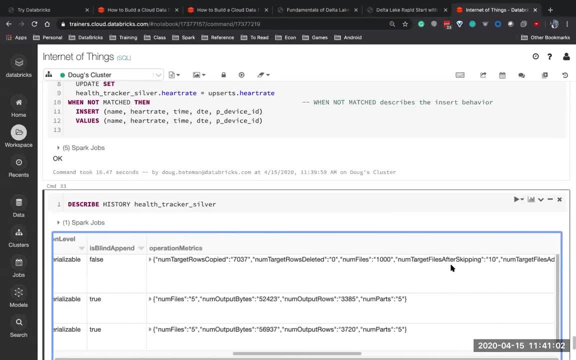 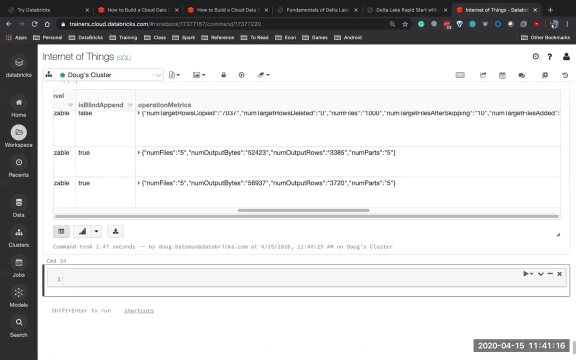 Alright, so we have written this out, but I'm a little bit concerned about how many files I have. I have 1000 files that got written out. That's a lot of files that got written out. So I'm going to jump ahead. We do this technically later in the course, but I'm going to jump ahead a little bit and showcase. 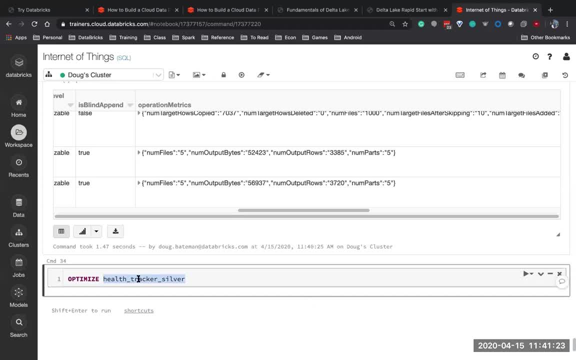 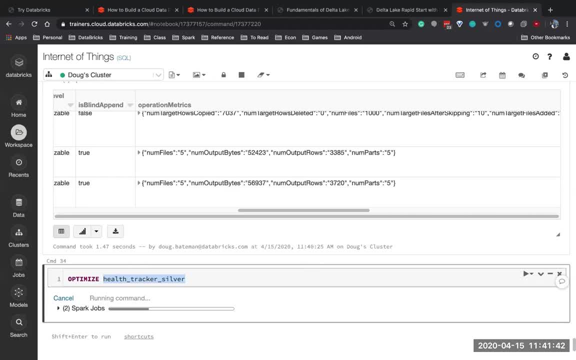 data. So previously we had appended data, but then we discovered there was dirty data and we wanted to append some new data And we also wanted to fix some negative values data And we also wanted to fix some negative values file And we also wanted to fix some negative values. 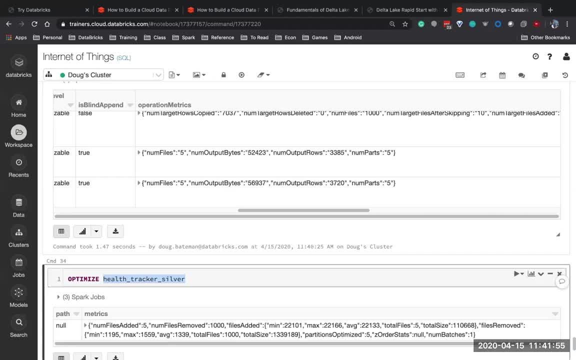 And that's where we did the insert. so in this narrative here we weren't just appending anymore, We're actually fixing and it's contrived, because I wanted to show you the merge command. So the insert into only appends, whereas the merge command Какcers nur наappăm. 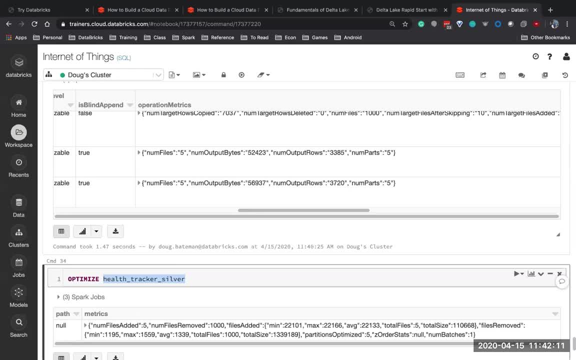 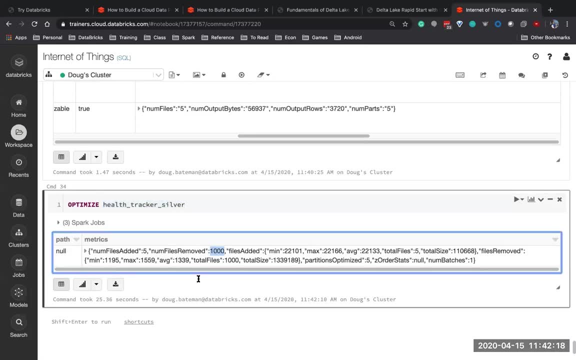 command appends and updates both, which is really nice. but now here I did this optimize command and it removed a thousand files and leaves me with only five files that are larger, so that querying this table will now be much more efficient. so the optimized command will compact small files into big files. 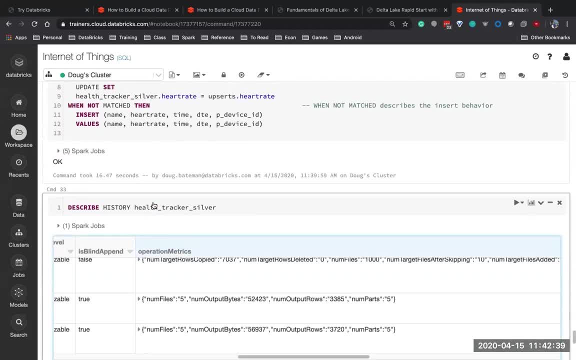 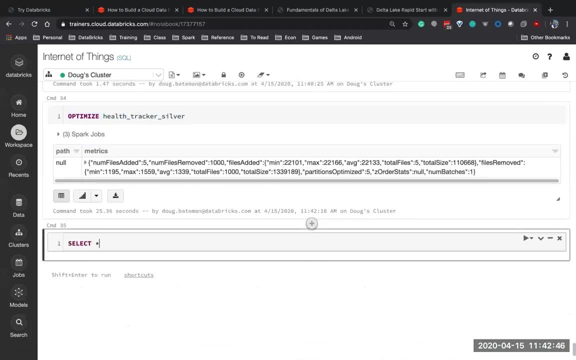 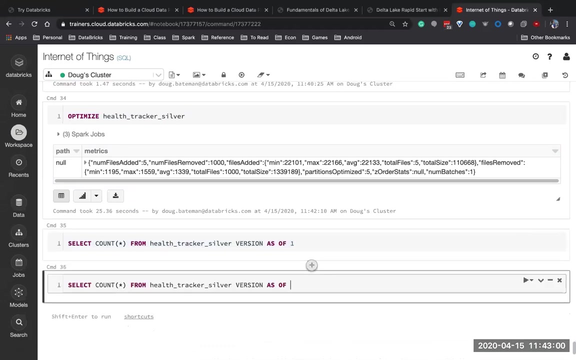 speeding up queries. I wish I had done a query before I optimized. actually, there's a way to do that. let's do select, select max star or count star from health tracker zero version as of one and compare it as of our latest version two. I just want to show you the performance difference I get by optimizing the table. 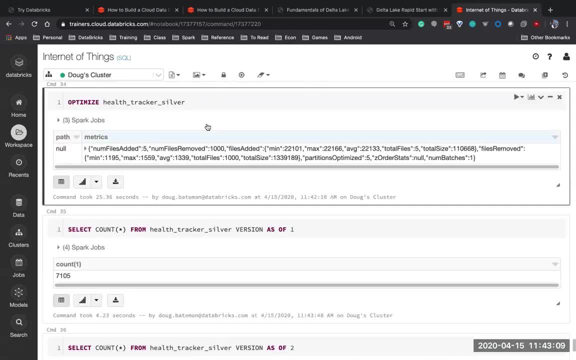 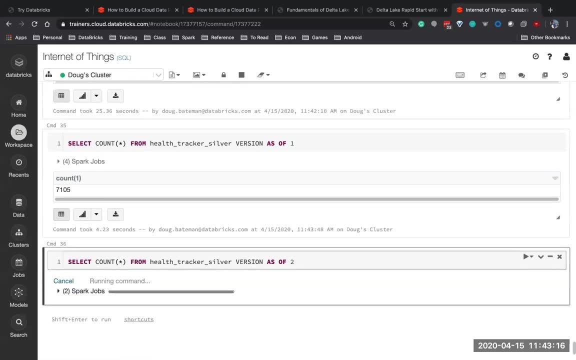 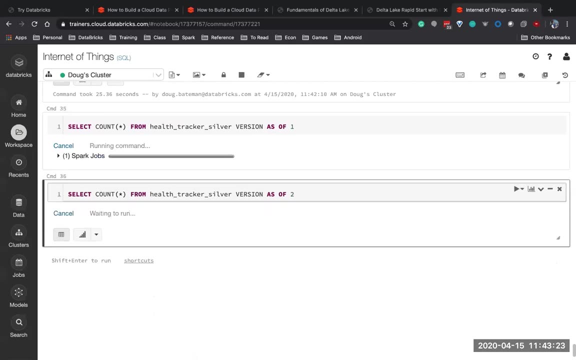 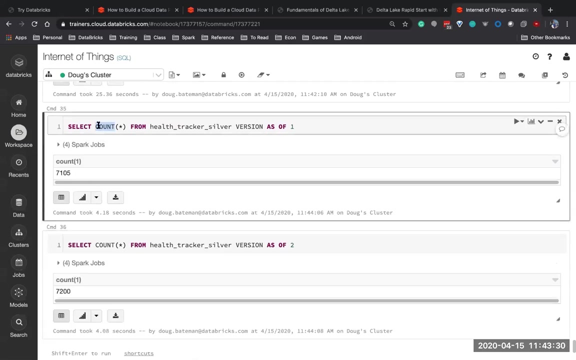 because I don't want to read a thousand files. if I could get away with reading only one file, oh shoot. in this case, the query optimizer is cheating me, because what the query optimizer is able to do is get the counts from the metadata, and it's not even looking at the data on disk. so 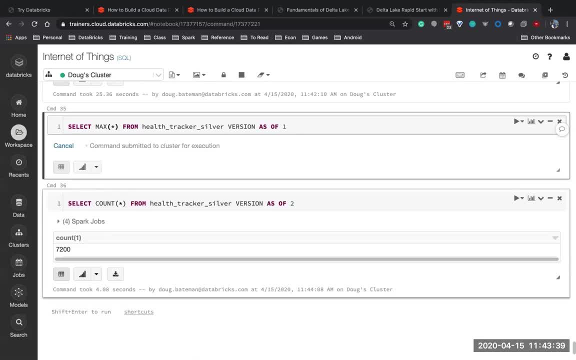 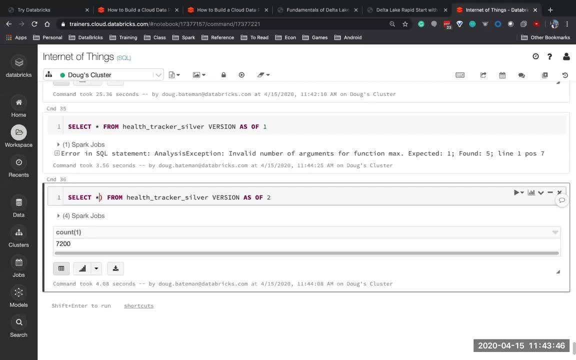 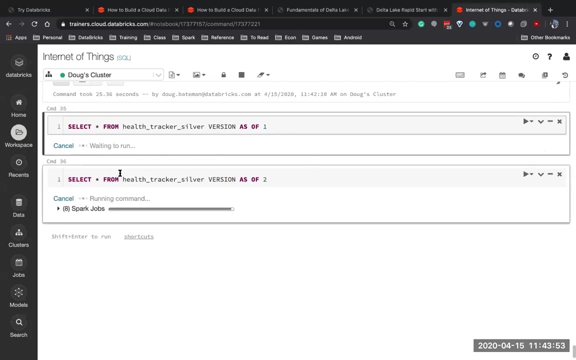 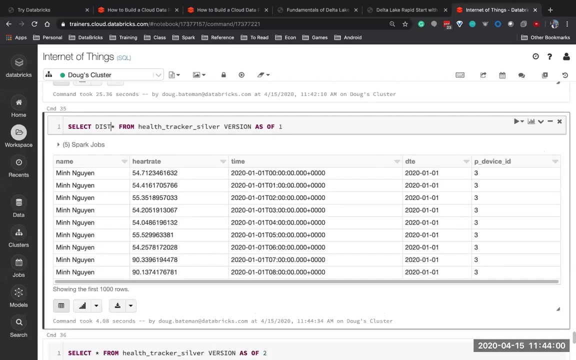 let's do this instead. let's just do a select star on both of these. oh, I know what I could do to make it touch all the data. I could throw in a distinct. I want to keep the query optimizer from being able to be too smart because I want to show the performance. 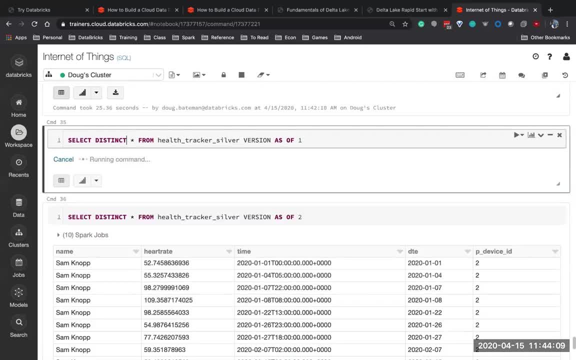 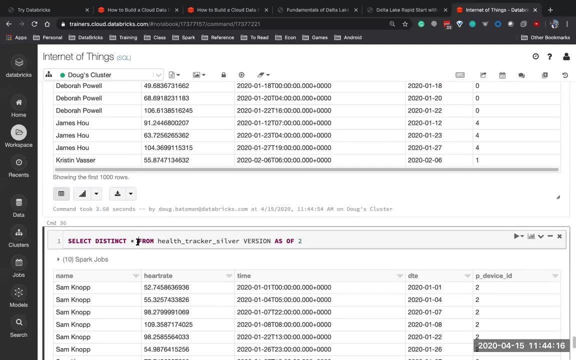 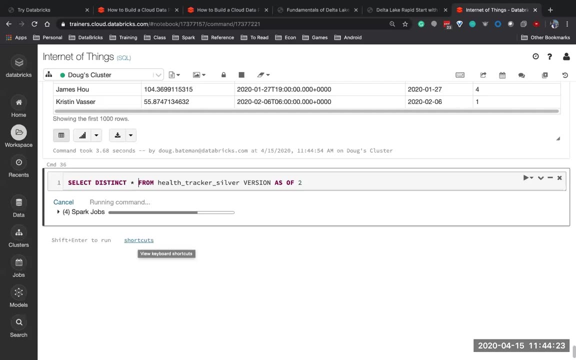 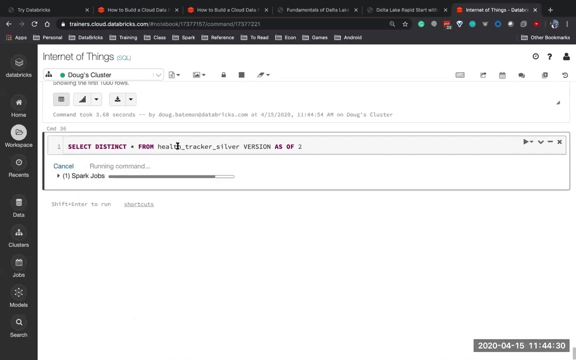 difference. so if I do a distinct it's going to actually have to read all the data. so version one, doing a distinct operation, took three point six, eight seconds. version two, with fewer files, let's see how long it takes. oh, it took longer. well, that made a liar out of me. maybe it's versions three and 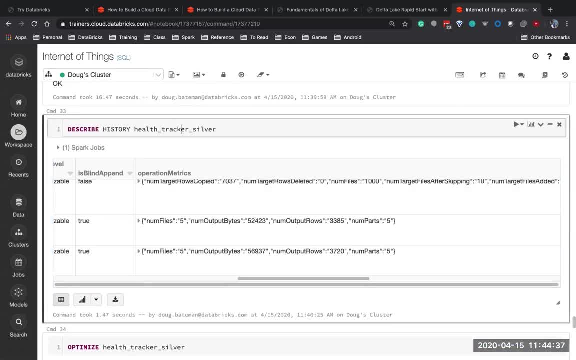 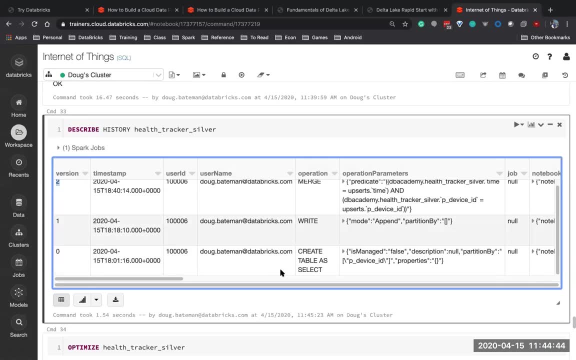 four. I bet you that's it. let's go back here. it's versions three and four. I want to be comparing our two and three. okay, it was versions two and three. version two was the merge, version three was the optimized. here we go. so I want to compare how long it takes to. 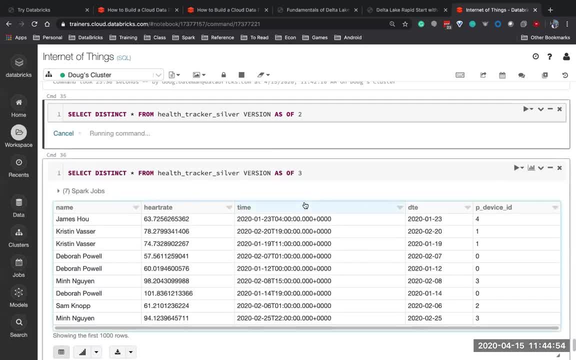 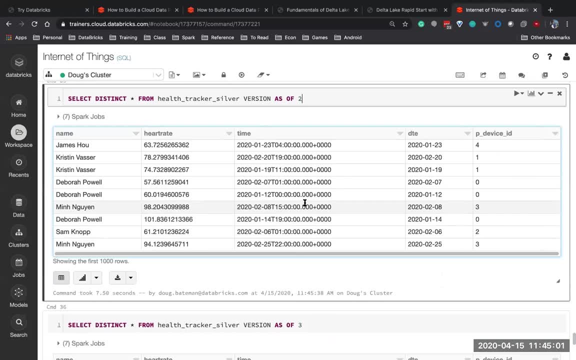 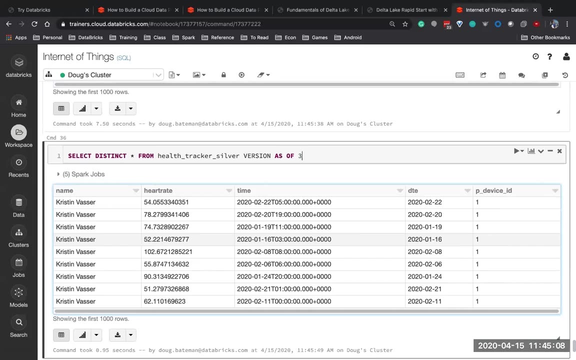 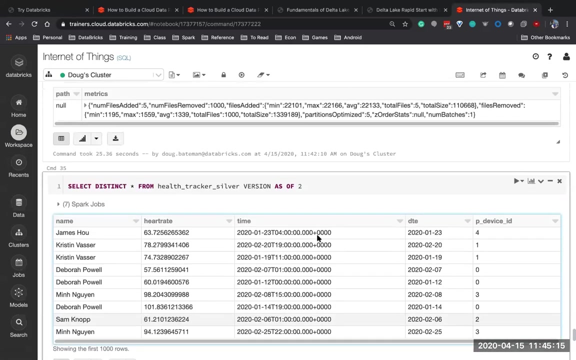 compare version two. it takes roughly six seconds to do version two. let's find out seven point five seconds, whereas our latest version, that's optimized, is a version two. it took point nine five seconds because what it did is it compressed all these small files into fewer big files. so often when we're 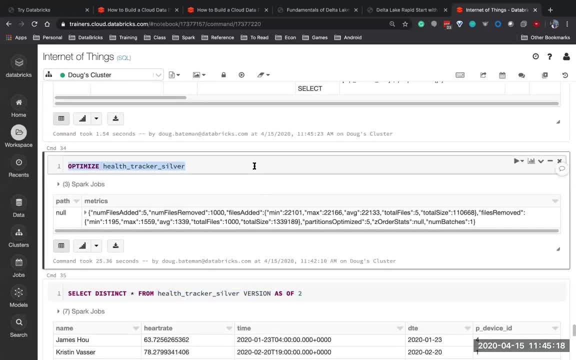 doing manipulations on our data sets, we end up with this file fragmentation problem, and the optimized command is part of Delta and it speeds up the performance by reducing the total number of the flans. now somebody asked why is an optimized just done automatically and why is it not optimized just done automatically? 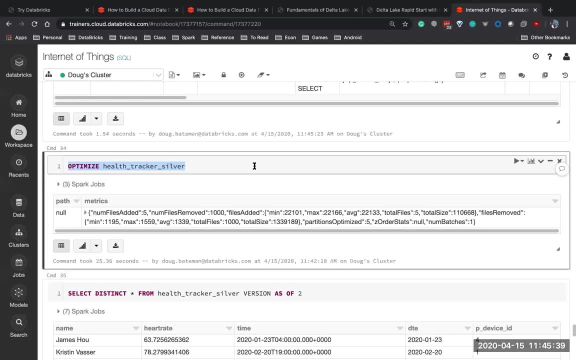 and it speeds up the performance by reducing the total number of the plans. now somebody asked: why isn't optimized just done automatically? now somebody asked: why isn't optimized just done automatically? now somebody asked: why isn't optimized just done automatically? there is, in fact, a way we can turn on. 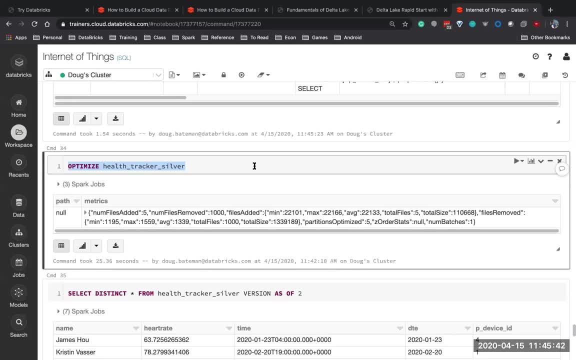 there is in fact a way we can turn on. there is in fact a way we can turn on: auto optimize in spark in this example. auto optimize in spark in this example. auto optimize in spark in this example. optimized was not enabled to be. optimized was not enabled to be. 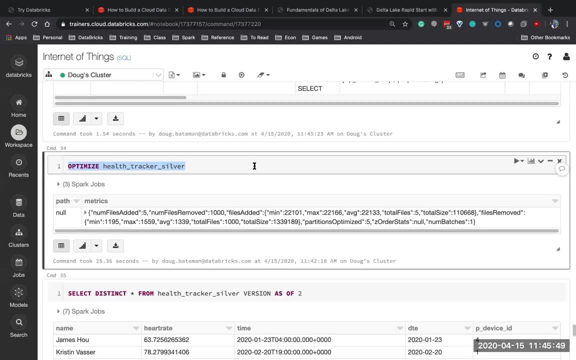 optimized was not enabled to be automatic. but there are some settings automatic. but there are some settings automatic. but there are some settings that we can configure there in the, that we can configure there in the, that we can configure there in the databricks- documentation- to turn on auto. 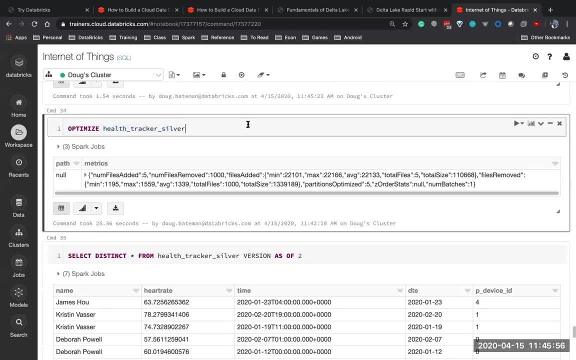 databricks documentation to turn on auto. databricks documentation to turn on auto optimize. the reason we don't do it optimize, the reason we don't do it optimize, the reason we don't do it automatically by default, is that the automatically by default is that the automatically by default is that the optimization command itself. you notice. 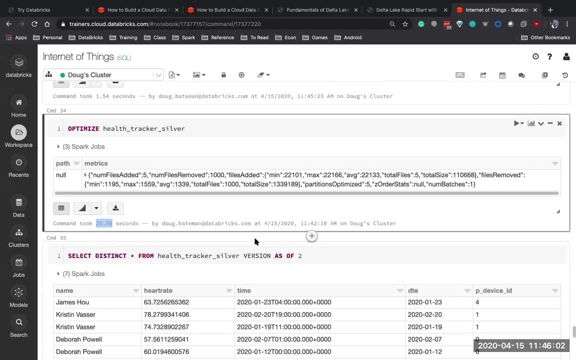 optimization command itself. you notice optimization command itself. you notice, took 25 seconds to run. took 25 seconds to run. took 25 seconds to run. it took 25 seconds to run. so it took 25 seconds to run. so it took 25 seconds to run. so you have to decide how frequently you 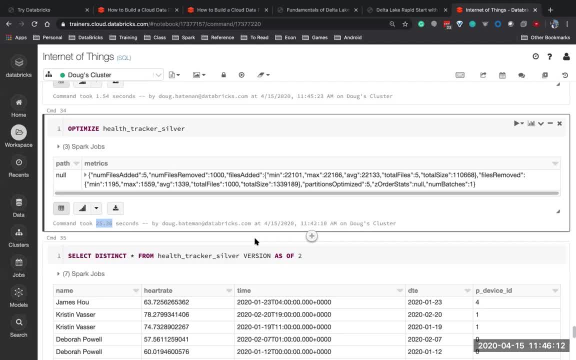 you have to decide how frequently you you have to decide how frequently you want to optimize, want to optimize, want to optimize, and there are ways you can configure and there are ways you can configure and there are ways you can configure databricks to do it for you. 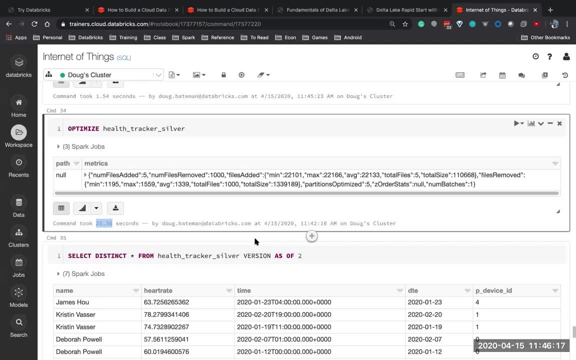 databricks to do it for you. databricks to do it for you whenever it thinks it's time to optimize, whenever it thinks it's time to optimize, whenever it thinks it's time to optimize. but the optimization step will take time. but the optimization step will take time. 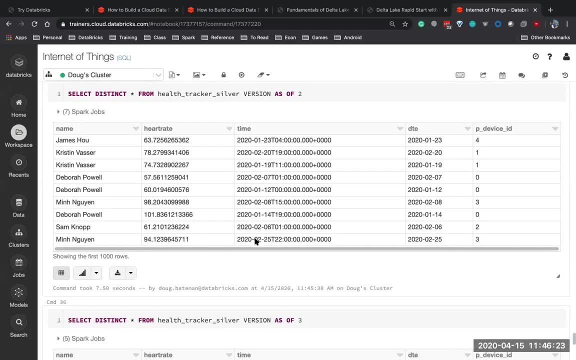 but the optimization step will take time, but once it's optimized your queries, but once it's optimized your queries, but once it's optimized, your queries will be a lot faster, will be a lot faster, will be a lot faster, which is really really nice. and now, jesse, 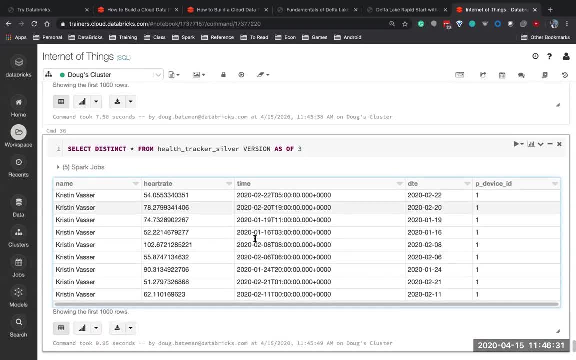 which is really really nice. and now jesse, which is really really nice. and now jesse asked a good question. he said: did it asked a good question? he said: did it asked a good question? he said: did it leave the old files in place and the? leave the old files in place and the? 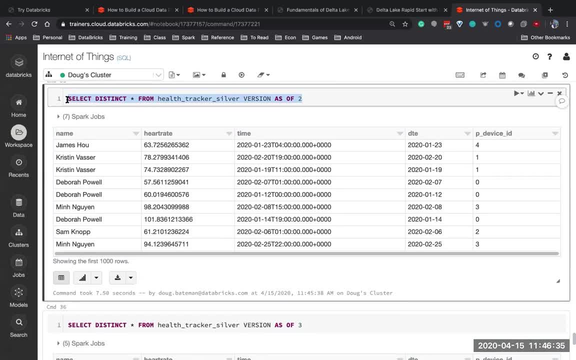 leave the old files in place. and the answer is yes. answer is yes. answer is yes. that's why i was able to query the old. that's why i was able to query the old. that's why i was able to query the old version, version, version and query the new version. 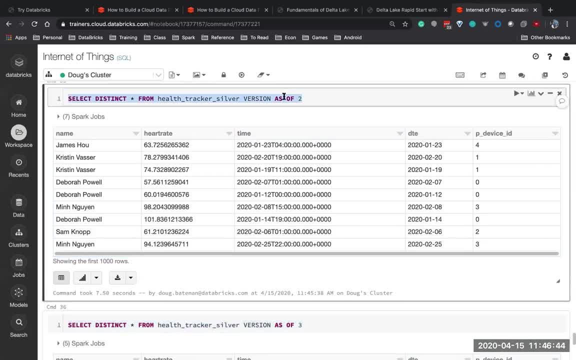 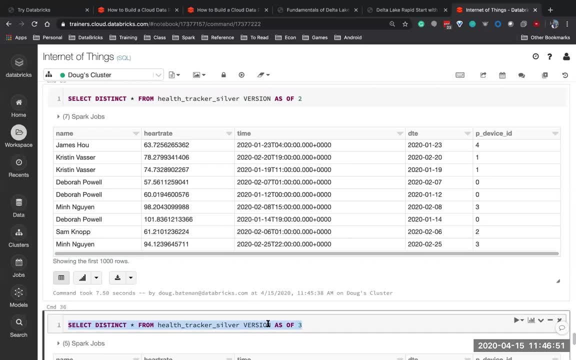 and query the new version. and query the new version. the old files are still there and i can. the old files are still there and i can. the old files are still there and i can. the reason we do that, the reason we do that, the reason we do that, is because you don't want to just delete. 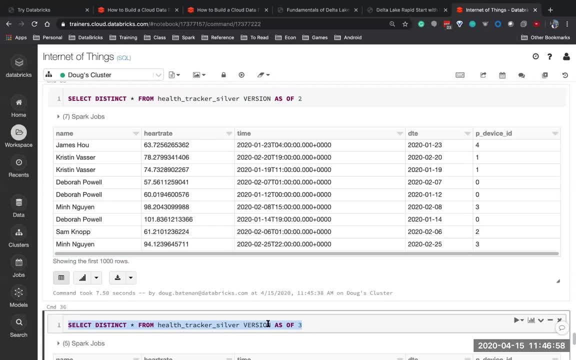 is because you don't want to just delete, is because you don't want to just delete the old files on disk, while other the old files on disk, while other the old files on disk. while other people may have a job running that needs, people may have a job running that needs. 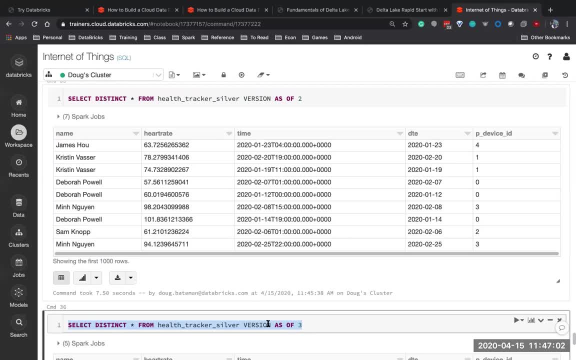 people may have a job running that needs them, them them. so, by default, databricks is not going to so, by default, databricks is not going to. so, by default, databricks is not going to allow you to delete, allow you to delete, allow you to delete those unoptimized files for at least a 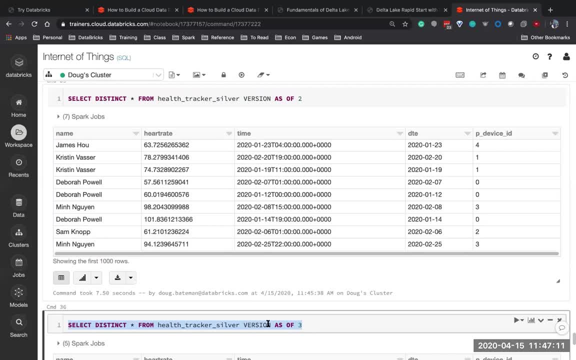 those unoptimized files for at least a those unoptimized files for at least a week, week week: we want to leave them around for a week. we want to leave them around for a week. we want to leave them around for a week to make sure that any queries that are 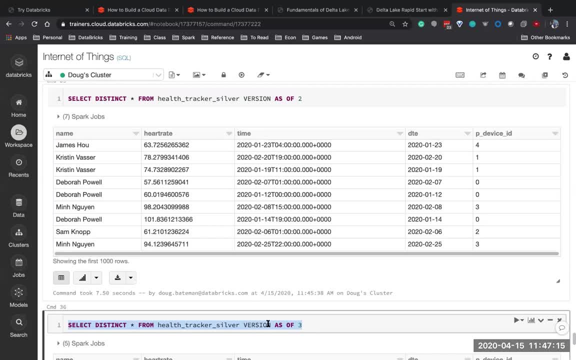 to make sure that any queries that are to make sure that any queries that are still running, still running, still running, still have access to the old files and still have access to the old files and still have access to the old files. and then then then there's a command we can run later. 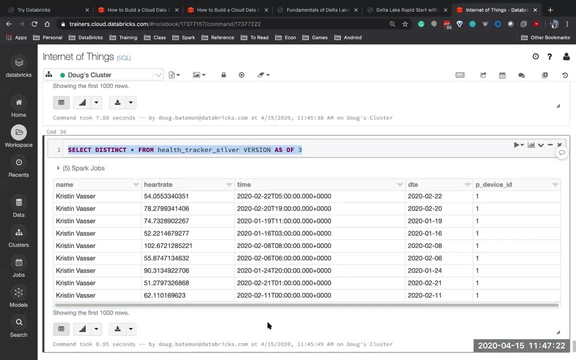 there's a command we can run later. there's a command we can run later called vacuum, called vacuum, called vacuum. that will delete the files after a. that will delete the files after a. that will delete the files after a certain amount of time has passed, and certain amount of time has passed. and. 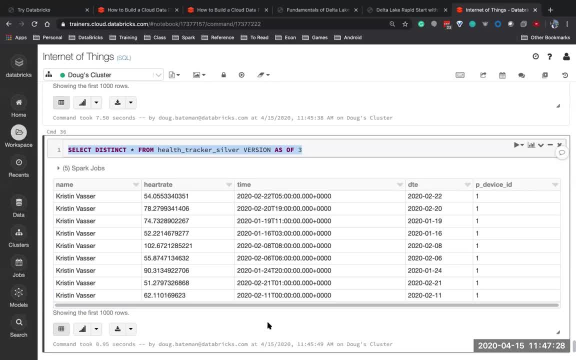 certain amount of time has passed, and that's actually going to come up in our. that's actually going to come up in our. that's actually going to come up in our course, course, course. so i jumped ahead a little bit because i. so i jumped ahead a little bit because i. 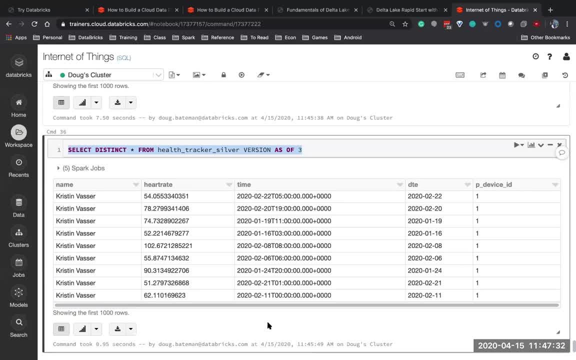 so i jumped ahead a little bit because i just didn't like seeing a thousand files, just didn't like seeing a thousand files, just didn't like seeing a thousand files. we actually teach optimize and vacuum. we actually teach optimize and vacuum. we actually teach optimize and vacuum further downstream, and i just moved it. 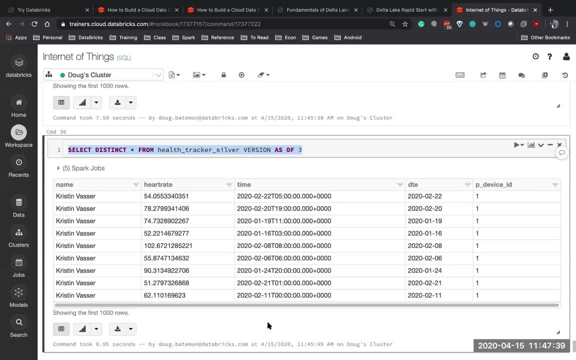 further downstream and i just moved it further downstream and i just moved it up ahead a little bit. now we are going to run out of time very now. we are going to run out of time very now. we are going to run out of time very soon and i wanted to be a little bit. 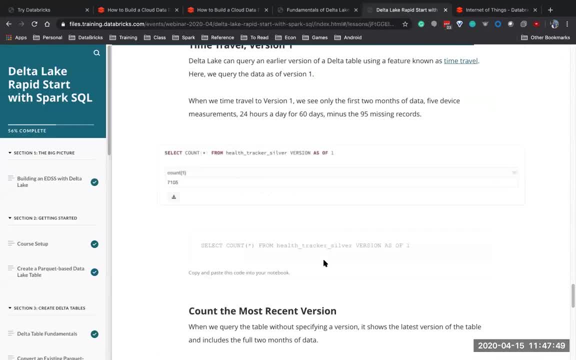 soon, and i wanted to be a little bit soon, and i wanted to be a little bit further ahead than we are now, further ahead than we are now, further ahead than we are now, let's see. so we just did the upsert. let's see, so we just did the upsert. 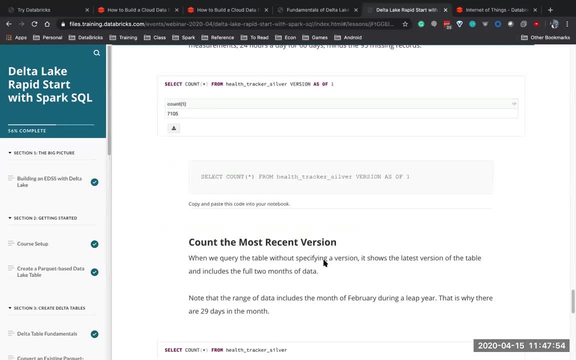 let's see. so we just did the upsert. we saw now that we could do counts, and we saw now that we could do counts, and we saw now that we could do counts and we could do time travel, we could do time travel, we could do time travel. so let's see, here, let's do the count. 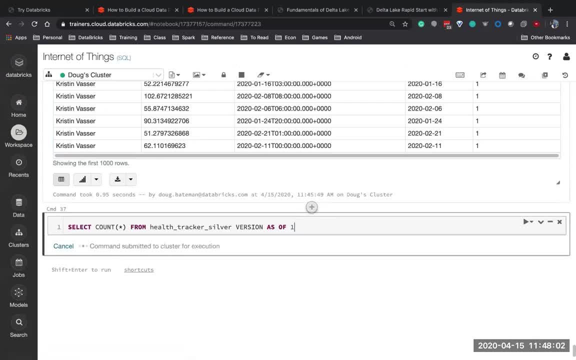 so let's see here, let's do the count. so let's see here, let's do the count of the number of rows before we did the, of the number of rows before we did the, of the number of rows before we did the upsert, upsert. 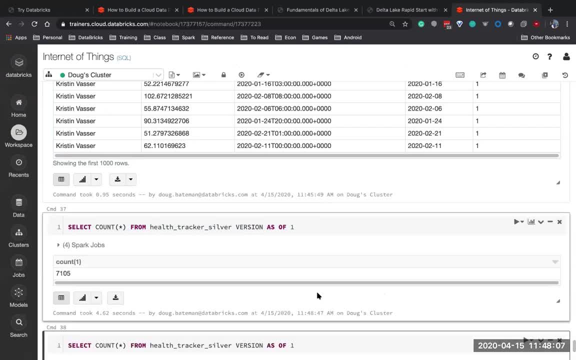 upsert and compare that to the number of rows and compare that to the number of rows and compare that to the number of rows in the latest version of the data, in the latest version of the data, just to see that we did in fact repair. just to see that we did in fact repair. 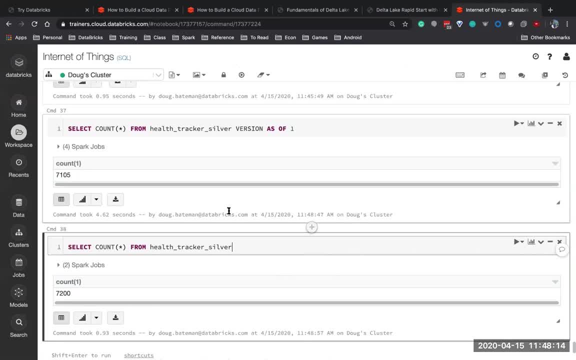 just to see that we did in fact repair our table, our table, our table. there we go. i have new rows added: 85 new. there we go. i have new rows added: 85 new- there we go. i have new rows added: 85 new rows. and 65 broken rows were also fixed. 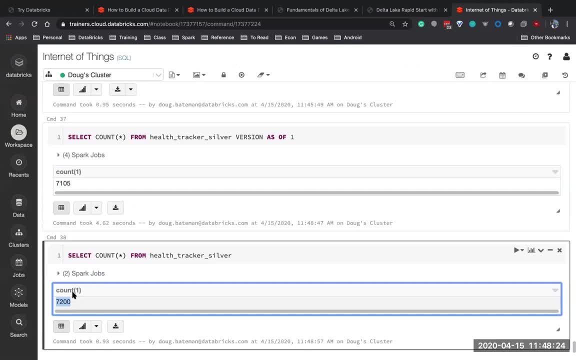 rows and 65 broken rows were also fixed. rows and 65 broken rows were also fixed, which is really cool. that's the merge command. that's what that's the merge command. that's what that's the merge command. that's what allows us to do these updates in an 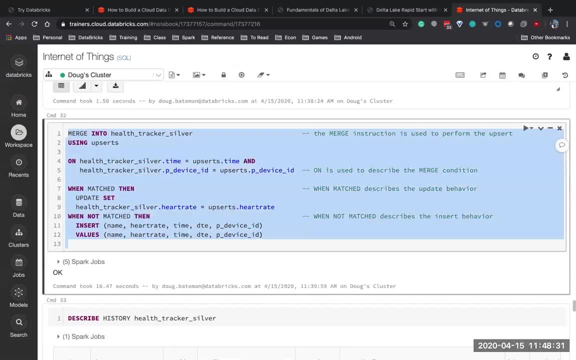 allows us to do these updates in an allows us to do these updates in an efficient format. efficient format, efficient format. the reason we want to use the merge, the reason we want to use the merge, the reason we want to use the merge command, is because we don't want to run. 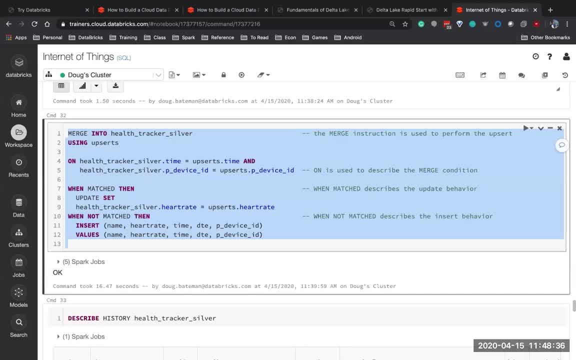 command is because we don't want to run command is because we don't want to run. a single update, a single update, a single update, line by line by line. that would be very line by line by line. that would be very line by line by line. that would be very row we want to do. 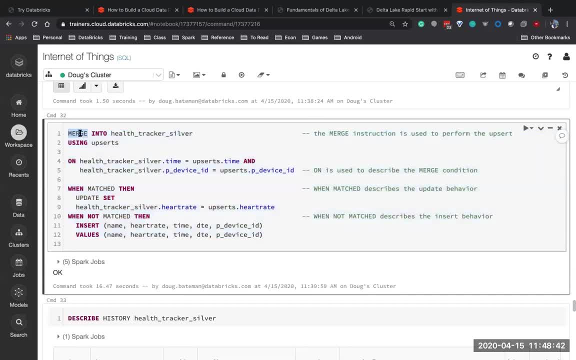 row. we want to do row, we want to do batch updates, and that's where the merge batch updates and that's where the merge batch updates and that's where the merge command, command, command kicks in and is incredibly powerful. all right, let's see if we're at a good 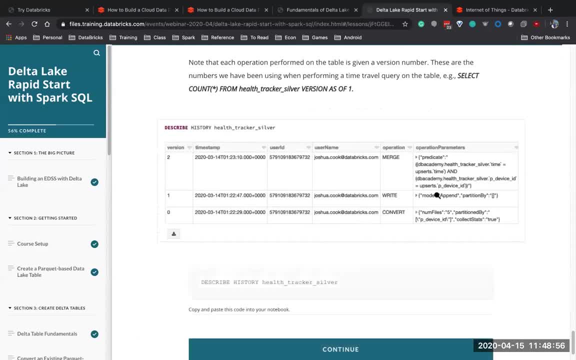 all right, let's see if we're at a good. all right, let's see if we're at a good stopping point, stopping point, stopping point. yep, i showed you describing the history. yep, i showed you describing the history. yep, i showed you describing the history of the table already. 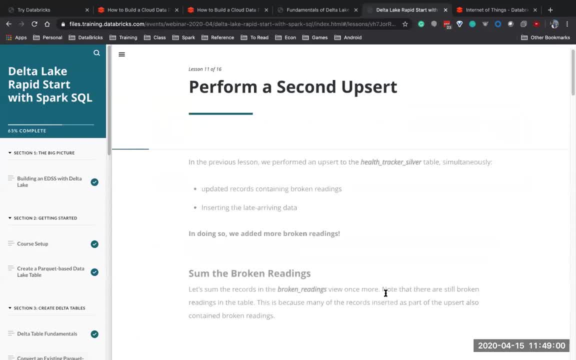 of the table already, of the table already. so you're able to see the history, and so you're able to see the history, and so you're able to see the history and the merge and the optimization, the merge and the optimization, the merge and the optimization. um, we can do an additional upsert next. 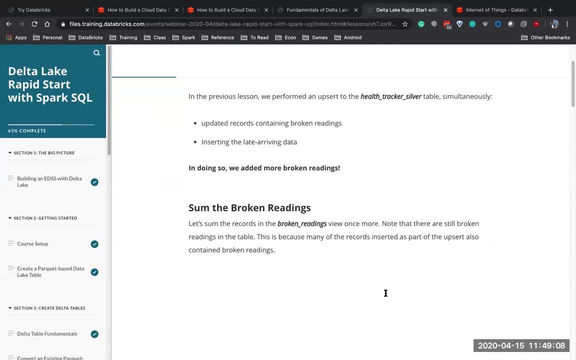 um, we can do an additional upsert next. um, we can do an additional upsert next to deal with broken readings. to deal with broken readings, to deal with broken readings. i'm going to save that for i believe. i'm going to save that for i believe. 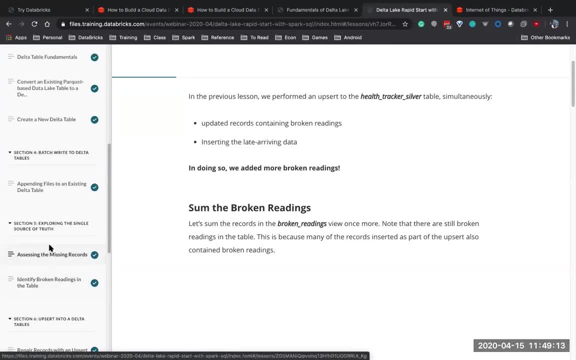 i'm going to save that for, i believe, the next course. let's see here. the next course. let's see here, the next course, let's see here. um, we still have to deal with, um, we still have to deal with, um, we still have to deal with. where are we um? 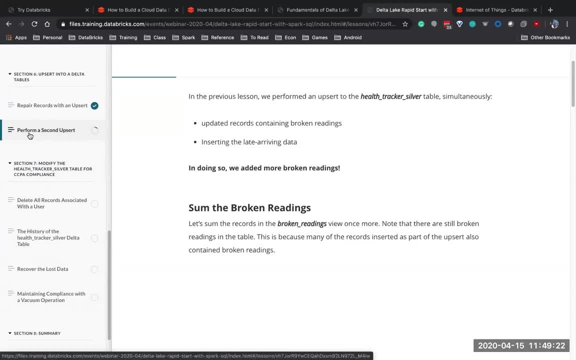 where are we um? where are we um? oh good, we are pretty much on schedule. oh good, we are pretty much on schedule. oh good, we are pretty much on schedule. um, we will do the second insert as a um. we will do the second insert as a um. we will do the second insert as a review in the next session. 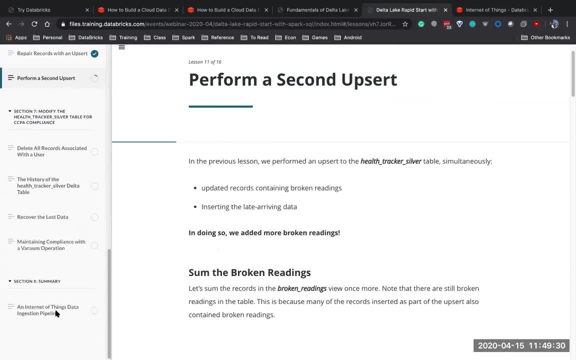 review in the next session. review in the next session, and then we will deal with deleting old, and then we will deal with deleting old, and then we will deal with deleting old records. we'll talk about optimizing records, we'll talk about optimizing records, we'll talk about optimizing and we'll talk about gdbr compliance. 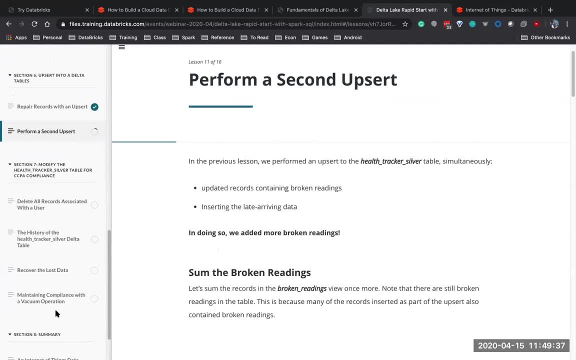 and we'll talk about gdbr compliance, and we'll talk about gdbr compliance and streaming and streaming and streaming in the next session, um so in the next session, um so in the next session, um. so i'm going to leave this last upsert for i'm going to leave this last upsert for. 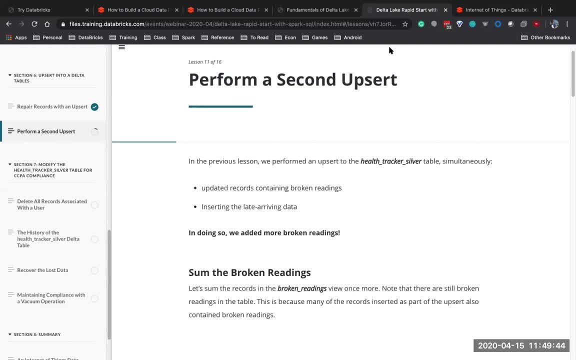 i'm going to leave this last upsert for next session, next session, next session, because it'll serve as a good review of, because it'll serve as a good review of, because it'll serve as a good review of doing upsets, doing upsets, doing upsets. um, in the meantime, you guys again, 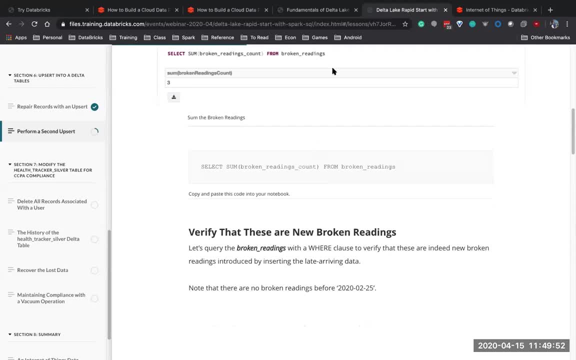 um in the meantime, you guys again. um in the meantime, you guys again. remember the link? it was tinyurlcom. remember the link? it was tinyurlcom. remember the link? it was tinyurlcom slash. let's see, i'm gonna scroll up on slash. let's see, i'm gonna scroll up on. 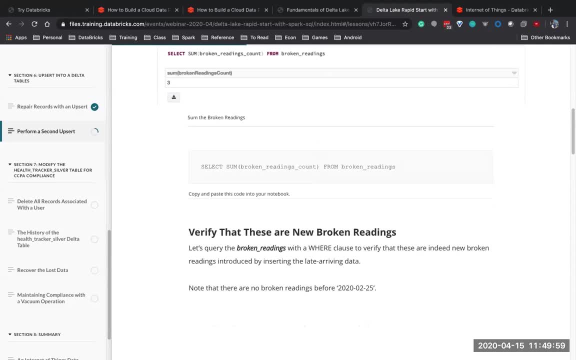 slash. let's see, i'm gonna scroll up on our chat history and grab it- our chat history- and grab it our chat history and grab it: tinyurlcom slash cloud dash data. tinyurlcom slash cloud dash data. tinyurlcom slash cloud dash data dash platform. let me go back in our 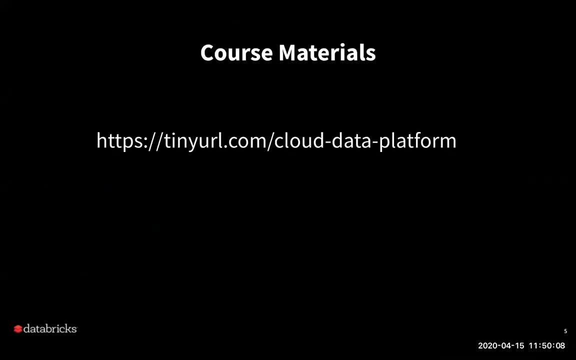 dash platform. let me go back in our dash platform. let me go back in our slides again. tinyurlcom slash cloud slides again. tinyurlcom slash cloud slides again. tinyurlcom slash cloud dash data, dash platform. dash data, dash platform. dash data, dash platform. and at this point i would like to take: 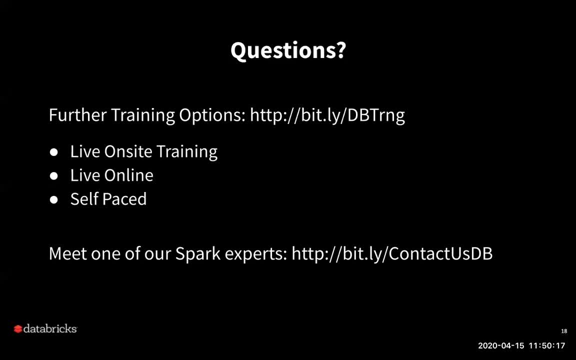 and at this point i would like to take- and at this point i would like to take some q a, some q a, some q a and questions and remember there's lots and questions and remember there's lots and questions and remember there's lots more training available on the databricks. 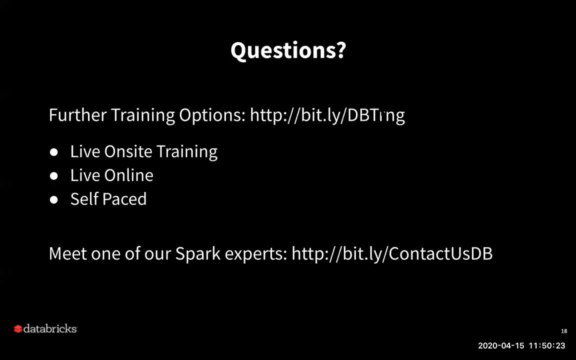 more training available on the databricks. more training available on the databricks website: website, website. here's a short link to the databricks. here's a short link to the databricks. here's a short link to the databricks website or academydatabrickscom website or academydatabrickscom. 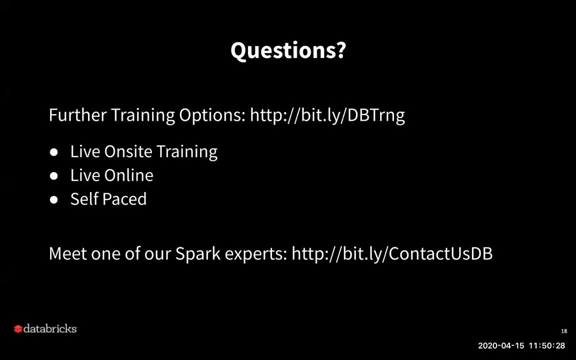 website or academydatabrickscom. we have live online training that you. we have live online training that you. we have live online training that you can take, can take, can take. you can even register for a three, or you can even register for a three, or you can even register for a three or four day class. we have performance. 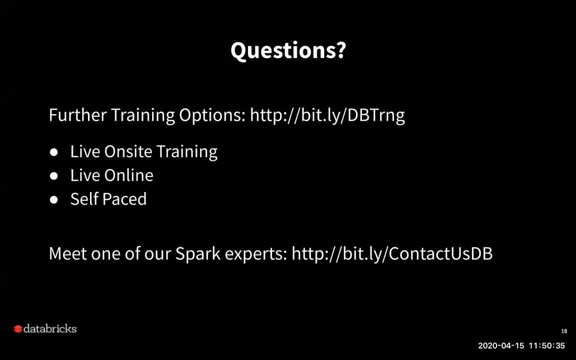 four day class: we have performance four day class: we have performance tuning classes that go tuning classes that go tuning classes that go deep into how spark works. i really love deep into how spark works. i really love deep into how spark works. i really love our performance tuning courses. 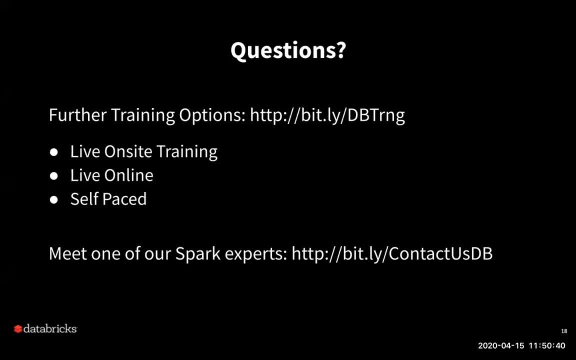 our performance tuning courses. our performance tuning courses. there's also some really good self-paced. there's also some really good self-paced. there's also some really good self-paced training for people just getting started. training for people just getting started. training for people just getting started. and if your company becomes a databricks, 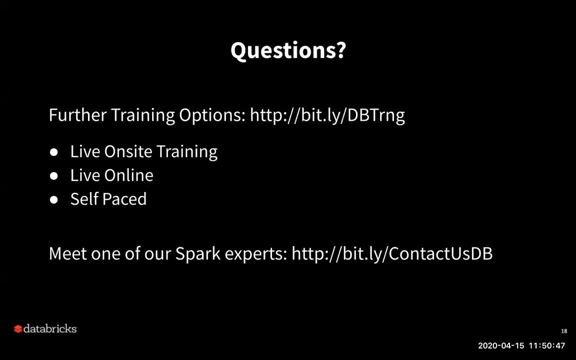 and if your company becomes a databricks? and if your company becomes a databricks customer, customer, customer, we make that training available for free. we make that training available for free. we make that training available for free. otherwise, you can simply purchase the. otherwise, you can simply purchase the. 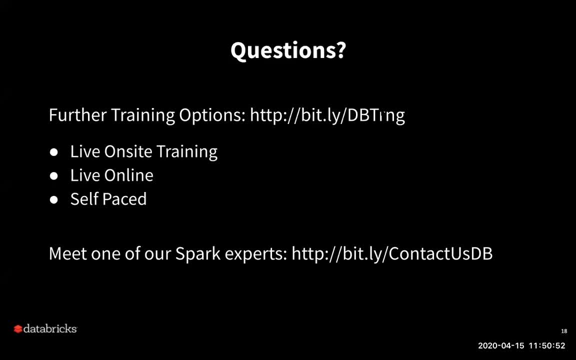 otherwise, you can simply purchase the courses, courses, courses on our website. um, if you'd like to talk on our website? um, if you'd like to talk on our website? um, if you'd like to talk to somebody at databricks, to somebody at databricks, to somebody at databricks, feel free to go to this link. bitly dot, or. 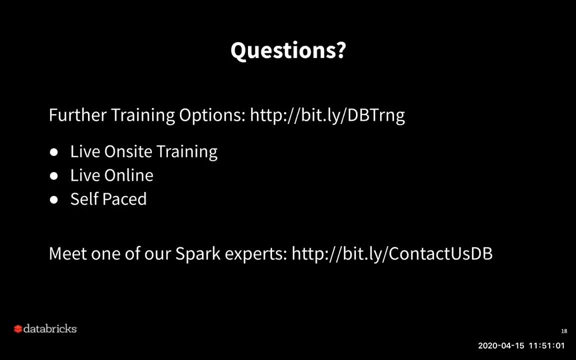 feel free to go to this link bitly dot. or feel free to go to this link bitly dot or bitly slash, bitly slash, bitly dot or bitly slash. contact us databricks or db. contact us databricks or db. contact us databricks or db and you could speak to one of our people. 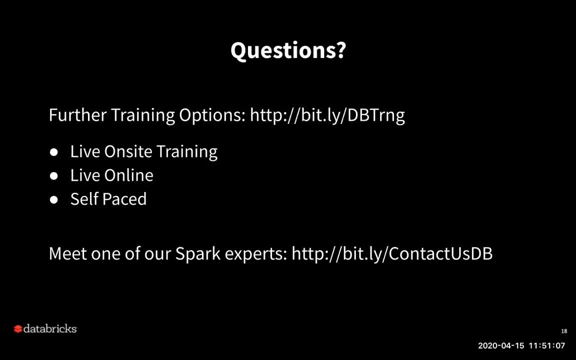 and you could speak to one of our people. and you could speak to one of our people about about, about using databricks or setting up a trial of using databricks, or setting up a trial of using databricks or setting up a trial of databricks for your company. 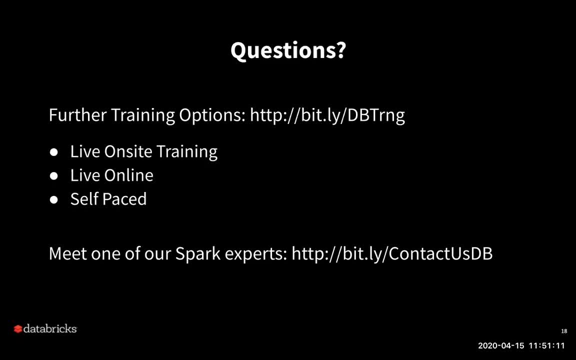 databricks for your company. databricks for your company. now i'm going to go ahead and answer some. now i'm going to go ahead and answer some. now i'm going to go ahead and answer some q a that people have, q a that people have, q a that people have. let's see here, um. 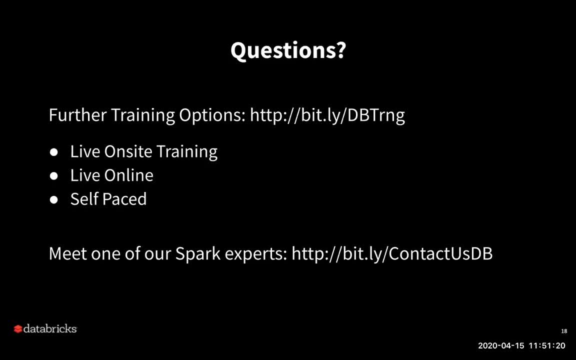 let's see here, um, let's see here, um, there's one question about azure data. there's one question about azure data. there's one question about azure data. factory, that's a little bit out of scope. factory, that's a little bit out of scope. factory, that's a little bit out of scope. so, daryl, what i'm going to suggest is: 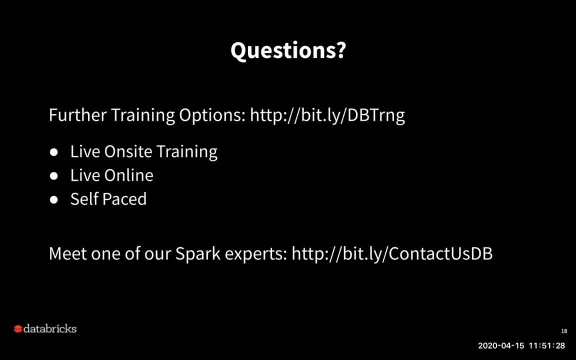 so, daryl, what i'm going to suggest is. so, daryl, what i'm going to suggest is that that that either have you reach out to support, or either have you reach out to support, or either have you reach out to support or, uh, follow up offline for that question. 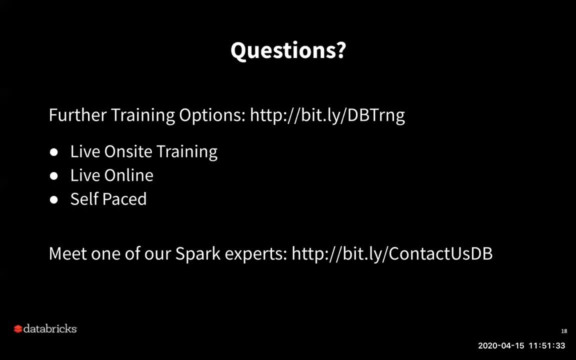 uh follow up offline for that question. uh follow up offline for that question. um, but really, if you were able to uh um, but really, if you were able to uh um, but really, if you were able to uh reach out to our support team, reach out to our support team. 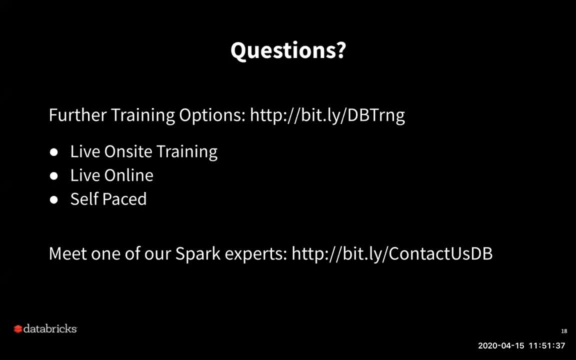 reach out to our support team. we should be able to help you a little. we should be able to help you a little. we should be able to help you a little bit with using delta as a sync for azure bit, with using delta as a sync for azure. 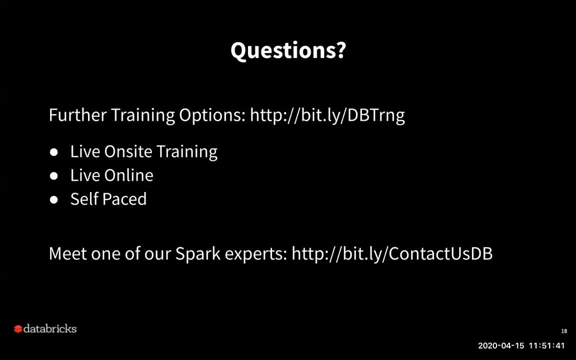 bit with using delta as a sync for azure data factory. we have built in some data factory. we have built in some data factory. we have built in some integrations, integrations, integrations, um. somebody else had asked: could i use? um. somebody else had asked: could i use. 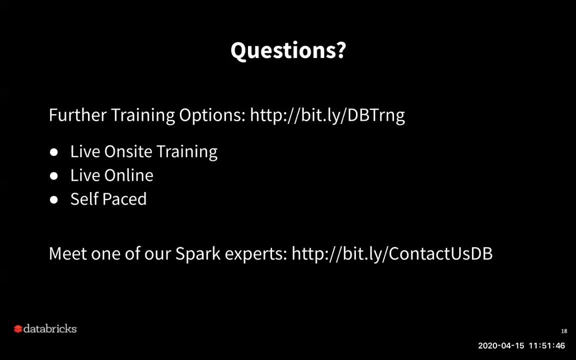 um. somebody else had asked: could i use delta with data factory, delta with data factory, delta with data factory: yes. can i use um delta with yes. can i use um delta with yes. can i use um delta with athena? the answer is yes, there is athena. the answer is yes, there is. 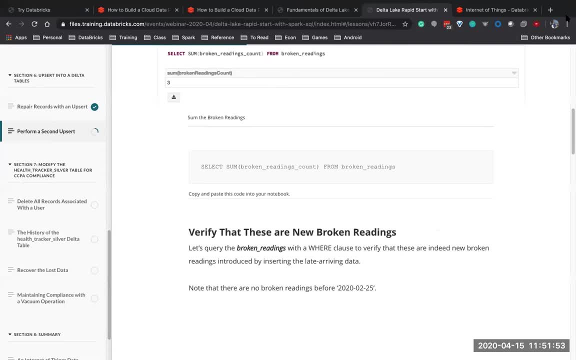 athena? the answer is yes, there is documentation for how to do these things. documentation for how to do these things, documentation for how to do these things on the databricks website. so if i search on the databricks website, so if i search on the databricks website, so if i search for athena or presto, for example, 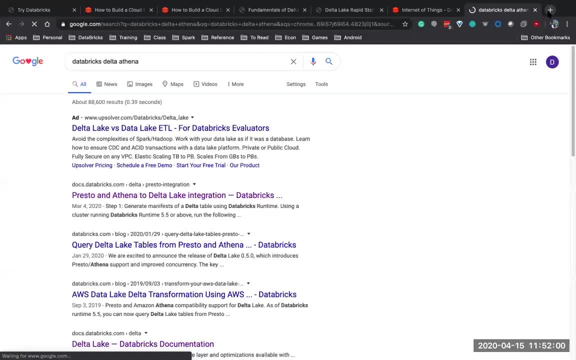 for athena or presto, for example, for athena or presto. for example, databricks, databricks, databricks. delta, athena, delta, athena, delta, athena. there we go, there is a link, presto, and there we go. there is a link, presto, and. 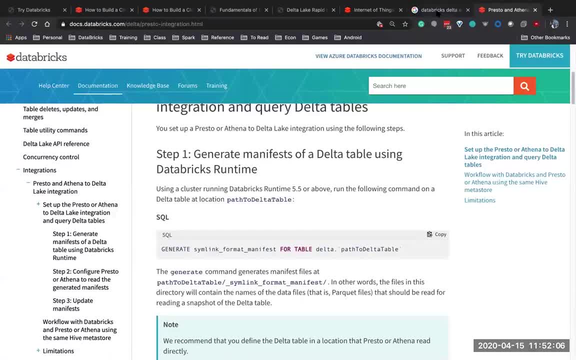 there we go. there is a link, presto, and athena delta lake integration and it athena delta lake integration and it athena delta lake integration, and it talks about how to do. it. talks about how to do. it talks about how to do it. let's do the same thing here instead of. 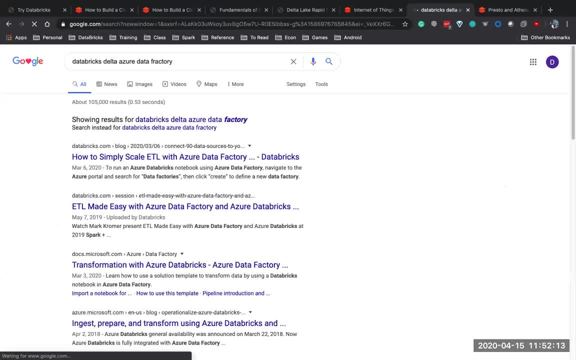 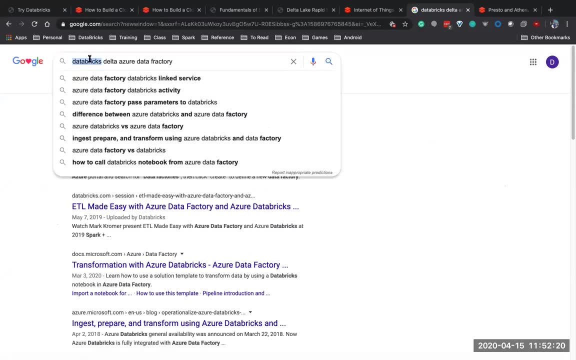 let's do the same thing here instead of. let's do the same thing here. instead of athena, let's use azure data factory athena. let's use azure data factory athena. let's use azure data factory um with delta, or is it with delta? 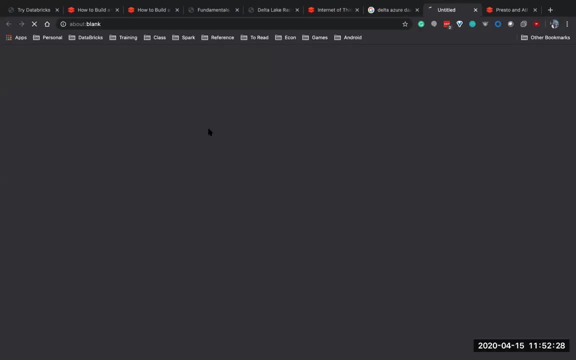 delta loading from database. using delta loading from database. using delta. loading from database. using watermark with azure data factory. watermark with azure data factory. watermark with azure data factory. let me search for the word delta and let me search for the word delta and let me search for the word delta, and there's a nice example article there for. 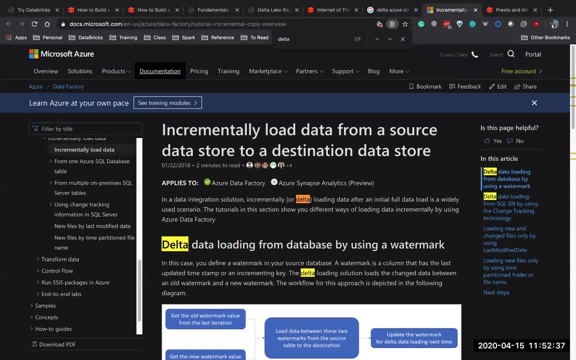 there's a nice example article there for there's a nice example article there for you, you, you, uh, let's take a look at some other. uh, let's take a look at some other. uh, let's take a look at some other questions in here. um, people want to know. 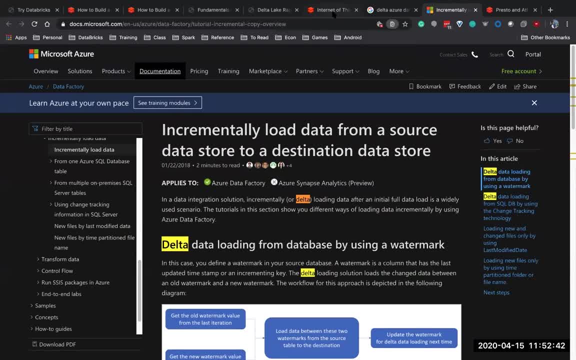 questions in here. um, people want to know questions in here. um, people want to know: where can you get this notebook? where can you get this notebook? where can you get this notebook for practice? and rather than distributing for practice, and rather than distributing for practice, and rather than distributing the notebook that i just wrote what i'm 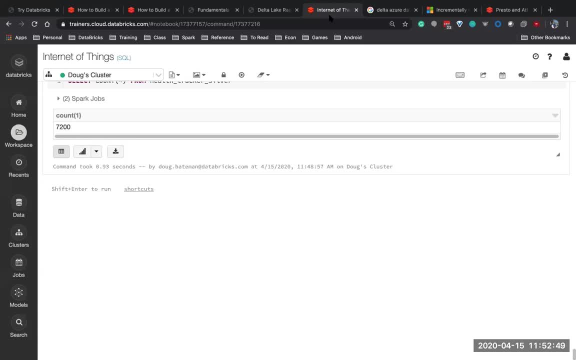 the notebook that i just wrote what i'm, the notebook that i just wrote, what i'm going to point you to, going to point you to, going to point you to, is that link again that we gave you? is that link again that we gave you? is that link again that we gave you here? 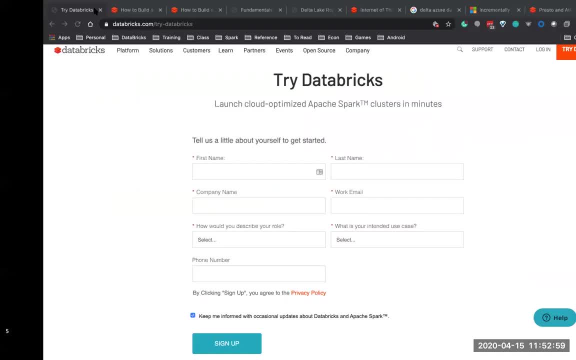 cloud dash data dash platform and that's cloud dash data dash platform and that's cloud dash data dash platform. and that's going to let you access the source, going to let you access the source, going to let you access the source materials that i was using, materials that i was using. 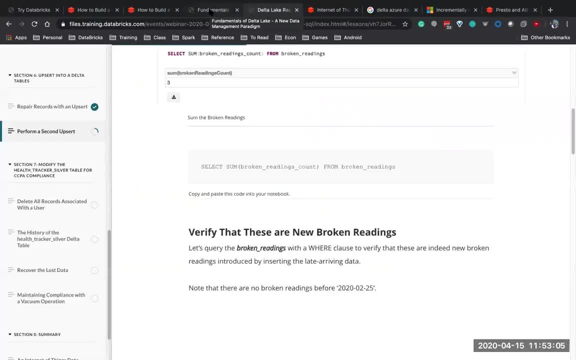 materials that i was using. so you'll be able to go through this on. so you'll be able to go through this on. so you'll be able to go through this on your own, your own, your own, and actually run it. i do think there's a. 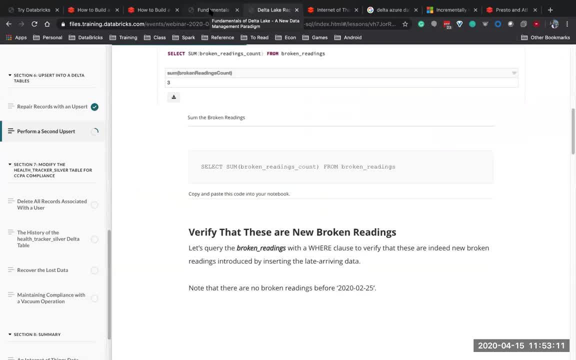 and actually run it. i do think there's a and actually run it. i do think there's a lot of value in having the instructor, lot of value in having the instructor, lot of value in having the instructor me here explaining what's going on and me here explaining what's going on, and 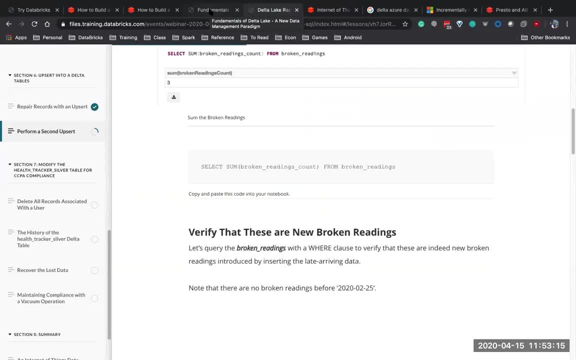 me here explaining what's going on and giving you that extra level of depth. giving you that extra level of depth, giving you that extra level of depth beyond this, as well as answering beyond this, as well as answering beyond this, as well as answering questions, questions, questions. but i really recommend people go and 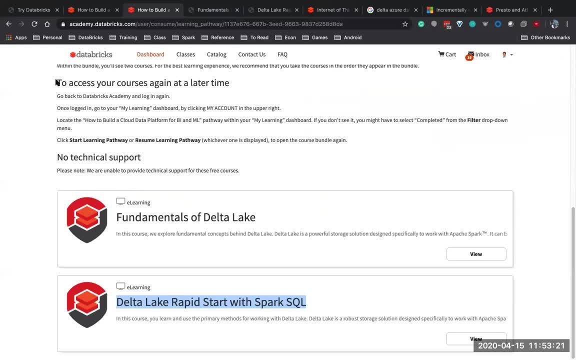 but i really recommend people go and but i really recommend people go and actually try this out yourselves. actually try this out yourselves. actually try this out yourselves. you're able to do it if you just come. you're able to do it if you just come. you're able to do it if you just come into the databricks academy link that i. 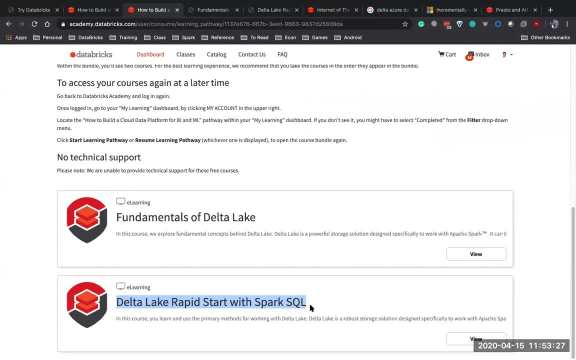 into the databricks academy link that i into the databricks academy link that i just gave you, just gave you, just gave you. and do the delta lake rapid start with and do the delta lake rapid start with and do the delta lake rapid start with spark sql. 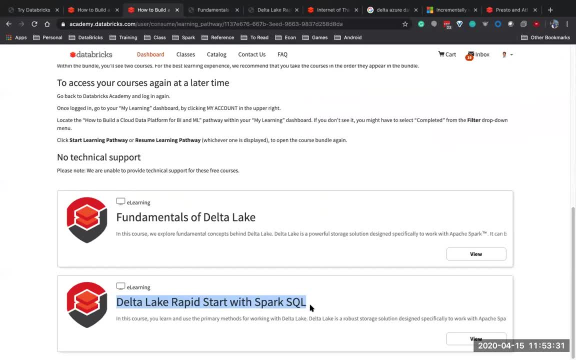 spark sql, spark sql. and for those of you who are interested, and for those of you who are interested, and for those of you who are interested in it with uh python or scala, they are in it with uh python or scala. they are in it with uh python or scala. they are working on a delta lake. rapid start in. 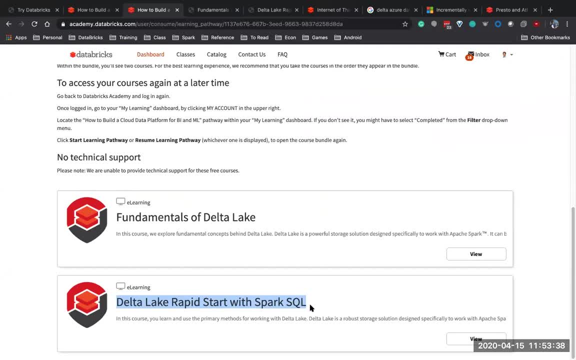 working on a delta lake rapid start in working on a delta lake rapid start in this other programming language, this other programming language, this other programming language. it's just not been released yet, but i it's just not been released yet. but i it's just not been released yet. but i think there's a lot of value in learning. 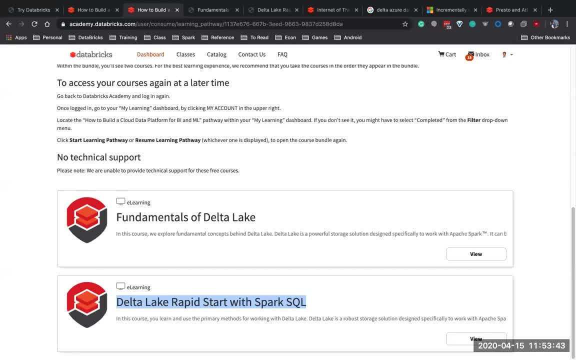 think there's a lot of value in learning, think there's a lot of value in learning how to do it with spark sql as well, and if you're watching this in a and if you're watching this in a and if you're watching this in a recording, check the website. 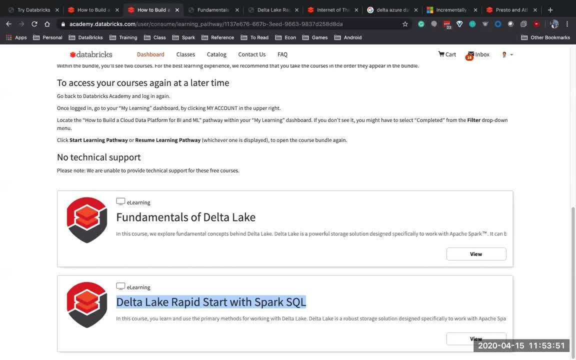 recording. check the website recording. check the website. those may at some point be released. those may at some point be released. those may at some point be released relatively soon. i know we plan to do relatively soon. i know we plan to do relatively soon. i know we plan to do that this quarter. 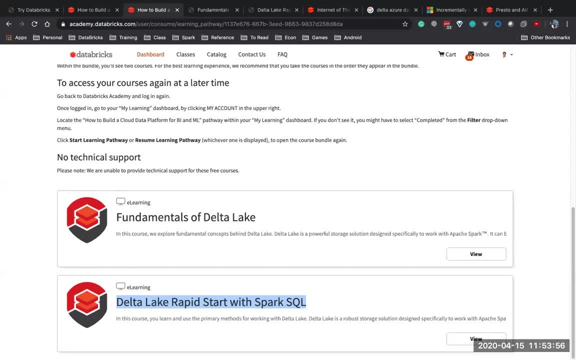 that this quarter, that this quarter, um does optimize have an impact on um? does optimize have an impact on um? does optimize have an impact on version history? was a question for version history. was a question for version history. was a question for rukward uh. farouk asked and the answer. rukward uh farouk asked and the answer rukward uh farouk asked and the answer to that we actually saw. if i show the to that we actually saw, if i show the to that we actually saw, if i show the history: history. 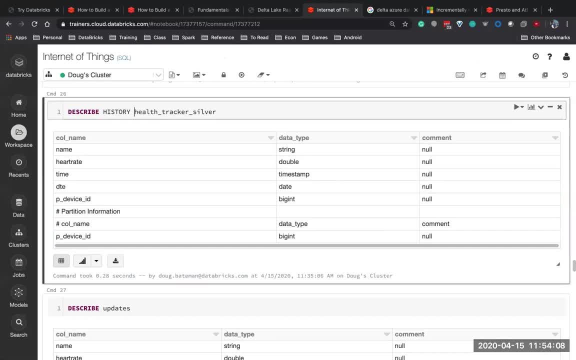 history. so if i do describe history, so if i do describe history, so if i do describe history, i am able to see a new version of the. i am able to see a new version of the. i am able to see a new version of the history, history. 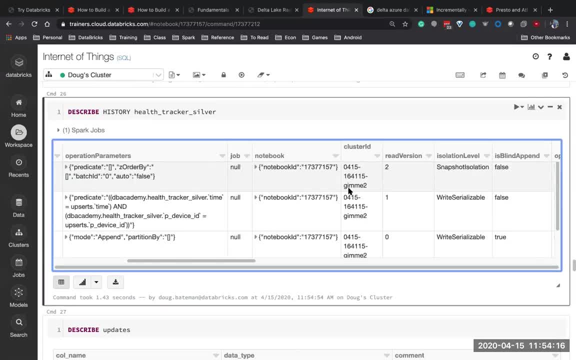 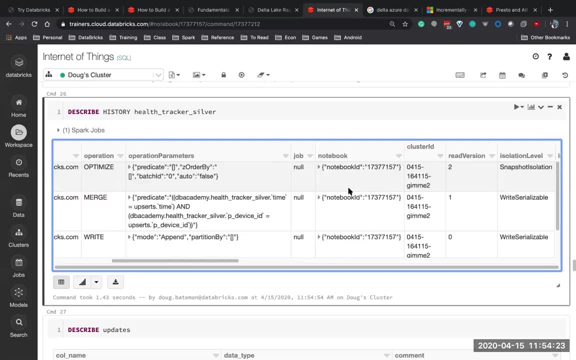 history show up in this history. but show up in this history. but show up in this history, but it's actually marked, it's actually marked. it's actually marked as. let's see if i could find it as. let's see if i could find it as. let's see if i could find it. well, you don't see it in here, but in. 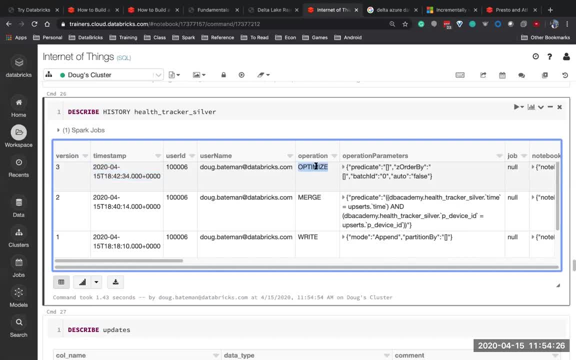 well, you don't see it in here, but in well, you don't see it in here, but in the metadata, the metadata, the metadata. it knows that the optimize command, it knows that the optimize command, it knows that the optimize command doesn't actually change data, it just 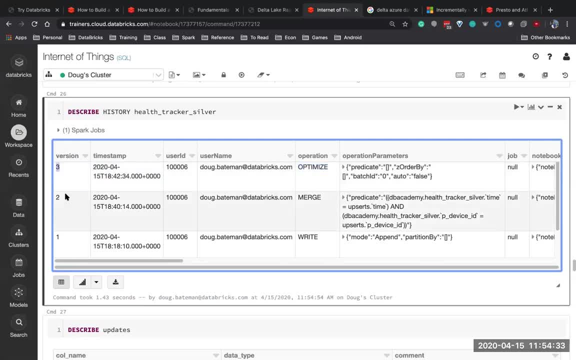 doesn't actually change data. it just doesn't actually change data. it just reorganizes it, reorganizes it, reorganizes it. so if i was to ask what's the difference? so if i was to ask what's the difference? so if i was to ask what's the difference between version 3 and version 2? 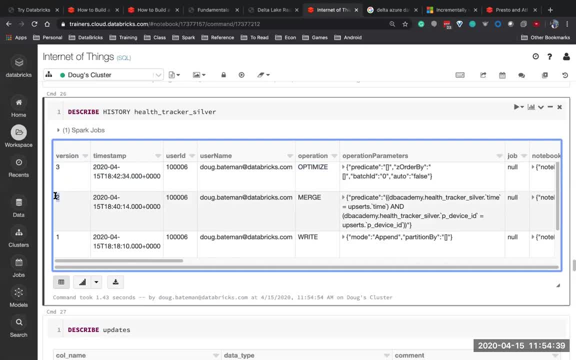 between version 3 and version 2, between version 3 and version 2. spark would immediately be able to figure. spark would immediately be able to figure. spark would immediately be able to figure out that there was no out, that there was no out, that there was no actual data changed. it was just a. 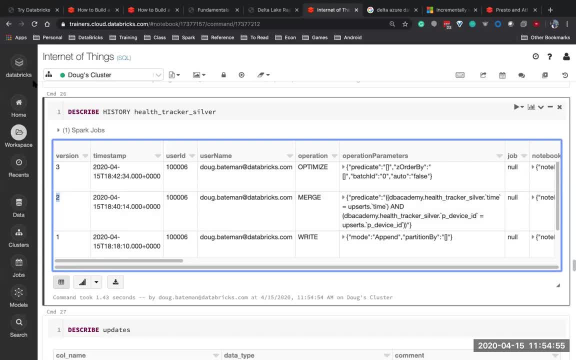 actual data changed. it was just a actual data changed. it was just a. and that's some of the metadata that's and that's some of the metadata that's and that's some of the metadata that's stored in that json file in the json log. stored in that json file in the json log. 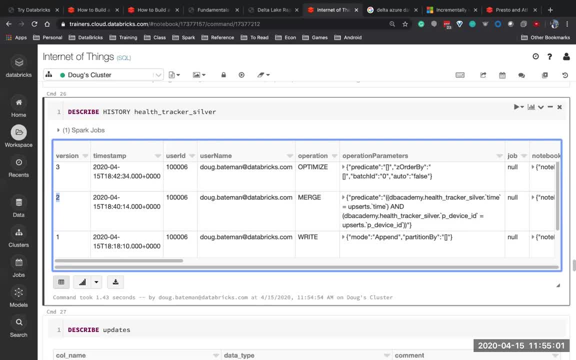 stored in that json file, in the json log: um, um, um. let's see here other questions that let's see here, other questions that let's see here, other questions that people ask, people ask. people ask um: are there any recommendations of? are there any recommendations of? are there any recommendations of optimization that databricks is? 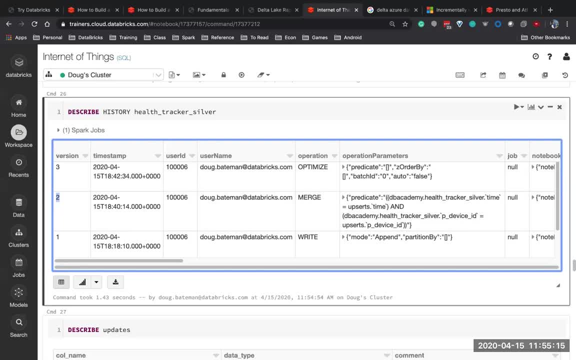 optimization that databricks is optimization that databricks is providing when we execute sql. rather providing when we execute sql, rather providing when we execute sql, rather than blindly providing the optimize, than blindly providing the optimize, than blindly providing the optimize command. so the optimize command is actually. so the optimize command is actually. 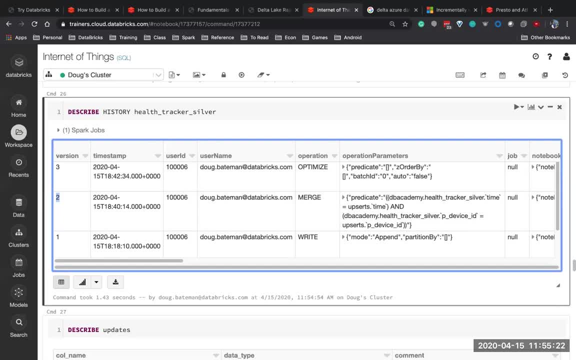 so the optimize command is actually really smart. its job is to combine small really smart. its job is to combine small really smart. its job is to combine small files into big files, files into big files, files into big files. if i was to run optimize twice, you'll. 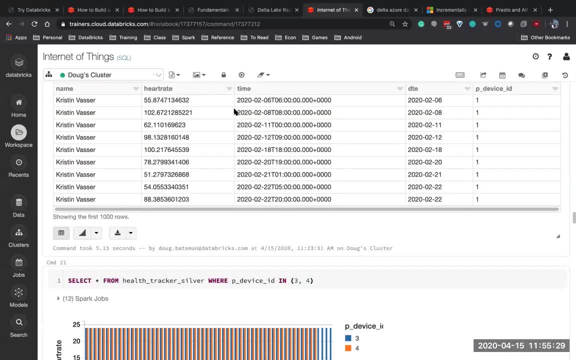 if i was to run, optimize twice, you'll. if i was to run optimize twice, you'll notice the second time i run, optimize, notice. the second time i run, optimize notice. the second time i run, optimize is actually going to be very fast, is actually going to be very fast. 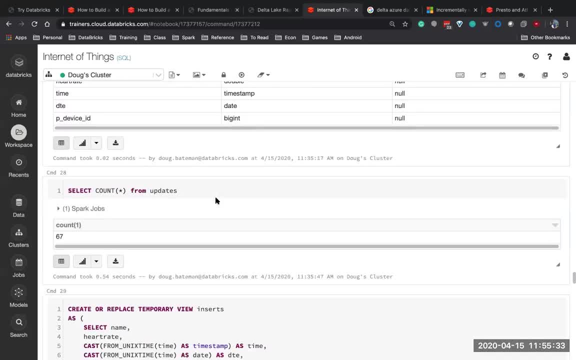 is actually going to be very fast because it's already got big files. so because it's already got big files, so because it's already got big files, so let me see if i could find where the. let me see if i could find where the. let me see if i could find where the optimize command was. 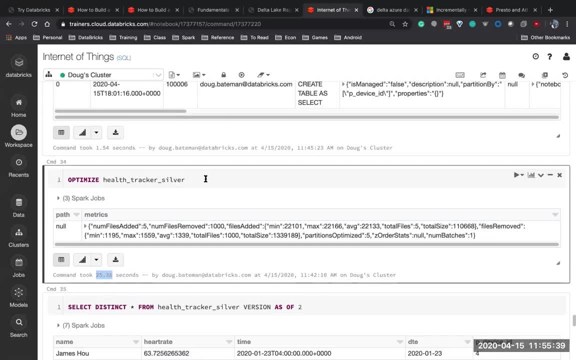 optimize command was. optimize command was there. it is so the first time i ran it there. it is so the first time i ran it there. it is so the first time i ran it. it took 25 seconds to combine small files. it took 25 seconds to combine small files. 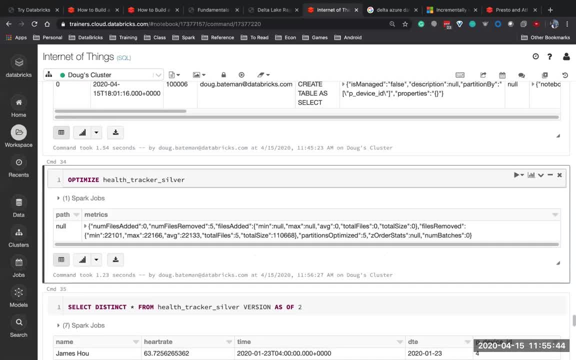 it took 25 seconds to combine small files of the big files of the big files of the big files. the second time i run it: boom one second. the second time i run it: boom one second. the second time i run it boom one second because it's determined it's already. 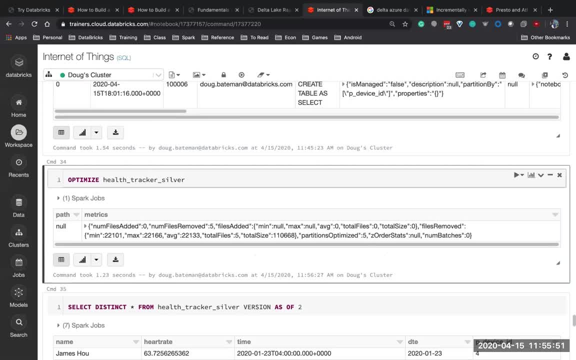 because it's determined, it's already. because it's determined, it's already optimized. i don't need to do it again. optimized. i don't need to do it again. optimized. i don't need to do it again. so typically, you're going to do optimize. so typically, you're going to do optimize. 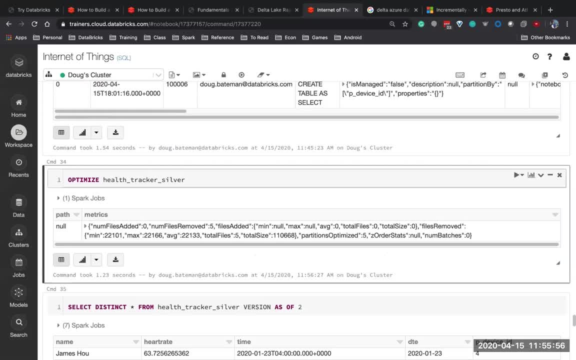 so typically you're going to do optimize after a big etl operation. you're going after a big etl operation, you're going after a big etl operation, you're going to do your etl and then you're going to to do your etl and then you're going to. 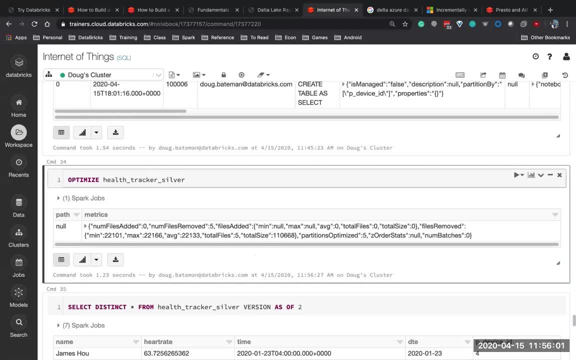 to do your etl and then you're going to run, optimize, run, optimize, run, optimize so that people who are querying the, so that people who are querying the, so that people who are querying the tables are querying optimized versions. tables are querying optimized versions. tables are querying optimized versions of those tables. 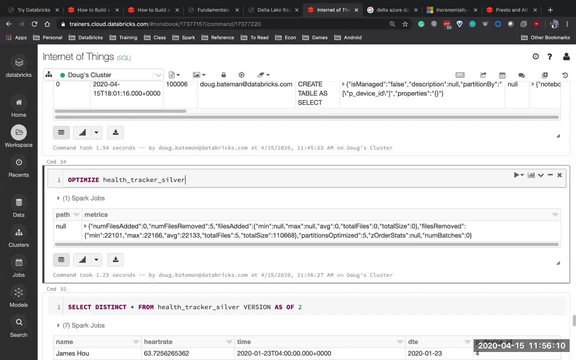 so optimize when you're complete with, so optimize when you're complete with, so optimize when you're complete with your etl, your etl, your etl. i wouldn't optimize every step in the. i wouldn't optimize every step in the. i wouldn't optimize every step in the middle of my etl, because you're wasting. 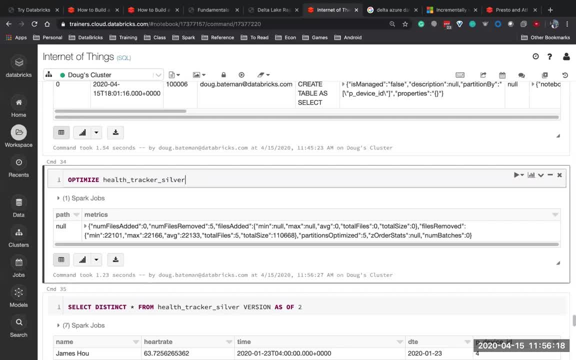 middle of my etl because you're wasting middle of my etl, because you're wasting time, time, time. the real goal of optimize is when you're. the real goal of optimize is when you're. the real goal of optimize is when you're done with your updates. 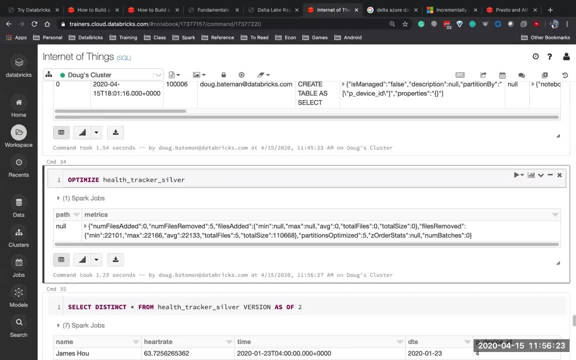 done with your updates, done with your updates, make it fast. and that would be the make it fast, and that would be the make it fast, and that would be the guidance that i would give you, guidance that i would give you guidance that i would give you. uh, somebody else asked: is time travel? 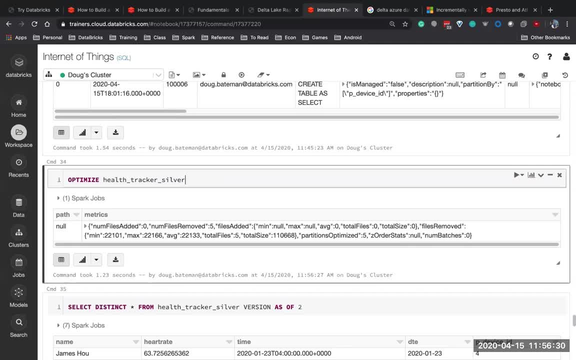 uh, somebody else asked: is time travel? uh, somebody else asked: is time travel only possible past one week? so time only possible past one week. so time only possible past one week. so time travel is possible. travel is possible. travel is possible as long as the old files are still. 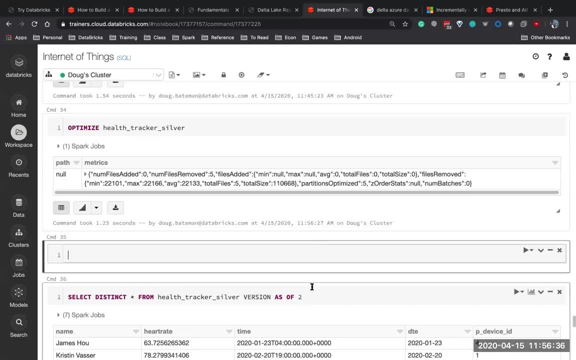 as long as the old files are still, as long as the old files are still around, around, around. so i will be able to time travel. so i will be able to time travel, so i will be able to time travel indefinitely backwards in time until, indefinitely backwards in time, until. 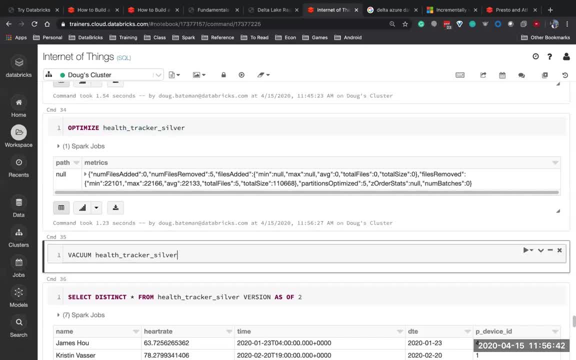 indefinitely backwards in time, until somebody vacuums up the old files. somebody vacuums up the old files, somebody vacuums up the old files. so when i run a vacuum statement, so when i run a vacuum statement, so when i run a vacuum statement and i'm deleting old files, that's when 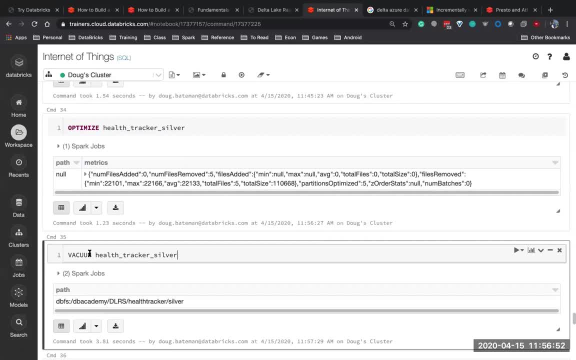 and i'm deleting old files. that's when and i'm deleting old files. that's when i can no longer. i can no longer. i can no longer access old versions now vacuum by default- access old versions- now vacuum by default. access old versions- now vacuum by default is going to retain things that are. is going to retain things that are is going to retain things that are newer than a week. so it only is going to newer than a week. so it only is going to newer than a week. so it only is going to get rid of versions. get rid of versions. get rid of versions older than one week by default. older than one week by default. older than one week by default, and my data has nothing that's older by, and my data has nothing that's older by, and my data has nothing that's older by one week. so you'll notice that i'm still. 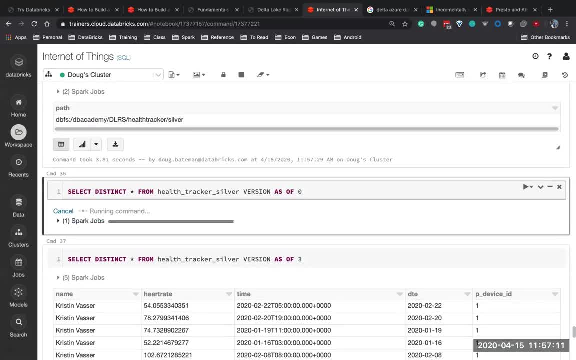 one week, so you'll notice that i'm still one week, so you'll notice that i'm still able to time travel all the way back, to able to time travel all the way back, to able to time travel all the way back to version zero. version zero. 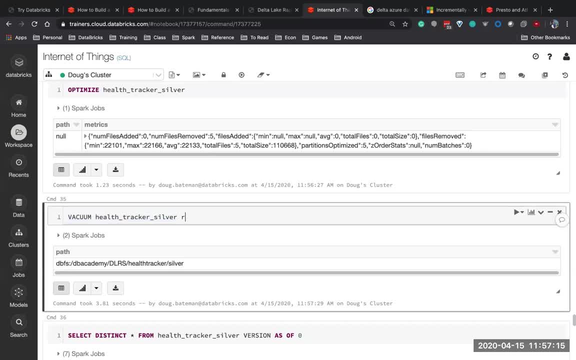 version zero now if i never ran the vacuum command now, if i never ran the vacuum command now, if i never ran the vacuum command, or if i set the retention period, or if i set the retention period, or if i set the retention period to be a year. 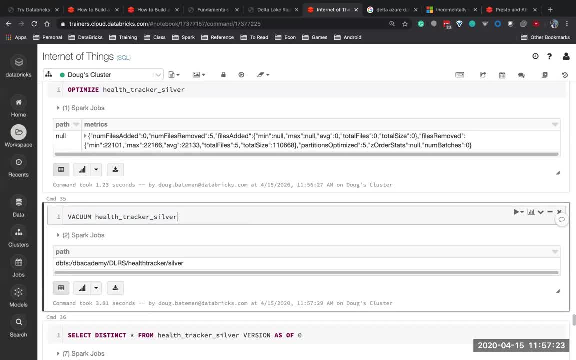 to be a year to be a year and you can tweak the retention period. and you can tweak the retention period of the vacuum command. if i said no, i of the vacuum command. if i said no, i of the vacuum command. if i said no, i want to be able to keep stuff for a year. want to be able to keep stuff for a year. want to be able to keep stuff for a year, then it won't delete those files, and then it won't delete those files, and then it won't delete those files and i'm able to time travel further back. 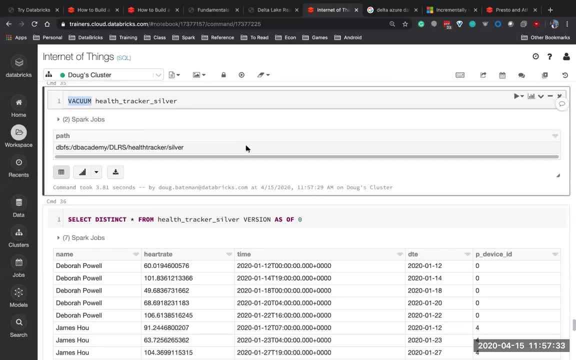 i'm able to time travel further back. i'm able to time travel further back, but time travel once you vacuum and the but time travel once you vacuum and the but time travel once you vacuum and the old files are deleted. old files are deleted, old files are deleted. you're no longer able to go that far back. you're no longer able to go that far back. you're no longer able to go that far back. so if i was to lower the retention, so if i was to lower the retention, so if i was to lower the retention period from a week down to a couple of, 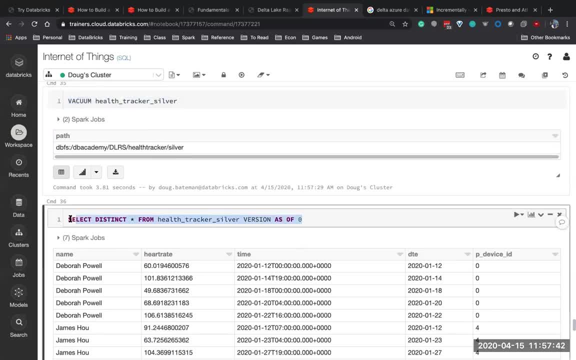 period from a week down to a couple of period, from a week down to a couple of hours, hours, hours. i would in fact get rid of old versions. i would in fact get rid of old versions. i would in fact get rid of old versions, and that's something that we're going to. 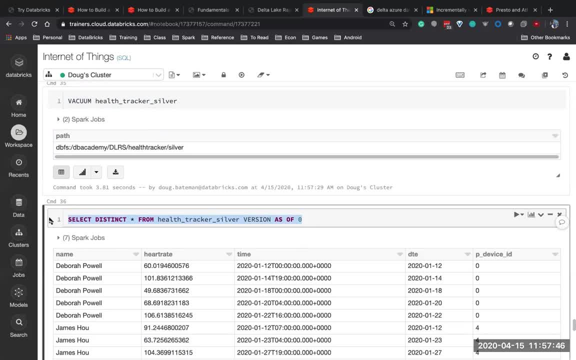 and that's something that we're going to, and that's something that we're going to do as part of gdpr compliance. do as part of gdpr compliance, do as part of gdpr compliance. so in in the next session, i'm actually. so in in the next session, i'm actually. 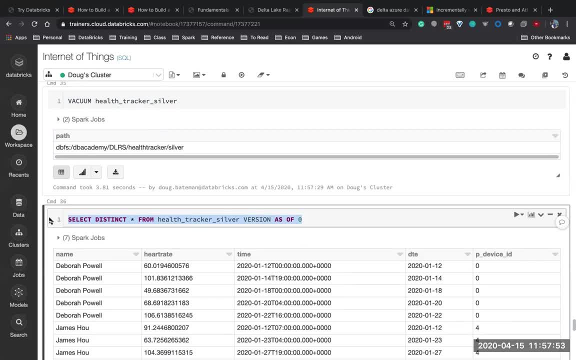 so in in the next session, i'm actually going to use the vacuum command, to going to use the vacuum command, to going to use the vacuum command to intentionally, intentionally, intentionally clean out old copies of the data. so clean out old copies of the data. so clean out old copies of the data so that i can tell the customer that i 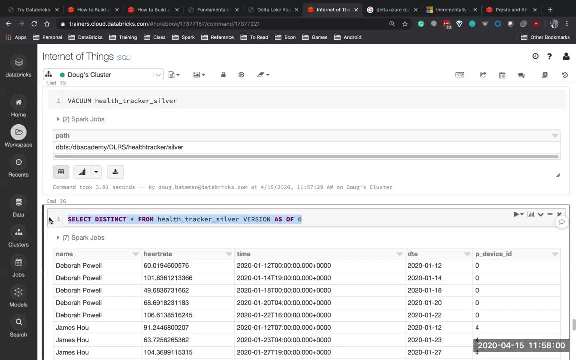 that i can tell the customer that i, that i can tell the customer that i truly have expunged, truly have expunged, truly have expunged their information from our system as part, their information from our system as part, their information from our system as part of. 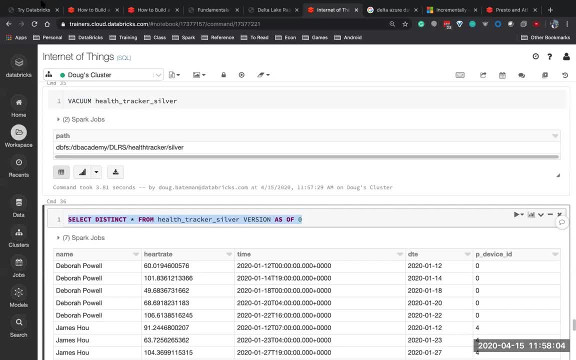 of of the european privacy regulations. now i'll um, i'm a lot asked. isn't the- now i'll um i'm a lot asked? isn't the- now i'll um, i'm a lot asked? isn't the number of files based on the number of number of files based on the number of? 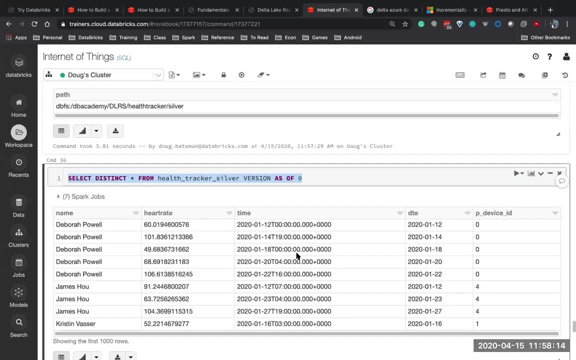 number of files based on the number of partitions, and the answer is yes, partitions, and the answer is yes, partitions, and the answer is yes. you'll remember initially after i did, you'll remember initially after i did, you'll remember initially after i did that merge, i had 1 000 files. 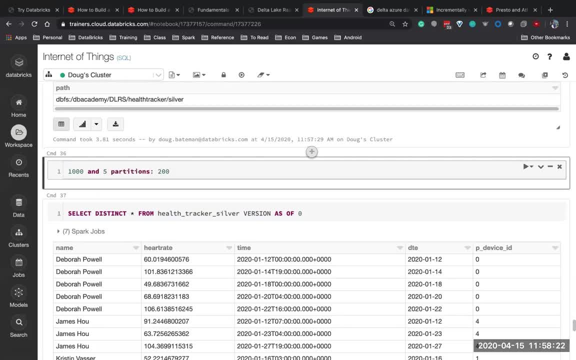 that merge. i had 1 000 files that merge. i had 1 000 files and five partitions. that meant i really and five partitions. that meant i really and five partitions. that meant i really had 200 files in each partition, had 200 files in each partition. 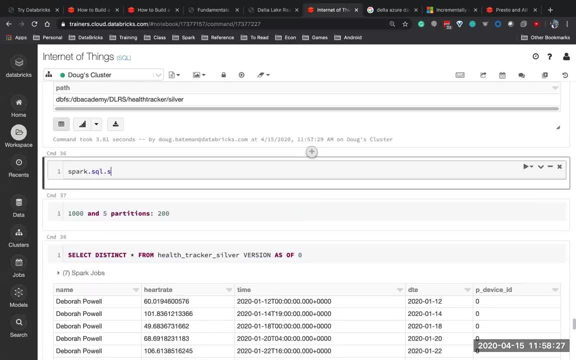 had 200 files in each partition. where did that 200 number come from? and where did that 200 number come from and where did that 200 number come from? and the answer it was that sparksql. the answer it was that sparksql. the answer it was that sparksql. shufflepartitions. 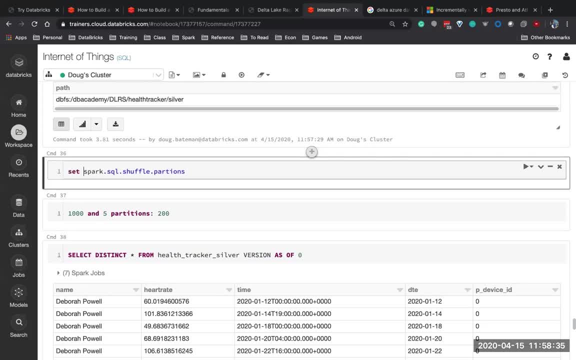 shufflepartitions. shufflepartitions or num partitions they'd have to look up, or num partitions they'd have to look up, or num partitions they'd have to look up. um as 200, so each partition had gotten um as 200, so each partition had gotten. 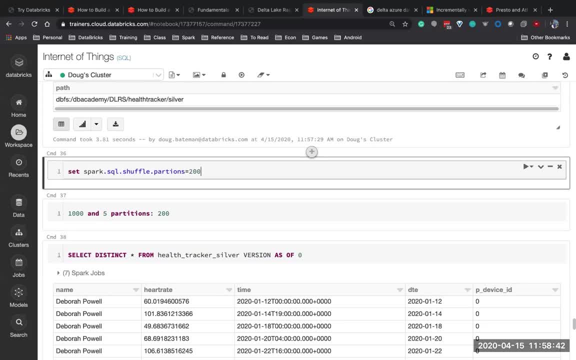 um as 200. so each partition had gotten 200 files. because it was a short, 200 files. because it was a short, 200 files, because it was a short operation, involved in my merge operation, involved in my merge operation, involved in my merge, and it had to shuffle the data. so five: 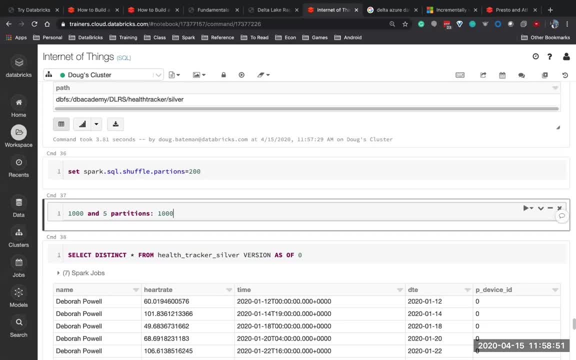 and it had to shuffle the data, so five. and it had to shuffle the data, so five. times 200 gave me the thousand files. times 200 gave me the thousand files. times 200 gave me the thousand files. and i really only wanted five files and i really only wanted five files. 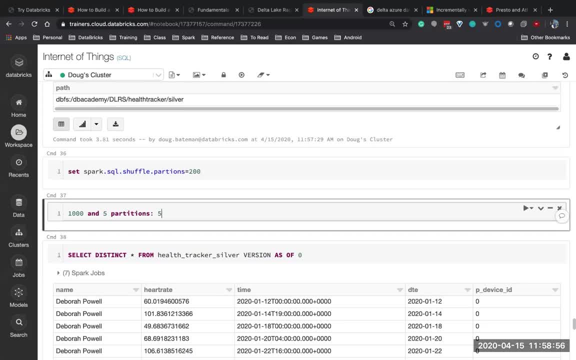 and i really only wanted five files because they were small, so i used. because they were small, so i used. because they were small, so i used optimize to compress them back down. optimize to compress them back down. optimize to compress them back down to be a smaller number again. 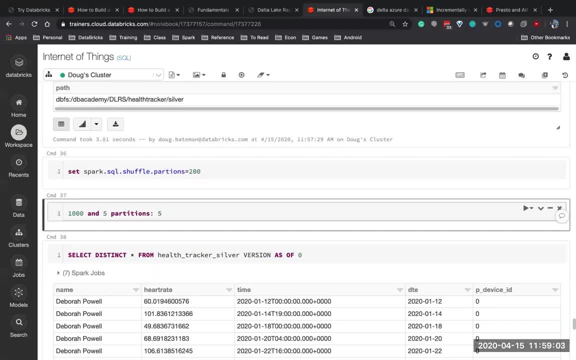 to be a smaller number again, to be a smaller number again, but each partition will have a minimum, but each partition will have a minimum, but each partition will have a minimum of one file and a maximum could be of one file, and a maximum could be of one file and a maximum could be thousands of files. and so what optimize? 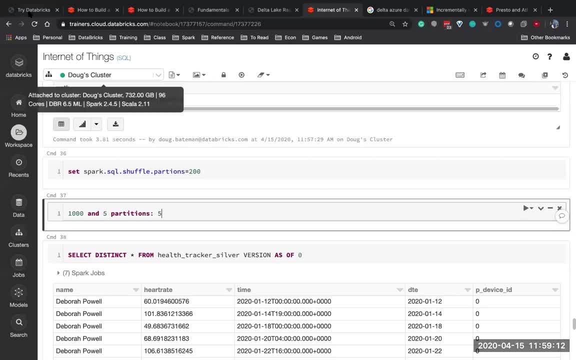 thousands of files. and so what? optimize thousands of files. and so what optimize did? is it grouped files within a did? is it grouped files within a did? is it grouped files within a partition? so somebody else asked: how do you do so? somebody else asked: how do you do?